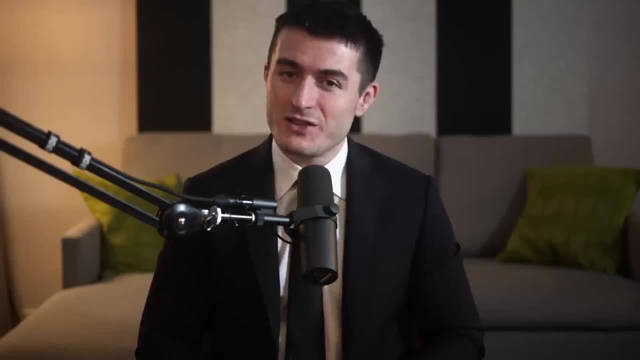 This was in 1994 at the legendary MIT leg lab. He wrote his PhD thesis on robot gymnastics, as part of which he was a professor at the University of Michigan. He was a professor at the MIT And he's of the original software for robot dynamics. he programmed a bipedal robot to do the 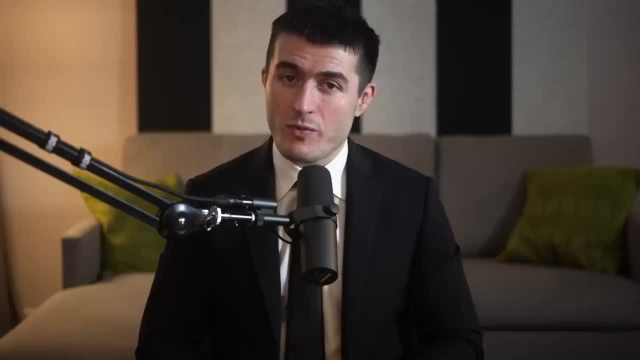 world's first three D robotics. somersault Robert is a great engineer, robotic system leader, and Boston Dynamics, to me as a roboticist, is a truly inspiring company. This conversation was a big honor and pleasure and I hope to do a lot of great work these. 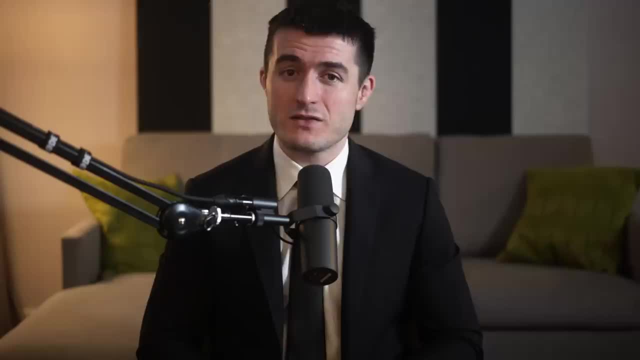 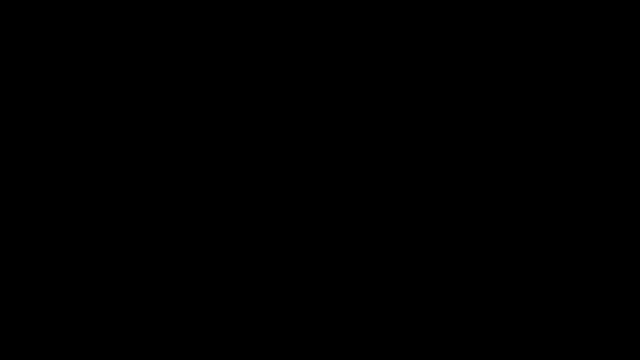 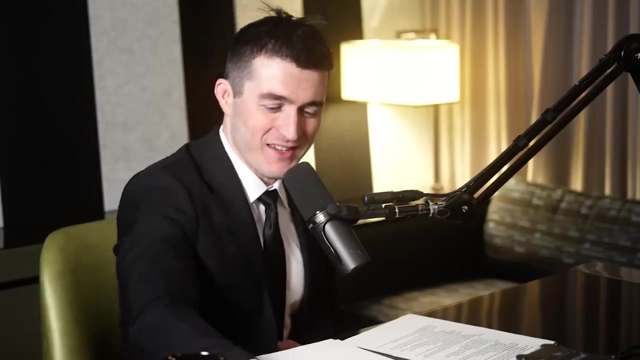 robots in the years to come. This is the Lex Friedman podcast. to support it, Please check out our sponsors in the description. And now, dear friends, Here's Robert Plater. When did you first fall in love with robotics? Let's start with love and robots. 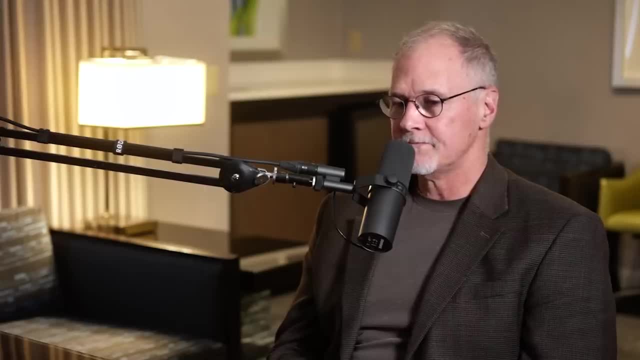 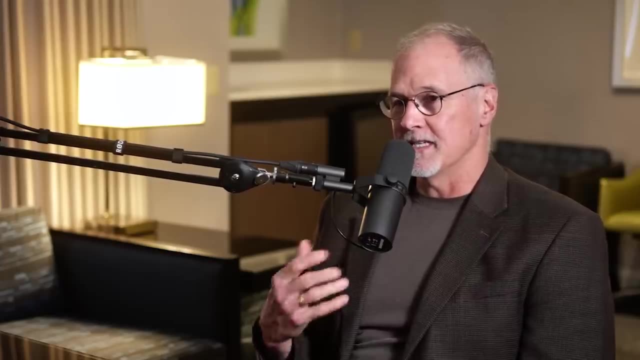 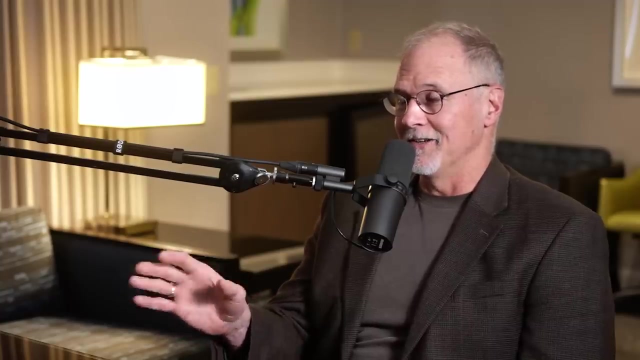 Well, love is relevant because I think the fascination, the deep fascination, is really about movement. And I was visiting MIT looking for a place to get a PhD and I wanted to do some laboratory work And one of my professors in the aero department said: 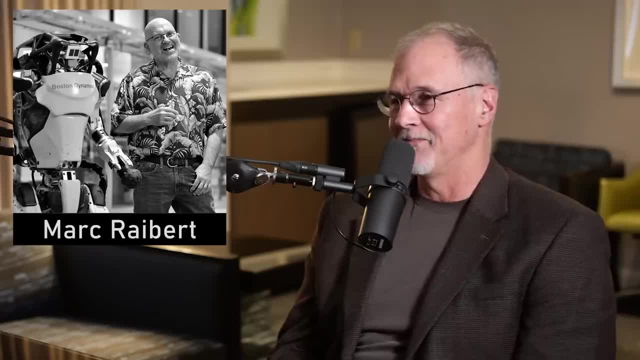 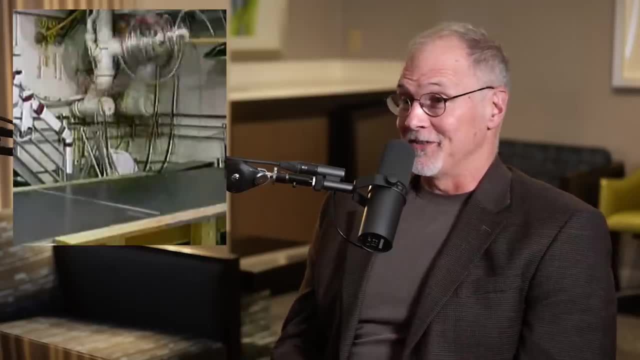 go see this guy, Mark Raybert, down in the basement of the AI lab, And so I walked down there and saw him. He showed me his robots and he showed me this robot doing a somersault And I just immediately went: whoa, you know. 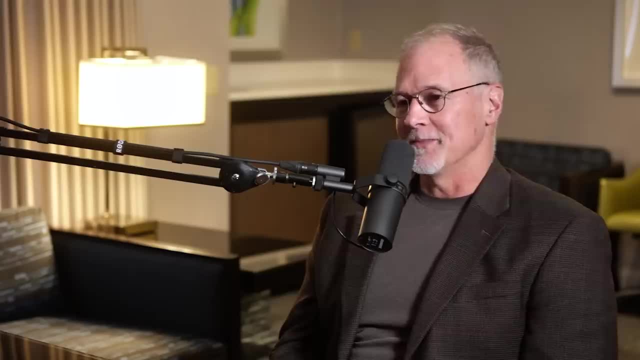 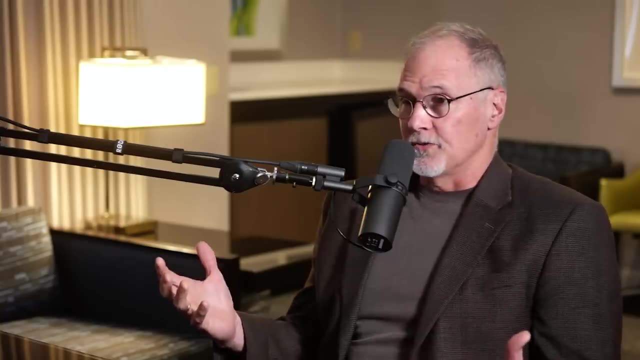 Robots can do that And because of my own interest in gymnastics, there was like this immediate connection And you know I was interested in- I was in an aero-astro degree- because you know, flight and movement was all so fascinating to me. 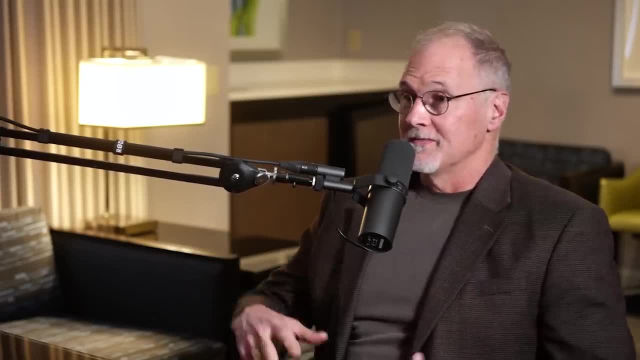 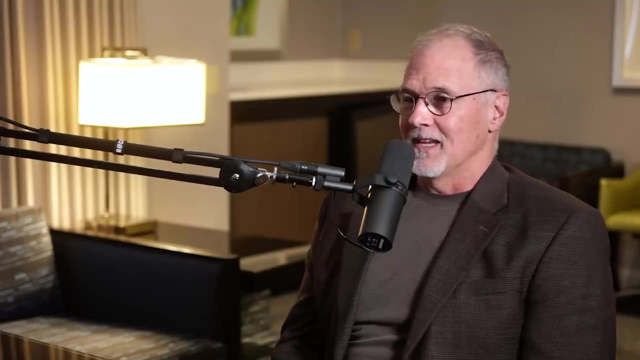 And then it turned out that you know, robotics had this big challenge: How do you balance, How do you build a legged robot that can really get around, And that, just that was a fascination, And it still exists today. We're still working on perfecting motion in robots. 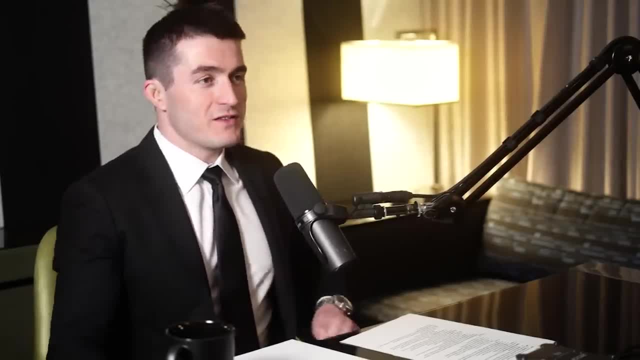 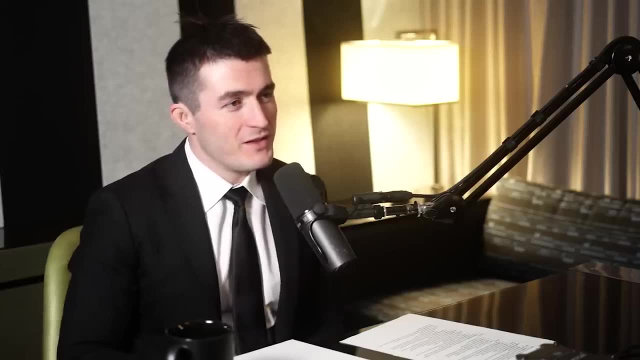 What about the elegance and the beauty of the movement itself? Is there something maybe grounded in your appreciation of motion, movement from your gymnastics days? Did you? was there something you just fundamentally appreciated about the elegance and beauty of movement? You know we had this concept in gymnastics. 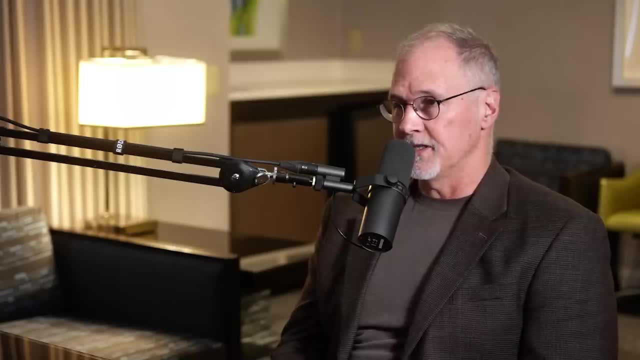 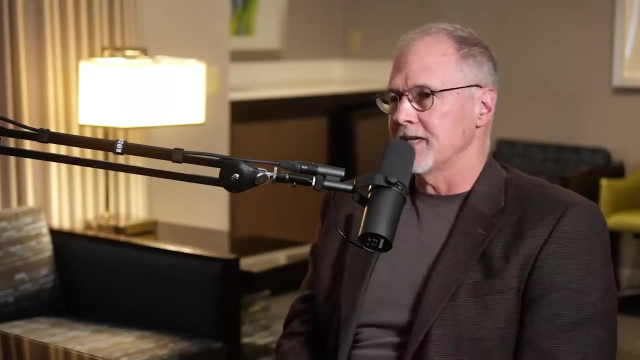 of letting your body do what it wanted to do. When you get really good at gymnastics, part of what you're doing is putting your body into a position where the physics and the body's inertia and momentum will kind of push you in the right direction. 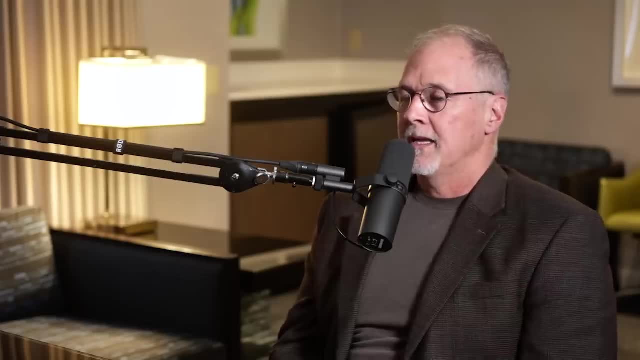 In a very natural and organic way, And the thing that Mark was doing, you know, in the basement of that laboratory, was trying to figure out how to build machines to take advantage of those ideas. How do you build something so that the physics of the machine? 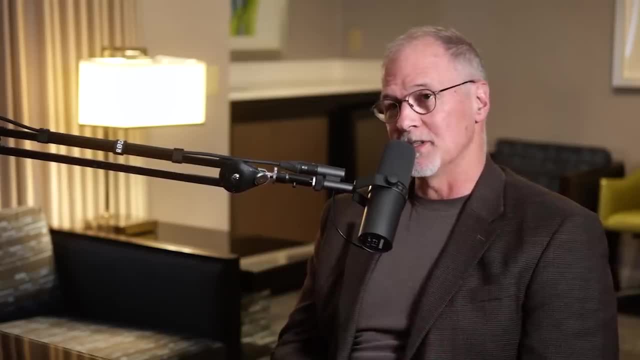 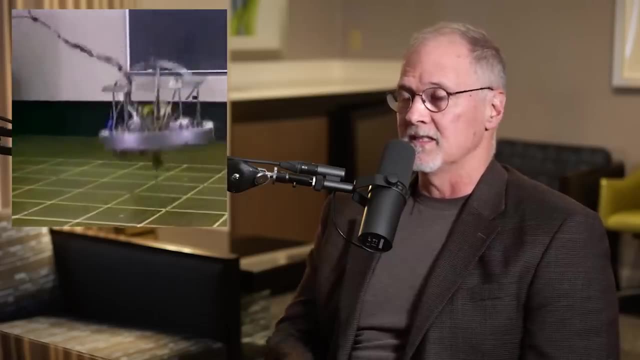 just kind of inherently wants to do what it wants to do And he was building these springy pogo stick type. you know, his first cut at legged locomotion was a pogo stick, where it's bouncing And there's a spring mass system. 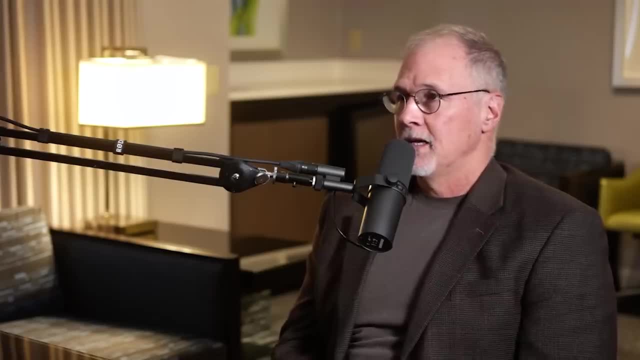 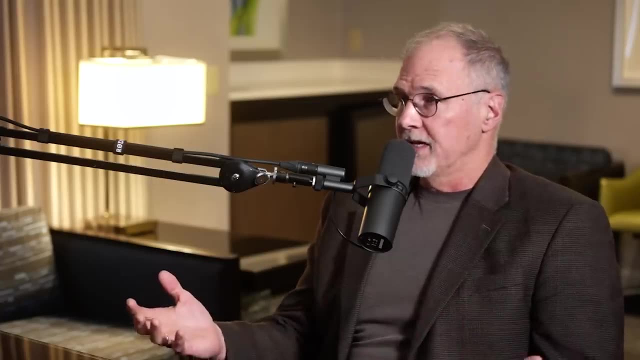 That's awesome. It's kind of oscillating, has its own sort of natural frequency there And sort of figuring out how to augment those natural physics with also intent: How do you then control that but not overpower it? It's that coordination that, I think, creates real potential. 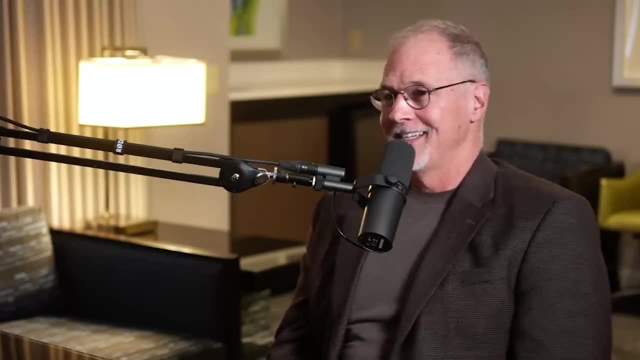 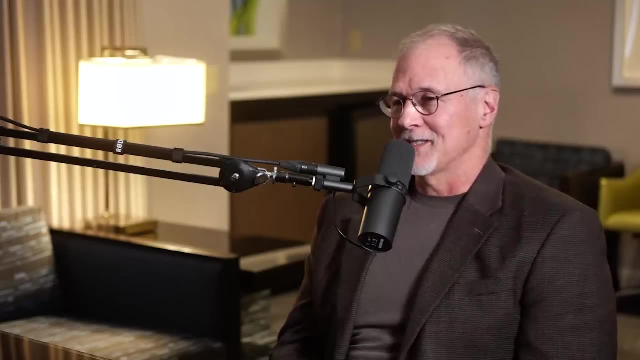 We could call it beauty, You know. you could call it- I don't know- synergy- People have different words for it, But I think that that was inherent from the beginning. That was clear to me, that that's part of what Mark was trying to do. 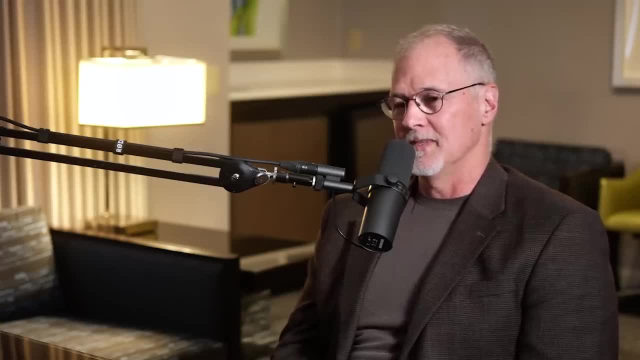 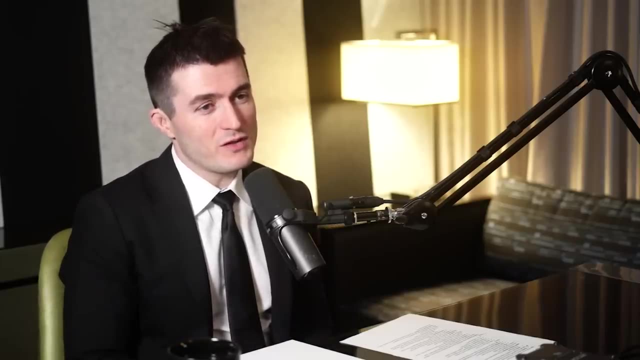 He asked me to do that In my research work, So you know that's where it got going. So part of the thing that I think I'm calling elegance and beauty in this case- which was there even with the pogo stick- is maybe the efficiency. 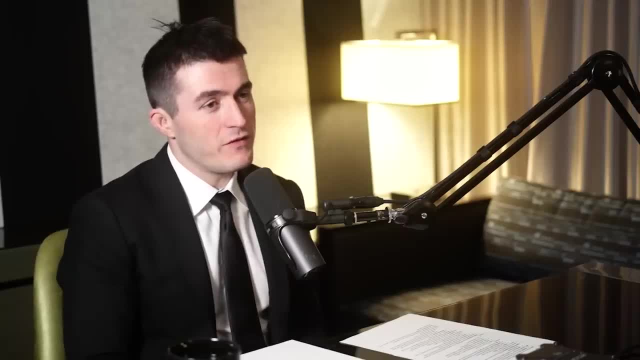 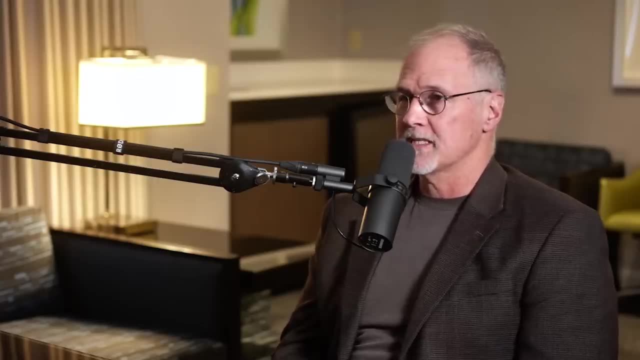 So letting the body do what it wants to do, Trying to discover the efficient movement, It's definitely more efficient. It also becomes easier to control in its own way, because the physics are solving some of the problem itself. It's not like you have to do all this calculation and overpower the physics. 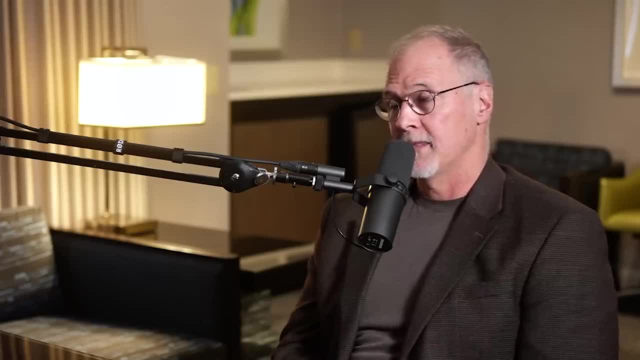 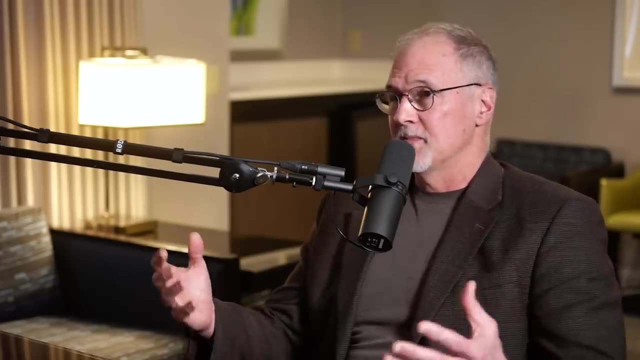 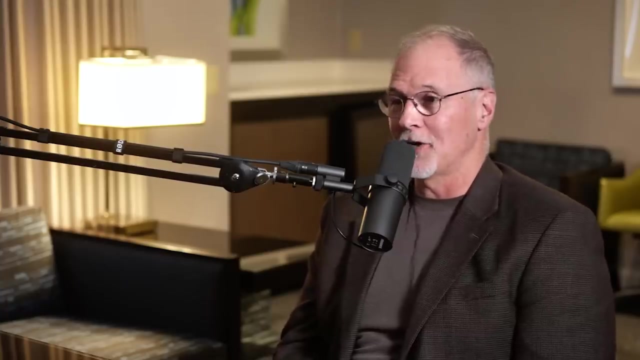 The physics Naturally, inherently, want to do the right thing. There can even be, you know, feedback mechanisms, stabilizing mechanisms that occur simply by virtue of the physics of the body. And it's not all, not all in the computer or not even all in your mind as a person. 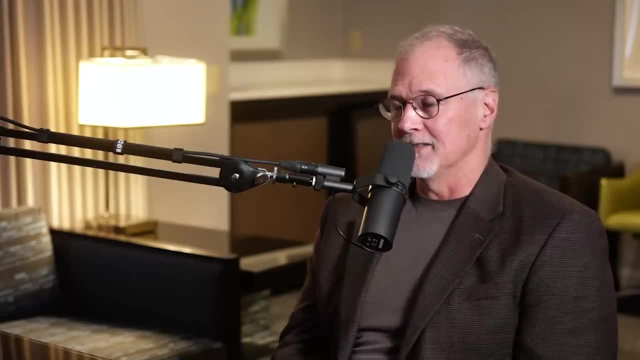 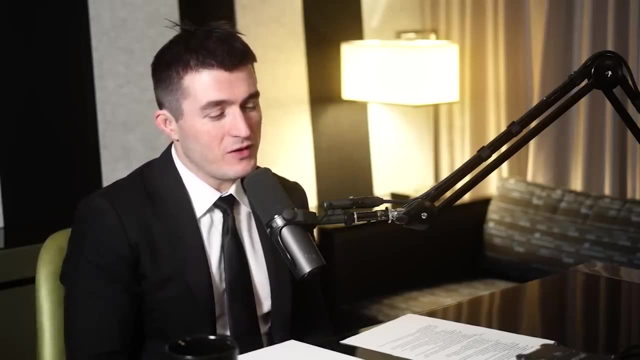 And I. there's something interesting in that that melding. You were with Mark for many, many, many years, but you were there in this kind of legendary space of uh leg lab and MIT in the in the basement. all great things happen in the basement. 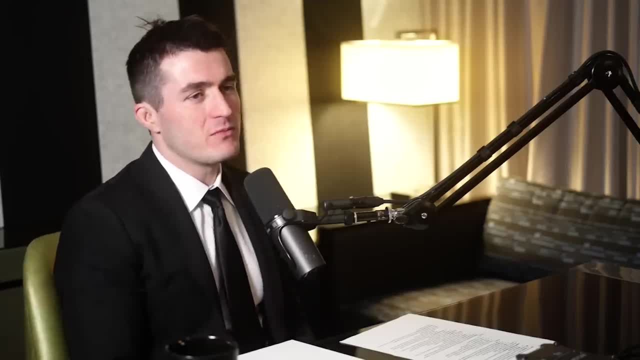 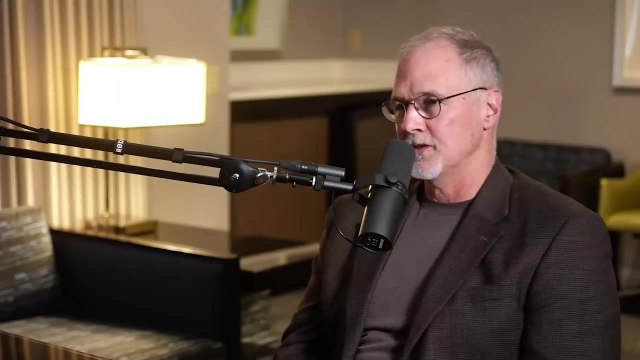 Is there some memories? uh, is there some memories from that time that you have Because it's so? it's such cutting edge work in in in robotics and artificial intelligence. The memories, the distinctive lessons I would say I learned in that in that time period. 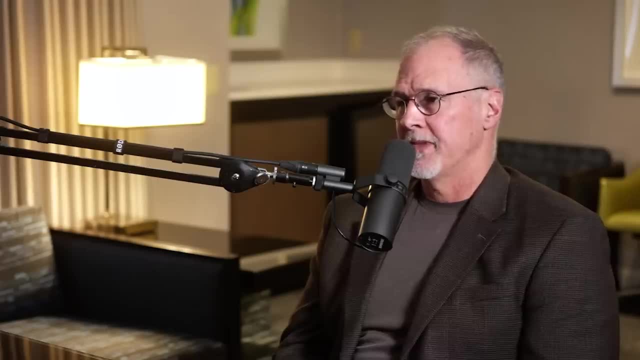 And um, and that I think Mark was a great teacher of was: uh, it's okay to pursue your interests, your curiosity. do something because you love it. Um, you'll do it a lot better if you love it. Um. that that is a lasting lesson that I think, uh, we apply at the company still. 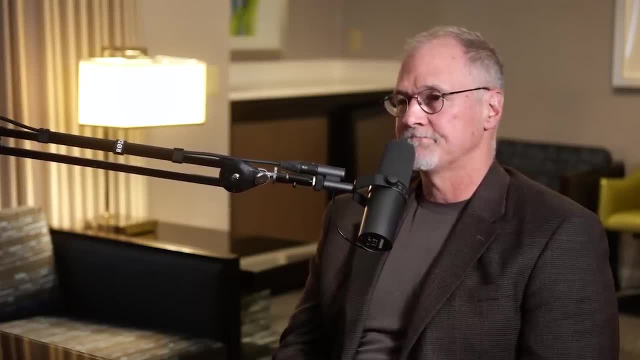 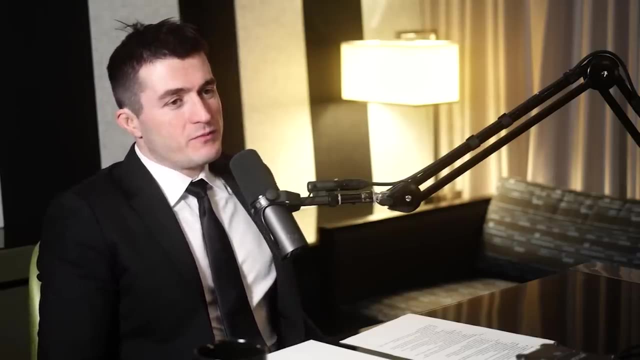 Um, and really is a core value. So the interesting thing is I got to um, uh with people like Ross, Cedric and um and others Like the students that work at those robotics labs are like some of the happiest people I've ever met. 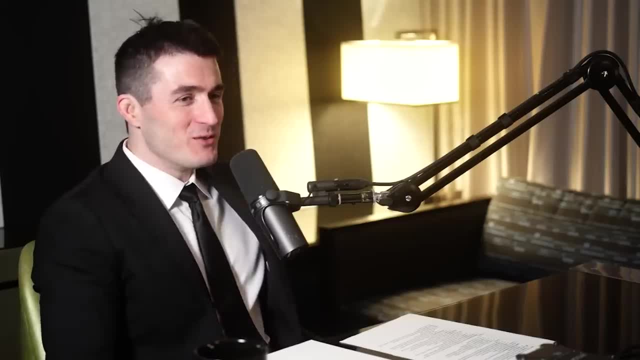 I don't know what that is. I meet a lot of PhD students. A lot of them are kind of broken by the wear and tear of the process. Uh, but roboticists are, while they work extremely hard and work long hours, there's um, uh, there's a happiness there. 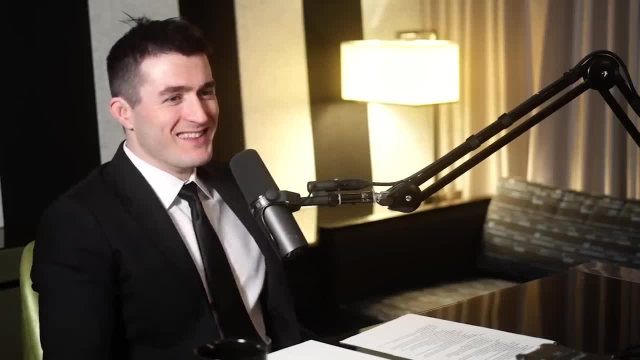 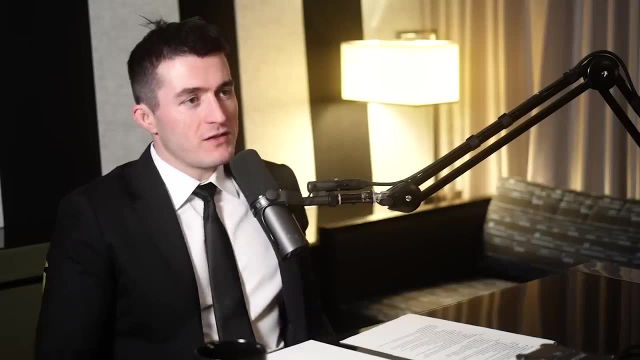 The only other group of people I've met like that are people that skydive a lot Like, for some reason, there's a deep fulfilling happiness, Maybe from, um, like a long period of struggle to get a thing to work and it works and there's a magic to it. 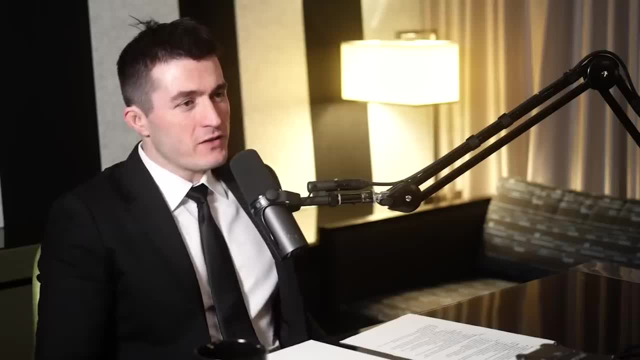 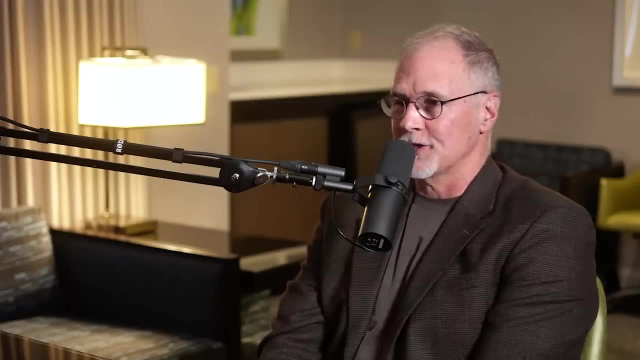 I don't know exactly, because it's so fundamentally hands-on and you're bringing a thing to life. I don't know what it is, but they're happy. We see, you know, our, our attrition at the company is really low. 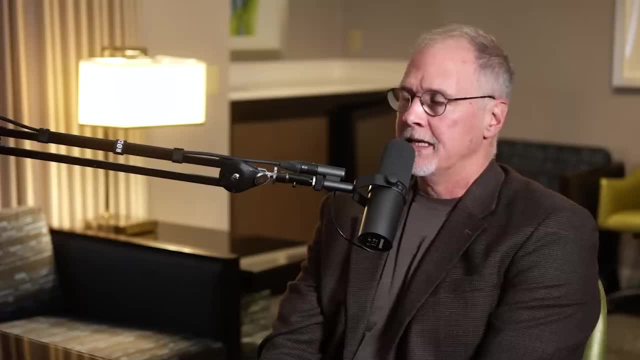 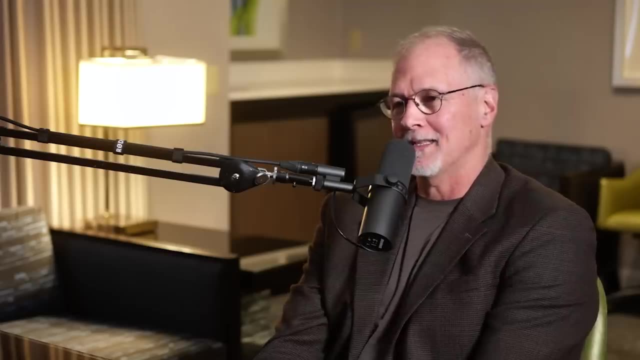 People come and they love the pursuit And I think part of that is that there's perhaps a natural connection to it. It's a little bit easier to connect when you have a robot that's moving around in the world And part of your goal. 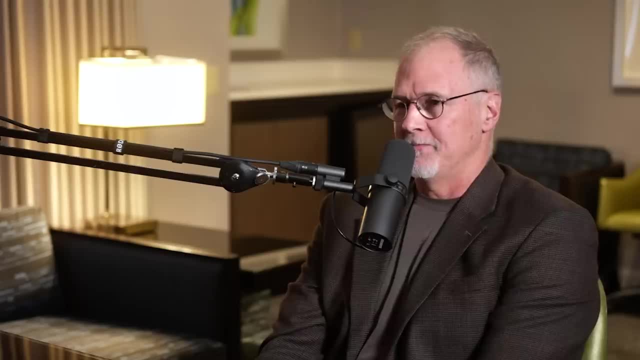 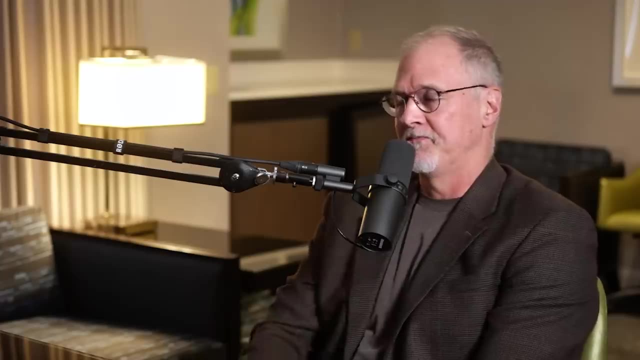 Is to make it move around in the world. You can identify with that And- and this is on a- this is one of the unique things about the kinds of robots we're building, is this physical interaction lets you perhaps identify with it. So I think that is a source of happiness. 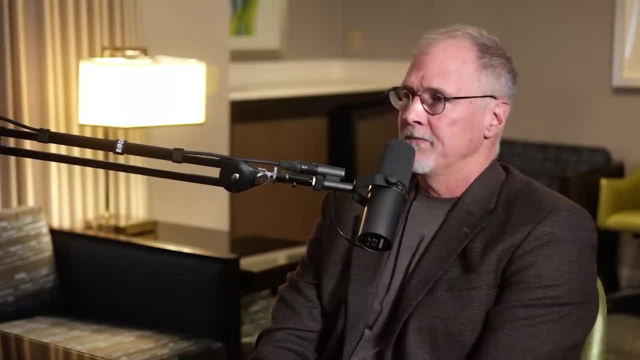 I don't think it's unique to robotics, I think anybody also- who is just pursuing something they love, it's easier to work hard at it and be good at it, And, um, not everybody gets to find that. Uh, I do. 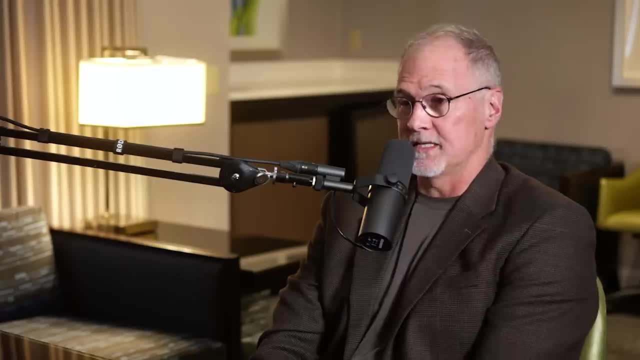 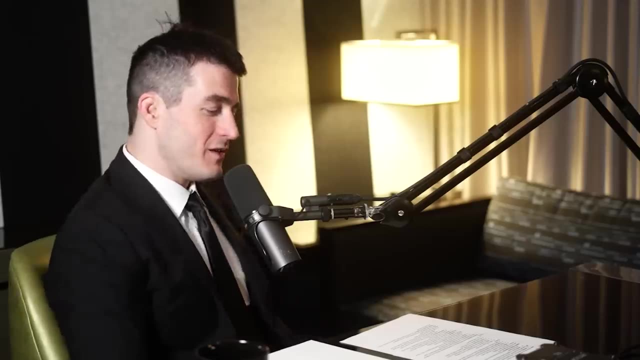 Feel lucky, uh, in that way, And I think, uh, we're lucky as an organization that we've been able to build a business around this and that keeps people engaged. So, if it's all right, let's linger on Mark for a little bit longer. Mark Raybert. 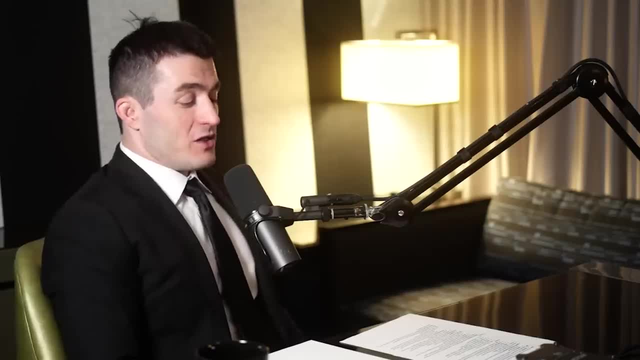 So he's a legend? Uh, he's a legendary engineer and roboticist. What, what have you learned about life, about robotics, from Mark through all the many years you worked with him? I think the most important lesson, which was: you know, have the courage of your convictions and and? 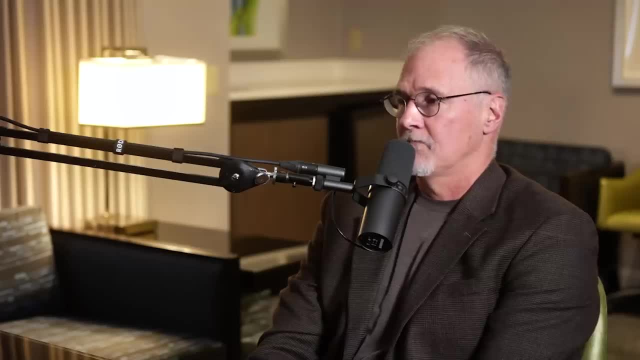 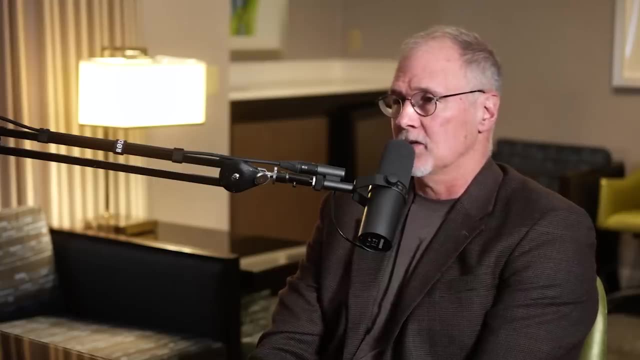 Do what you think is interesting? Um be willing to try to find big, big problems to go after And at the time you know, like at locomotion um, especially in a dynamic machine, nobody had solved it And that felt like a multi decade problem to go after. 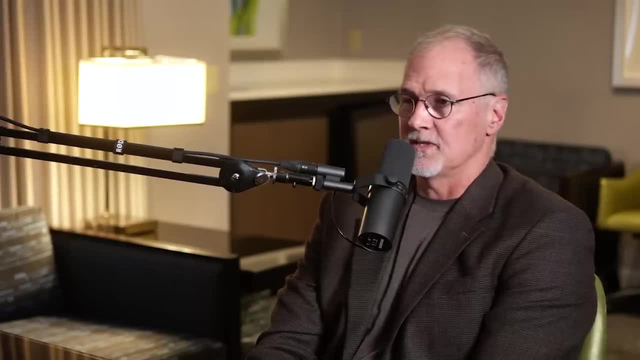 And so, you know, have the courage to go after that because you're interested. uh, don't worry if it's going to make money. you know that That's been um a theme, So that that's really, uh, probably the most uh, uh important lesson. 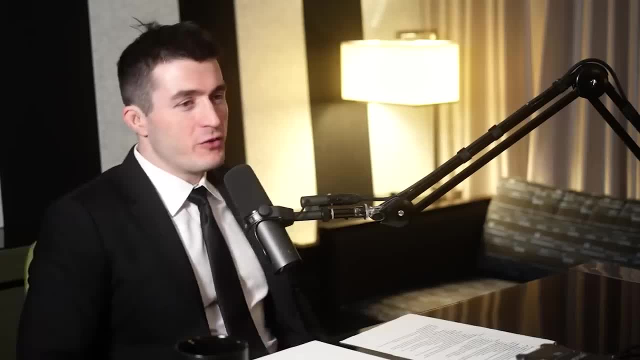 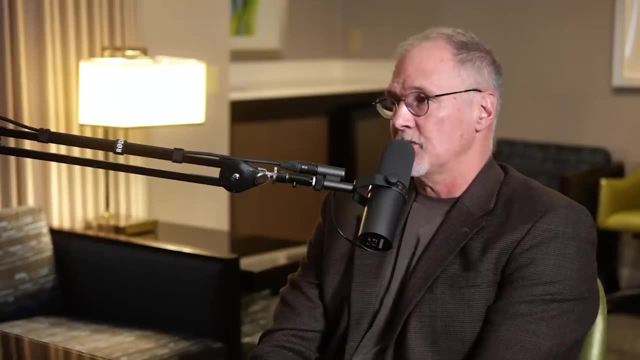 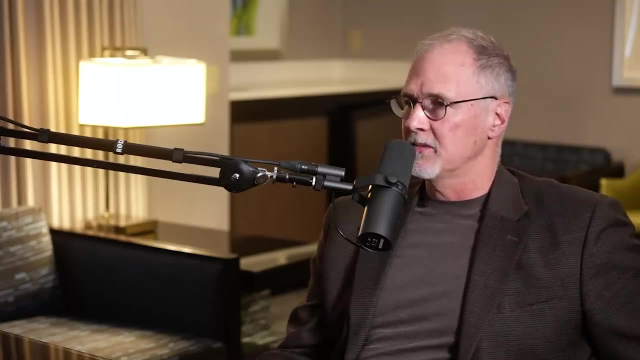 I think that, uh, I got from Mark. How crazy is the effort of doing legged uh robotics at that time especially, you know, Mark got some stuff to work, uh, starting from the simple ideas, So so maybe the other another important idea that has really become a value of the company is try to simplify a thing to the core essence. 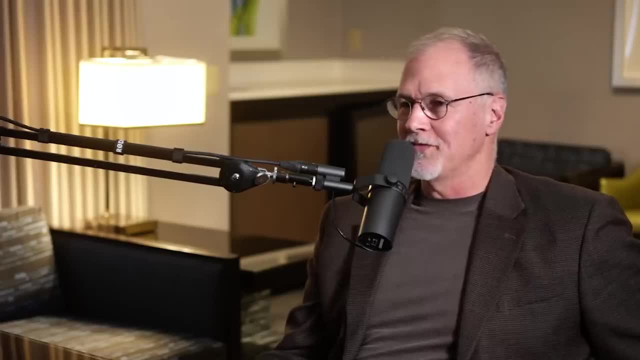 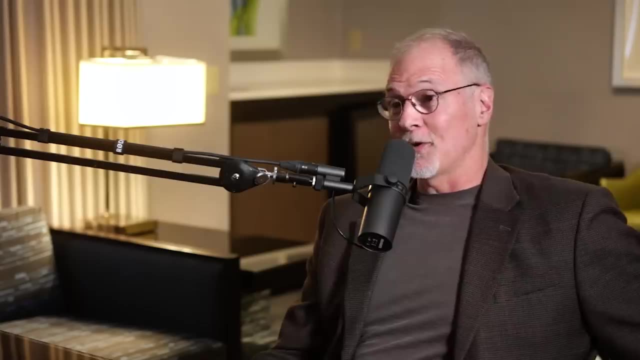 And, and. while you know, Mark was showing videos of animals running across the Savannah or uh uh, climbing mountains, what he started with was a pogo stick, because he was trying to reduce the problem to something that was manageable. and and and getting the pogo stick to balance. 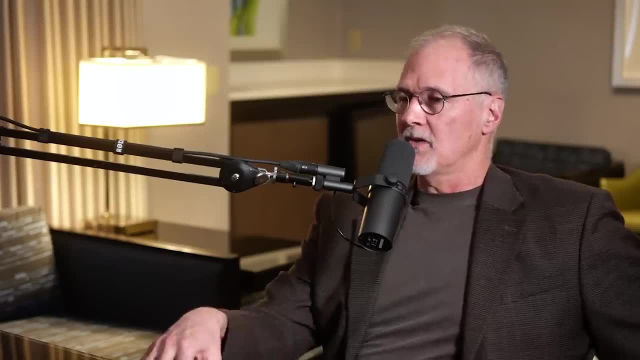 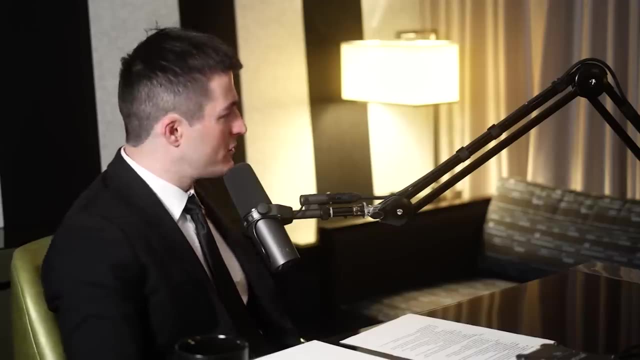 Had in it the fundamental problems that if we solve those, you could eventually extrapolate to something that galloped like a horse. And so look for those simplifying principles. Um, how, How tough is the job of simplifying a robot? 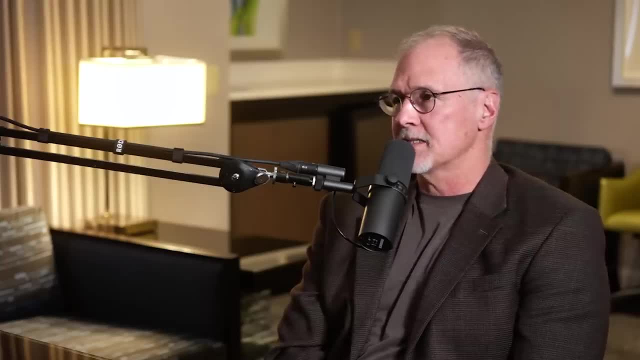 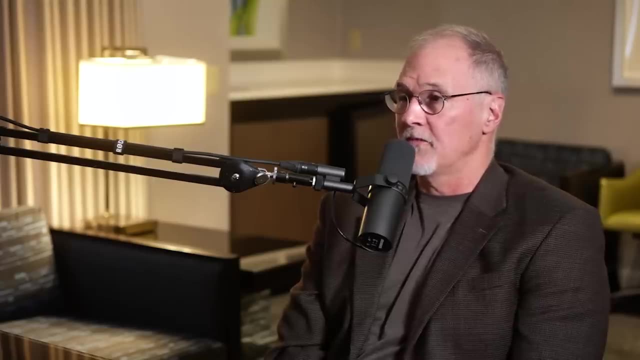 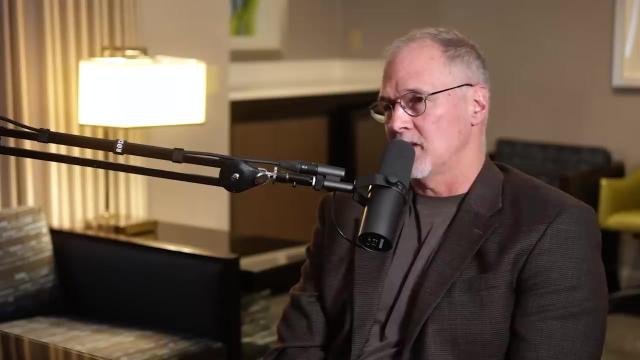 So I I'd say in the early days, the, the thing that made Boston, the researchers at Boston, dynamics special is that we, we worked on under figuring out what that, that central principle was, and then building software or machines around that principle. 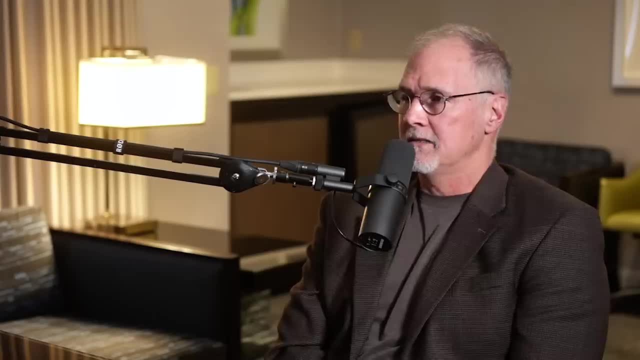 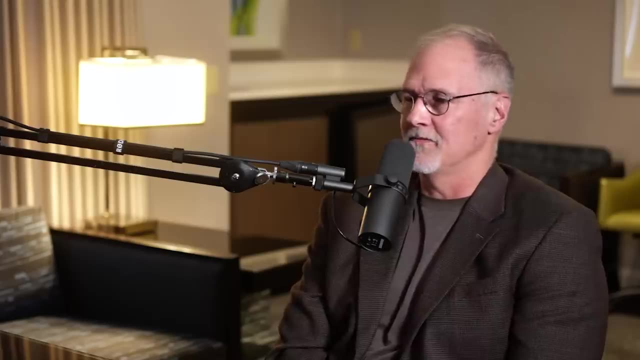 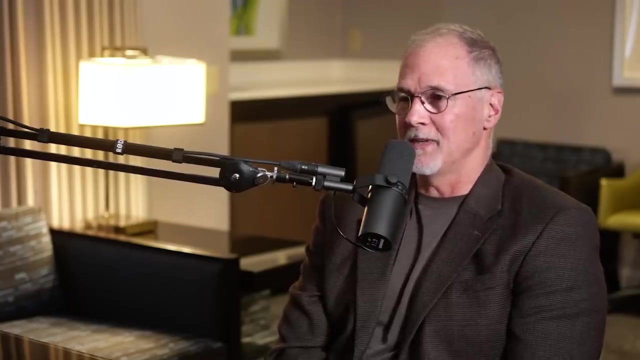 And that was not easy in the early days And and it it took um real expertise in understanding The dynamics of motion and feedback control principles, how to build an- you know, with the computers at the time, how to build a feedback control algorithm that was simple enough that it could run in real time at a thousand Hertz and actually get that machine to work. 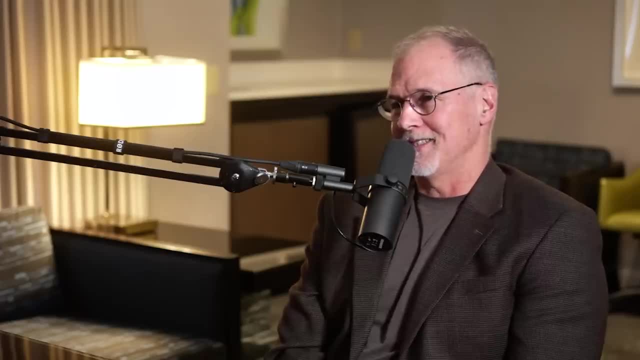 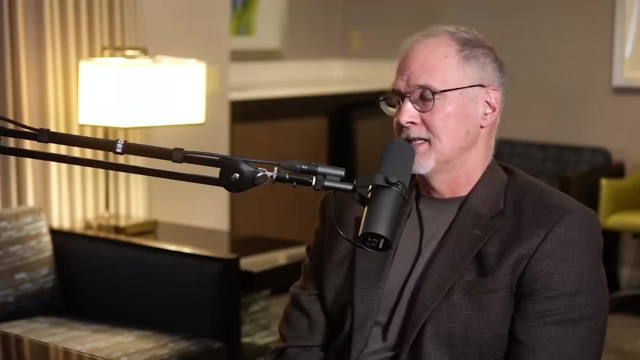 Um, and that was not something everybody was doing, you know, at that time. Now, the world's changing now, And I, I, I think the approaches to controlling robots are going to change, Um but Uh, and that they're going to become more broadly, um, available. 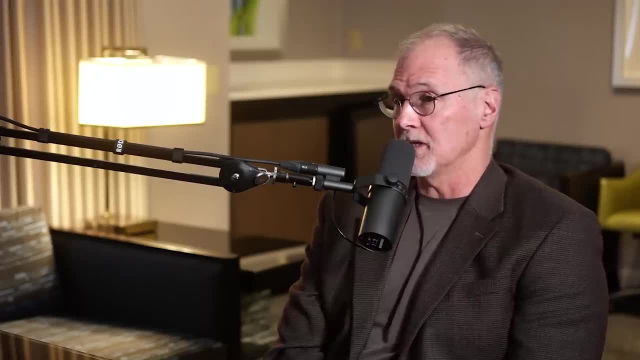 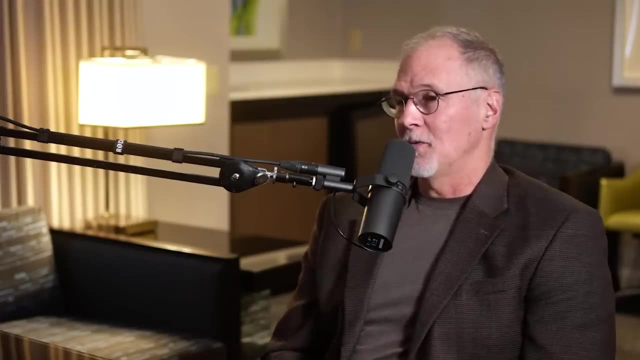 Um, but at the time there weren't many groups who could really sort of work at that principled level, uh, with both the software and and make the hardware work. And I'll, and I'll say one other thing about you were sort of talking about what are the special things? 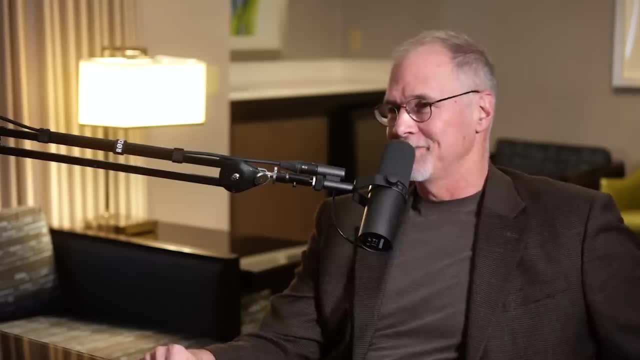 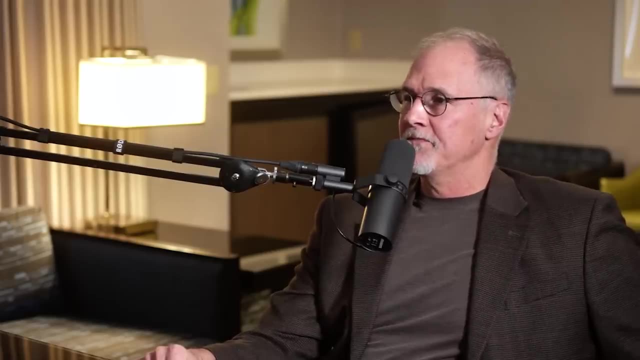 The other thing was: it's, it's, it's good to break stuff. you know um you know use the robots, Uh, break them, repair them, um you know, fix and repeat, test, fix and repeat. 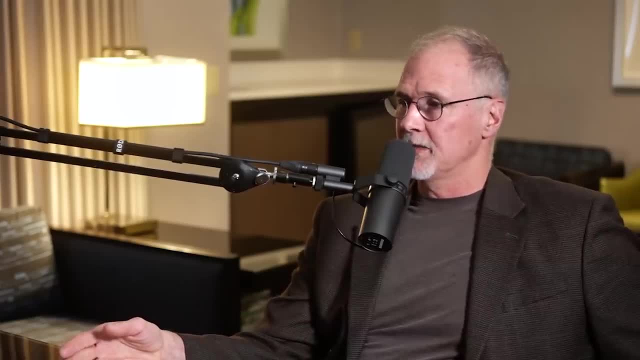 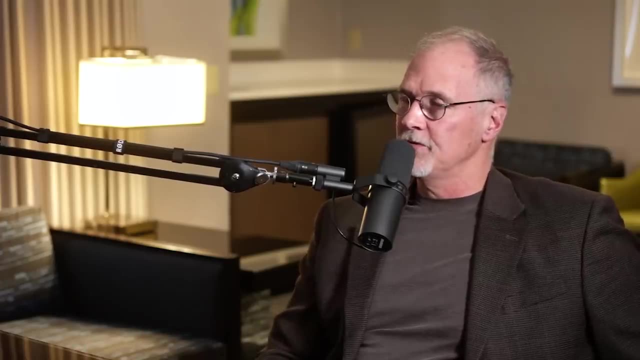 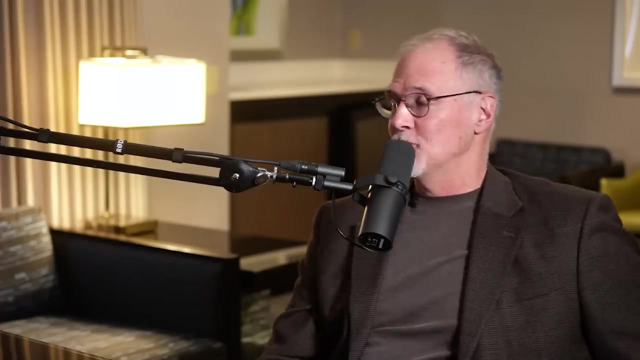 And that, and that's also a core principle that has become part of the company and it lets you be fearless in your work. too often, If you are working with a very expensive robot, maybe one that you bought from somebody else or that you don't know how to fix, then you treat it with kit gloves and you can't actually make progress. 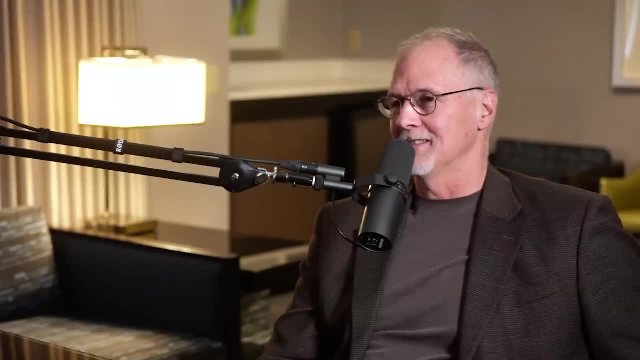 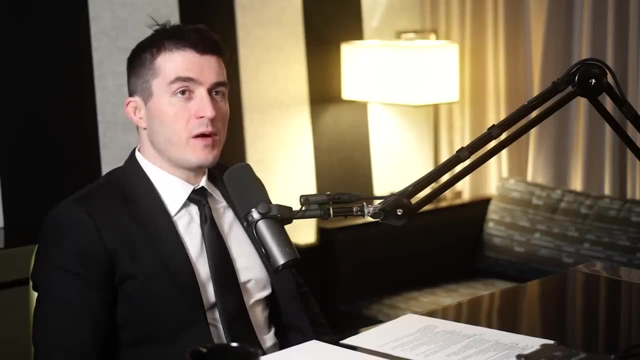 You have to be able to break something, And so I think that's uh been a uh a principle as well. So, just to linger on that, psychologically, how do you deal with that Cause? I remember I had, uh, uh, I built a RC car with that. 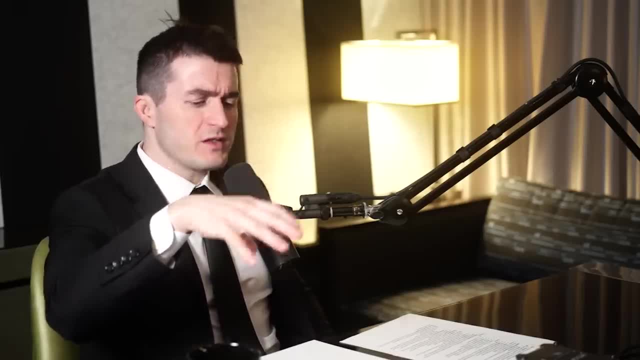 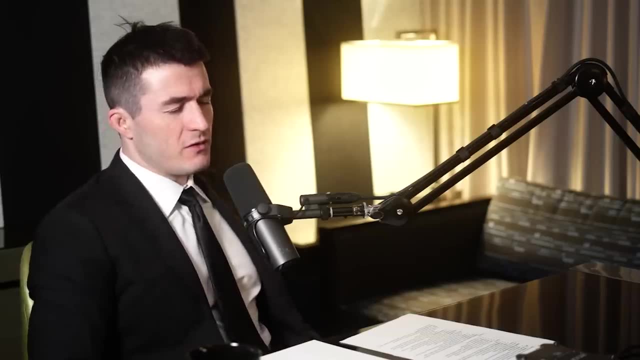 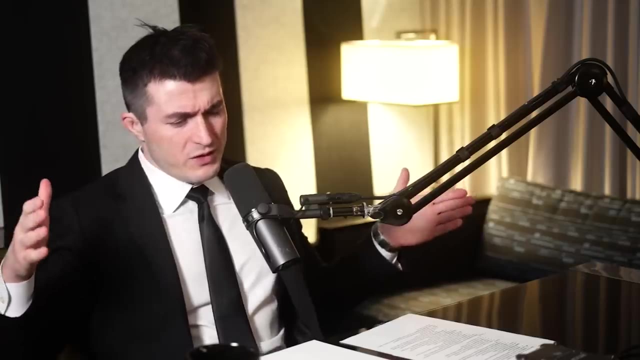 Some uh had some custom stuff like compute on it and all that kind of stuff, cameras And uh, because I didn't sleep much, the code I wrote had an issue where it didn't stop the car and the car got confused and at full speed at like 20, 25 miles an hour. 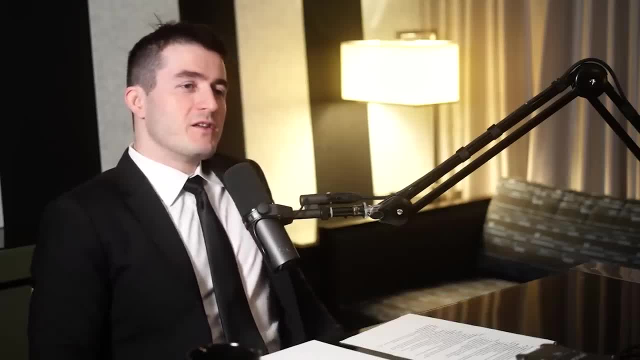 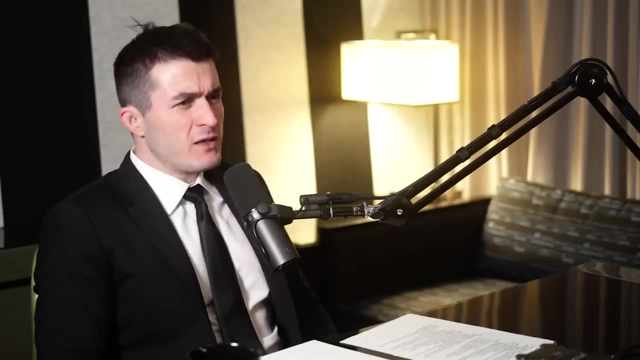 So, And I just remember sitting there alone in a deep sadness, um sort of full of regret, I think, almost anger, um, uh, but also like sadness because you think about, well, these robots, especially for autonomous vehicles, like like you should be taking safety very seriously even in these kinds of things. but just no, no good feelings. 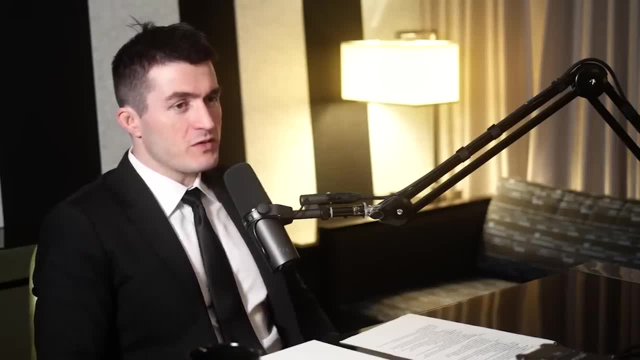 Um, and made me more afraid, probably, to do this kind of experiment. Um, and made me more afraid, probably, to do this kind of experiment In the future. perhaps the right way to have seen that is positively like it's it's too. 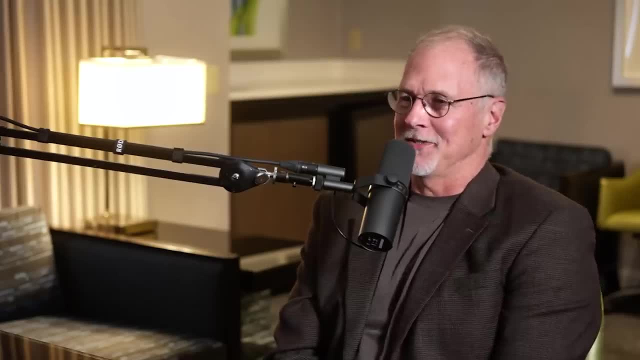 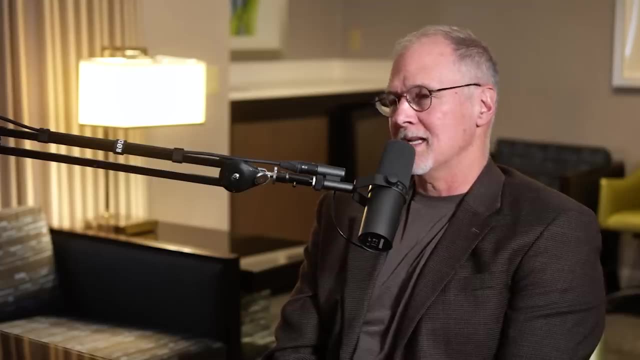 It depends if you could have built that car or, or, or just gotten another one right. That would have been the approach. Um, I remember um, when I got to grad school, um, you know, I got some training about um operating a lathe and a mill up in the machine shop and I could start to make my own parts. 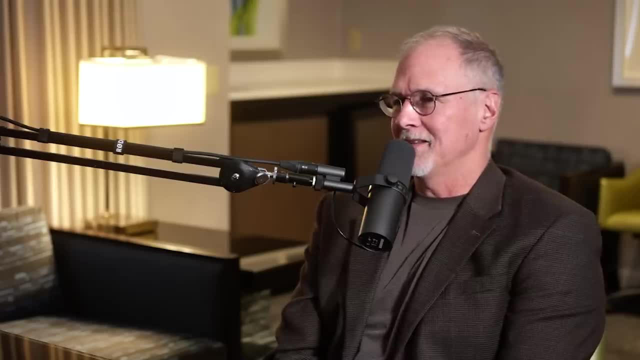 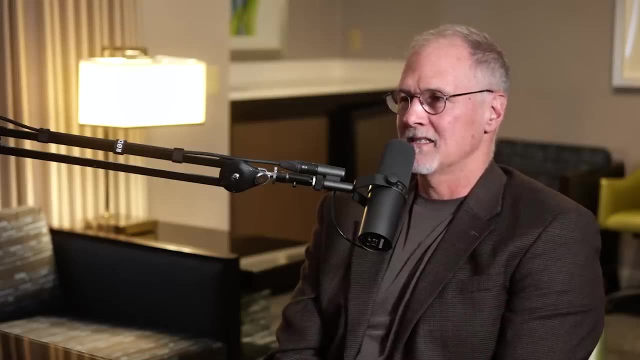 And I remember breaking some pieces Of equipment in the lab and then realizing, cause I, maybe this was a unique part and I couldn't go buy it. And I realized, oh, I can just go make it. That was an enabling feeling. 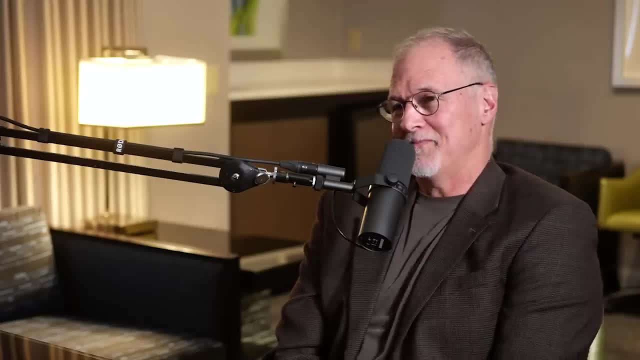 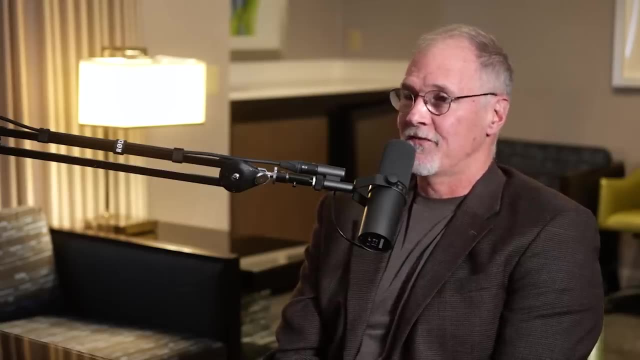 Yeah, Then you're not afraid. Yeah, It might take time. It might take more work than you thought it was going to be required to get this thing done, but you can just go make it, And that's freeing in a way that nothing else is. 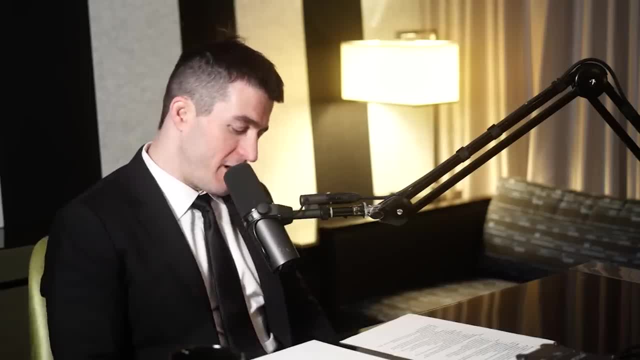 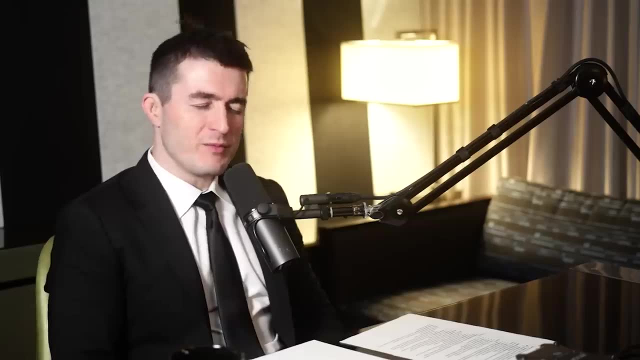 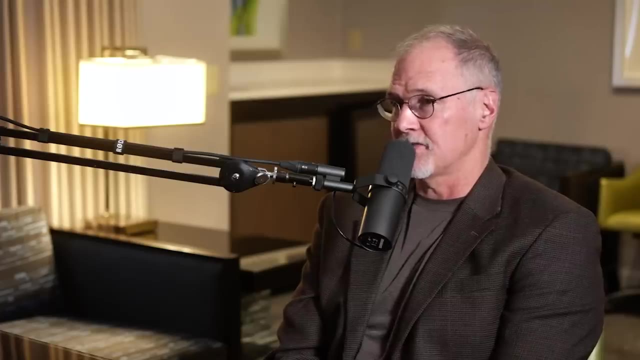 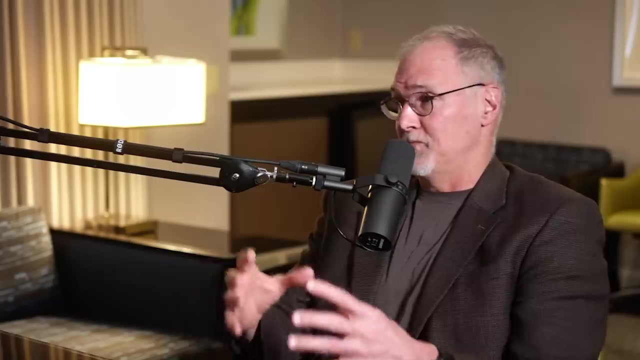 You mentioned, uh, the feedback control, The dynamics. sorry for the romantic question, but is in the early days, and even now is the dynamics probably more appropriate for the early days? Is it more art or science? There's a lot of science around it and and trying to develop, you know, scientific principles that let you extrapolate from like one legged machine to another. you know, develop a core set of principles, like like a spring mass. 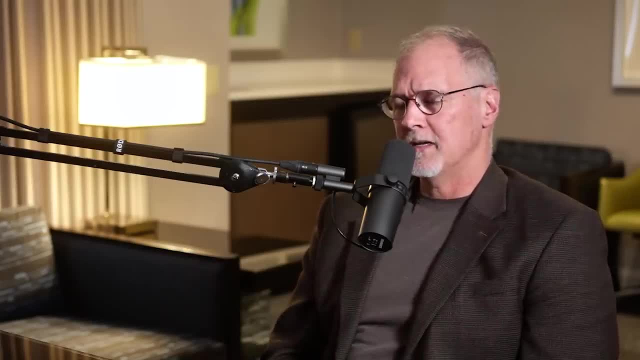 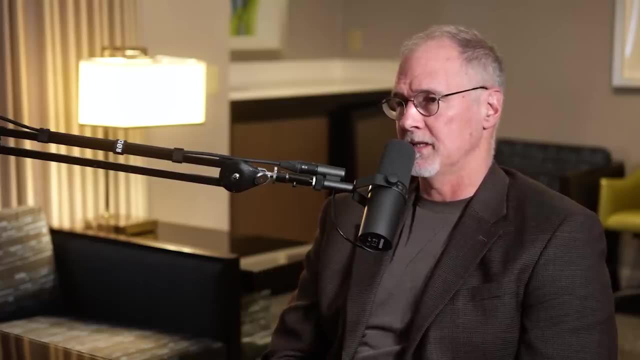 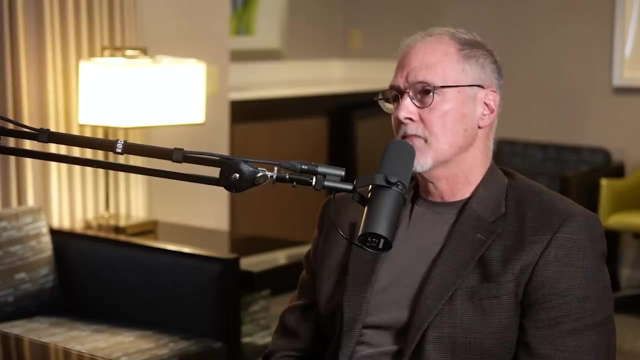 Bouncing system and then figure out how to apply that from a one legged machine to a two or a four legged machine. Those principles are really important and and- and we're definitely a core, a core part of our work- Um, there's also, you know, when we started to pursue humanoid robots, um, there was so much complexity in that machine that you know, one of the benefits of, of the humanoid form is you have some intuition. 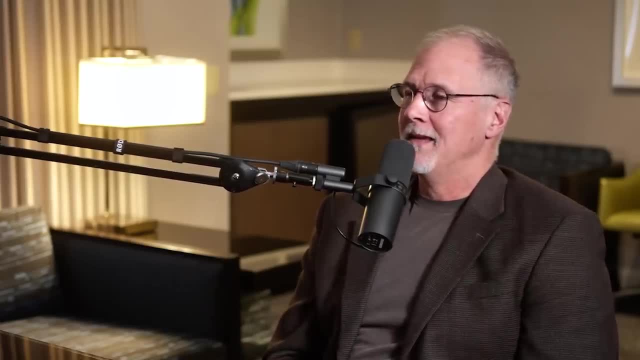 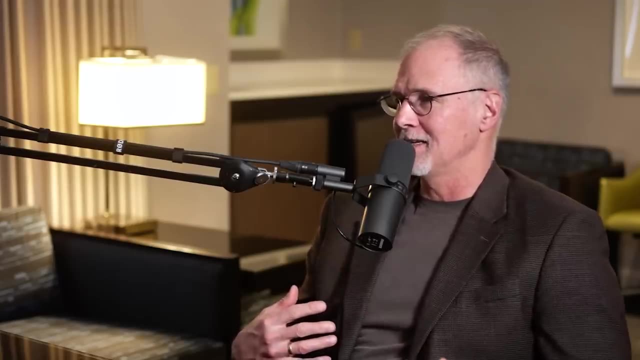 About how it should look while it's moving, And that's a little bit of an art, I think. And now it's- or maybe it's just- tapping into a knowledge that you have deep in your body and then trying to express that in the machine. 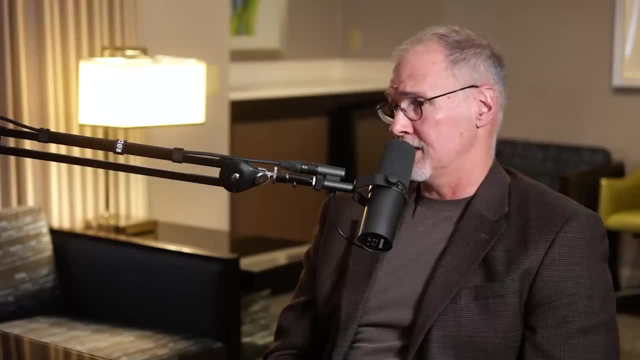 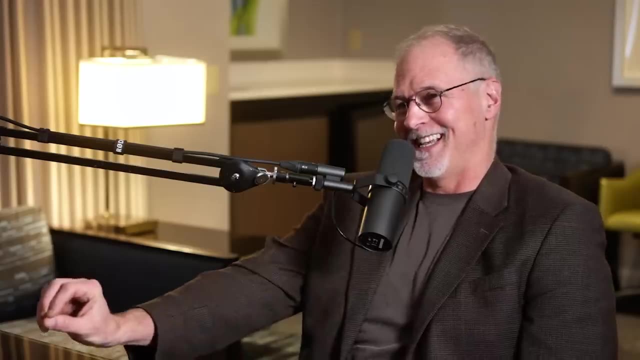 But that's an intuition. that's a little bit more on the art side. Maybe it it predates your knowledge. you know before you have the knowledge of how to control it. you try to work through the art channel and humanoids sort of make that available to you. 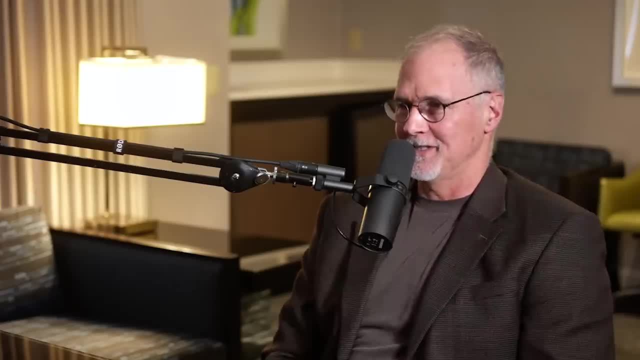 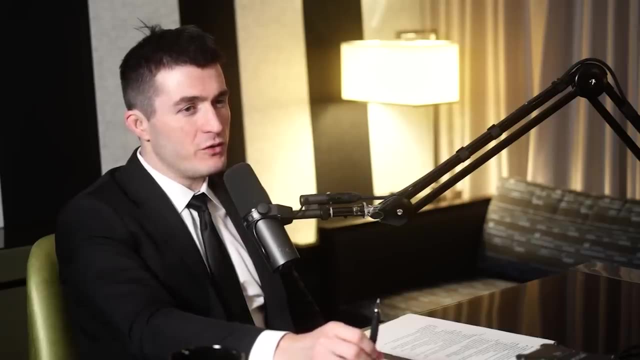 If it had been a different shape, maybe you wouldn't have had the same intuition. Yeah, so your knowledge about moving through the world is not made explicit to you, So you just- that's why it's art, And it might- yeah, it might- be hard to actually articulate exactly, you know. 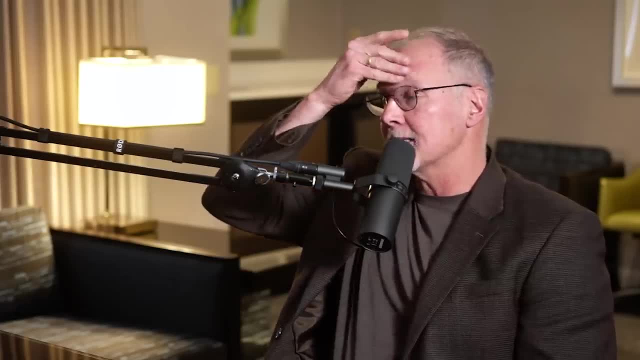 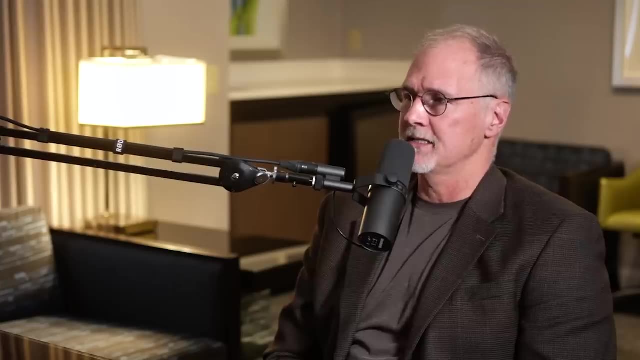 There's something about um and being a competitive uh athlete. there's something about seeing uh movement. You know a coach. one of the greatest strengths a coach has is being able to see, you know, some little change in what the athlete is doing. 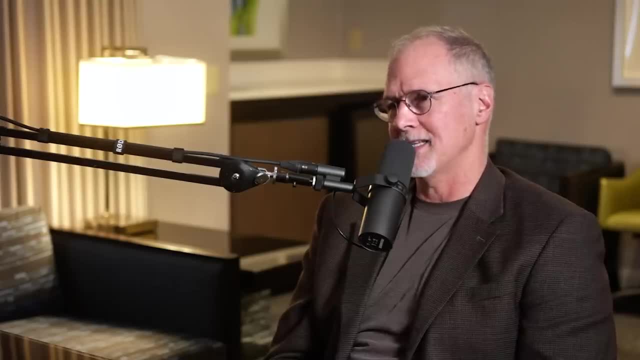 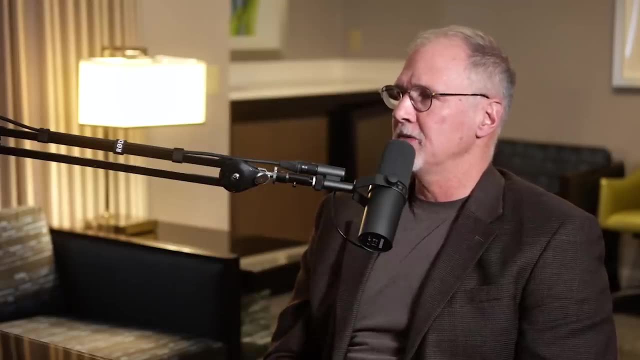 Yeah, Being able to articulate that to the athlete you know, and then maybe even trying to say, and you should try to feel this, Um, so there's something just in seeing. and again, you, you know, sometimes it's hard to articulate what it is you're seeing. 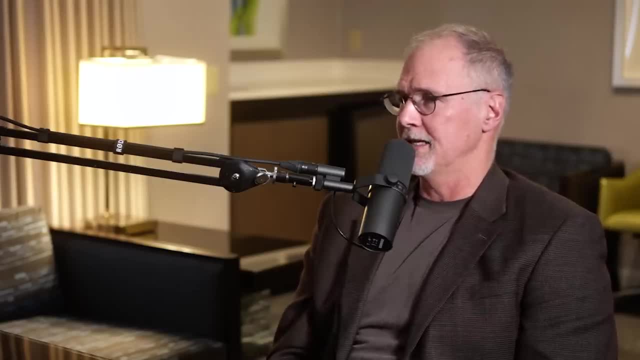 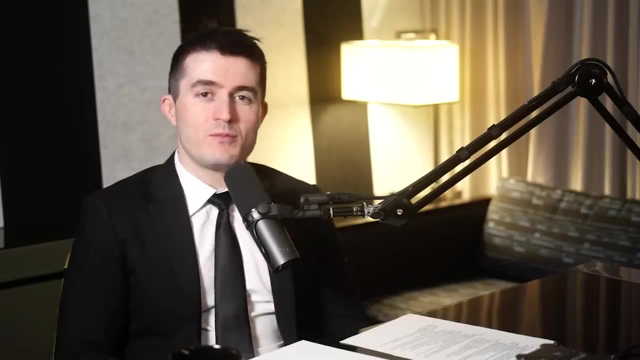 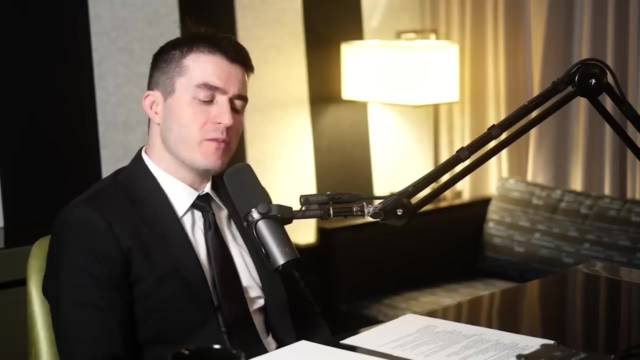 But there's a just perceiving the motion at a rate that is um, uh again, sometimes hard to put into words. Yeah, I wonder, uh, how it is possible to achieve sort of truly elegant movement. You have a movie like Ex Machina. 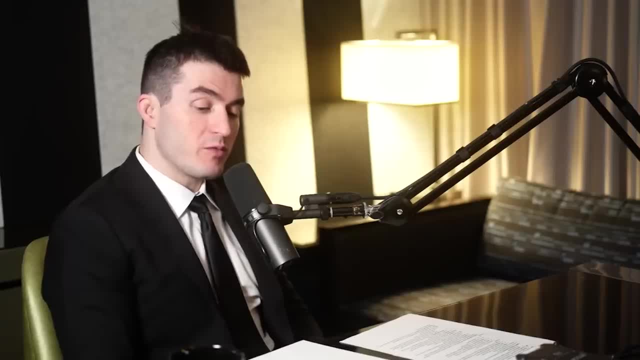 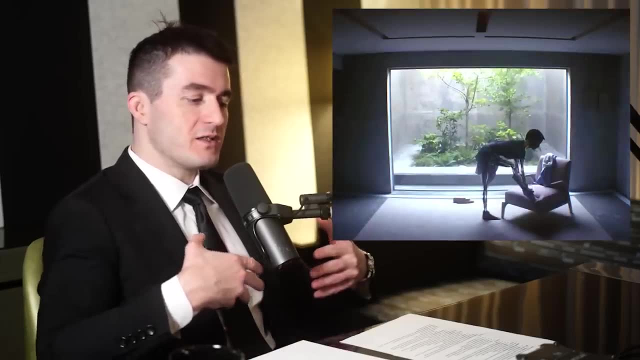 I'm not sure if you've seen it, but, uh, the main actress in that, who plays the AI robot, I think, is a ballerina. I mean just the natural um, the elegance and the- I don't know- eloquence of movement. 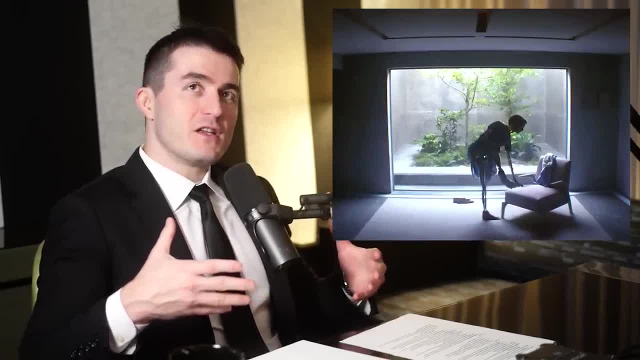 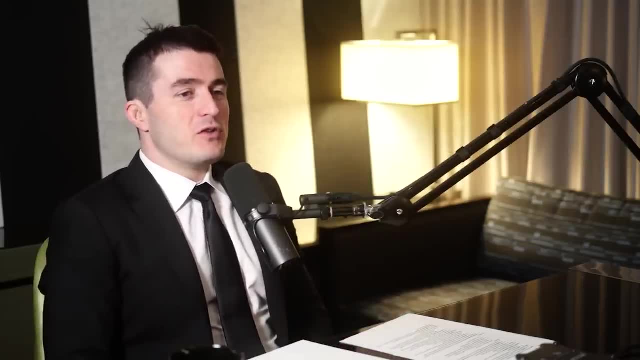 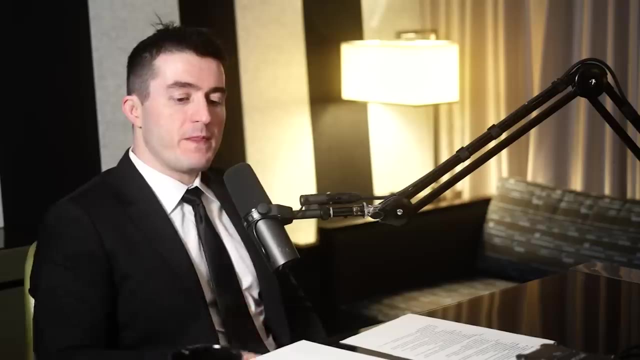 It's, it's, it looks efficient and easy and just it looks right. It looks beautiful, It looks right is sort of the key, Yeah. And then you, you look at um especially early robots. I mean They, they, they're so cautious in in the way they move um that it's not. it's not the caution, that looks wrong. 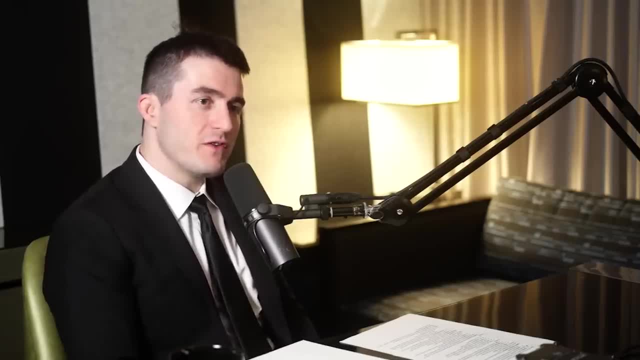 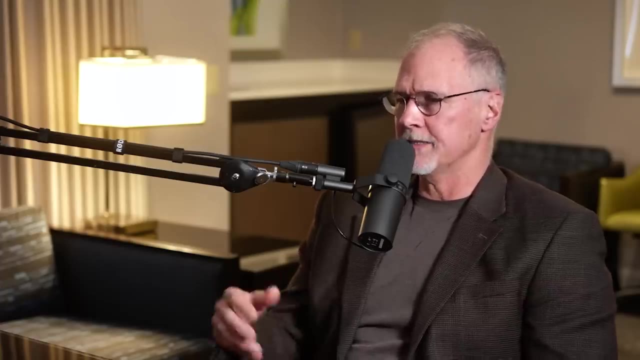 It's. it's something about the movement that looks wrong, that feels like it's very inefficient, unnecessarily so, And it's hard to put that into words exactly. We think that, and part of the reason why people are attracted to the machines we build is because the inherent dynamics of movement are are closer to right. 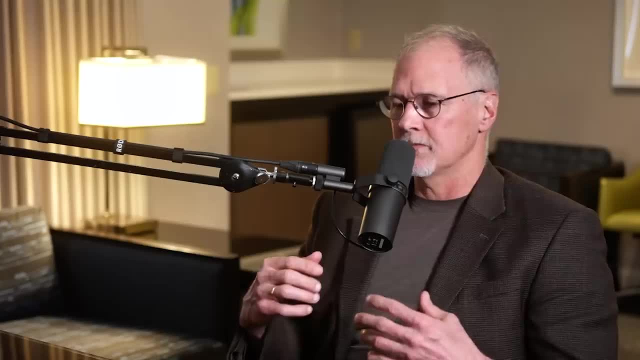 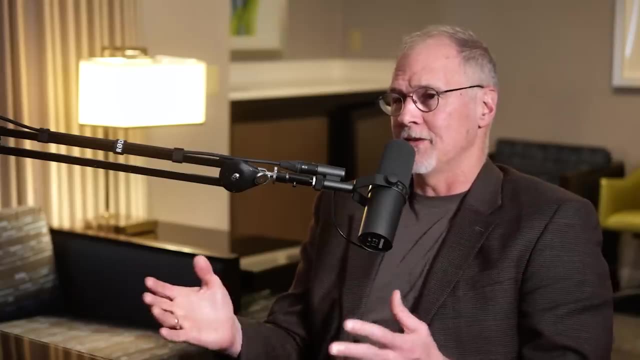 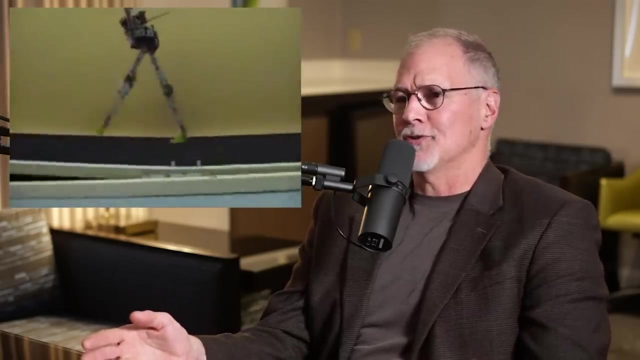 Um, because we we try to use, you know, walking gates or we build a machine around this gate where you're trying to work with the dynamics of the machine instead of to stop them. you know some of the early walking machines, you know you're essentially you're really trying hard to not let them fall over. 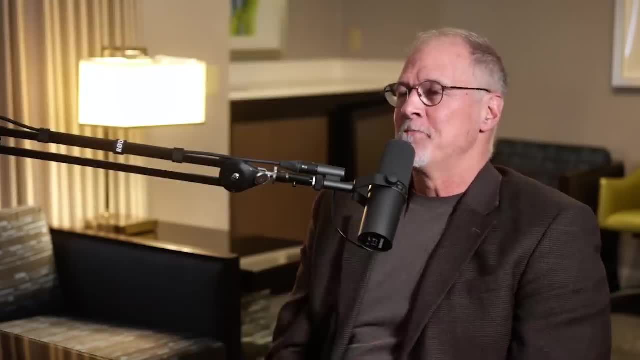 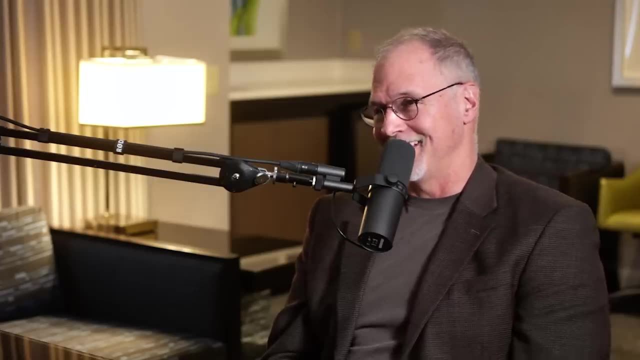 And so you're always stopping the tipping motion, you know, and sort of the insight of dynamic stability in a light machine is to go with it. You know, let the tipping happen. you know, let yourself fall, but then catch her, catch yourself with that next foot. 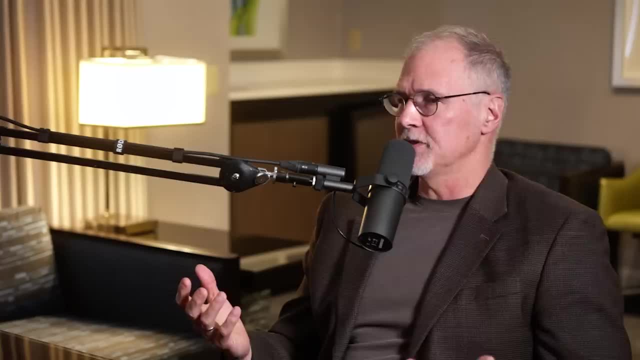 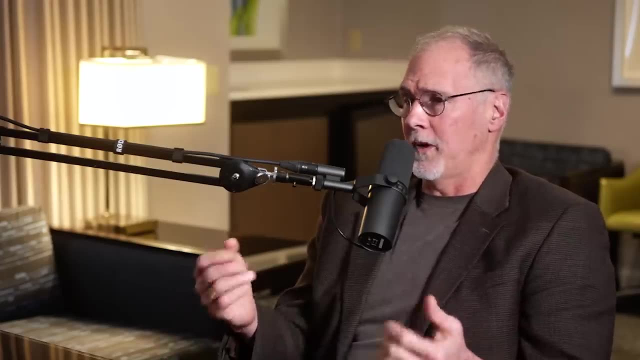 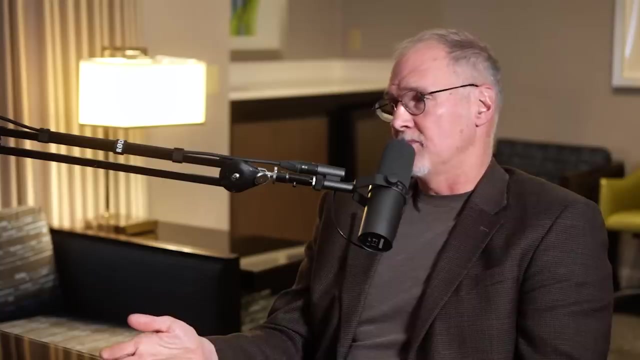 And there's something about getting those physics to be expressed in the machine that people interpret as lifelike or or elegant or just natural looking, And so I think if you get the physics right, it also ends up being more efficient. Likely there's a benefit that it probably ends up being more stable. 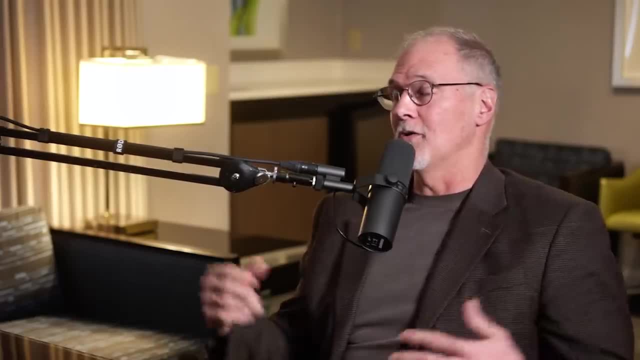 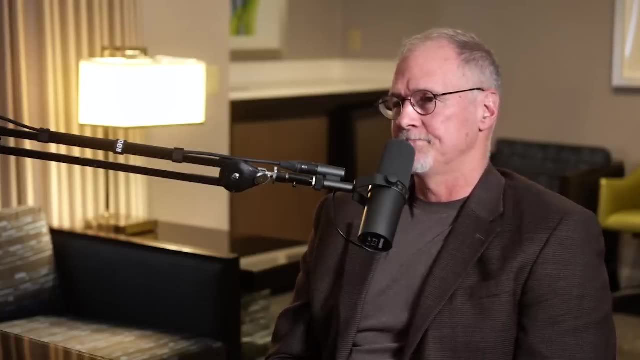 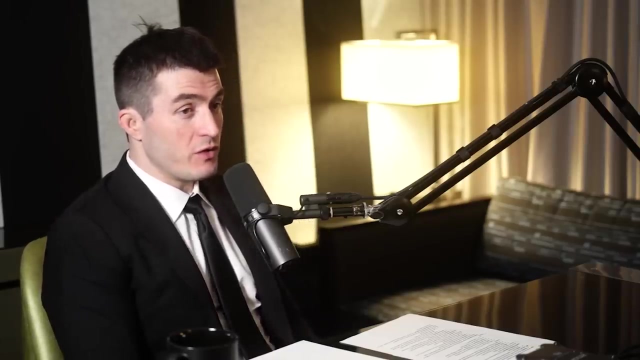 Yeah, In the long run, you know it could. it could walk stably over a wider range of conditions. Um, and it's uh, and it's more beautiful and attractive at the same time. So how hard is it to get the humanoid robot Atlas to do some of the things it's recently been doing? 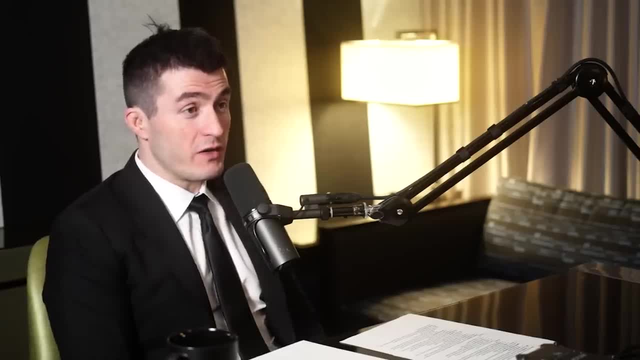 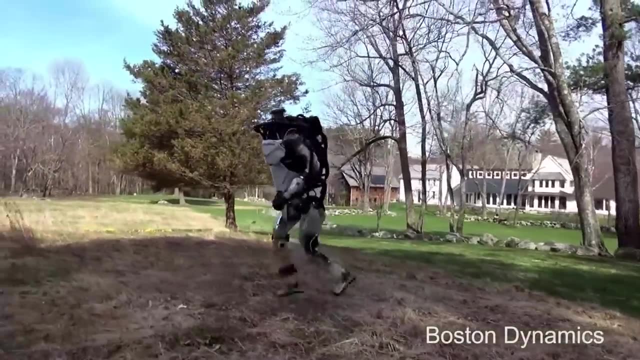 Let's forget the flips and all of that. Let's just look at the running. Maybe you can correct me, but there's something about running. I mean, that's not careful at all. That's, you're falling forward, You're jumping forward and are falling. 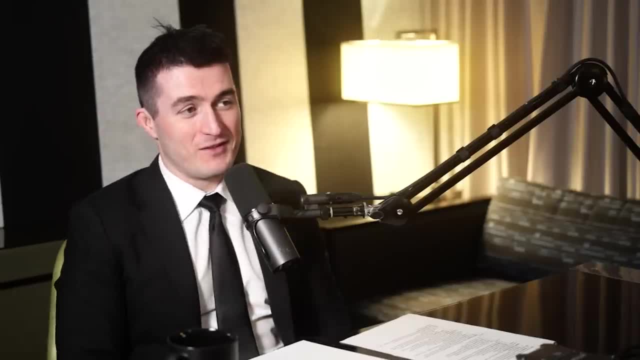 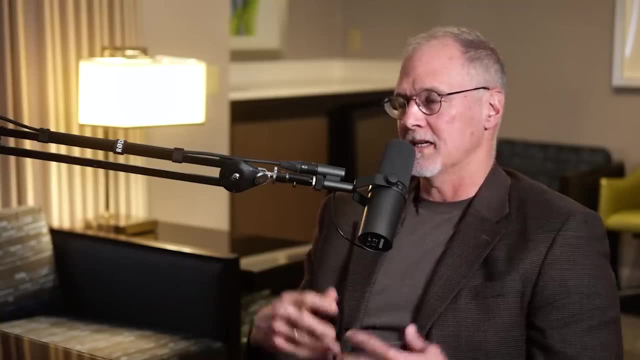 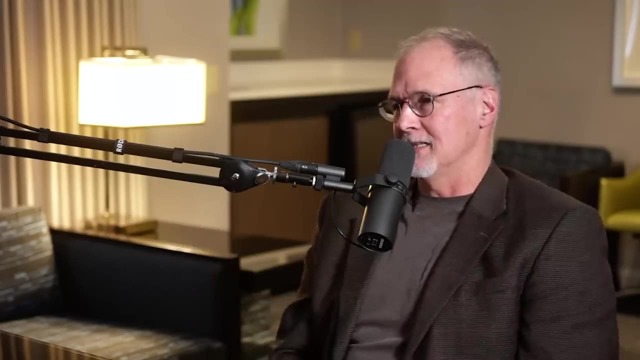 So How hard is it to get that right? Our first humanoid, we needed to deliver natural looking walking. You know we took a contract from the army. They wanted a robot that could walk naturally. They wanted to put a suit on the robot and be able to test it in a gas environment. 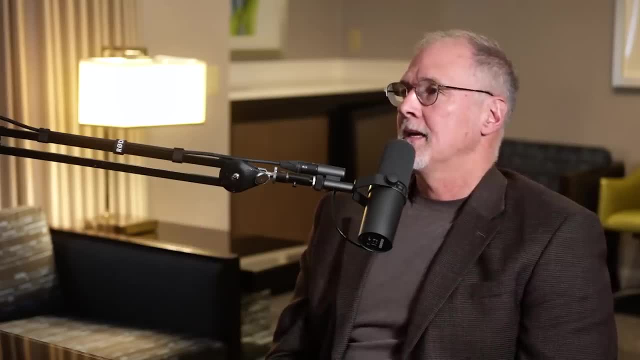 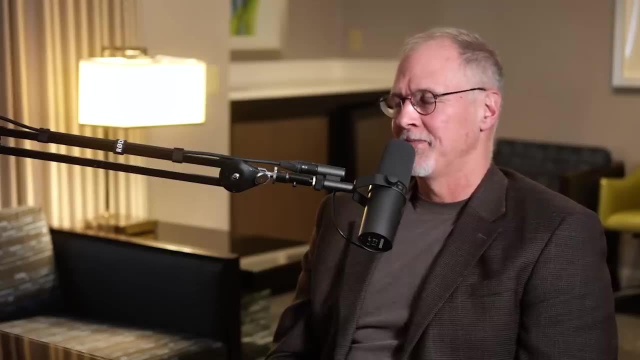 And so they wanted that the motion to be natural, Um and so our goal was a natural looking gate. It was really, it was surprisingly hard to get that to work. Um and we, But we did build a, an early machine. uh, we called it pet man prototype. 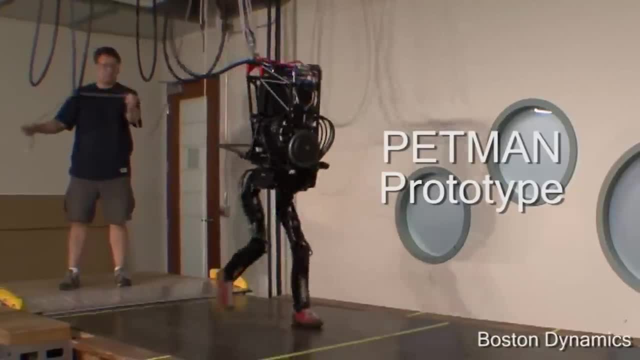 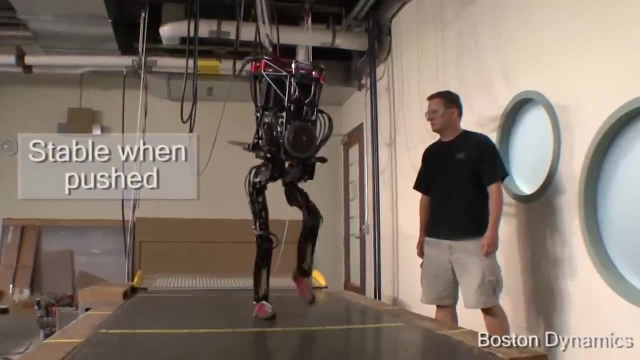 It was the prototype before the pet man robot And it had a really nice looking um gate where you know it would stick the leg out. It would do heel strike first before it rolled onto the toe, So you didn't land with a flat foot. 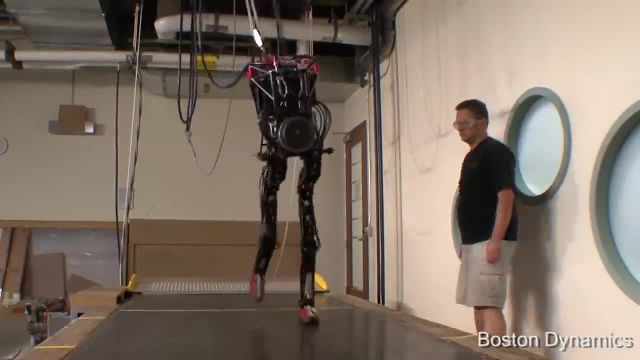 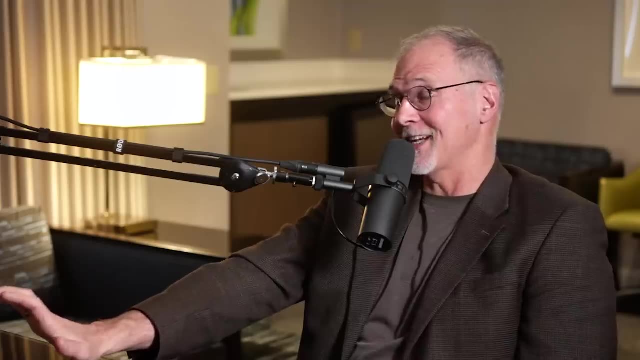 You extended your leg a little bit, Um, but even then it was hard to get the robot to walk where when, when you were walking did it fully extended its leg And essentially landed on an extended leg. And if you watch closely how you walk, you probably land on an extended leg. but then 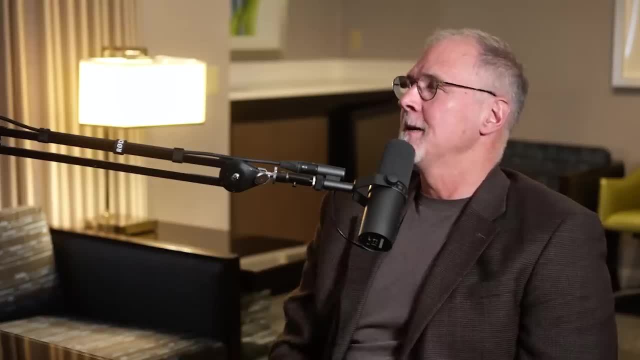 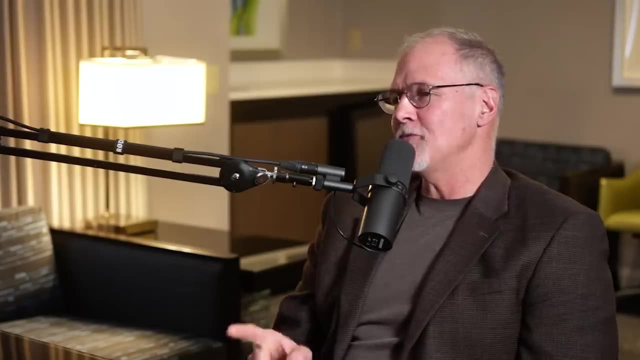 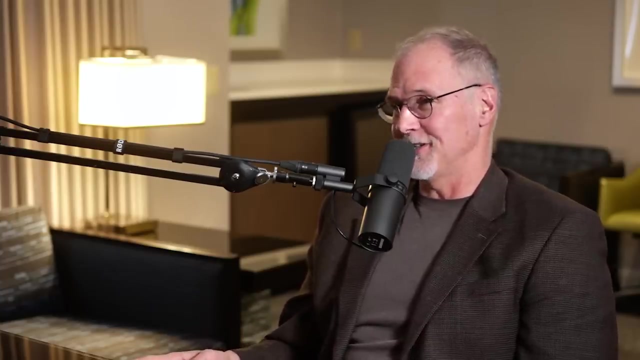 you immediately flex your knee as you start to make that contact and getting that all to work Well, it took such a long time. In fact, I probably didn't really see the nice natural walking that I expected out of our humanoids until maybe last year. 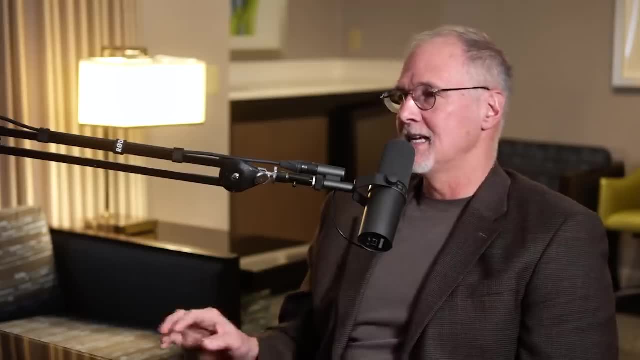 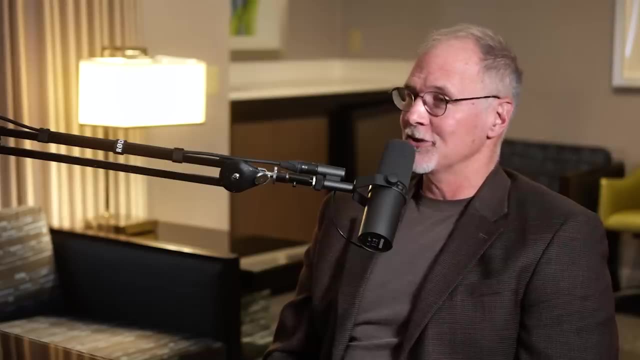 And the team was developing on our newer generation of Atlas- you know some new techniques, Um uh, for developing a walking control algorithm- and they got that natural looking motion as sort of a by-product of a of a just a different process that we're applying. 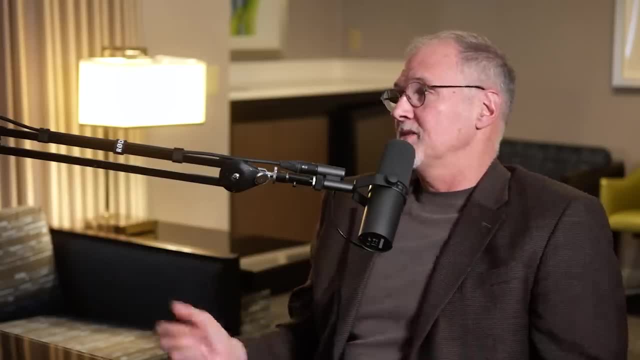 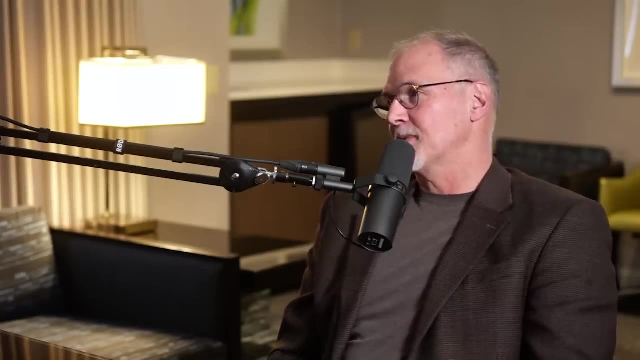 to developing the control. So that probably took 15 years- 10 to 15 years- to sort of get that from from. you know, the pet man prototype was probably in 2008.. And what was it 2022? last year that I think I saw a good walking on Atlas. 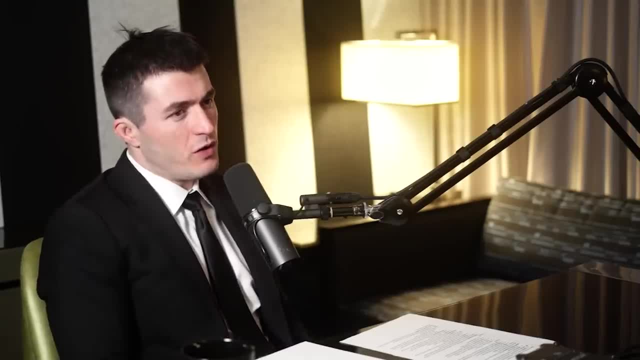 If you could just like linger on it. What are some challenges of getting good walking? So is it um? is this? is this partially like a hardware, like actuator problem? Is it the control? Is it the artistic element of just observing the whole system operating in different conditions? 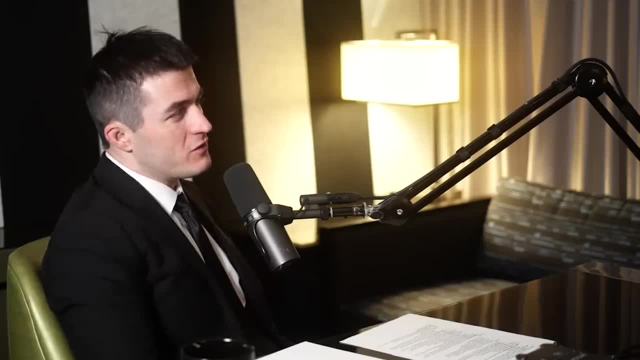 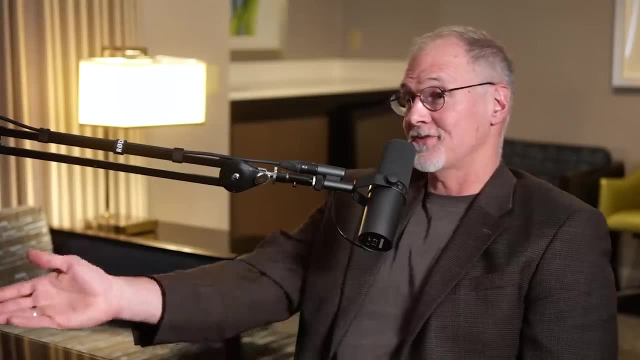 together. I mean, is there some kind of interesting quirks or challenges you can speak to, like the heel strike or all this kind of stuff? Yeah, So one of the things that makes the like this straight leg, uh, a challenge is you're. 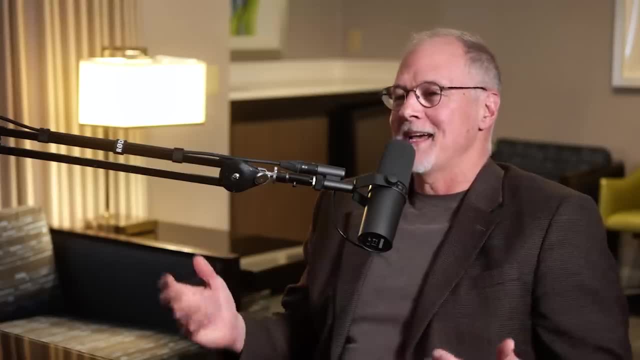 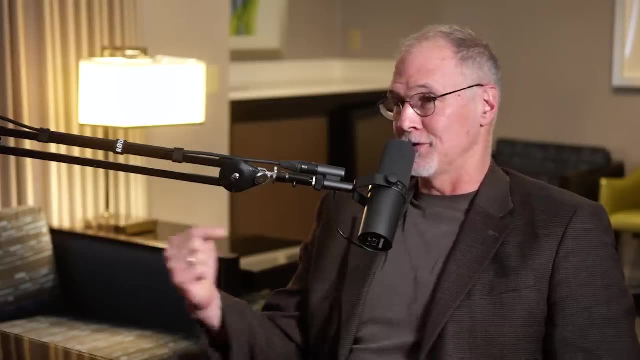 sort of up against uh, a singularity, a mathematical single singularity, where you know when, when your leg is fully extended, it can't go further. the other direction, right, There's only. you can only move in one direction, and that makes all of the calculations around. 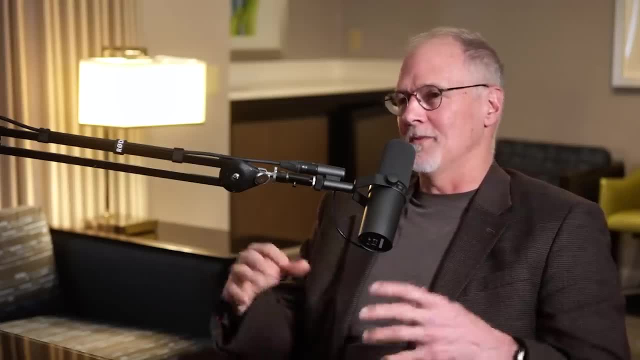 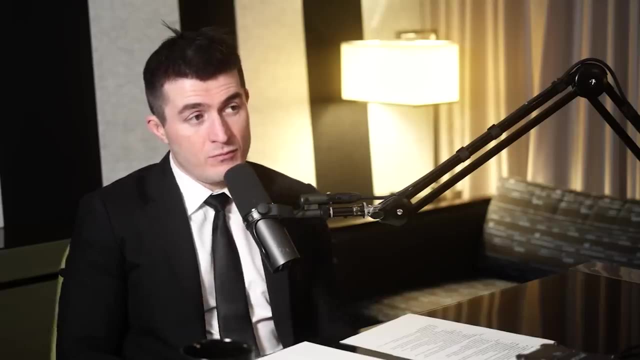 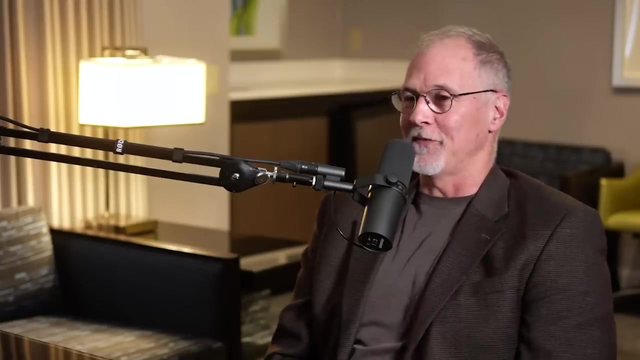 how to produce torques at that joint or positions, makes it more complicated, And so having all of the mathematics so it can deal with these singular configurations is one of many challenges, Uh, uh, that we face. and I'd say in in the, you know, in those earlier days again, we 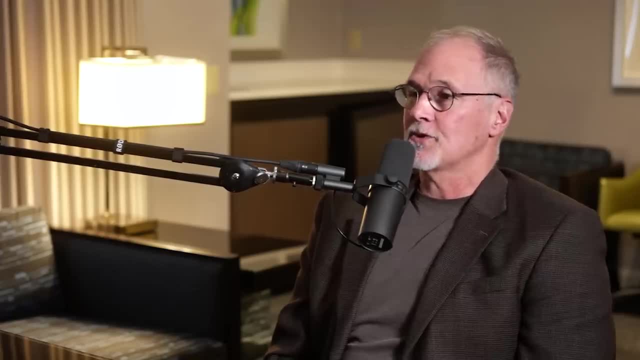 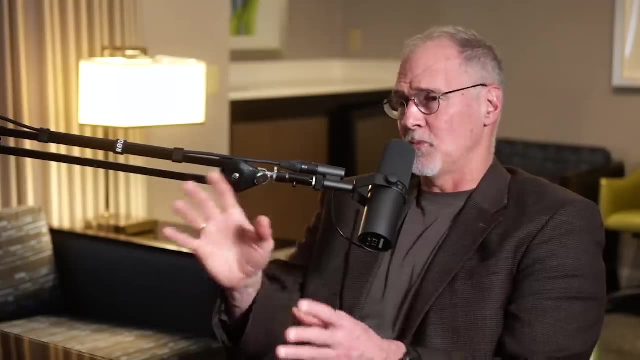 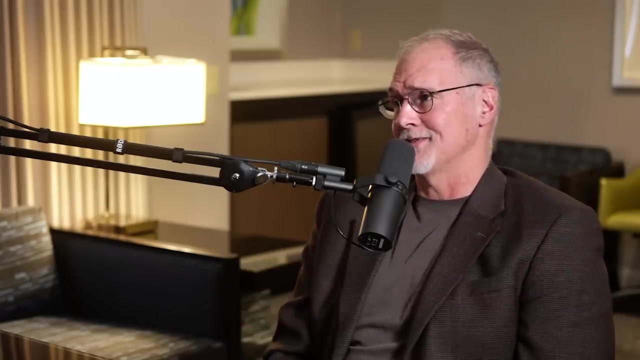 were working with these really simplified models. So we're trying to boil all the physics of the complex human body into a simpler subsystem that we can more easily describe in mathematics, And sometimes those simpler subsystems don't have all of that complexity of the straight. 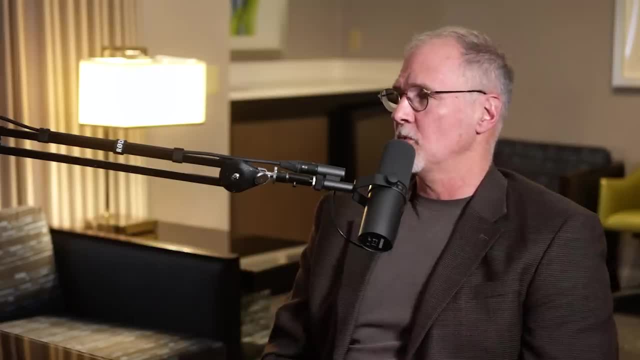 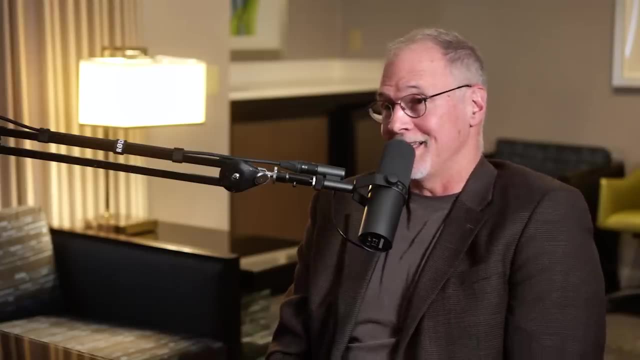 leg built into them And so, um, what's what's happened more recently is we're Able to apply techniques that let us take the full physics of the um uh robot into account and and deal with some of those uh strange situations like this, like the. 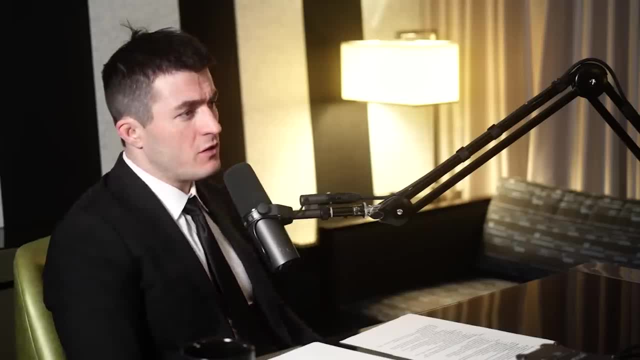 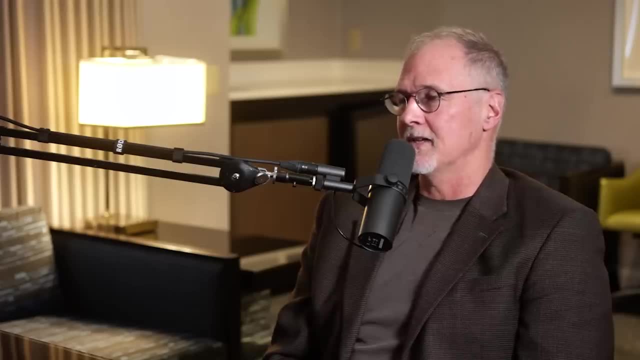 straight leg. So is there a fundamental challenge here? that it's- uh, maybe you can correct me, but is it under actuated? Are you falling? Under actuated is is the right word, right, You can't? you can't, uh, push the robot in any direction you want to, right. 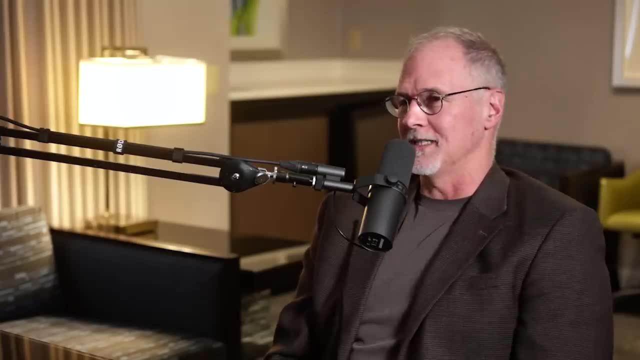 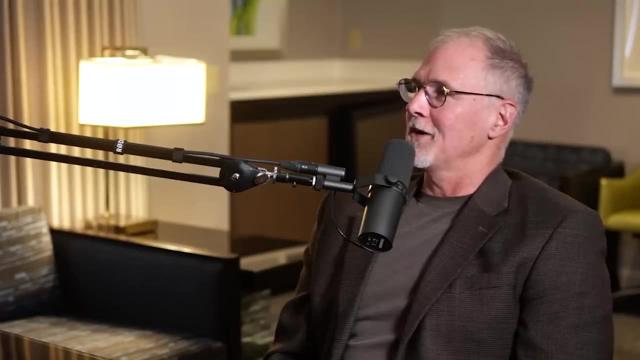 And so that that is one of the hard problems of of uh like a locomotive, And you have to do that for natural movement. It's not necessarily required for natural movement, It's just required. You know, we, we don't have, you know, a gravity force that you can hook yourself onto to apply. 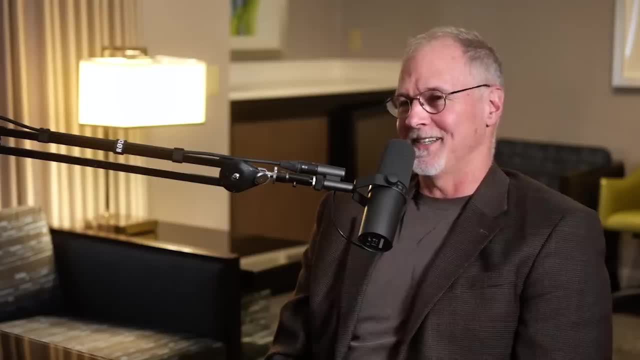 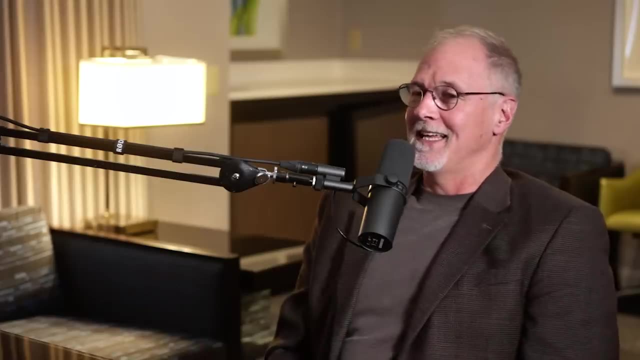 uh, an external force in the direction you want, at all times. right, The only, the only external forces are being mediated through your feet and how they get mediated depend on how you place your feet And, uh, you know you can't just. uh, you know God's hand can't reach down and give. 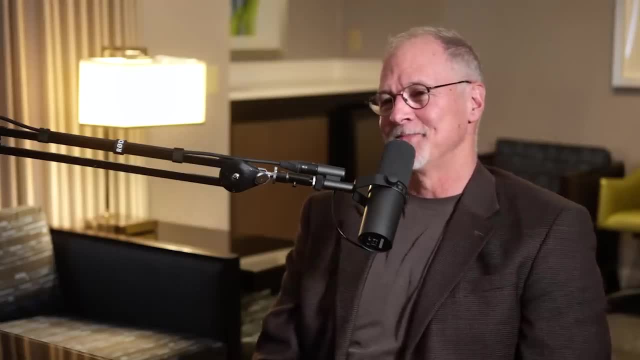 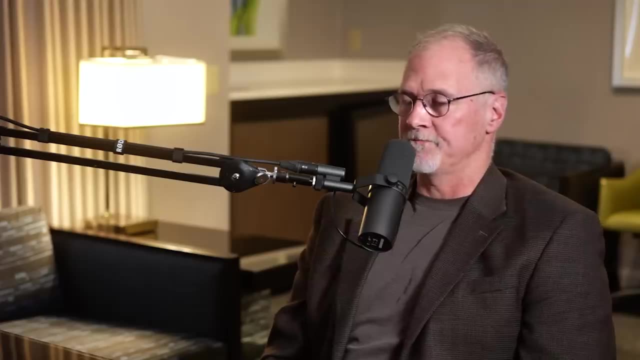 and push anything Any direction you want. you know, so is there. uh, is there some extra challenge to the fact that Alice is such a big robot? There is, the humanoid form is um um attractive in many ways, but it's also a challenge in. 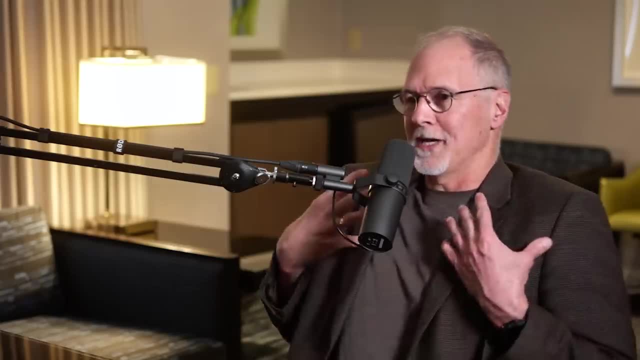 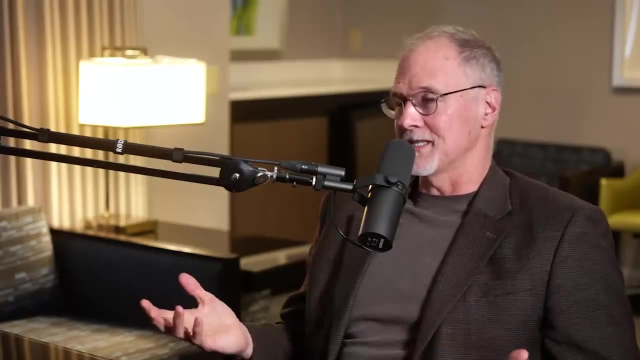 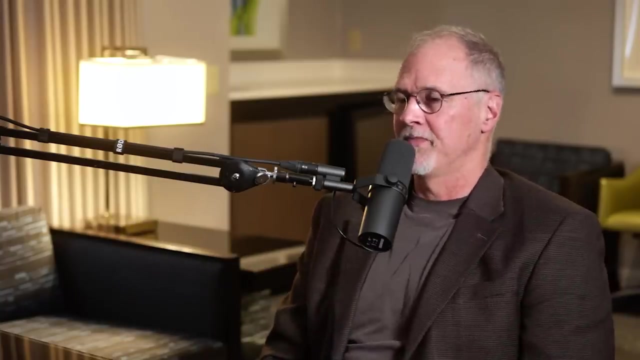 many ways. Um, you have this big upper body that has a lot of mass and inertia, um, and throwing that inertia around increases the complexity of maintaining balance, And as soon as you pick up something heavy in your arms, Yeah, It made that problem even harder. 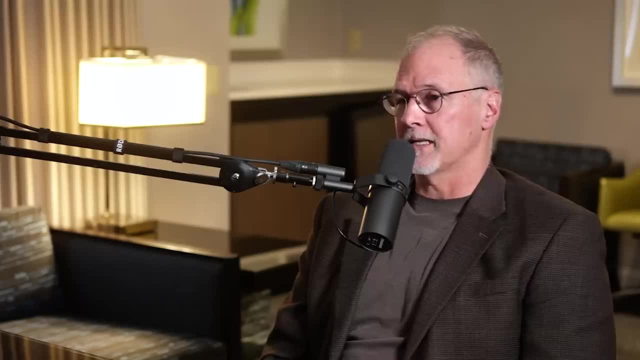 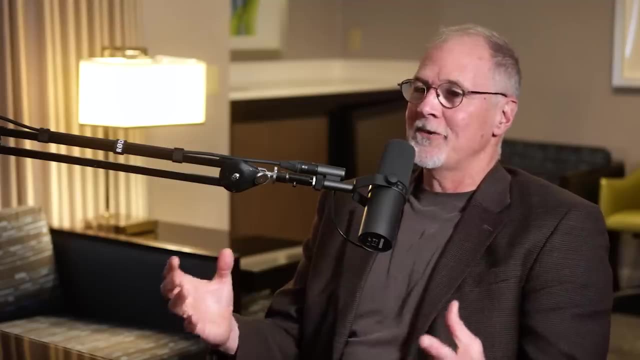 And so, uh, in the early work in the leg lab and in the early days at the company, you know we were pursuing these quadruped robots which had a a kind of built in simplification. You had this big, rigid body and then really light legs. 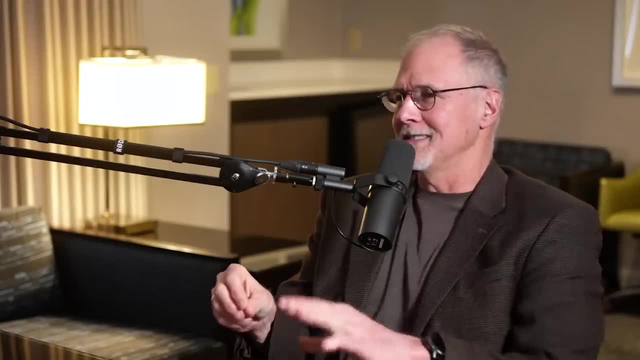 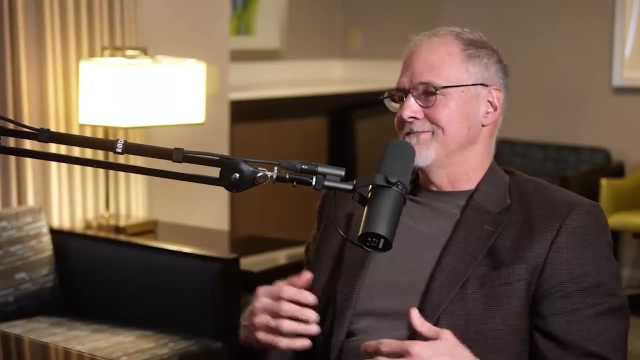 So when you swing the legs, the leg motion didn't impact the body motion very much. All the mass and inertia was in the body. but when you have the humanoid that doesn't work. You have big, heavy legs. you swing the legs, it affects everything else. 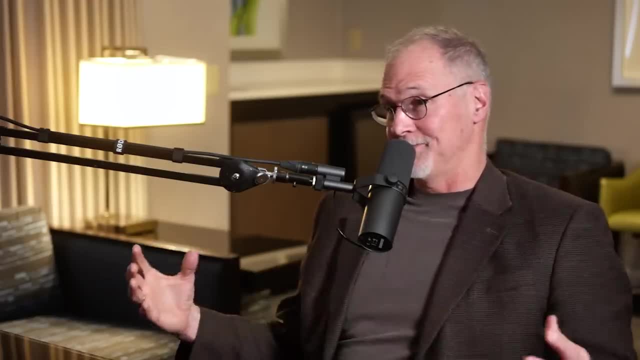 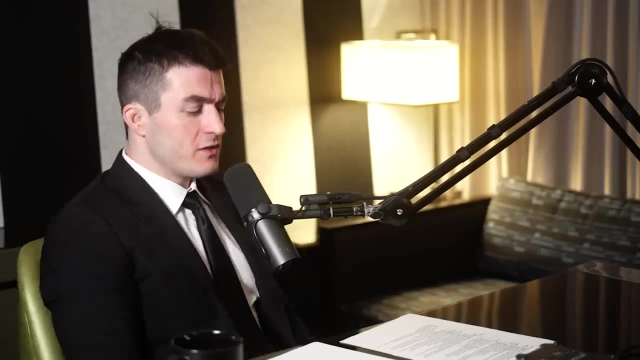 And so dealing with all of that interaction does make the humanoid a much more complicated platform, And I also saw that, uh, at least recently, you've been doing more explicit modeling of the stuff you pick up. Yeah, Just very, um, really interesting. 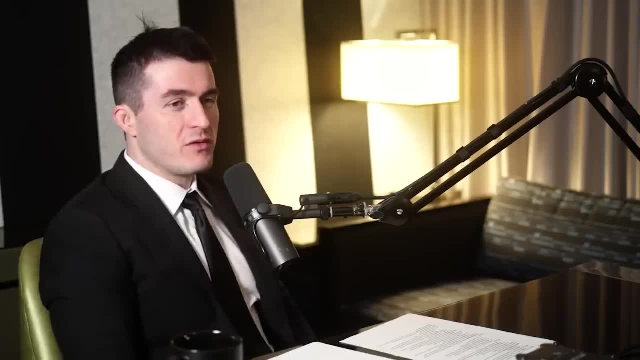 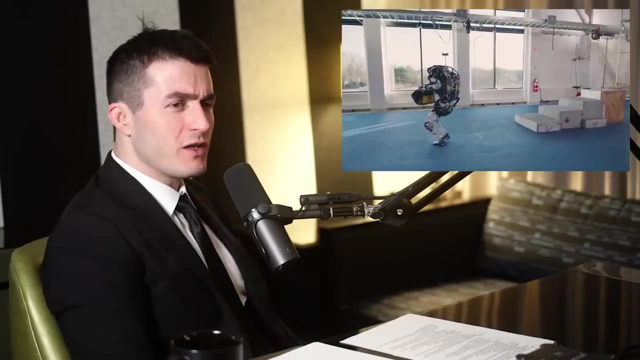 So you have to what model, the shape, the weight distribution, I don't know what like you have to under, like, include that as part of the modeling, as part of the planning, because okay, so for people who don't know, uh, so Atlas, at least in like a recent video, like throws a heavy bag, throws a bunch of stuff. 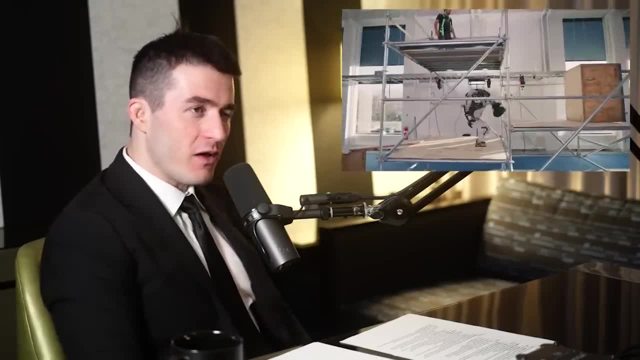 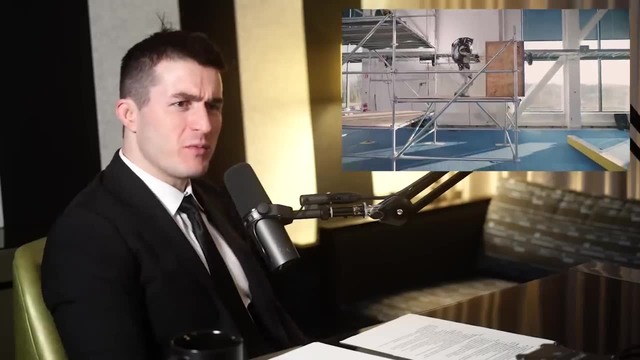 So what? what's involved in uh picking up a thing, a heavy thing, uh, and when that thing is a bunch of different nonstandard things, I think it also picked up like a barbell and uh to be able to throw it in some cases. 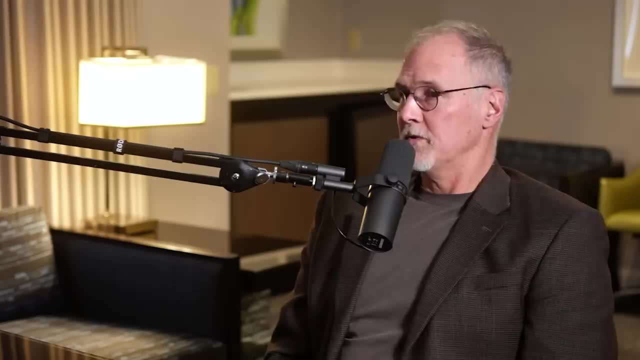 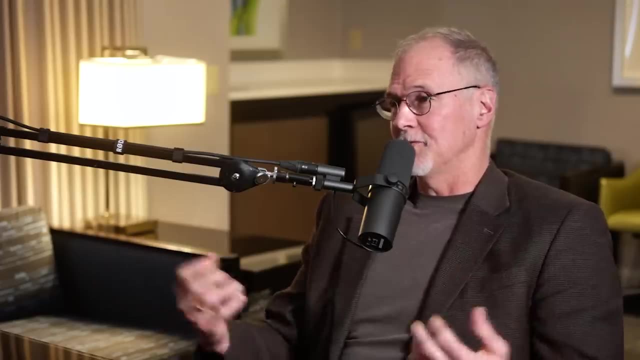 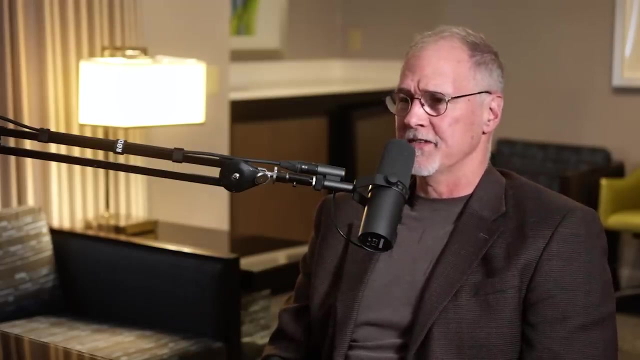 What's, what are some interesting challenges there. So we were definitely trying to show that the robot and the techniques we're applying to the robe, uh, to Atlas. let us deal with heavy things in the world, because if the robot's going to be useful, it's actually got to move stuff around and that and that needs to be significant stuff. 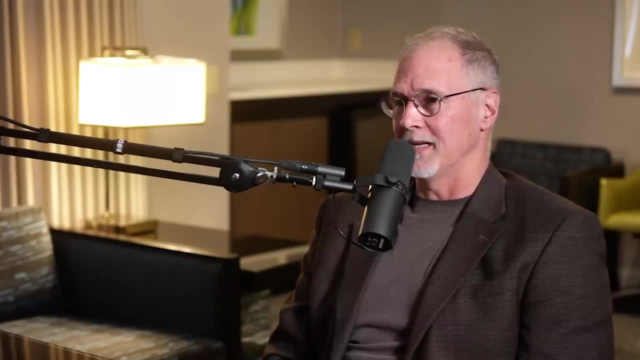 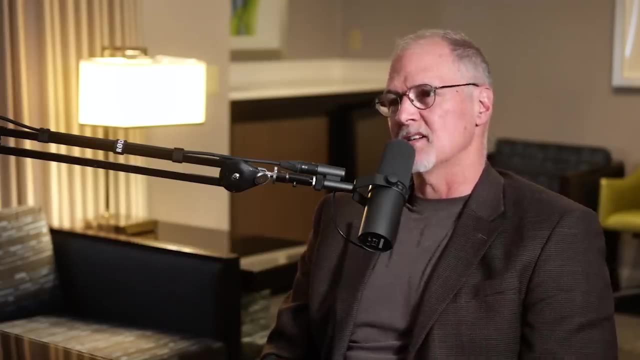 That's an appreciable portion of the body weight of the robot, And we also think this differentiates us from the other humanoid robot activities that you're seeing out there. Mostly, they're not picking stuff up- Yeah, And not heavy stuff anyway. 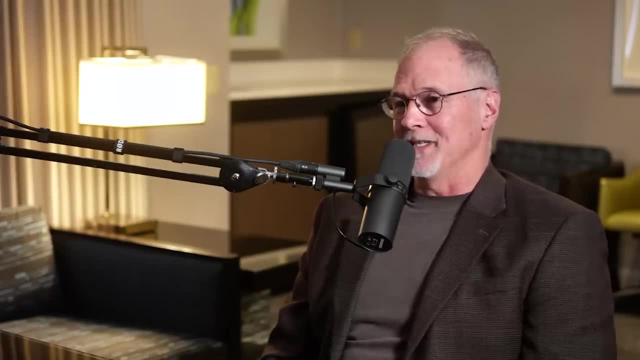 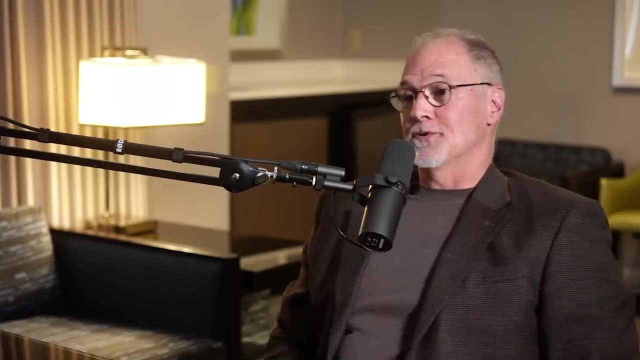 Um, but just like you or me, you know you need to anticipate that moment. you know you're reaching out to pick something up And as soon as you pick it up, your center of mass is going to shift. And if you're going to, you know, turn in a circle or you have to take that inertia into account. 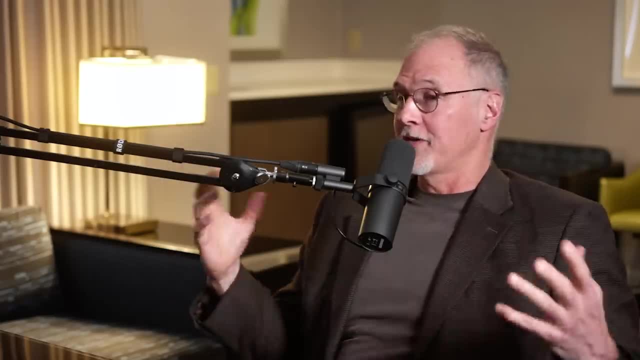 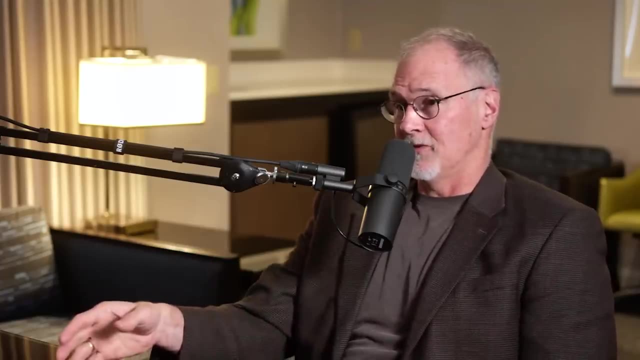 And if you're going to throw a thing you know you've got, all of that has to be sort of included in in the model of what you're trying to do. So the robot needs to have some idea or expectation of what that weight is. 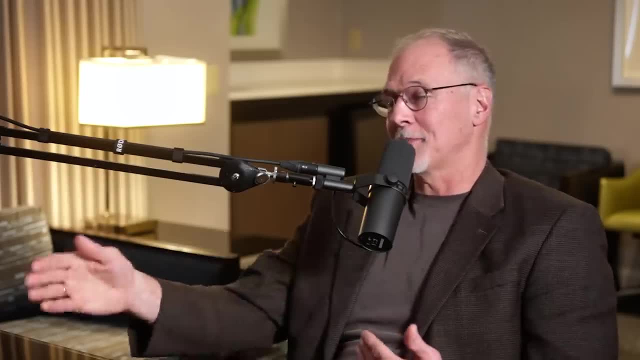 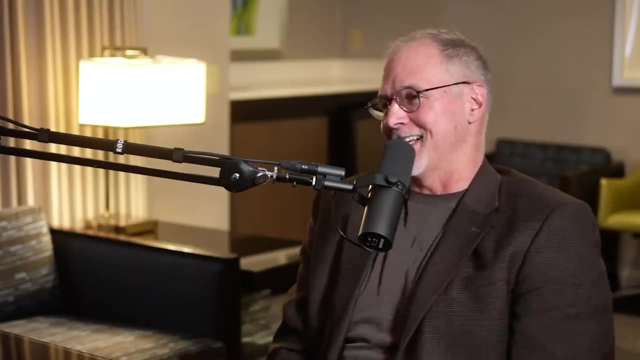 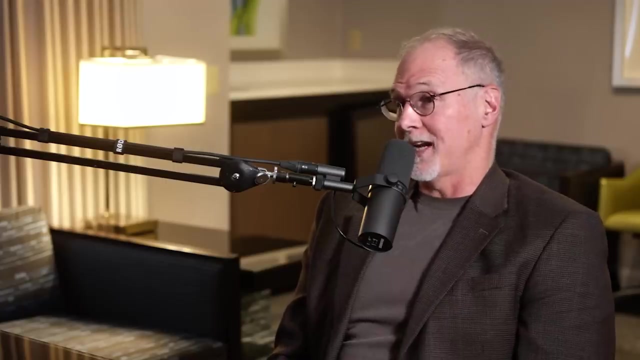 And then, and sort of predict, you know, think a couple of seconds ahead, How do I manage my, now, my, my body plus this big heavy thing together to get and and still maintain balance Right? And so, um, I, I, uh, that's a big change for us. 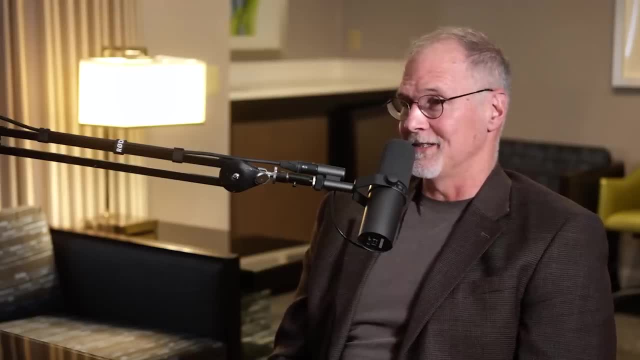 And I think the tools we've built are really allowing that to happen um quickly. now, Some of those motions that you saw in that most recent video, we were able to create in a matter of days. Yeah, It used to be that it took six months to do anything new, you know, on the robot. 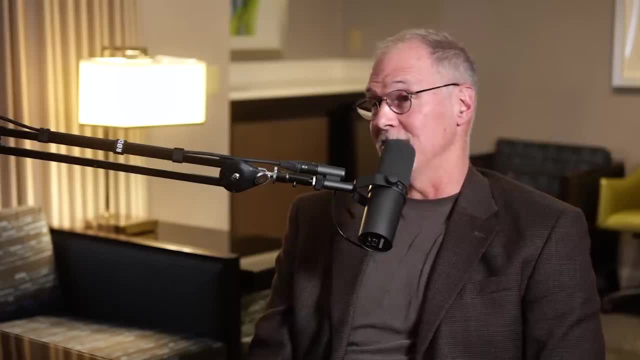 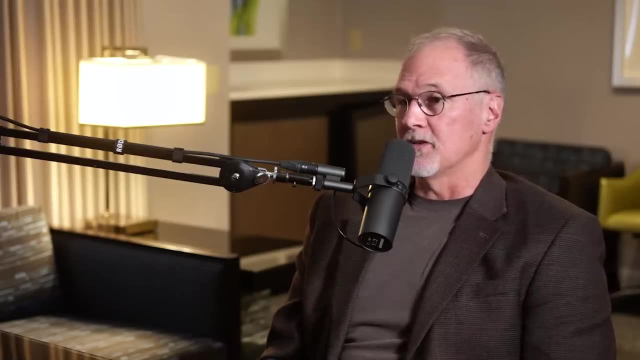 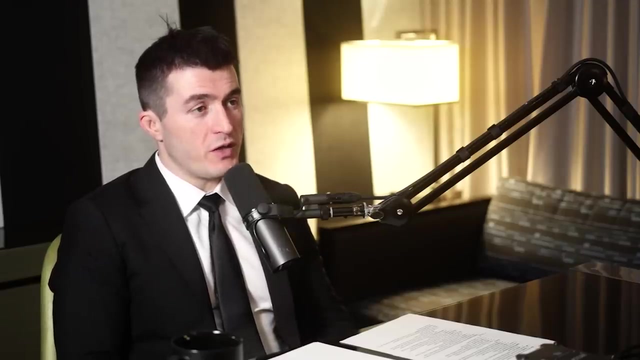 And now we're starting to develop the tools that let us do that in a matter of days, And so we think that's really exciting. That means that the ability to create new behaviors for the robot is going to be a quicker process, So being able to explicitly model new things that it might need to pick up new types of things. 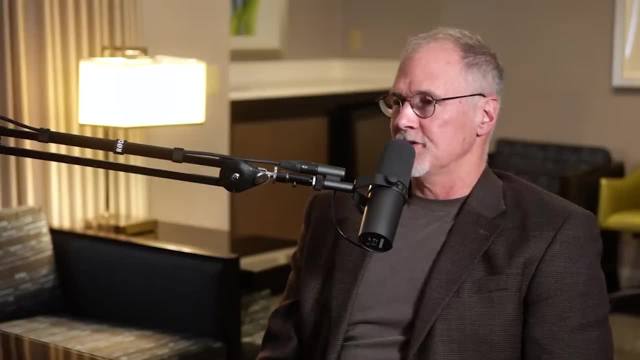 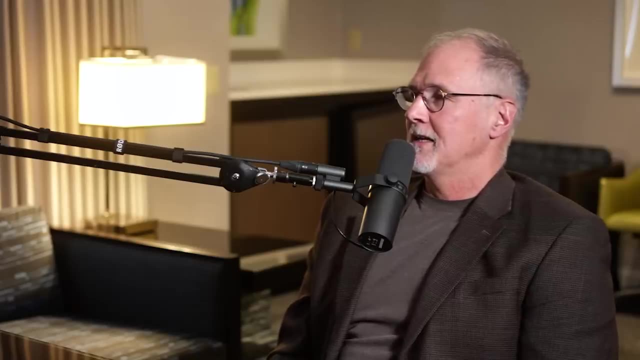 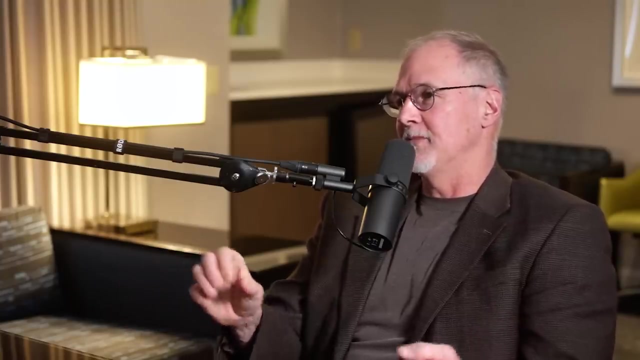 And you know, to some degree, you don't? you don't want to have to pay too much attention to each specific thing, Right? Um, there's sort of a generalization here. Uh, um, obviously, when you grab a thing, you have to conform your, your hand, your end effector, to the surface of that shape. 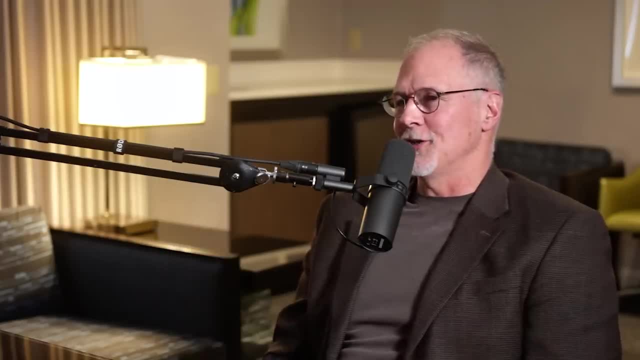 But once it's in your hands, it's probably just the mass and inertia that matter, And the the shape may, may not be as important, And so you know for some, in some ways, you want to pay attention to that detailed shape. 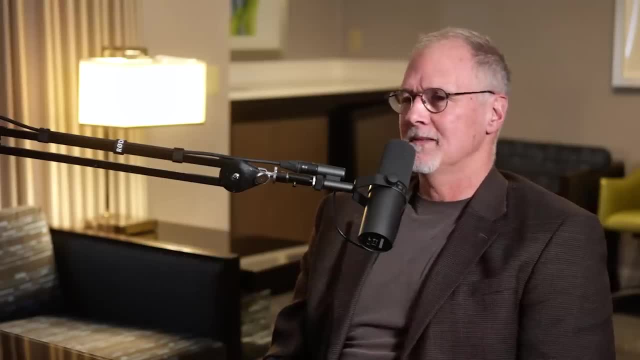 And and others. you want to generalize it and say, uh well, uh, all I really care about is the center of mass of this thing. Yeah, Especially if I'm going to throw it up on that scaffolding, And it's easier if the body is rigid. 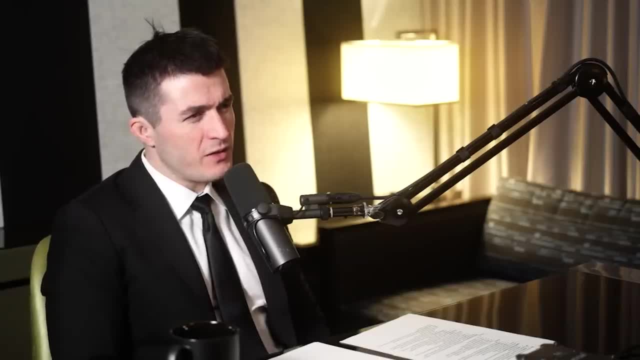 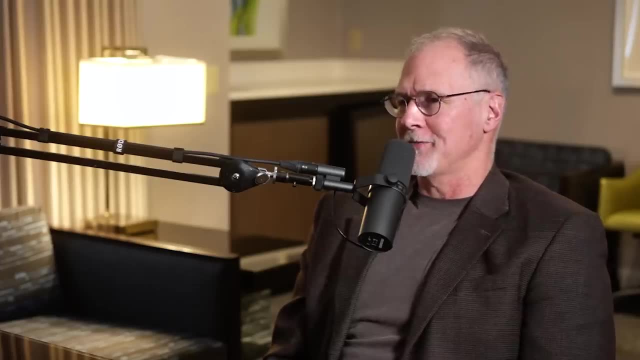 What if it's? there's some doesn't it throw like a sandbag type thing, That tool bag you know had loose, had loose stuff in it. So it it. it managed that There are harder things that we haven't done yet. 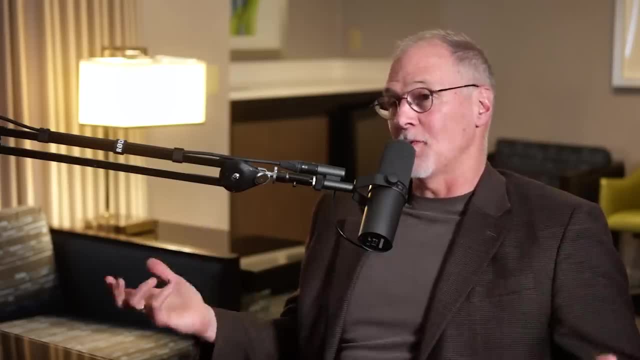 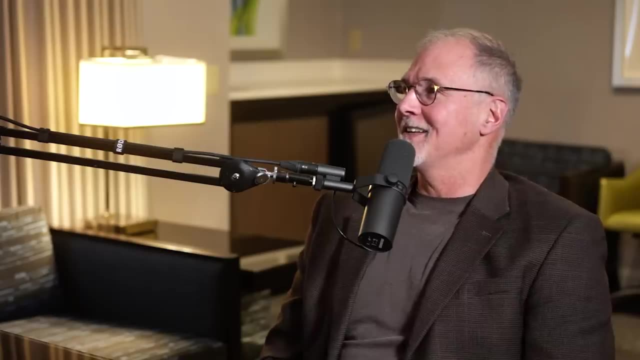 You know, we could have had a big jointed thing or I don't know, a bunch of loose wire or rope. What about carrying another robot? How about that? Yeah, we haven't. we haven't done that yet. Carry spot. 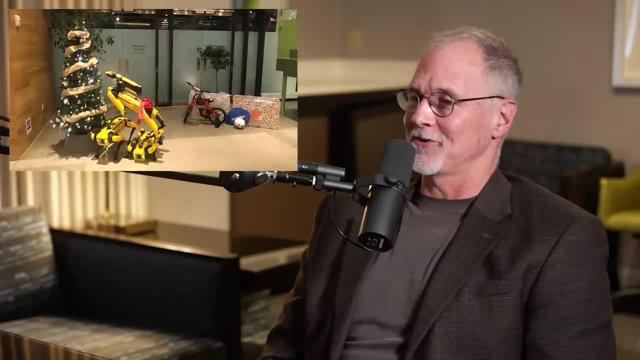 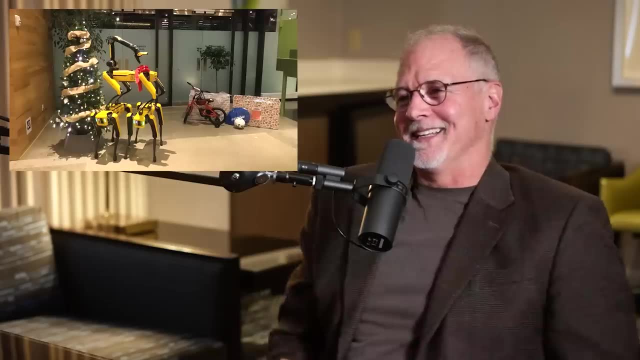 I guess we did a little bit of a. we did a uh a little A little skit around Christmas where we had two spots holding up another spot that was trying to put, you know, a bow on a tree. So I guess we're doing that in a small way. 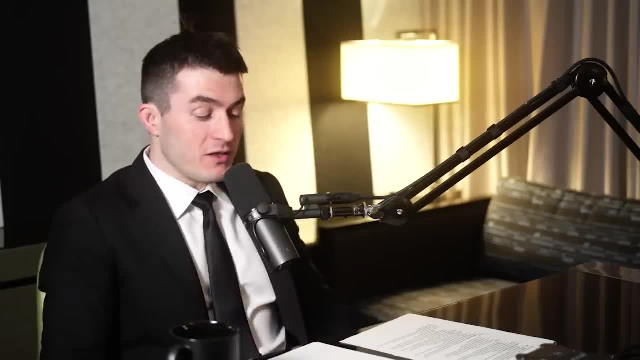 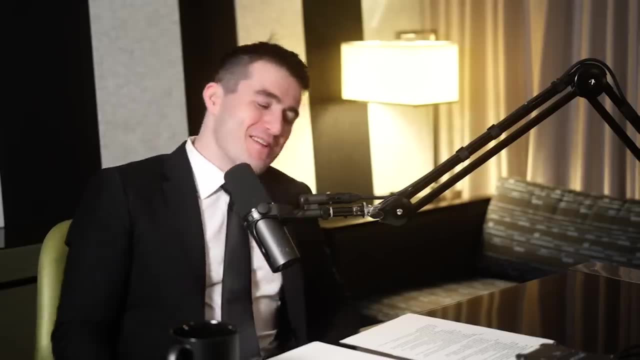 Okay, That's pretty good. Uh, let me ask the all important question. Uh, do you know how much Atlas can curl, Have you? I mean, you know this. for us humans, that's really one of the most fundamental questions you can ask another human being. 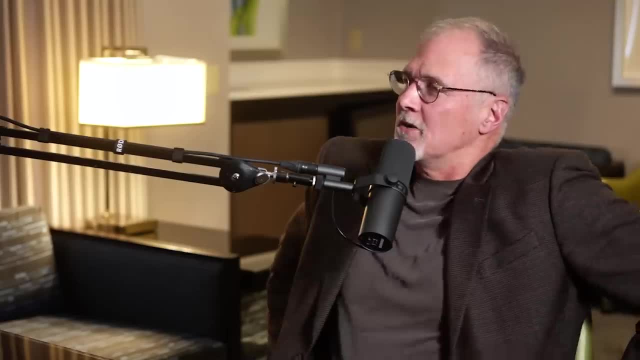 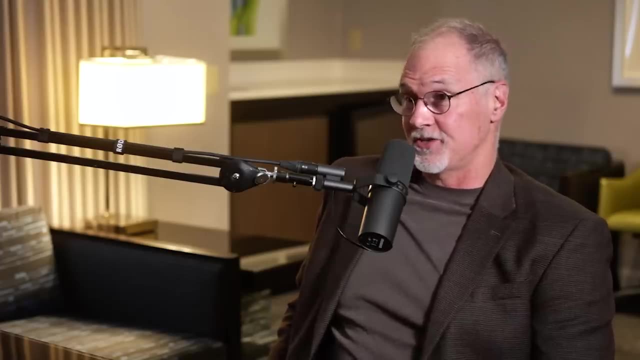 Curl bench Probably can't curl as much as we can yet. but a metric that I think is interesting is: um you know, another way of of looking at that strength is, you know, the box jump? So if, how high of a box can you jump onto? 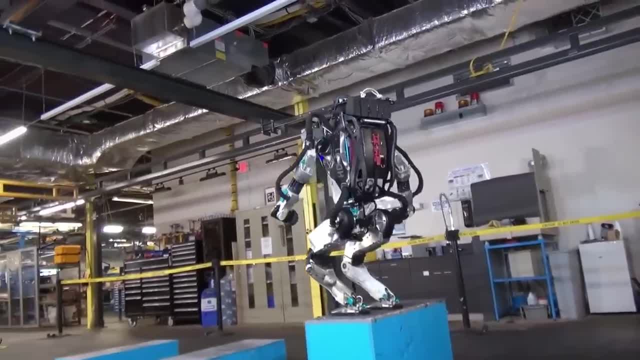 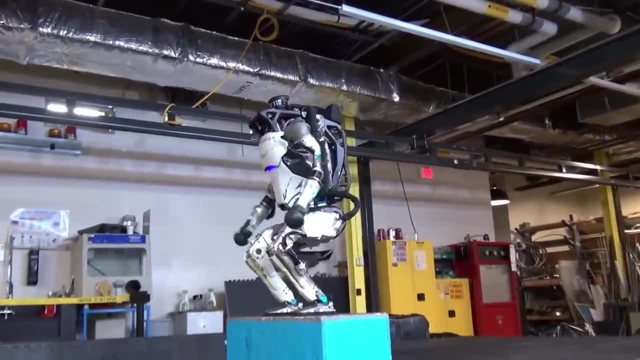 Question. And uh, Atlas- I don't know the exact height, It was probably a meter high or something like that- It was a pretty, pretty tall jump that Atlas was able to manage. uh, when we last tried to do this, 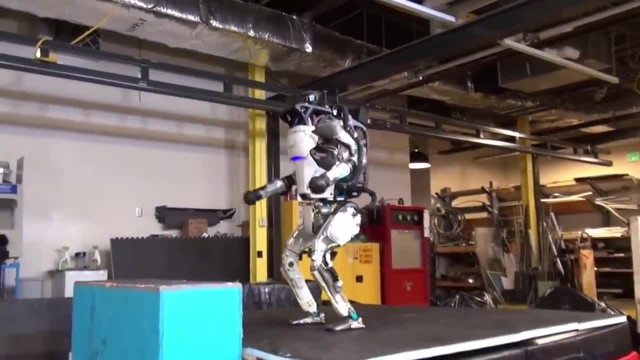 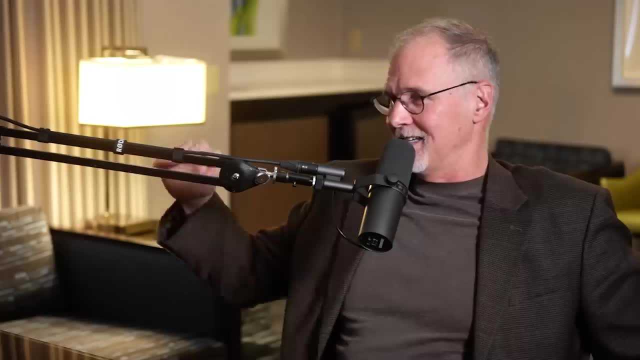 And, and I have video of, uh, my chief technical officer- Okay, Do you know how tall that is? Yeah, Doing the same jump And he really struggled, you know, to get up to human but the human getting all the way on top of this box. but then you know, Atlas was able to do it. 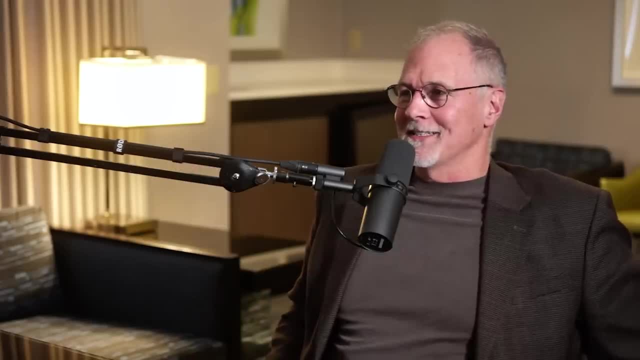 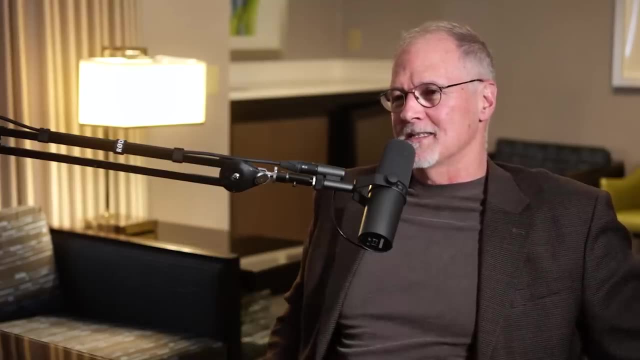 Um, we're now thinking about the next generation of Atlas and we're probably going to be in the realm of a person can't do it. you know, with this, with the next generation, the robots, the actuators are going to get stronger, where there really is the case that at least some of these joints, some of these motions, will be stronger. 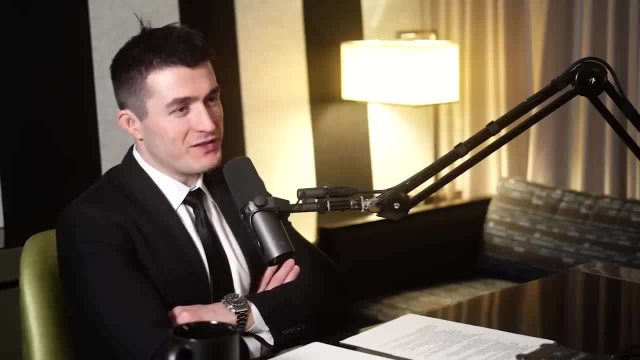 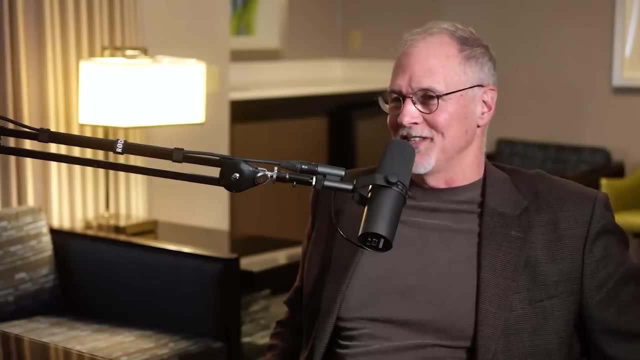 And to understand how high I can jump, you probably had to do quite a bit of testing. Oh yeah, And there's lots of videos of it trying and failing, And that's you know. that's all you know. we don't always release those, those videos, but they're a lot of fun to look at. 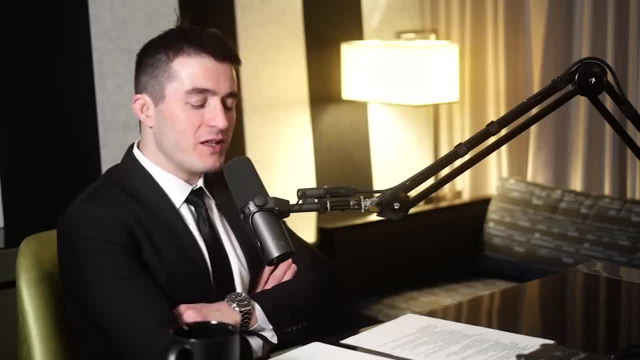 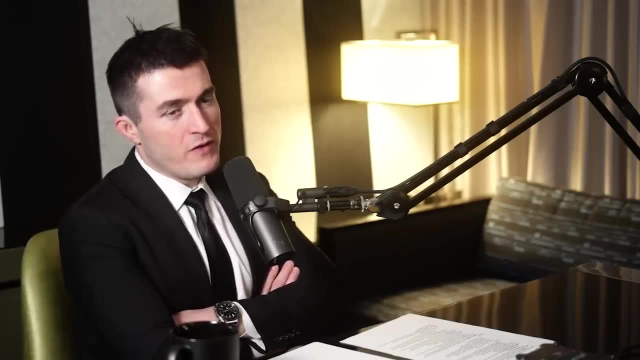 Uh, so we'll talk a little bit about that. Uh, but if can you talk to the jumping Cause you talked about the walking and it took a long time, many, many years- to get the walking to be natural, but there's also really natural looking, uh, robust, resilient jumping. 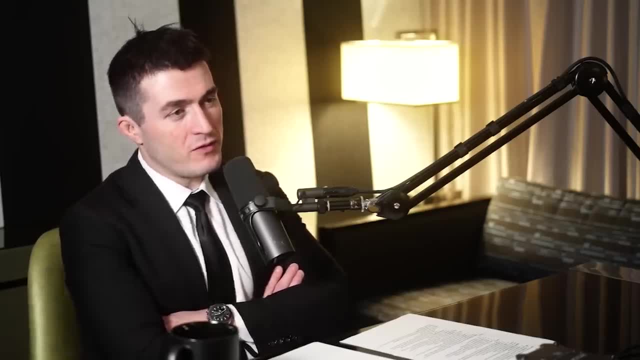 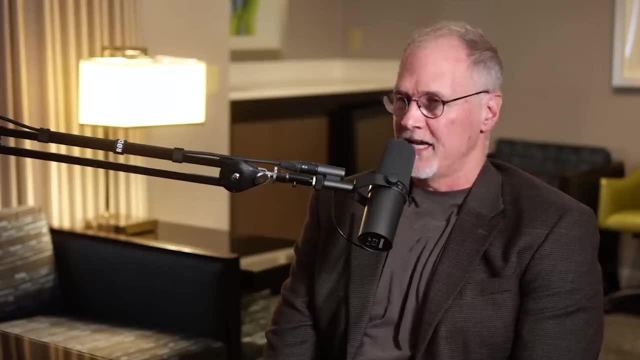 How hard is it to do the jumping? Well, again, this, This stuff has really evolved rapidly in the last few years. I you know, the first time we did a somersault, um, you know, there was a lot of kind of manual iteration. 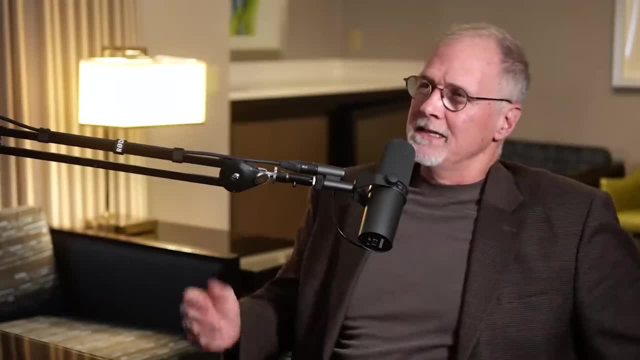 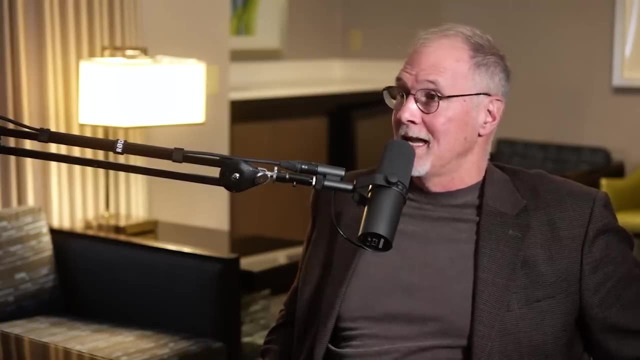 What is the trajectory? you know how hard do you throw you? In fact, in these early days- uh, I actually would- when I'd see early experiments that the team is doing, I might make suggestions about how to change the technique, again kind of borrowing from my own intuition about how backflips work. 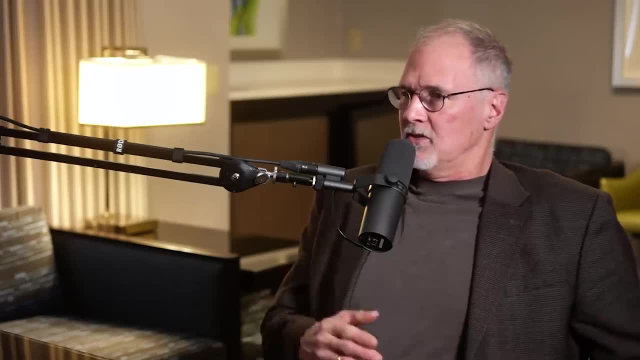 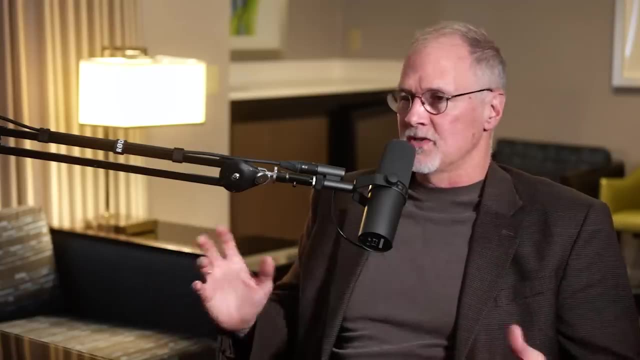 Um, but frankly they don't need that anymore. So in the in the early days you had to iterate kind of in almost a manual way, trying to change these trajectories of the arms or the legs, uh, to try to get you know, a successful backflip to happen. 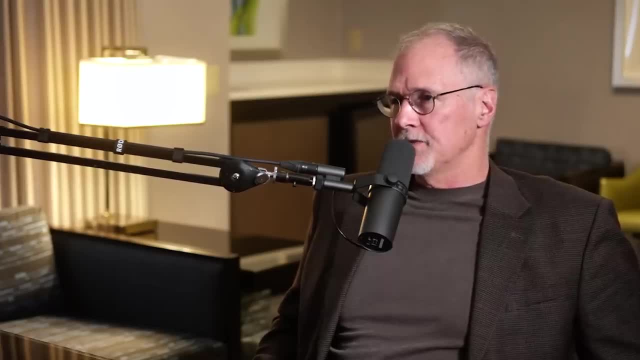 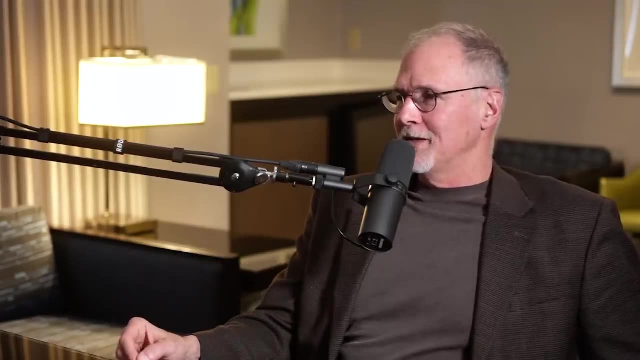 Um, but more recently we're running these model predictive uh uh control techniques where we're able to the robot essentially can think in advance for the next second or two about how its motion is going to transpire. And you can. 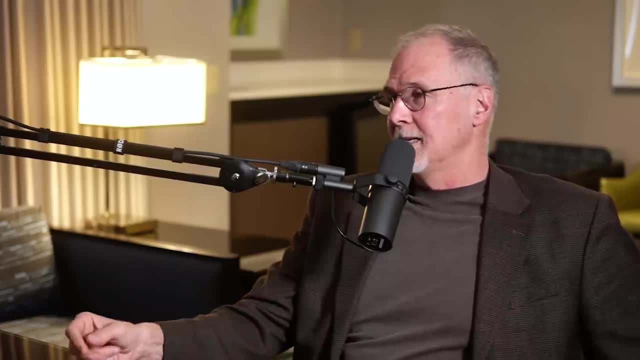 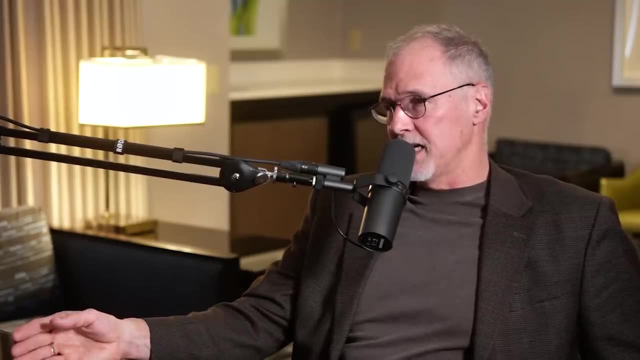 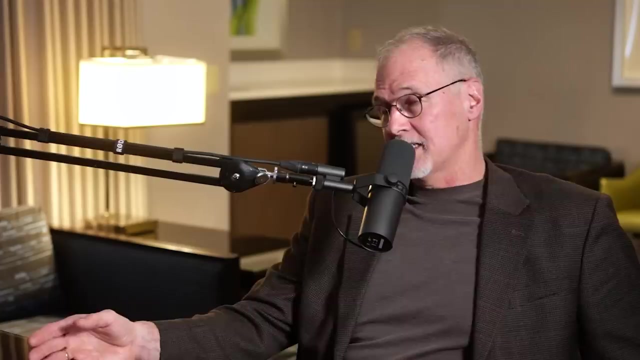 You know, solve for optimal trajectories to get from A to B. So this is happening in a much more natural way And we're really seeing an acceleration happen in the development of these behaviors, again partly due to these um optimization techniques, uh, sometimes learning techniques. 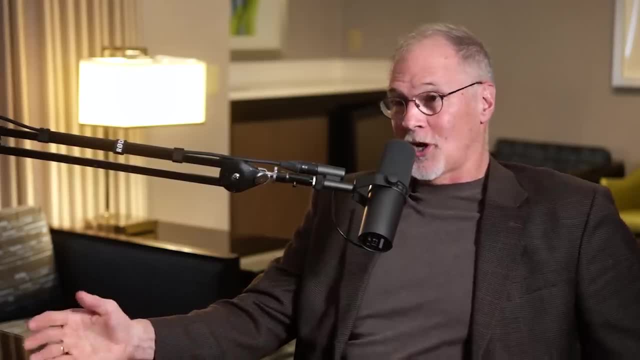 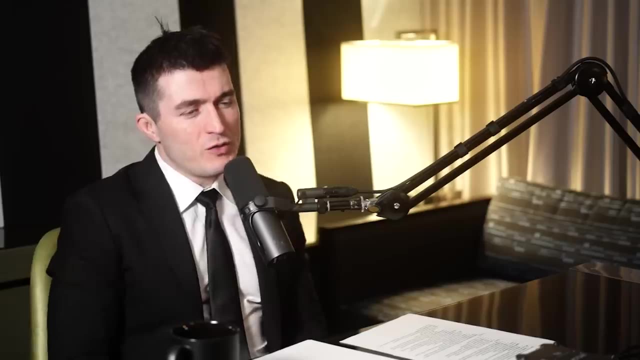 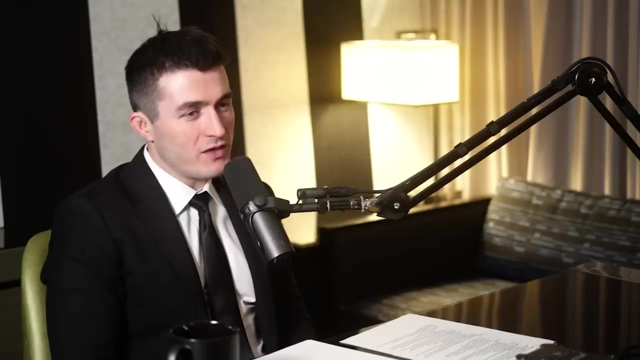 Um, so it's there's. it's hard in that there's a lot of mathematics and uh behind it. Um, but we're figuring that out So you can do model Predictive control for uh, I mean, I don't even understand what that looks like when the entire robot is in the air flying and doing a back. 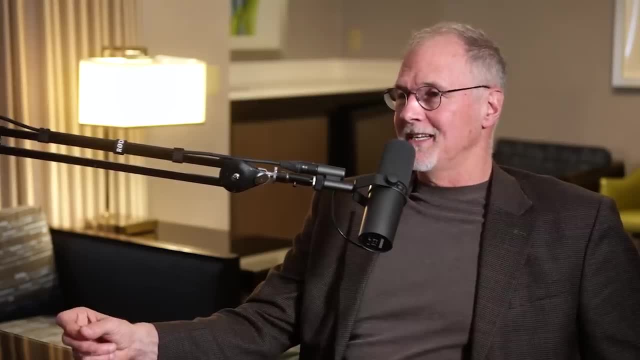 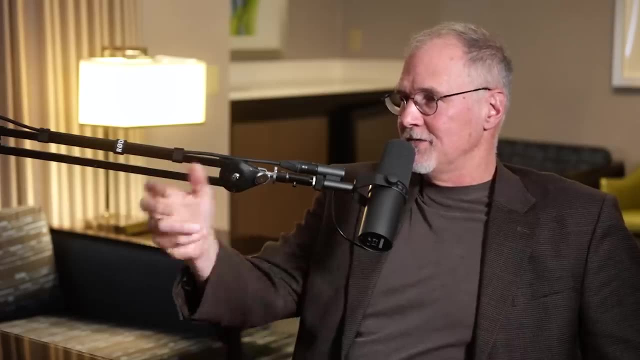 Yeah, I mean but, but. but that's the cool part, right? So you know you. you know the physics we we can calculate physics pretty well using you know Newton's laws about how it's going to evolve over time. 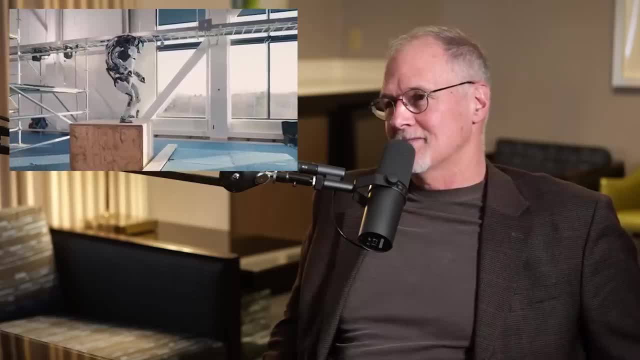 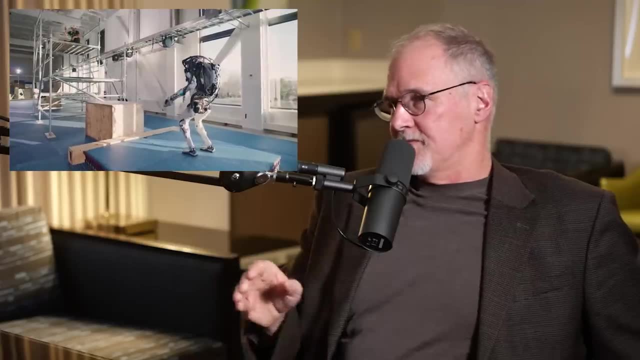 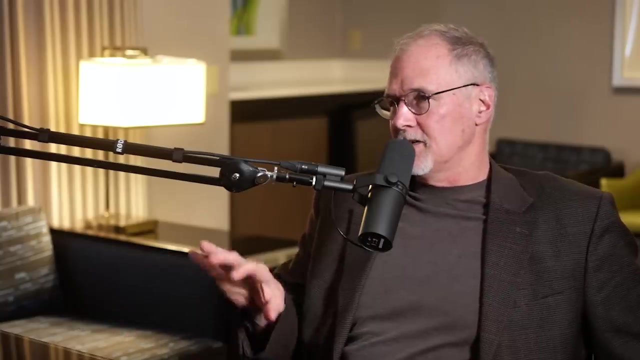 And the road here. this, this, the sick trick, which was a front somersault with a half twist, is a good example, right, But you saw the robot on various versions of that trick. I've seen it land in different configurations and it still manages to stabilize itself. 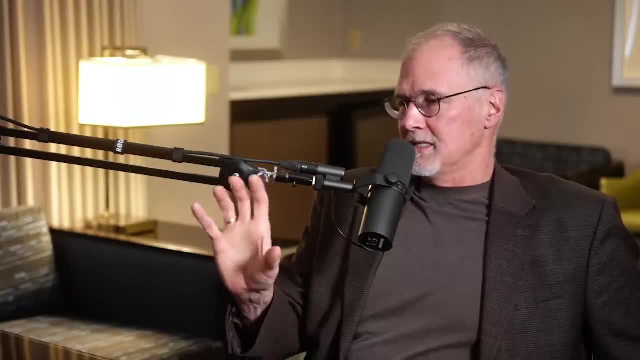 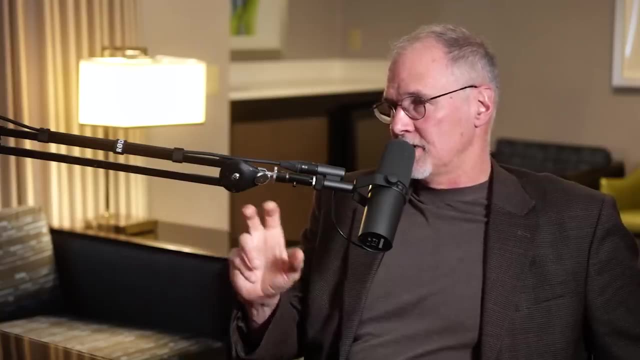 And so you know what this model predictive control means, is again the in real time, the robot is projecting ahead, you know, a second into the future and sort of exploring options. And if I, if I move my arm a little bit more this way, how is that going to affect the outcome? 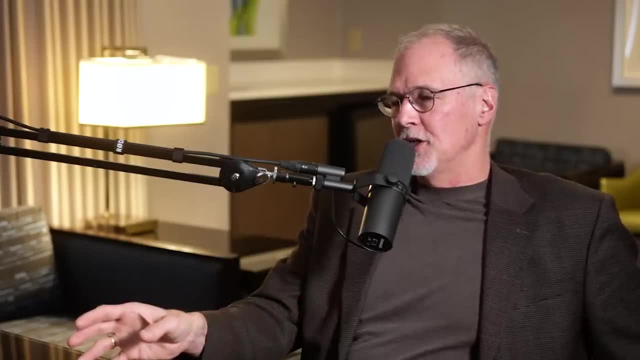 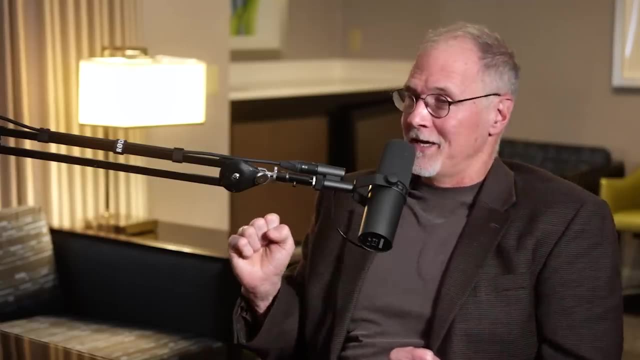 And so it can do these calculations- Many of them You know, uh- and- and basically solve where you know. given where I am now- maybe I took off a little bit screwy from how I had planned- I can adjust. 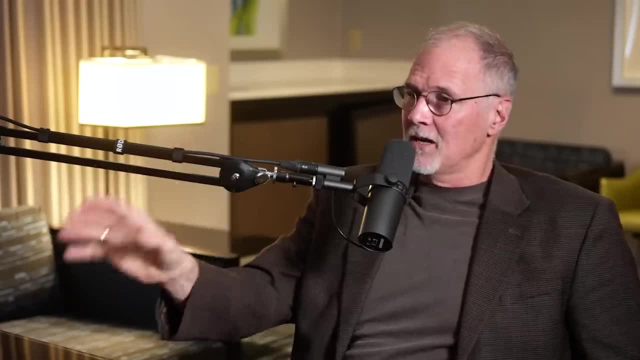 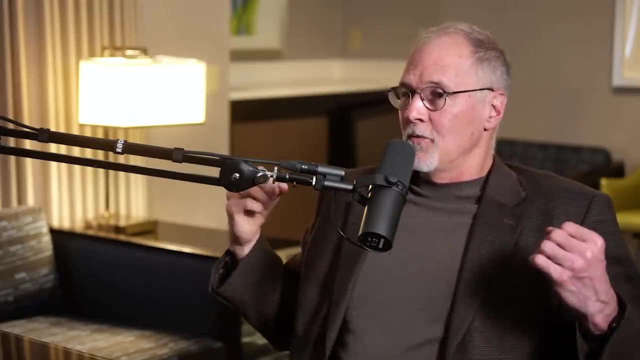 So you're adjusting in the air, just on the fly. So the the model predictive control lets you adjust on the fly And of course- I think this is what you know- people adapt as well. We, we, when, when we do it, even a gymnastics trick, we try to set it up. 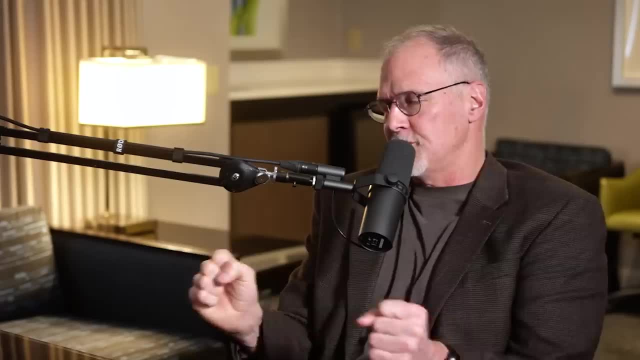 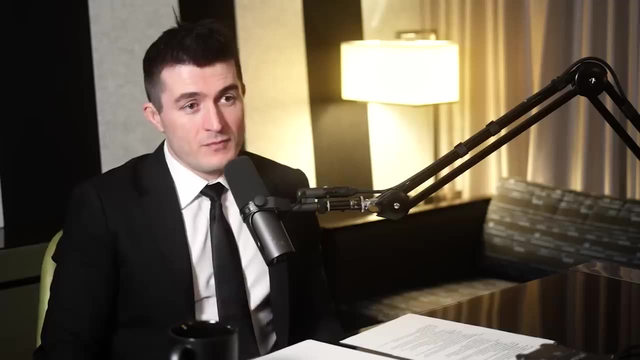 So it's as close to the same every time. but we figured out how to do some adjustment on the fly, And now we're starting to figure out that the robots can do this adjustment on the fly as well, Using these techniques in the air. 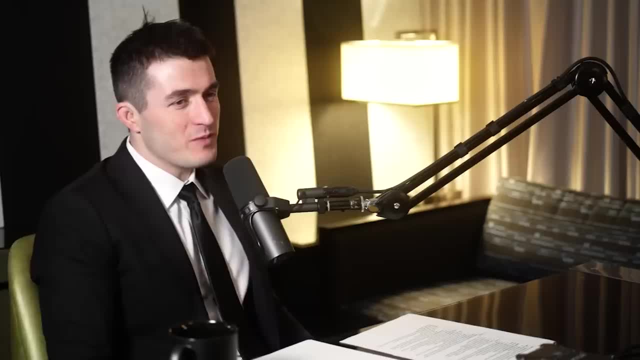 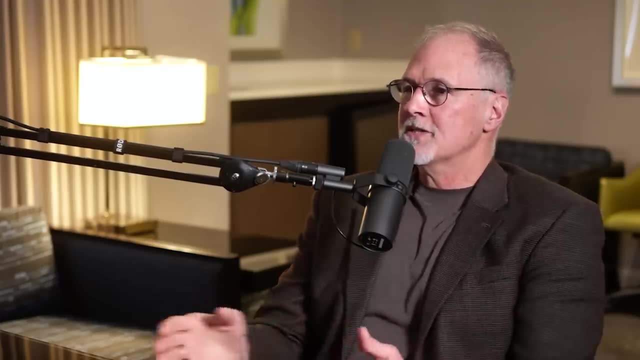 It's so. I mean it just feels, from a robotics perspective, just surreal. Well, that's sort of the you talked about underactuated, right? So when you're, when you're in the air, there's something. there's some things you can't change, right. 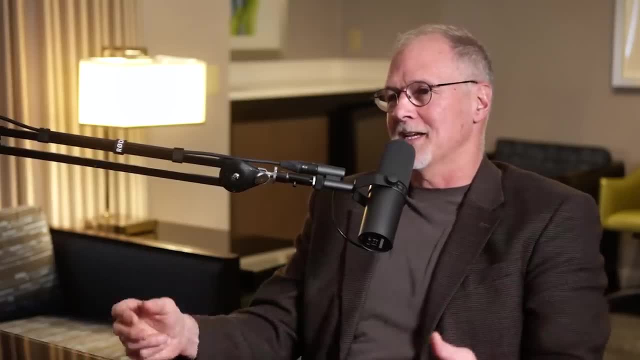 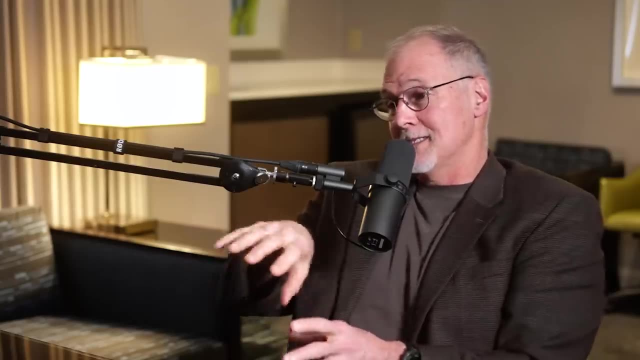 You can't change the momentum while it's in the air, Cause you can't apply an external force or torque, And so the momentum isn't going to change. So how do you work, within the constraint of that fixed Momentum, to still get from A to B, where where you want to be? 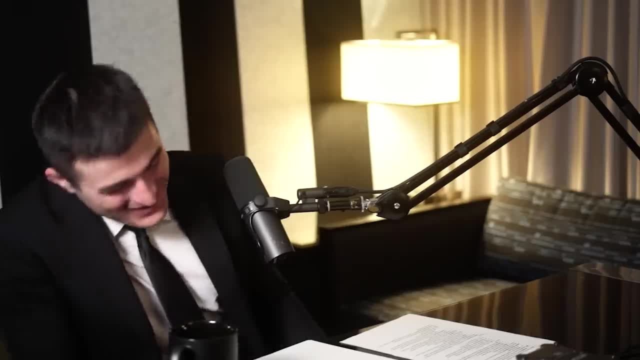 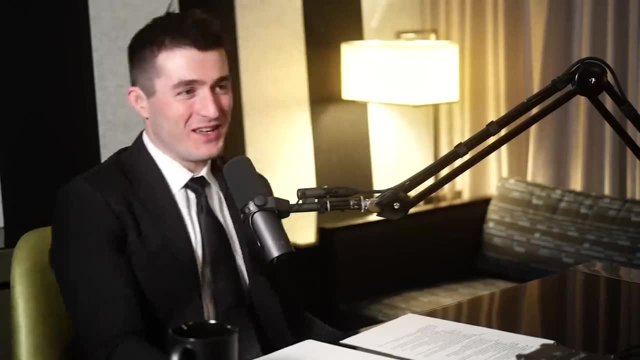 That's really undirected. You're in the air. I mean you become. you become a drone for a brief moment in time. No, you're not even a drone, Cause you can't, you can't hover, You can't go to. you're going to impact soon. 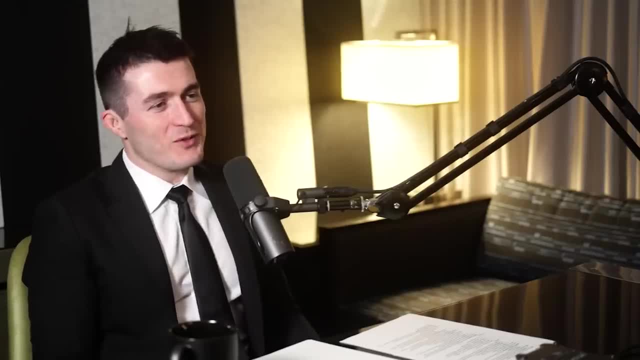 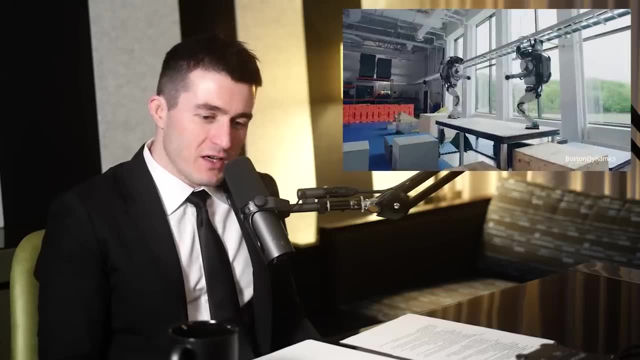 Be ready. Are you considered like a hover type thing or no, no, it's too much weight. I mean it's just, it's just incredible. I uh it just even to have the guts to try back flip. It was such a large body. 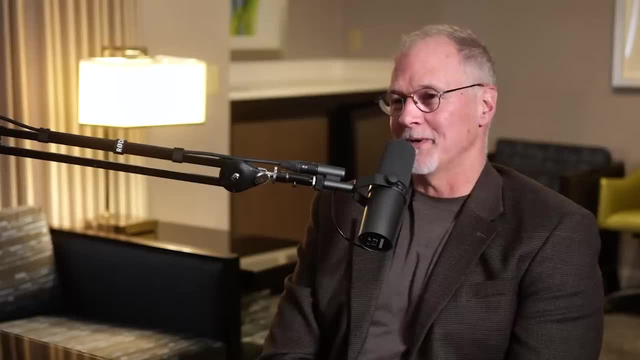 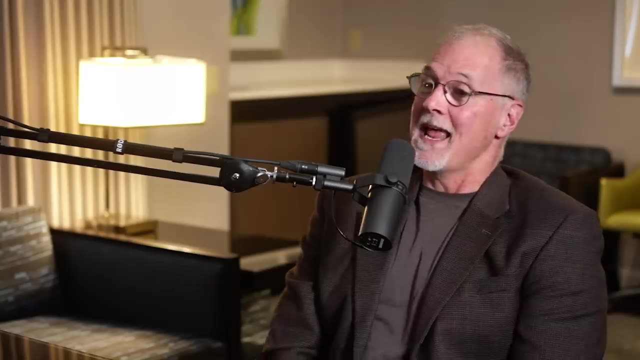 That's wild, but like uh, we definitely broke a few robots, but that's where the build it, break it, fix it. you know, uh strategy comes in and you gotta be willing to break And what ends up happening is you end up by breaking the robot repeatedly. 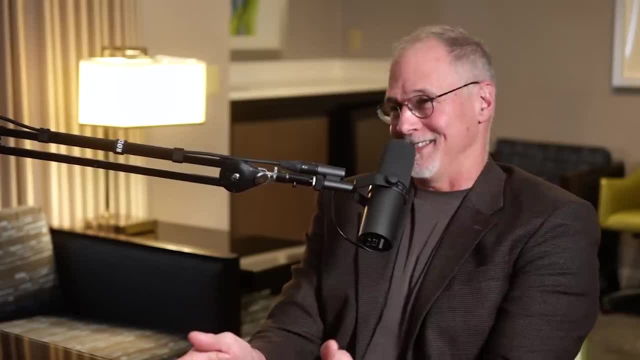 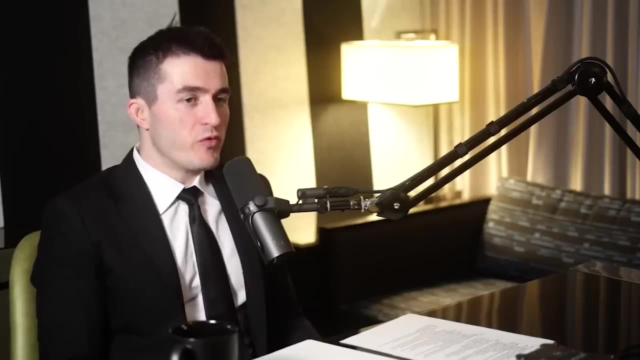 you find the weak points and then you end up redesigning it So it doesn't break so easily next time. you know, through the breaking process you learn a lot, like a lot of lessons, And you keep improving, not just how to make the back flip work. 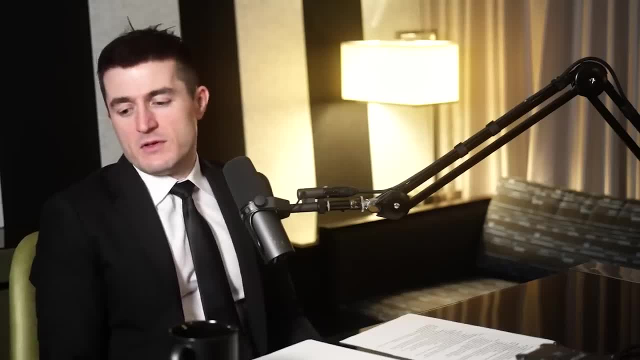 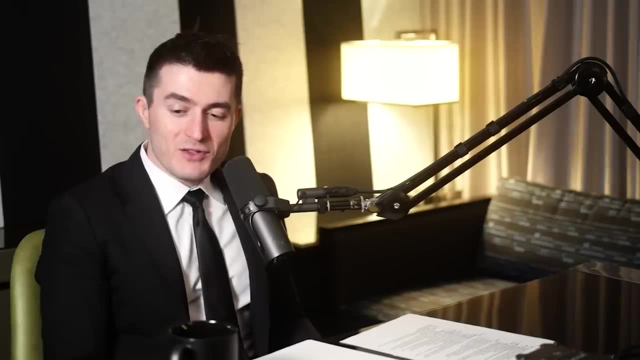 but everything and how to build the machine better. Yeah, Yeah, I mean, is there something about just the guts to come up with an idea of saying, you know what, let's try to make it to a back flip? Well, I think the courage to do a back flip in the first place and and to 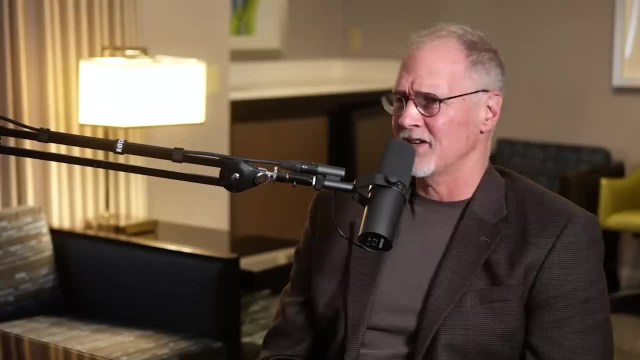 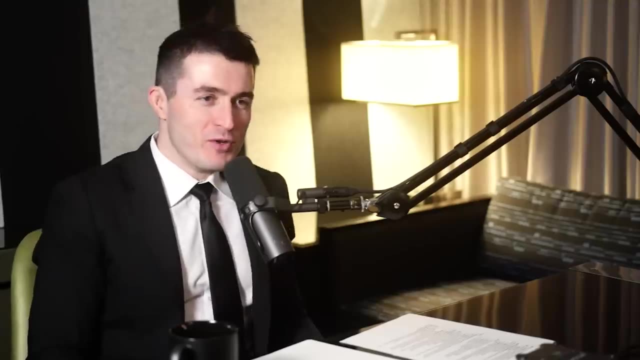 not worry too much about the ridicule of somebody saying: why the heck are you doing back flips with robots? Because a lot of people have asked that. you know why, why. why are you doing this? I go to the moon in this decade and do the other things. 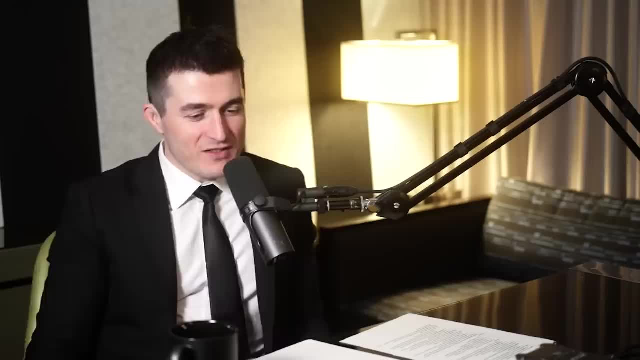 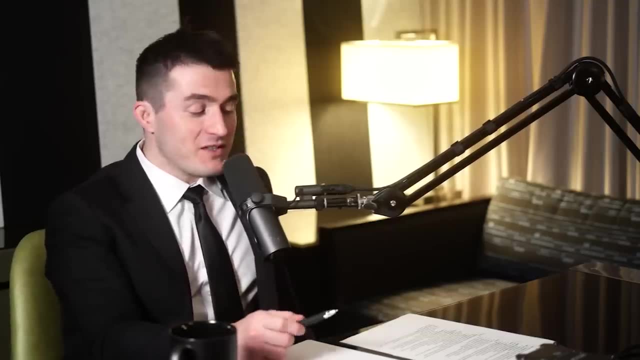 Yeah, Yeah, Okay, Not because it's easy, because it's hard. Yeah, exactly, Don't ask questions, Okay. So the, the jumping, I mean it's just, there's a lot of incredible stuff. If we can just rewind a little bit to the DARPA robotics challenge in 2015,, I 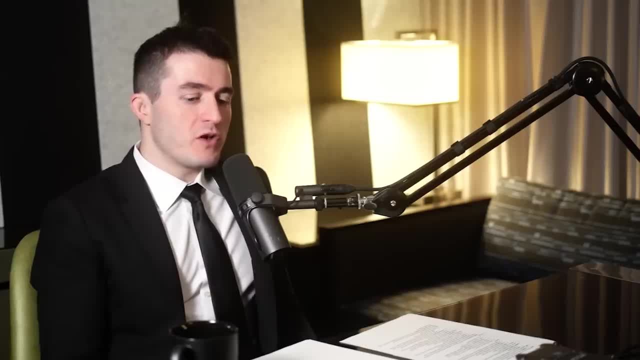 think, which was for people who are familiar with the DARPA challenges. it was first with autonomous vehicles And there's a lot of interesting challenges around that, And the DARPA robotics challenge. It was when, uh, humanoid robots were tasked to do all kinds of uh, you know. 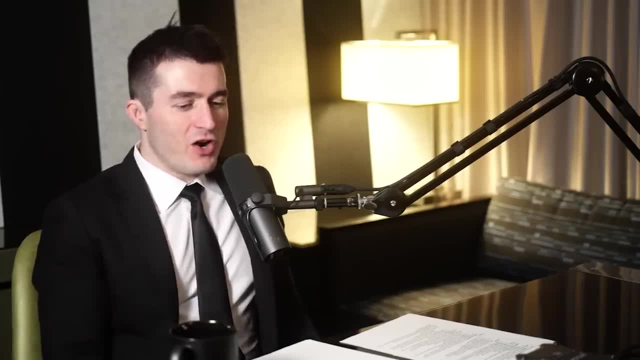 manipulation, walking, driving a car, all these kinds of challenges with, if I remember correctly, sort of some slight capability to communicate with humans. but uh, the communication was very poor. So basically it has to be almost entirely autonomous. You can have periods where the communication 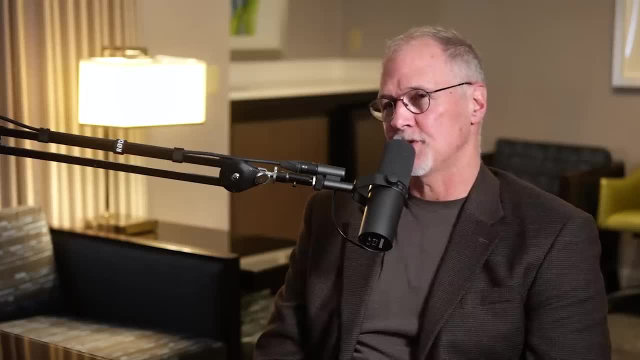 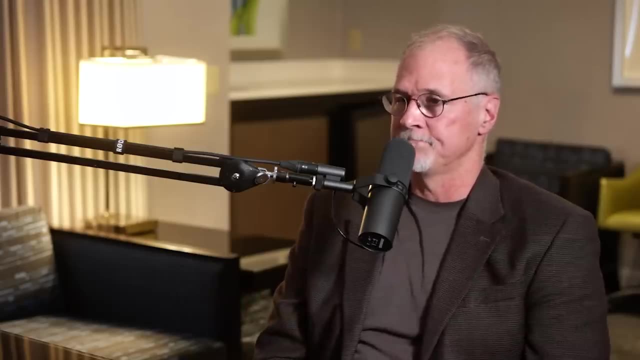 Was entirely interrupted and the robot had to be able to proceed. but you could provide some high level guidance to the robot, basically low, low bandwidth communications to steer it. I watched that challenge with kind of tears in my eyes eating popcorn, but it 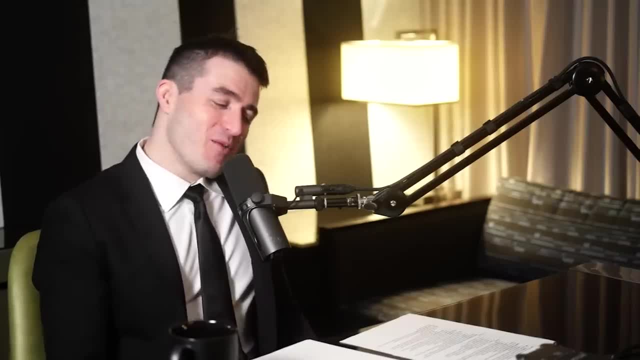 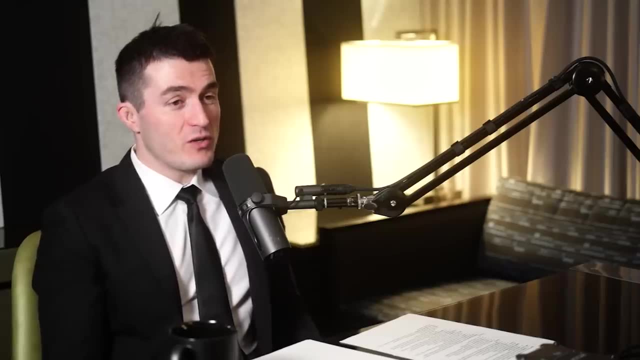 was hard, but I wasn't personally losing- uh, you know, hundreds of thousands, millions of dollars and many years of incredible hard work by some of the most brilliant roboticists in the world. So that that was why The tragic, well, that's why the tears came. 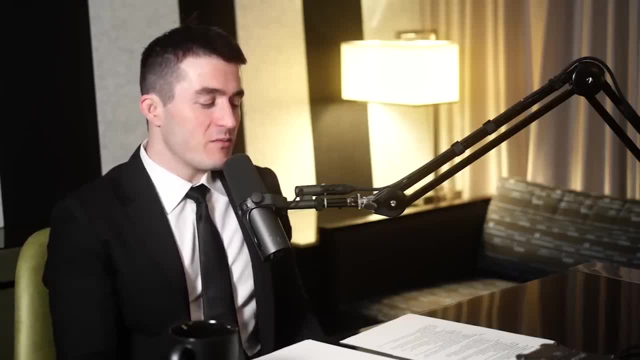 So, anyway, what, what have you? um, just looking back to that time, what have you learned from that experience? I mean, maybe if you could describe what it was, uh, sort of the setup for people who haven't seen it. well, so there was a contest where a bunch of 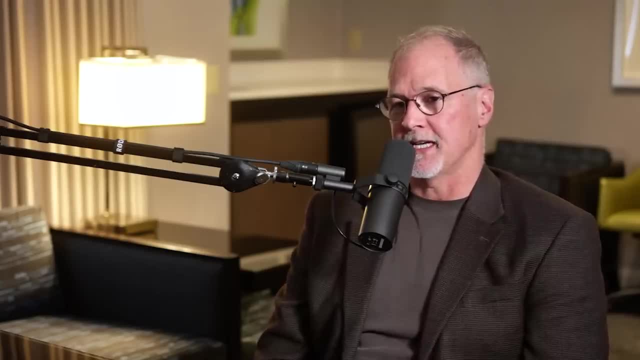 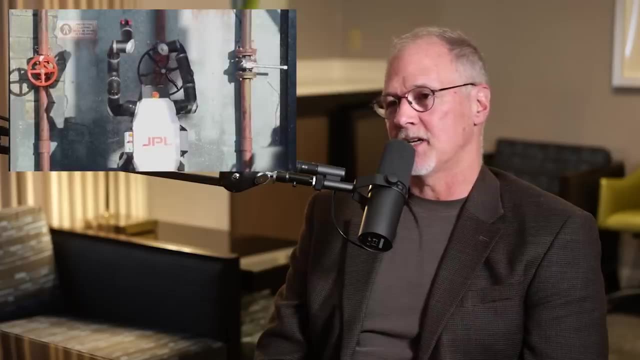 different um, robots were asked to do a series of tasks. uh, some of those that you mentioned: drive a vehicle, get out, open a door, go identify a valve, shut a valve, use a tool to maybe cut a hole. 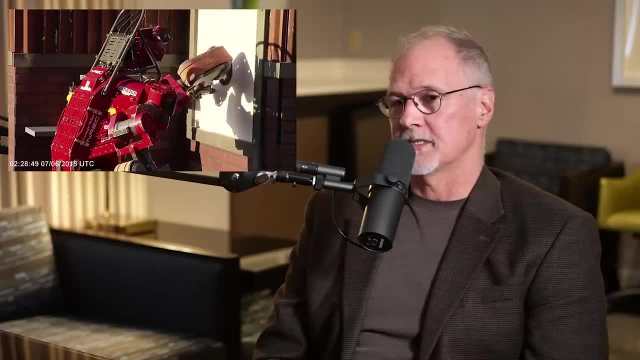 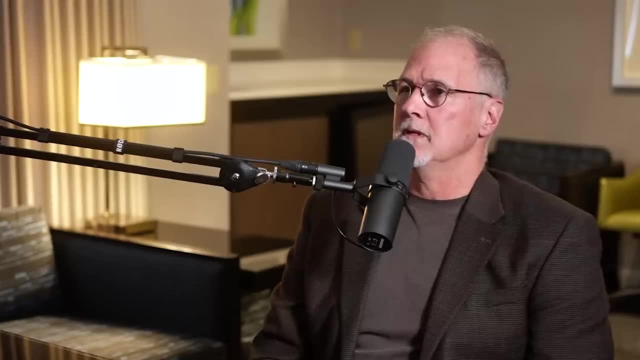 And um a surface and then crawl over some stairs and maybe some rough terrain. So it was the idea was have a, a general purpose robot that could do lots of different things. um had to be mobility and manipulation on board perception. 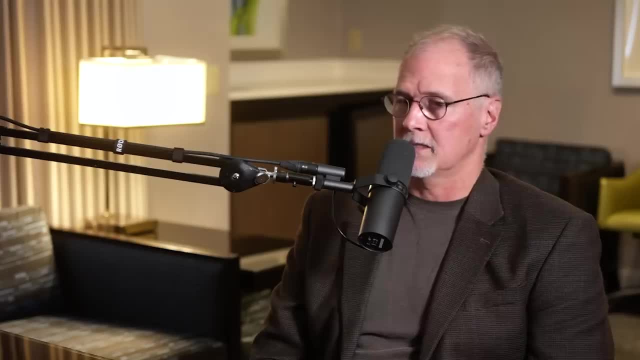 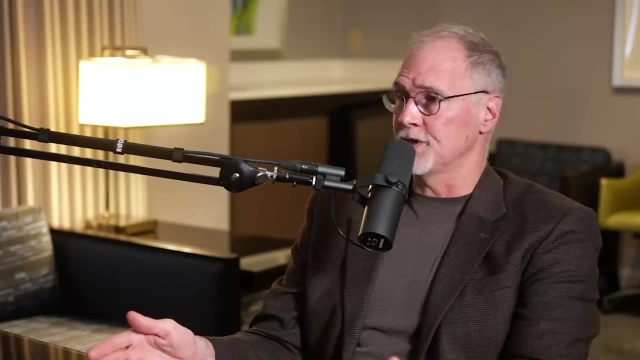 And there was a contest, uh, which DARPA likes, uh, at the time was running sort of follow on to the Yeah, Yeah, The grand challenge which was: let's, let's try to push vehicle autonomy along Right. 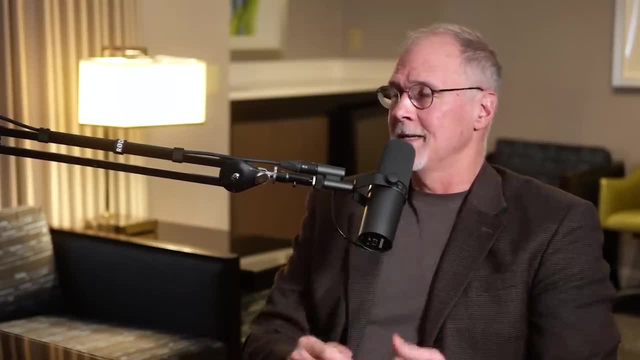 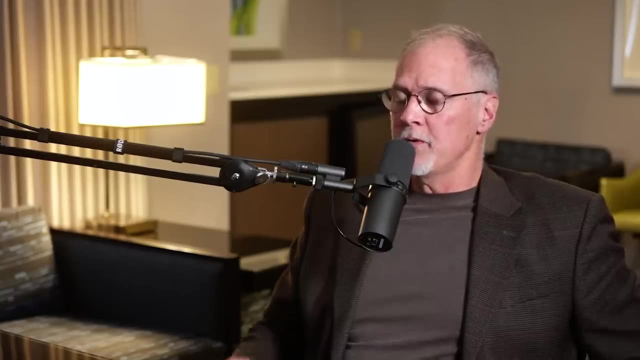 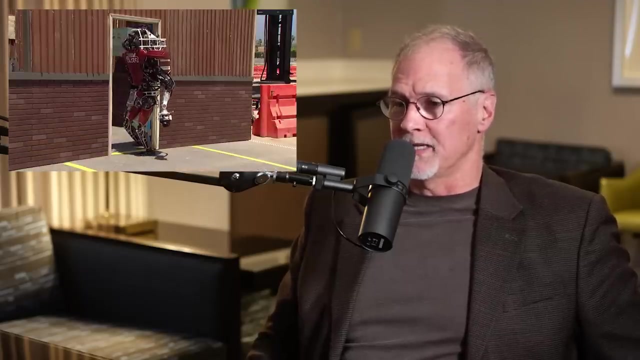 They, they, they encourage people to build autonomous cars, So they're trying to basically push an industry forward. And um, uh, we were asked our role in this was to build um a humanoid. at the time it was our sort of first generation Atlas robot. 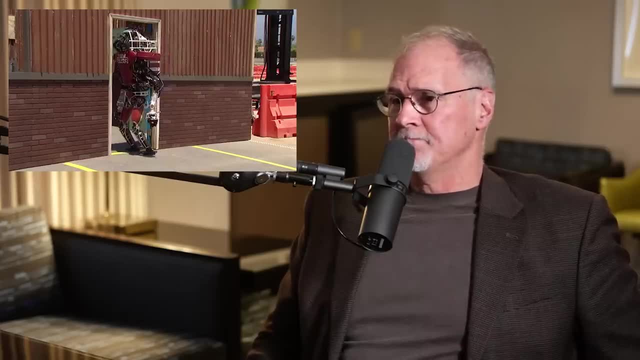 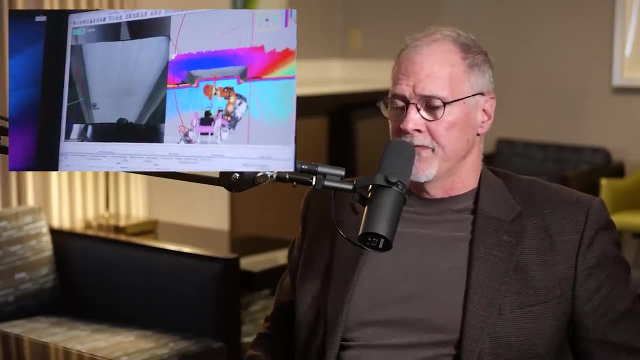 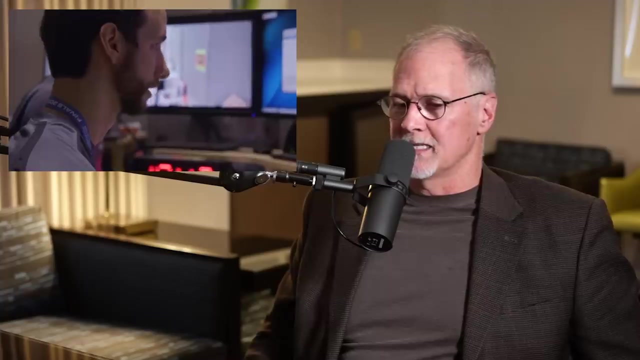 And we built maybe 10 of them, I don't remember the exact number- Uh, and DARPA distributed those to various teams. um, that sort of won a contest. uh showed that they uh, could you know, program these robots and then use them to compete. 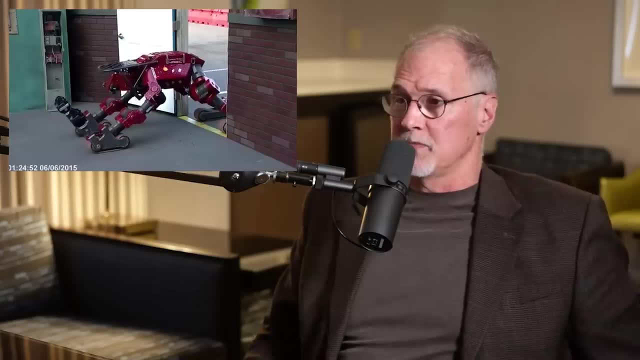 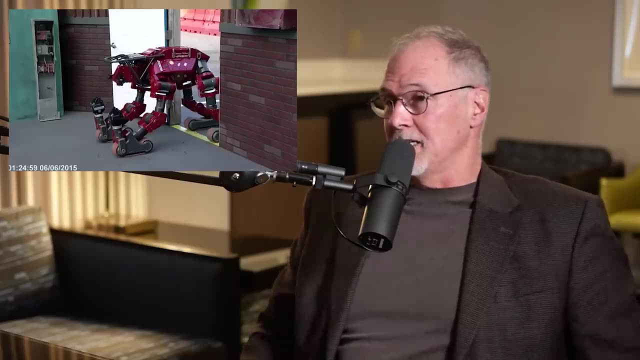 against each other, And then other robots were introduced as well. Some teams built their own robots. Carnegie um Mellon, for example, built their own robot And uh, and all these robots competed to see who could sort of get through this. this. 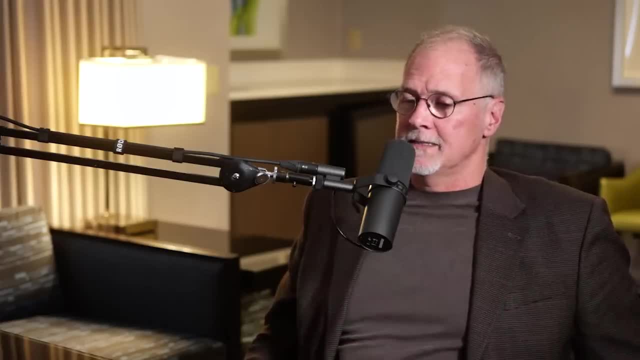 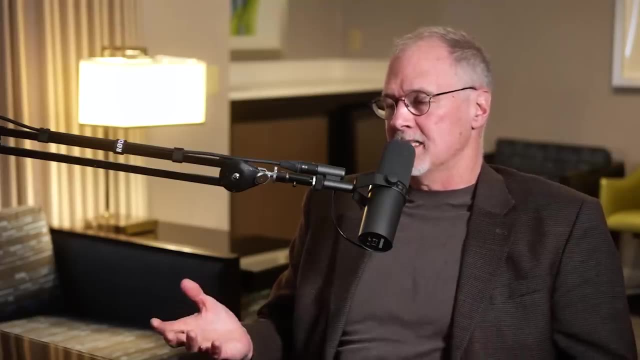 maze um the fastest And uh And um again. I think the purpose was to kind of push the whole industry forward. Uh, we provided the robot and some baseline software, but we didn't. we didn't actually. 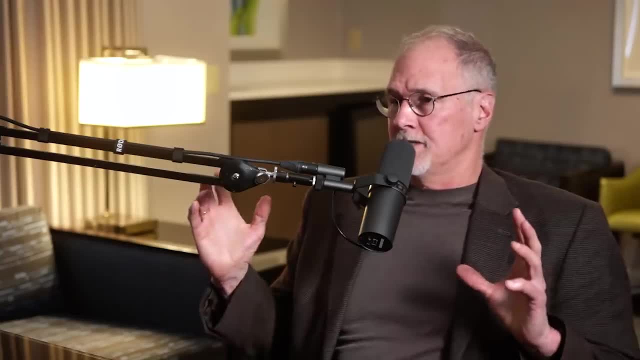 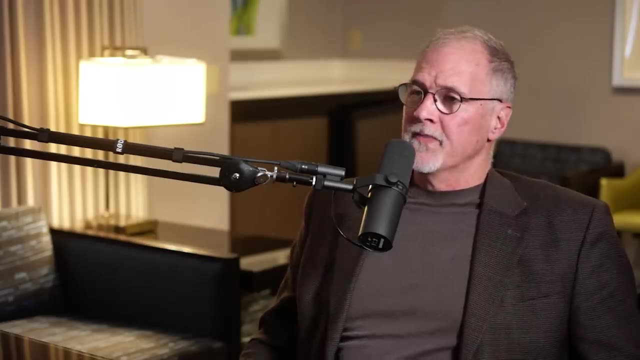 compete as a participant, uh, where we were trying to, uh, you know, drive the robot through this maze. Uh, we were just trying to support the other teams. It was humbling because it was. it was really a hard task. 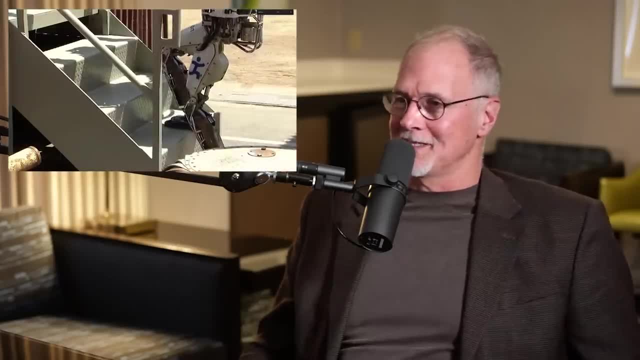 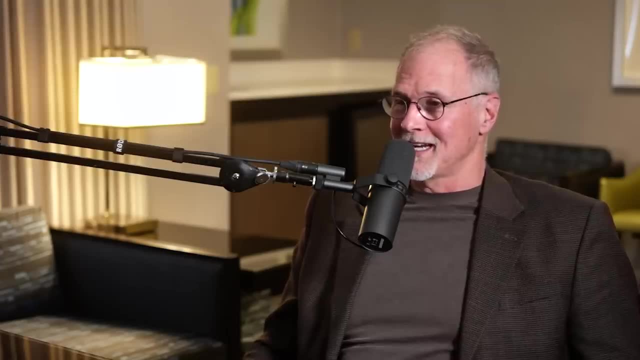 And and, honestly, the robots, the tears were because mostly the robots didn't do it. You know they fell down, You know, uh, repeatedly, um, it was hard to get through this contest. Uh, you know some did and and you know they were rewarded and won, but it was humbling. 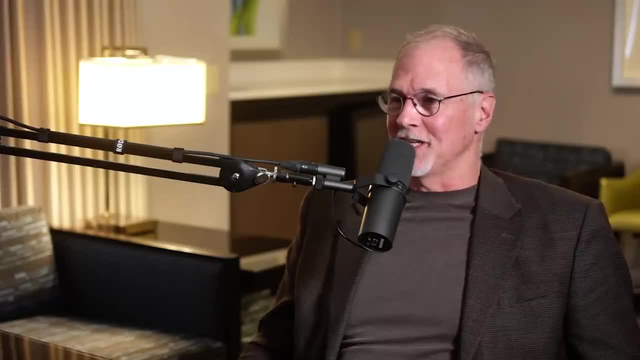 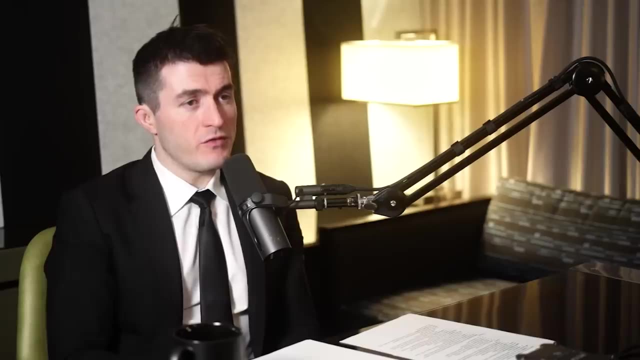 because of just how hard these tasks weren't all that hard. A person could have done it very easily, Um, but it was really hard to get the robots to do it. you know the general nature of it, the variety of it, the variety, and also that I don't know if the tasks were sort of 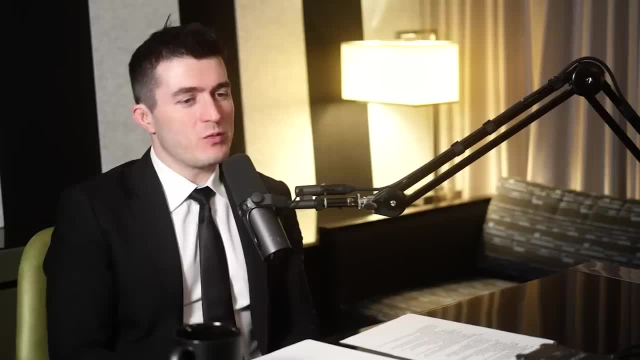 the task in themselves, Help us understand what is difficult and what is not. I don't know if that was obvious before the contest was designed, So you kind of try to figure that out. And I think Atlas is really a general robot platform and it's perhaps not best suited. 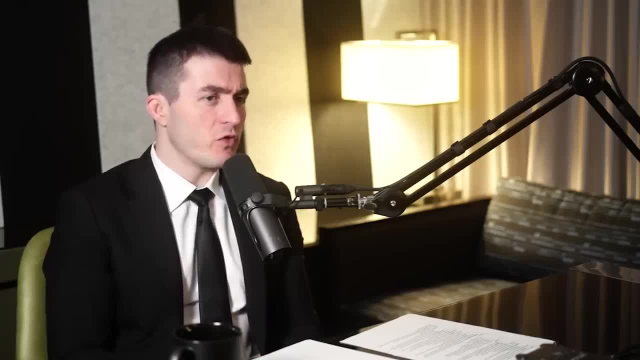 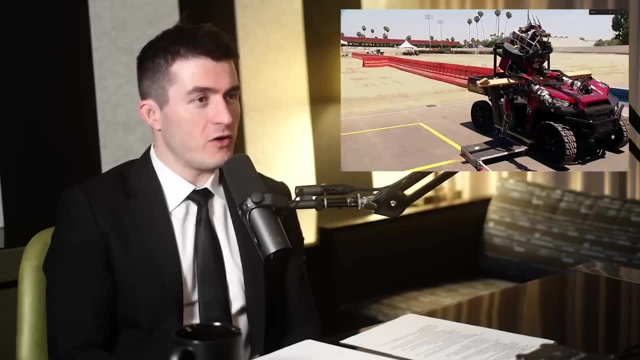 for the specific tasks of that contest, Like for just for example, probably the hardest task is not the driving of the car but getting in and out of the car. and Atlas, probably you know, if you had, if you had, if you had, I'm not sure. 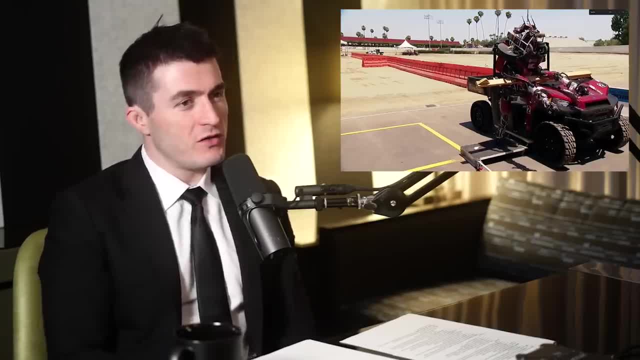 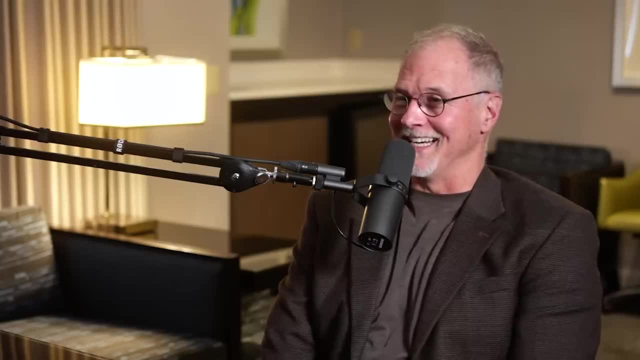 Yeah, You know, if you were to design a robot that can get into the car easily and get out easily, you probably would not make Atlas that particular car. Yeah, the robot was a little bit big to get in and out of that car right. 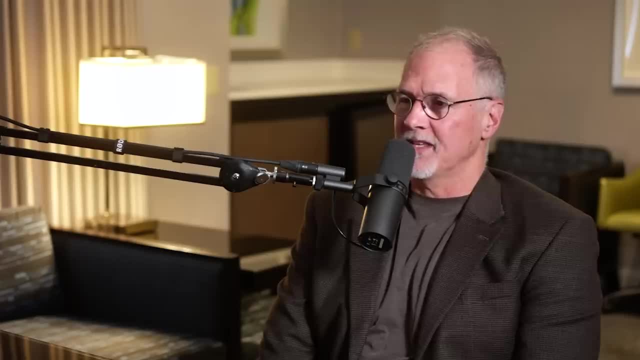 It doesn't fit. yeah, This is the curse of a general purpose robot: that they're not perfect at any one thing, but they might be able to do a wide variety of things, And that is the goal at the end of the day. 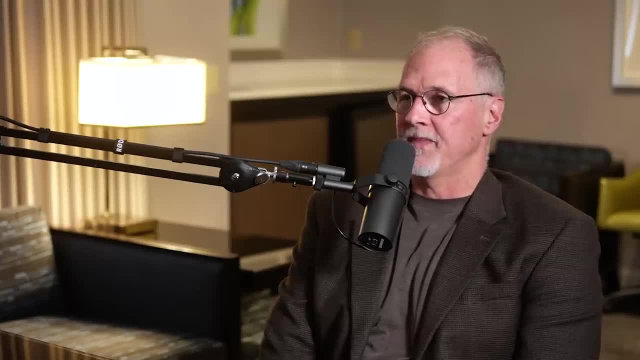 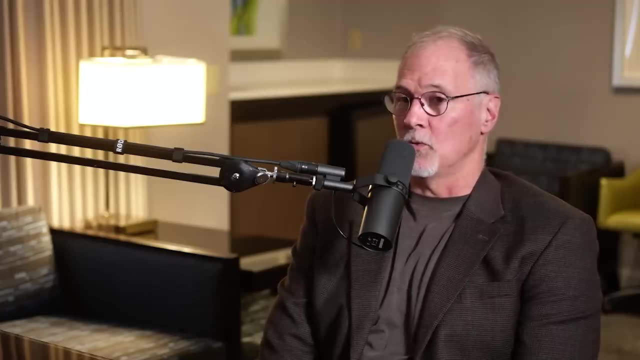 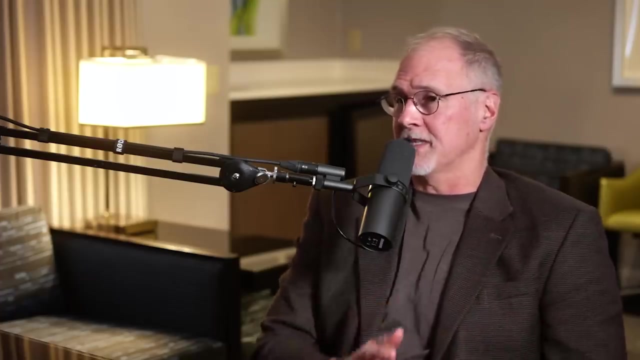 You know, I think we all want to build general purpose robots that can be used for lots of different activities. but it's hard And the wisdom in building successful robots up until this point have been: go build a robot for a specific task and it'll do it very well. 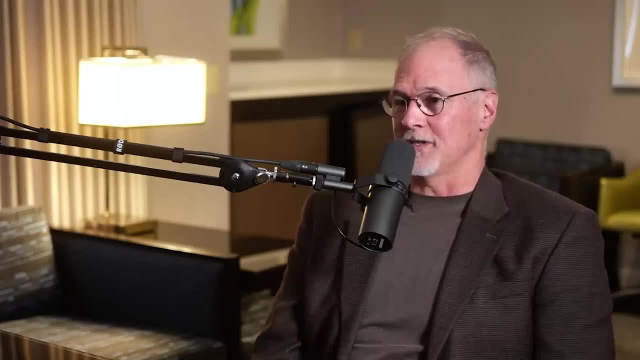 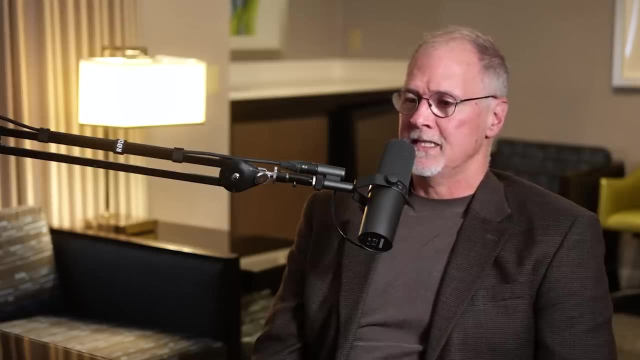 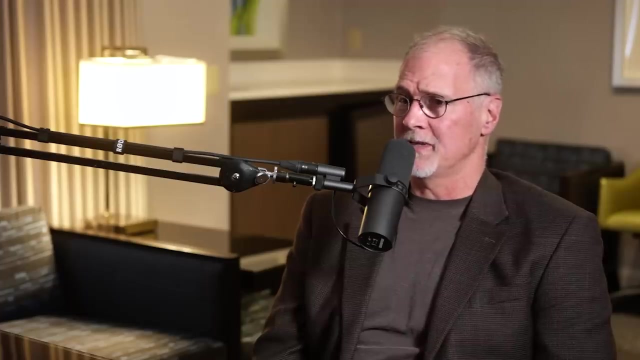 And as long as you control that environment, it'll operate perfectly. But robots need to be able to deal with uncertainty. If they're going to be useful to us in the future, They need to be able to deal with unexpected situations, and that's sort of the goal of a general purpose or multi-purpose robot, and that's just darn hard. 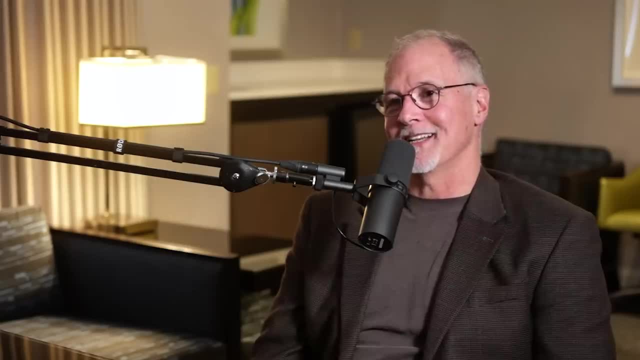 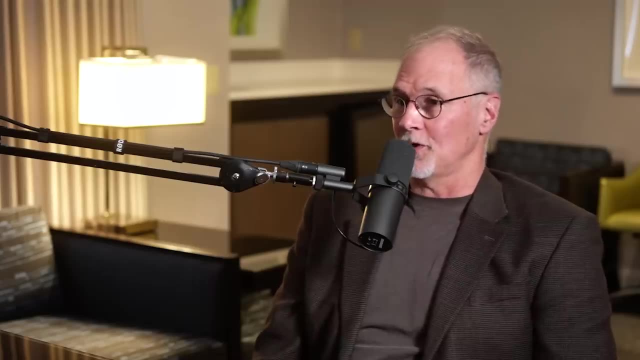 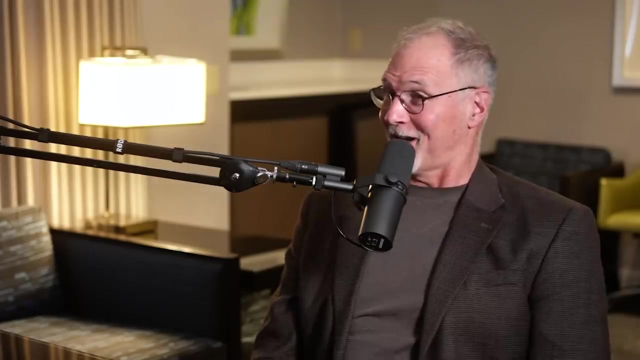 And so some of the others, these curious little failures, like I remember one of the a robot you know, the first, the first time you start to try to push on the world with a robot, you, you forget that the world pushes back and and will push you over if you're not ready for it. and the robot you know. 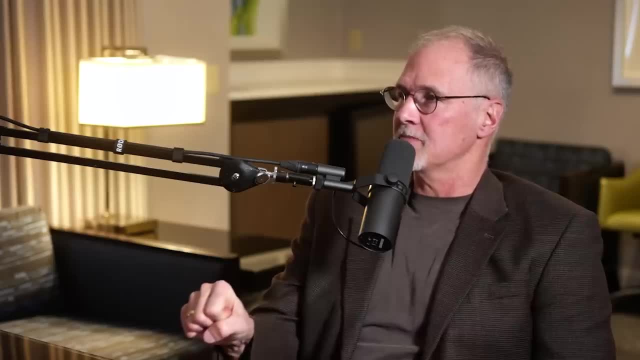 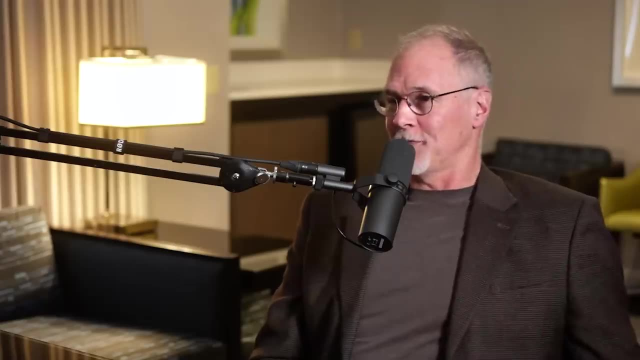 reach to grab the door handle. I think it missed the grasp of the door handle. Was expecting that its hand was on the door handle And so when it tried to turn the knob it just threw itself over. It didn't realize, oh, I had missed the door handle. 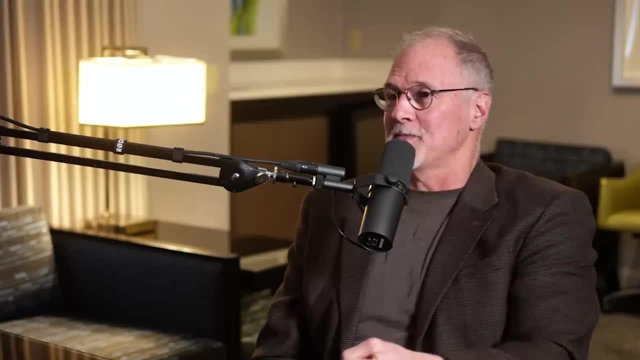 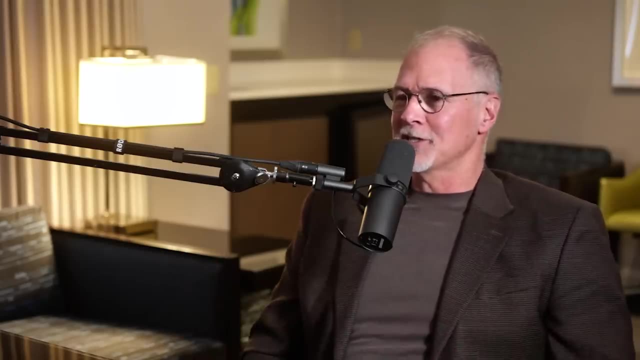 I didn't have. I didn't. I was expecting a force back from the door. It wasn't there, And then I lost my balance. So these little simple things that you and I would take totally for granted and deal with, the robots don't know how to deal with yet. 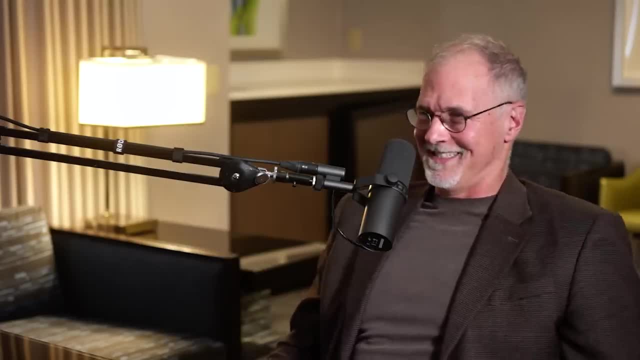 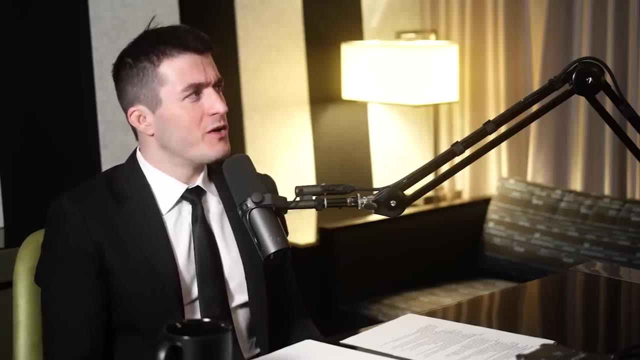 And so you have to start to deal with all of those Uh circumstances. Well, I think a lot of us experienced this in uh, even when sober, but drunk too. uh sort of you pick up a thing and expect it to be what is it? 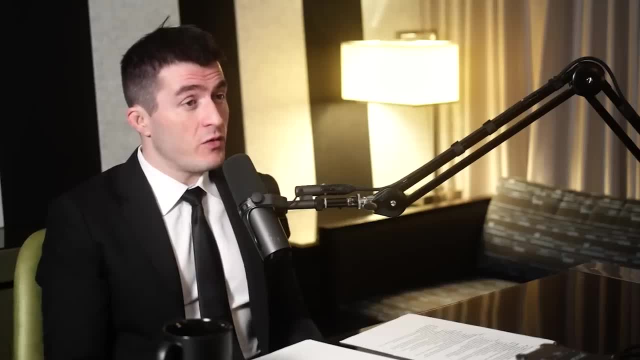 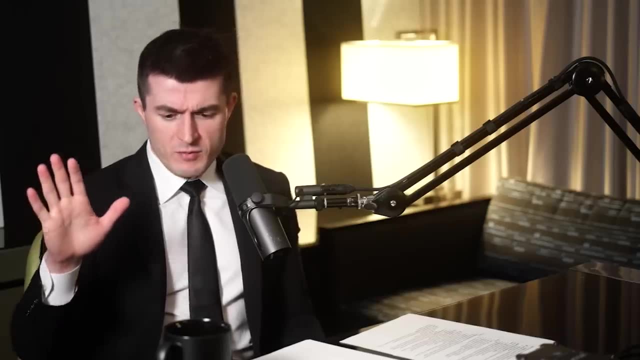 Heavy And it turns out to be light, Oh yeah, And then so the same. and, I'm sure, if your depth perception, for whatever reason, is screwed up, if you're, if you're drunk or some other reason, and then you think you're putting your hand on the table and you miss it. 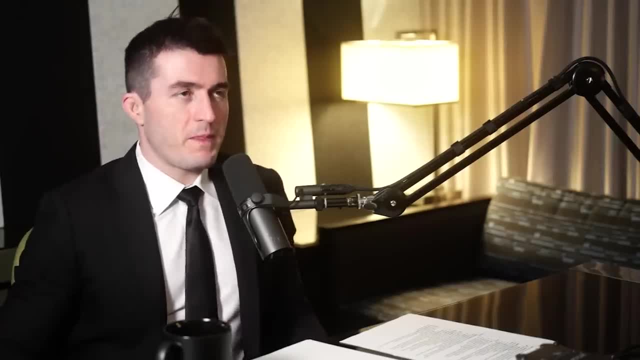 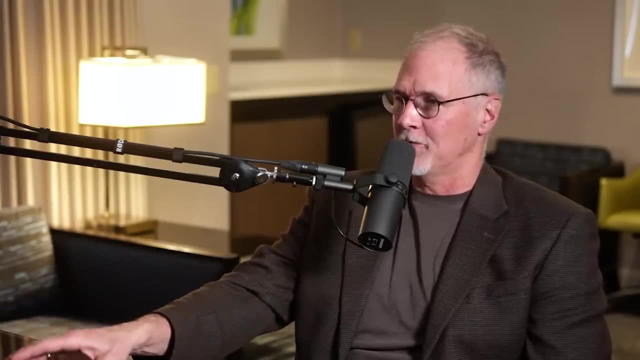 I mean, it's the same kind of situation, Yeah, Um, but there's, Which is why you need to be able to predict forward just a little bit, And so that's where this model of predictive control stuff comes in: predict forward what you think's gonna happen. 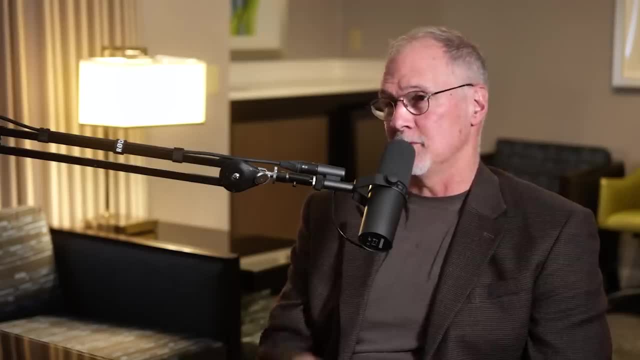 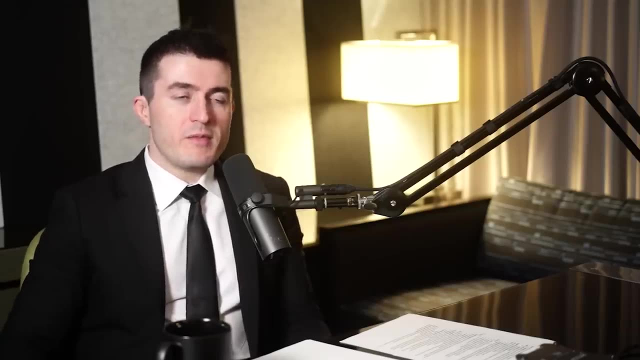 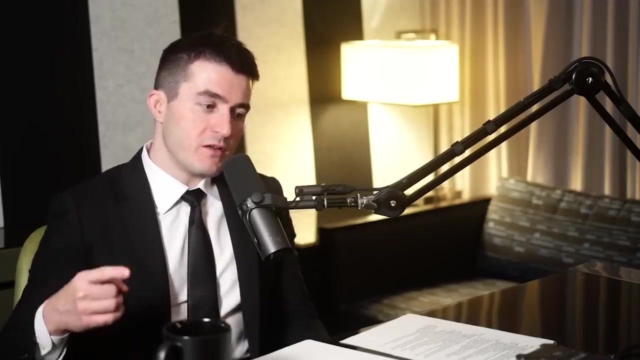 And then if and if that does happen, you're in good shape. If something else happens, you better start predicting again. So, re like, re, re, uh, regenerate a plan, Yeah, When you don't, I mean that. um, that also requires a very uh fast feedback loop of updating uh what you're putting. 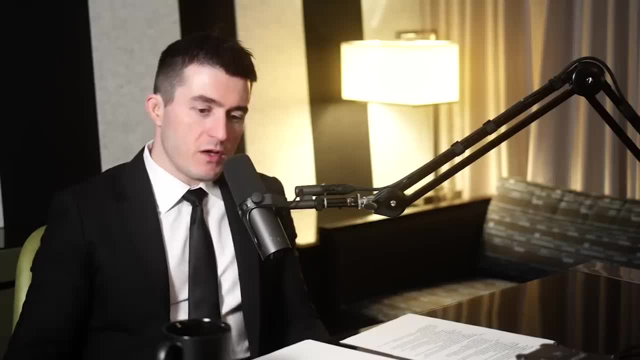 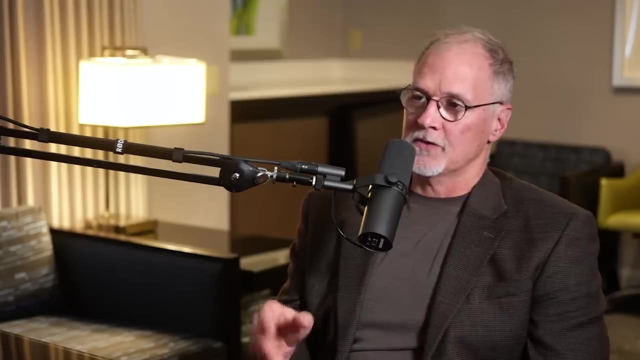 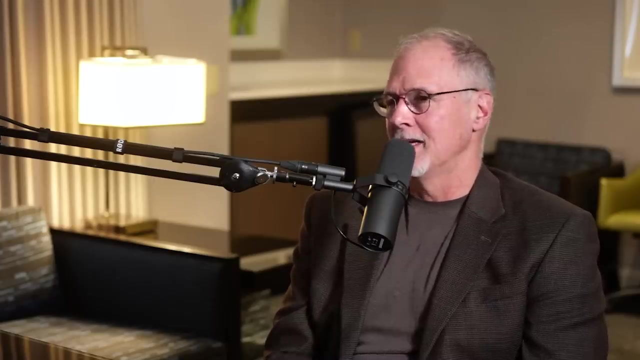 Your prediction how it matches to the actual real world. Yeah, Those things have to run pretty quickly. What's the challenge of running things pretty quickly, A thousand Hertz, of acting and sensing quickly? You know there's a few different layers of that. you you want at the lowest level, you like to run things typically at around a thousand Hertz, which means that you know at each joint of the robot you're measuring position or force and then trying to control your actuator. Whether it's a Hydraulic or electric motor- trying to control the force coming out of that actuator. And you want to do that really fast, something like a thousand Hertz, And that means you can't have too much calculation going on at that joint. 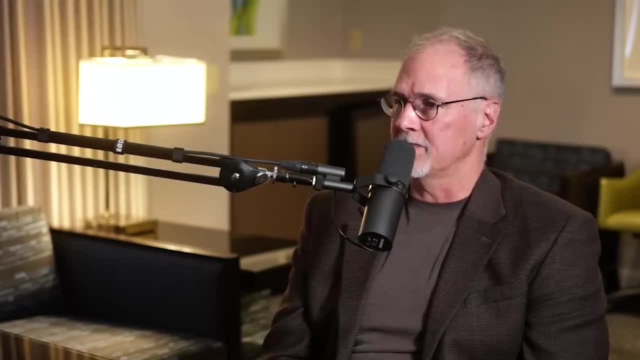 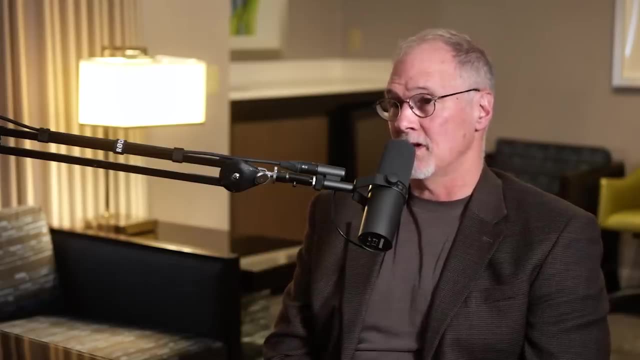 Um, but that's pretty manageable these days and and it's fairly common. And then there's another layer that you're probably calculating, you know, maybe at a hundred Hertz, maybe 10 times slower- which is now starting to look at the overall body motion and thinking. 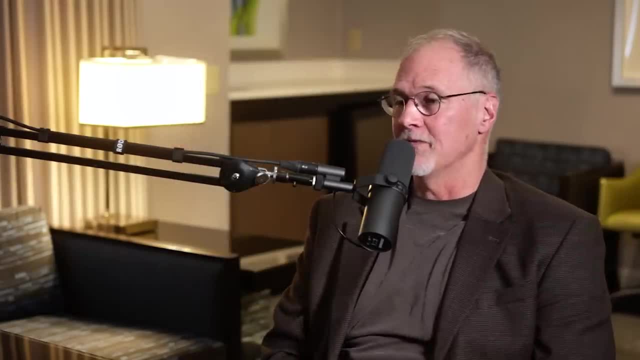 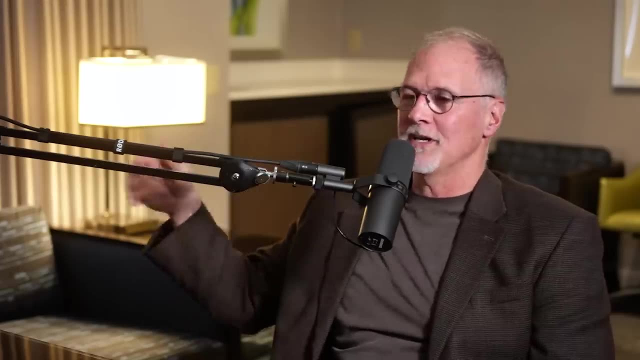 About the, The larger physics of, of the um, of the robot Um, and then there's yet another loop that's probably happening a little bit slower, which is where you start to bring you know your perception and your vision and things like that. 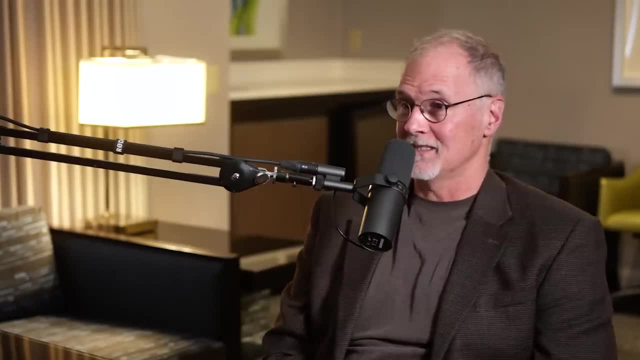 And so you need to run all of these loops sort of simultaneously. You do have to manage your, your computer time so that you can squeeze in all the calculations you need in real time in a very consistent way. Um, and the amount of 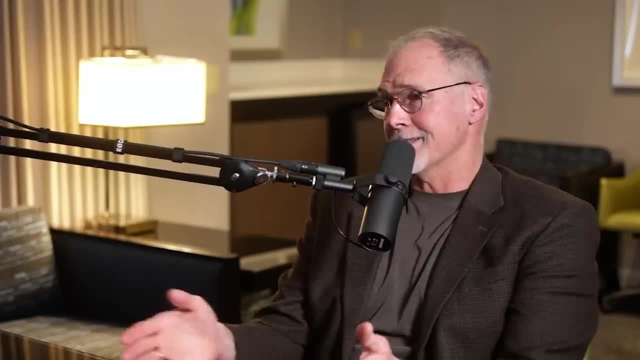 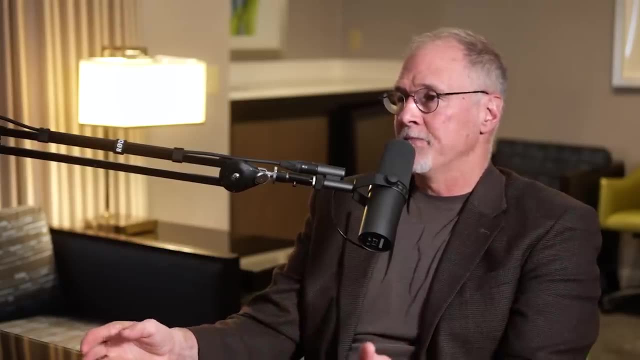 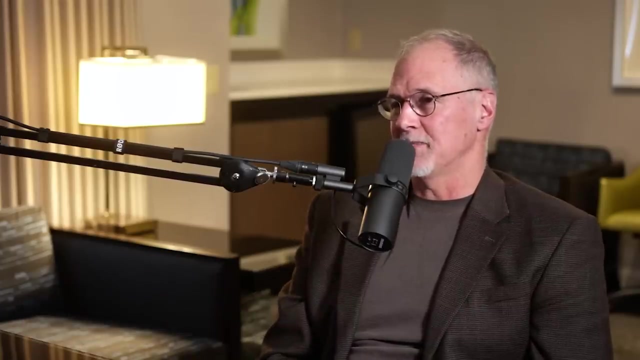 Calculation we can do is increasing as computers get better, which means we can start to do more sophisticated calculations. I can have a more complex model doing my forward prediction and and that might allow me to do even better predictions as I, as I get better and better. And and it used to be again. we ha, you know, 10 years ago we had to have pretty simple models that we were running, you know, at those fast rates, Cause the computers weren't as capable about calculating forward with a, a sophisticated model. 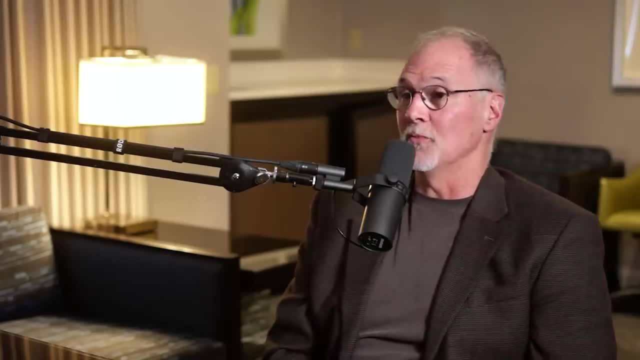 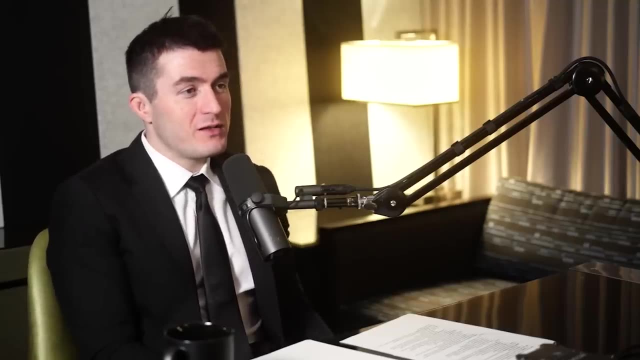 But as, as computation gets better, we can, we can do more of that. What about the actual pipeline of software engineering? How easy it is to keep updating Atlas like do continuous development on it. So how many computers are on there? 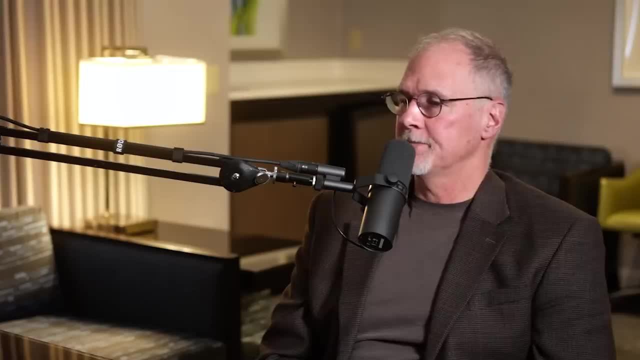 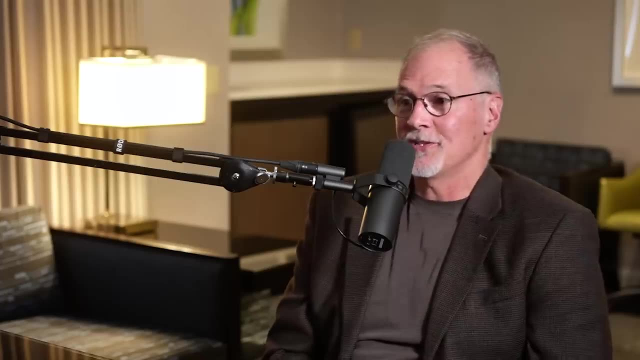 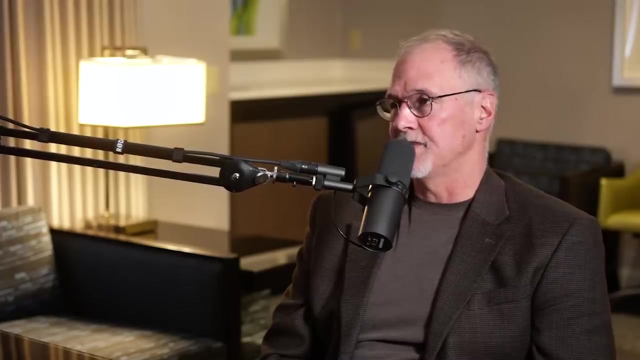 Is there a nice pipeline. It's an important part of um building a team um around it, which means you know Um you need to also have software tools, simulation tools. you know, so um we have always made strong use of uh physics-based simulation tools to do uh some of this. 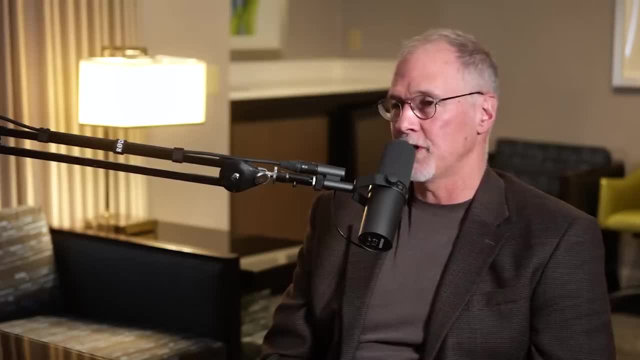 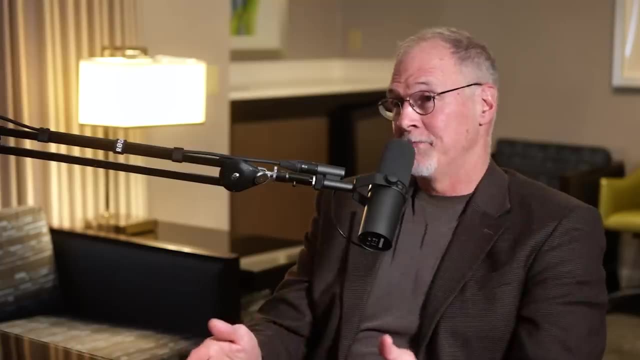 Calculation, basically test it in simulation before you put it on the robot. but you also want the same code that you're running in simulation to be the same code you're running on the hardware, And so even getting to the point where it was the same code going from one to the other. 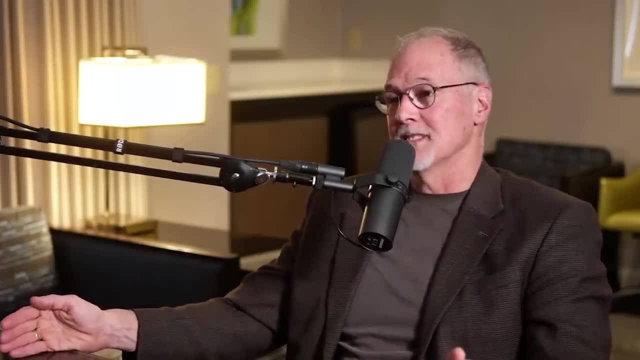 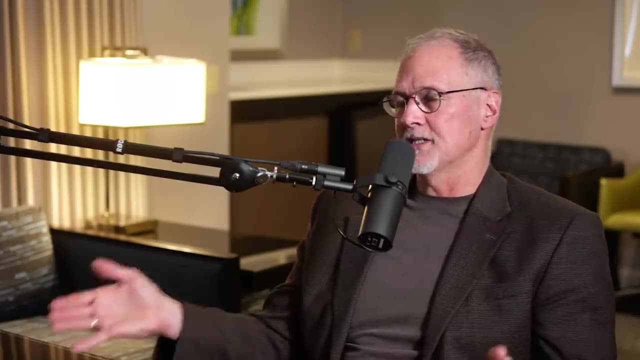 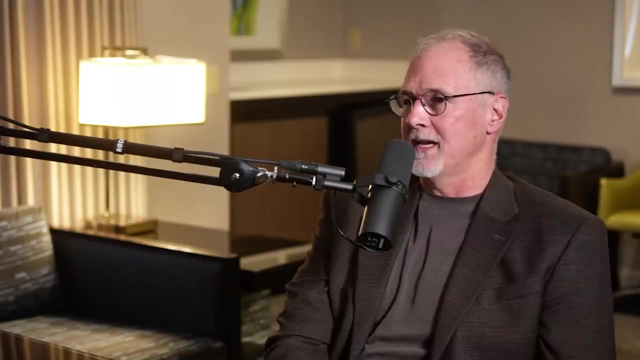 We Probably didn't really get that working until you know, a few years, several years ago, Um, but that was a, you know, that was a bit of a milestone. And so you want to work, certainly work- these pipelines so that you can make it as easy as possible and have a bunch of people working in parallel, especially when you, you know, we only have, you know, four of the Atlas robots, the modern uh Atlas robots at the company. 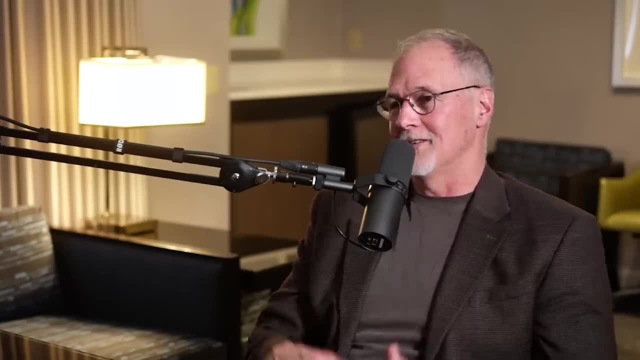 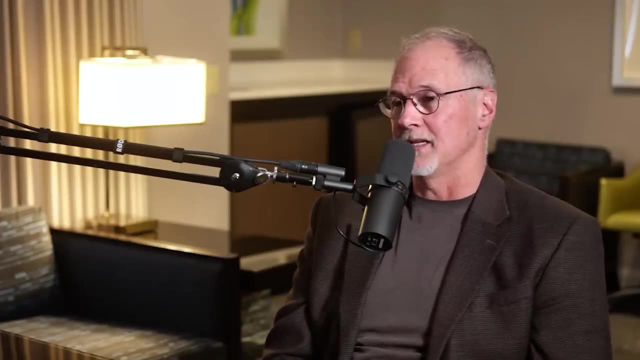 And you know we probably have, you know, 40 developers. they're all trying to gain access to it, And so you need to share resources and Use some of these, uh, some of the software pipeline. Well, that's a really exciting step to be able to run the exact same code in simulation as on the actual robot. 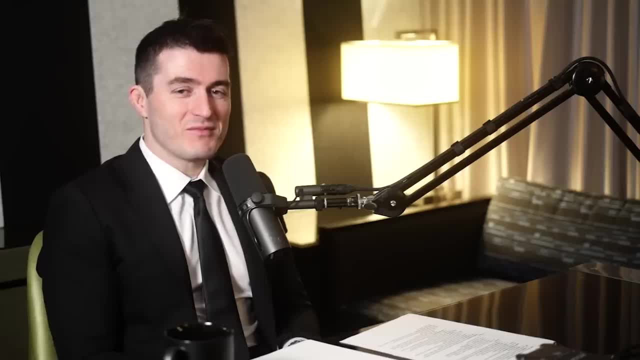 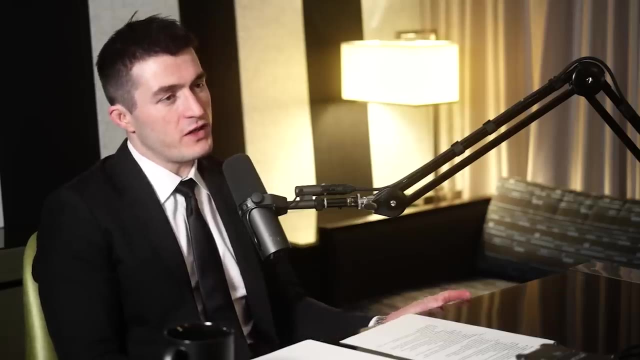 Uh, how hard is it to do? Uh, realistic simulation, physics-based simulation of, of of Atlas, such that I mean the, the dream is like if it works in simulation works perfectly in reality. how hard is it to sort of close? keep working on closing that gap. 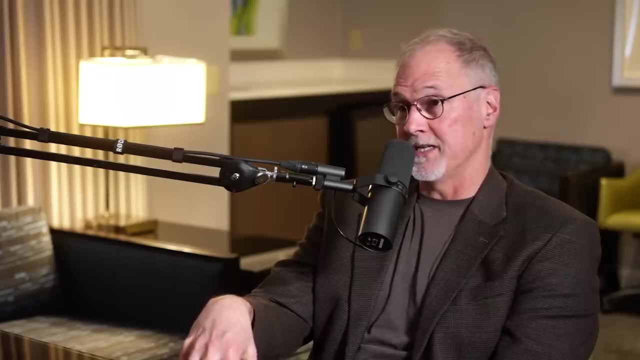 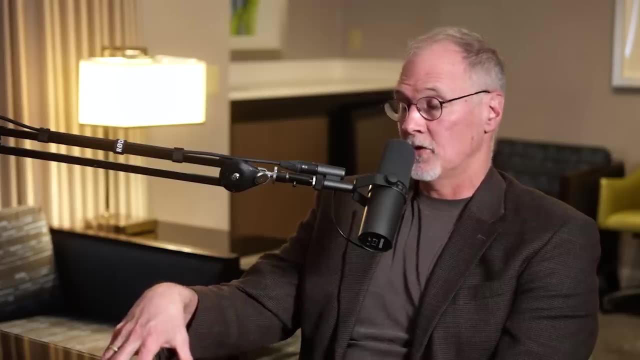 The root of some of our physics-based simulation tools really started at MIT And um. we built some some, some good physics-based modeling tools there- the early days of the company. we were trying to develop those tools as a commercial product. 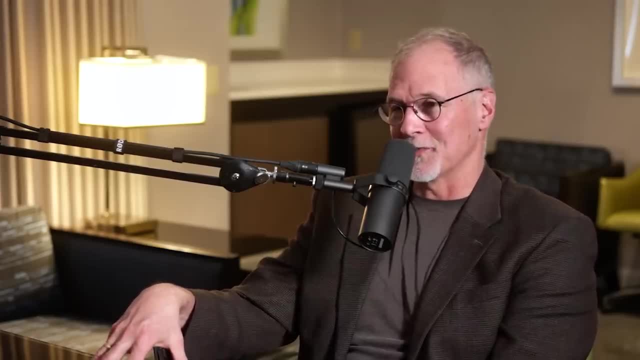 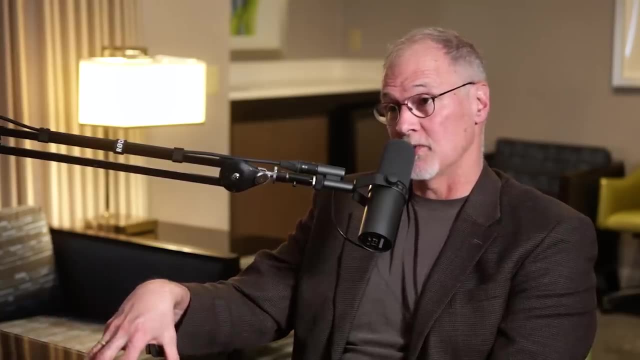 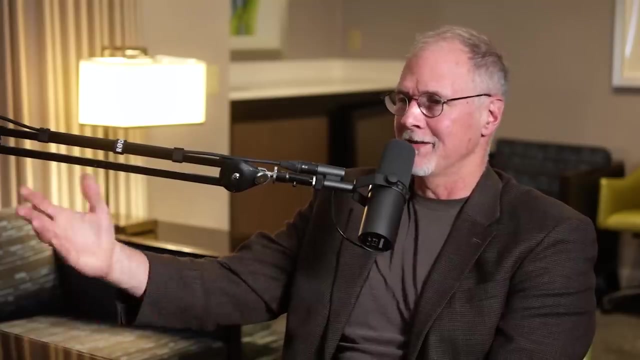 So we continued to develop them. It wasn't a particularly successful commercial product, but we ended up with some nice physics-based simulation tools So that when we started doing legged robotics again, we had a really nice tool to work with, and the things we paid attention to were were things that weren't necessarily handled very well in the commercial tools you could. 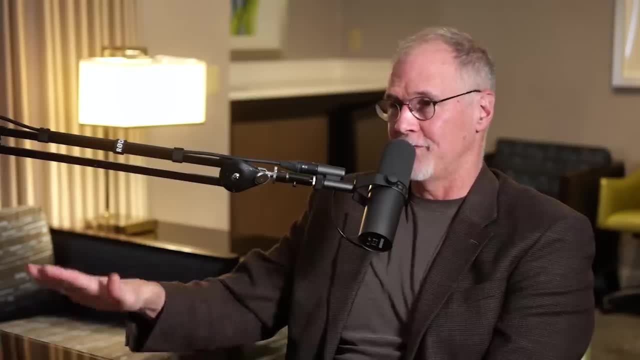 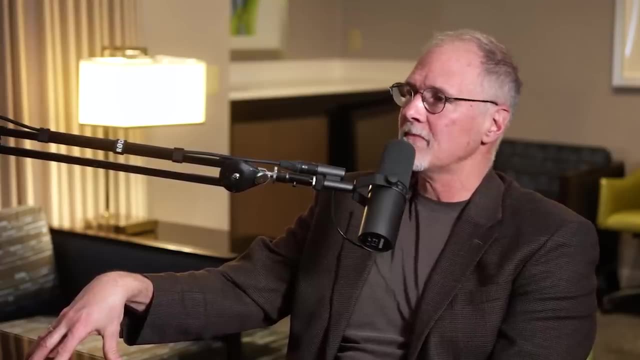 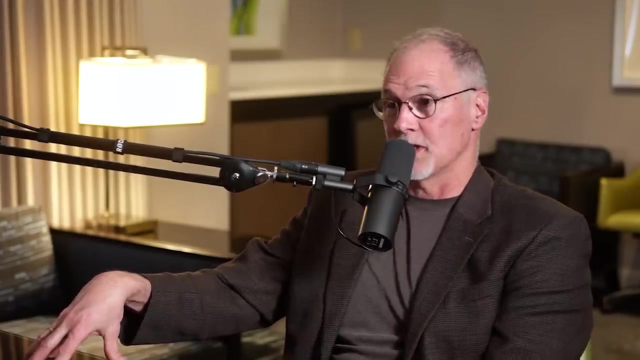 Buy off the shelf. like like interaction with the world, like foot ground contact, And so trying to model those contact um events well in a way that captured the important parts of of the interaction was a really important element. uh, to get right. 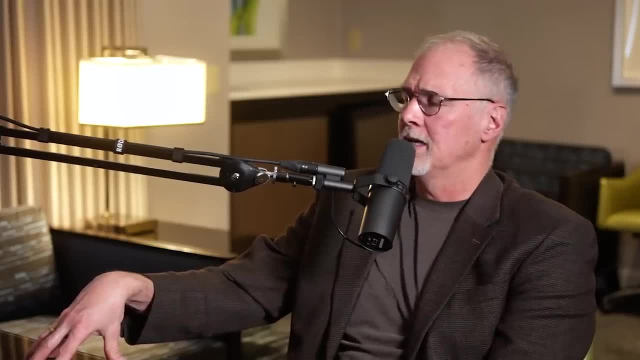 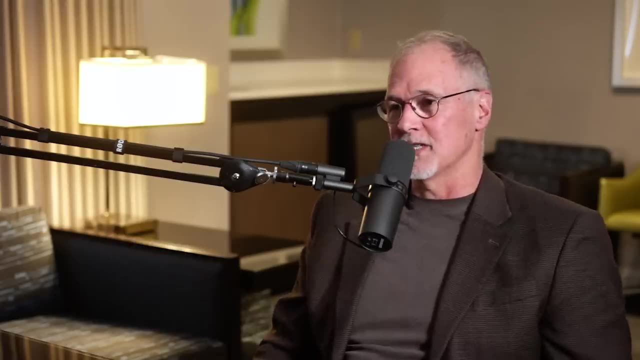 And to also do in a way that was computationally feasible, um, and could run fast, because if you, if your simulation runs too slow, you know, then your developers are sitting Around waiting for stuff to run and compile. So it it's always about efficient, uh uh fast operation as well. 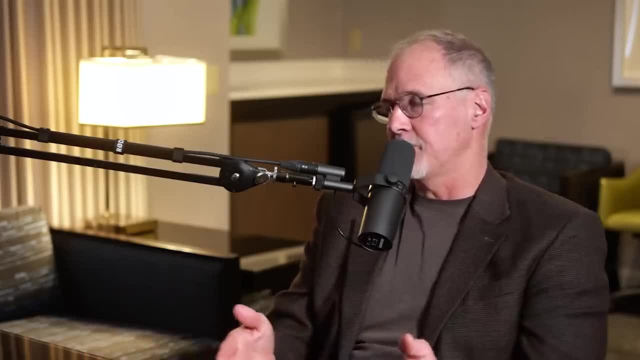 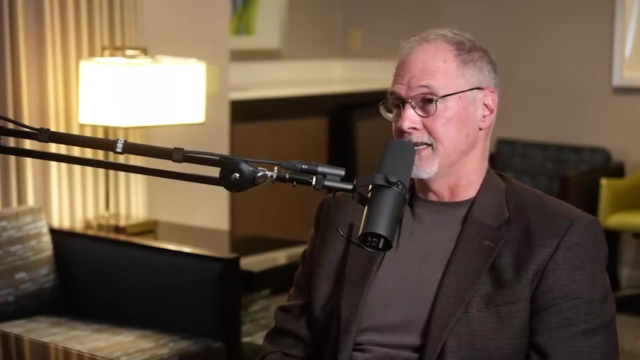 So that's been a big part of it. You know, I think developing those tools in parallel to the development of the, of the platform, and trying to scale them has has really been, uh, essential, I'd say, to us being able to assemble a team of people that could do this. 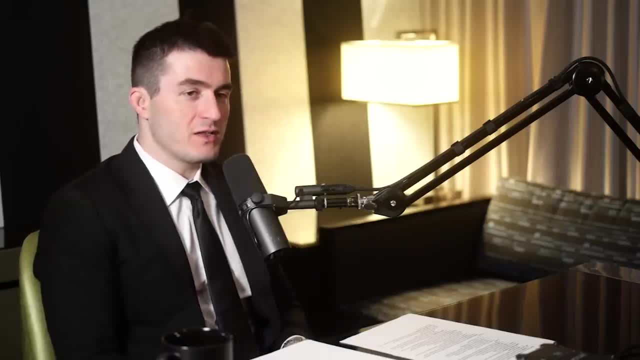 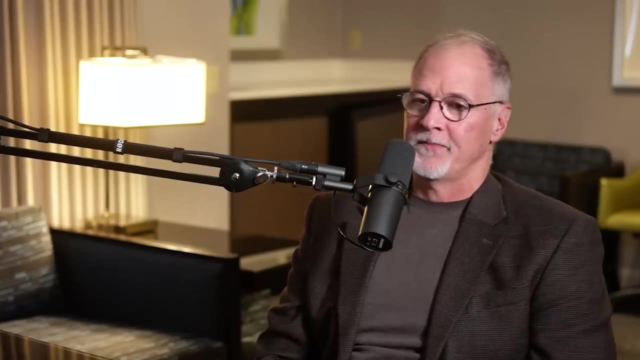 Yeah, How to simulate contact periods of foot, ground contact, but sort of for manipulation, Um, Because don't you want to model all kinds of surfaces? Yeah, So it will be even more complex with manipulation, because there's a lot more going on. you know, and you need to capture, I don't know- things slipping and moving. you know in your, in your, in your hand. 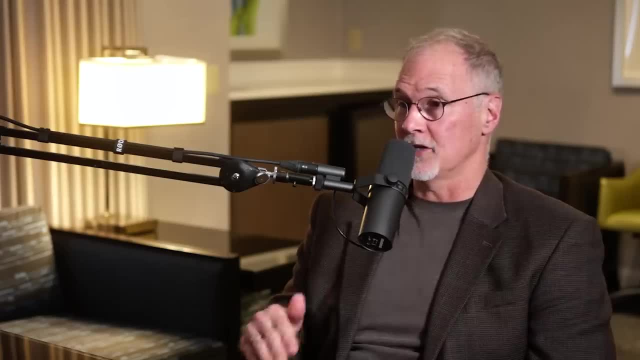 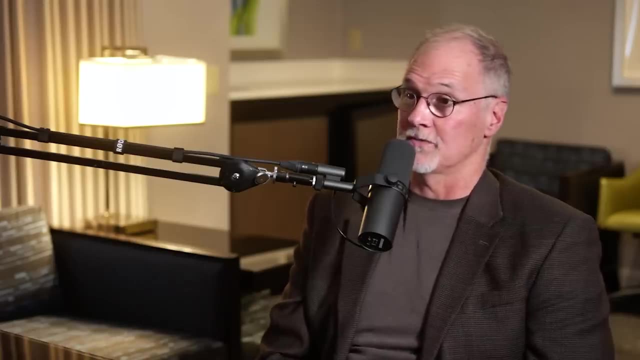 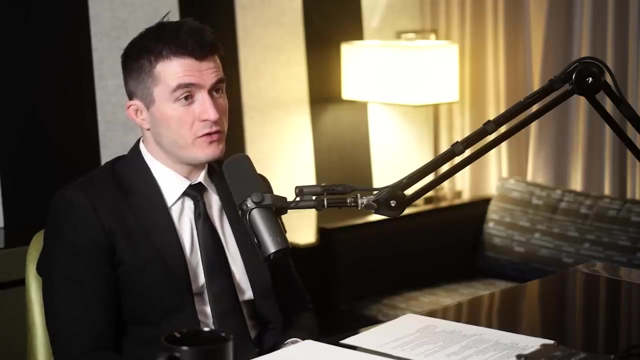 Um, it's a level of complexity that I think goes above foot ground. uh, contact when you really start doing dexterous manipulation. So there's challenges I had still. So how far, How far are we away from me being able to walk with Atlas in the sand along the beach and us both drinking a beer out of a can, out of a can? 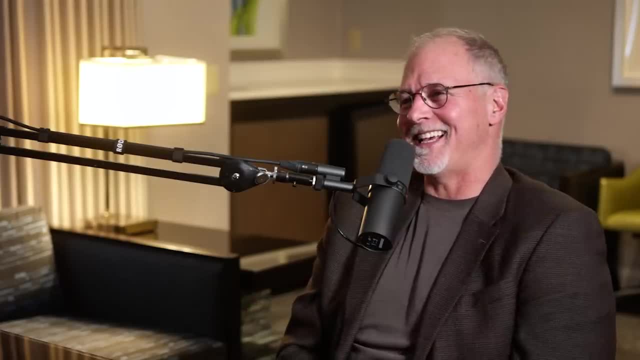 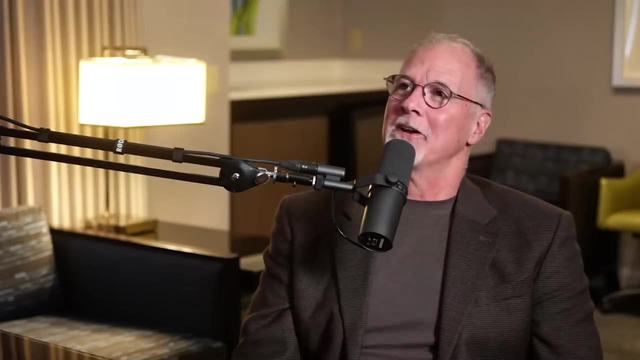 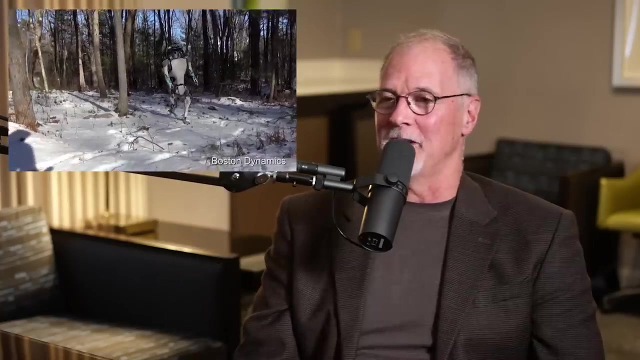 Maybe Atlas could spill his beer cause he's got nowhere to put it. Atlas could walk on the sand, So can it? Yeah, Yeah, Yeah, I mean you know, have we really had him out on the beach? You know we take them outside often. you know rocks, hills, that sort of thing, even just around our lab in Waltham. 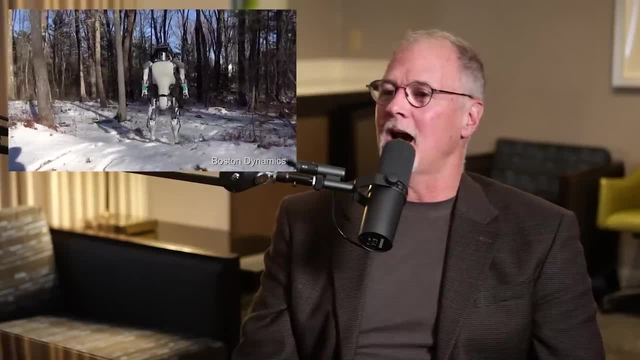 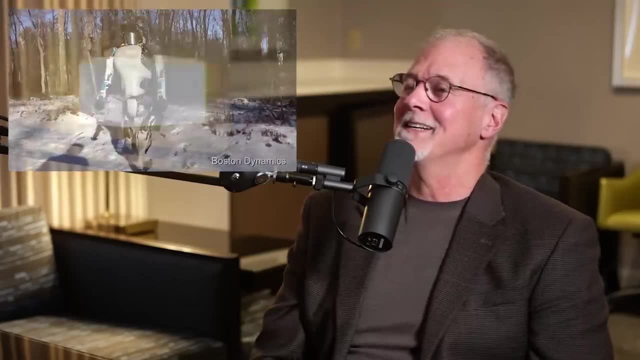 We probably haven't been on the sand, but I'm I. I don't doubt that we could deal with it. Uh, we, we, we might have to spend a little bit of time to sort of make that work, but we did take. uh, we, we had a had to take big dog to Thailand years ago. 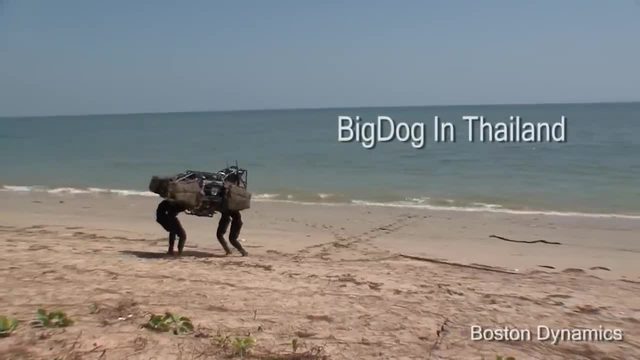 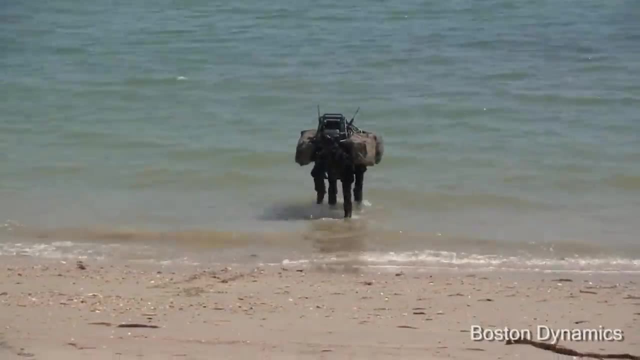 And, uh, we did this great video of the robot walking in the sand, walking into the ocean up to I don't know it's belly or something like that, And then turning around and walking out, All while playing some cool beach music. 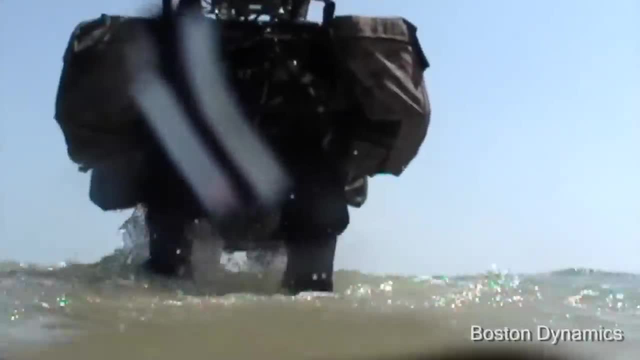 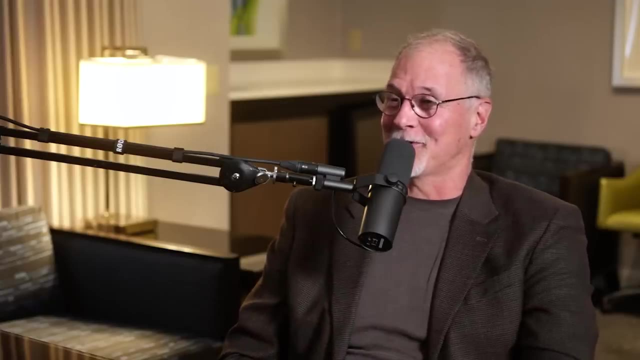 Great show. But then you know, we didn't really clean the robot off and the salt water was really hard on it. So, uh, you know, we we put it in a box, shipped it back. By the time it came back we had some problems with corrosion. 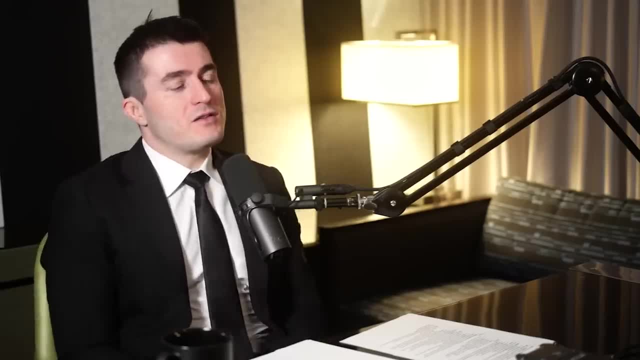 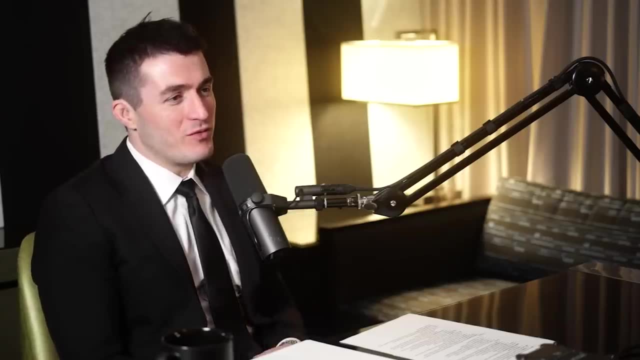 So it's the salt, it's the salt water. It's not like Salt stuff, It's not like sand getting into the components or something like this. But I'm sure if, if this is a big priority, you can make it like waterproof. 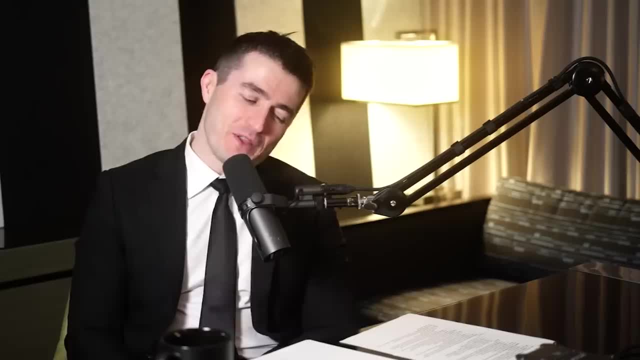 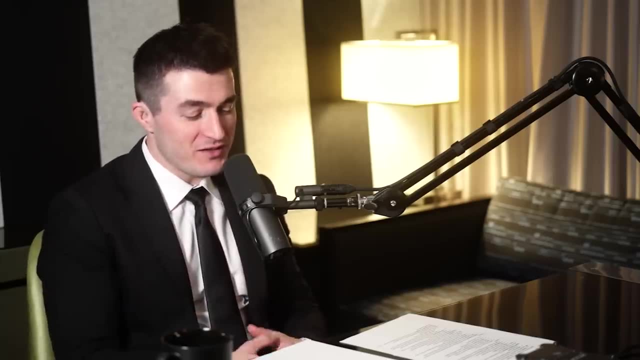 Right, That just wasn't our our goal at the time. Well, it's a personal goal of mine: Do it Walk along the beach, But it's a human problem too. You get sand everywhere It's. it's just a jam mess. 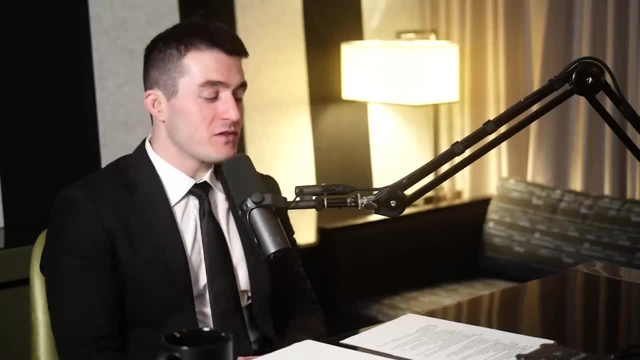 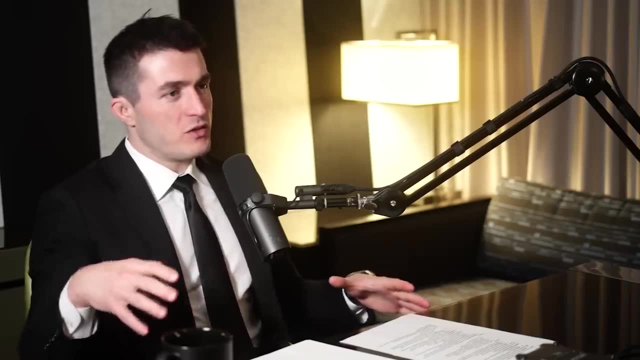 So soft surfaces are okay. So I mean, can we just linger on the robotics challenge There was um? there's a pile of- uh like rubble they had to walk over. Is that? um? how difficult is that task? 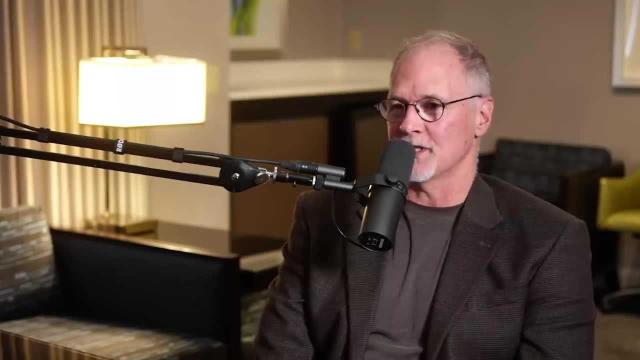 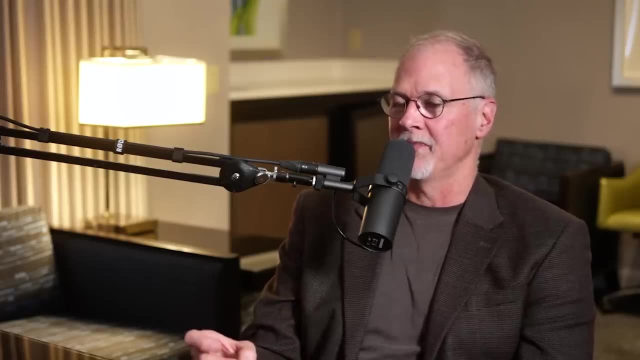 In the early days of developing Big Dog, the loose rock was the epitome of the hard walking surface, Because you step down and then the rock, And you had these little point feet on the robot and the rock can roll and and you have. 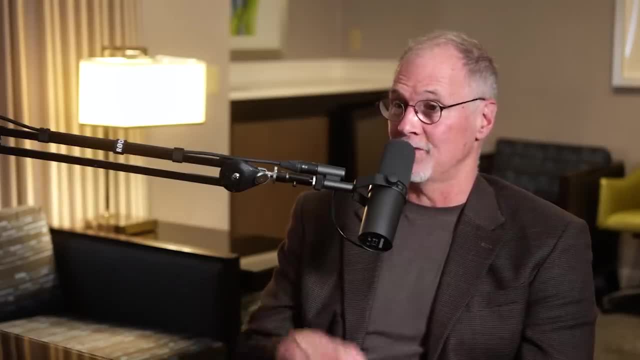 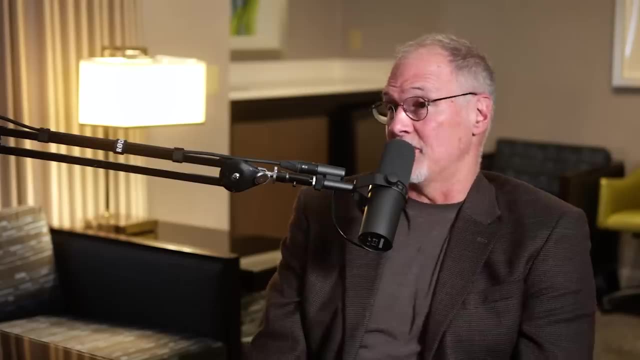 to deal with that last minute. you know, change in your foot placement, Yeah, So you, you step on the thing and that thing responds to you stepping on it, Yeah, And and it moves where your point of support is, And so it's really that that became kind of the essence of the test. 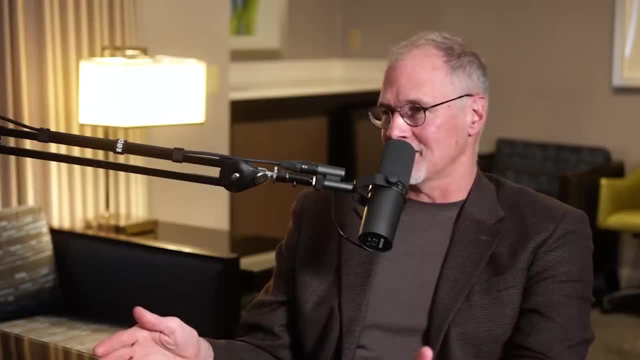 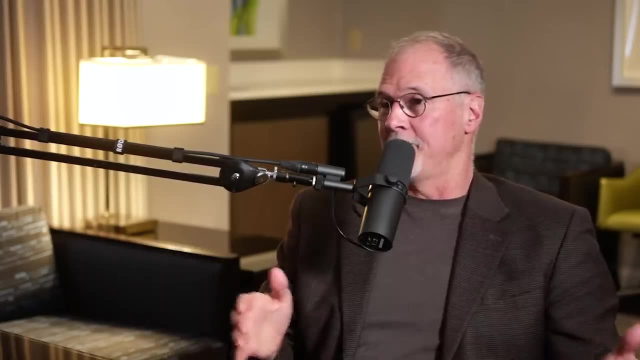 And so that was the beginning of us starting to build rock piles in our parking lots and and we would actually build boxes full of rocks and bring them into the lab, And then we would have the robots walking across these boxes of rocks, because that became the essential test. 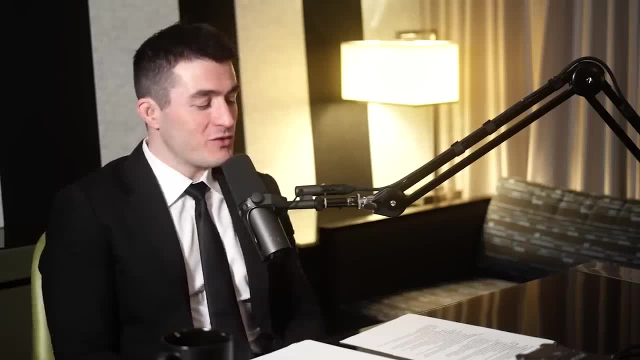 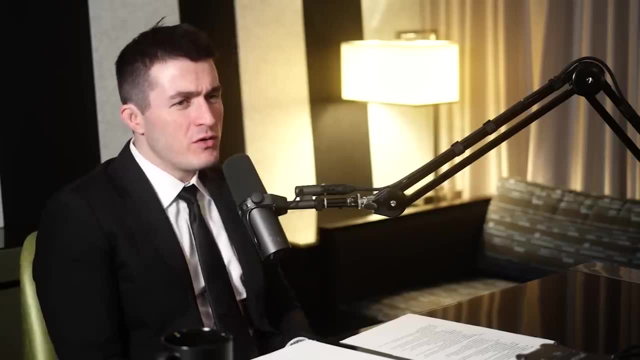 So you mentioned Big Dog. Can you, can we maybe take a stroll through the history of Boston Dynamics? So what and who is Big Dog, By the way, is who do you try not to anthropomorphize? the robots? Do you try not to? do you try to remember that they're? this is. 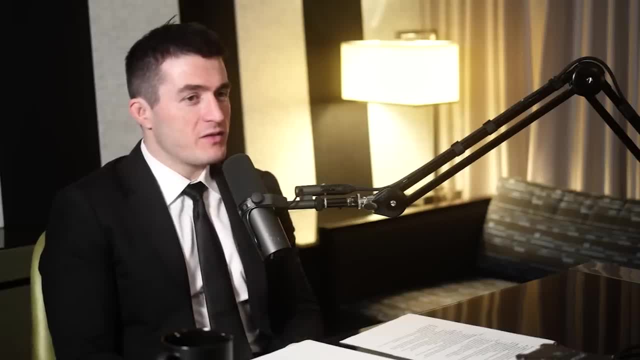 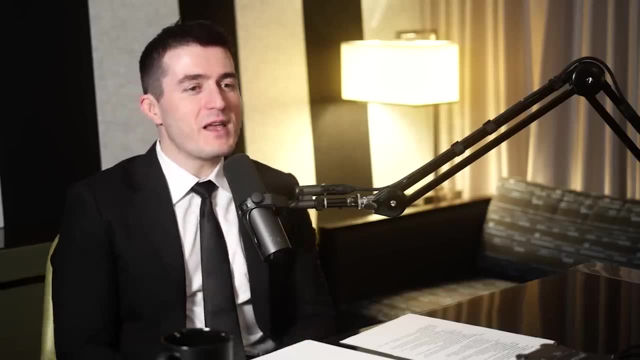 this is like the division I have, because I for me, it's impossible for me. There's a magic to the, to the being that is a robot. It is not human, but it is it. the the same magic that a living being has when it moves about the world is there in the robot. 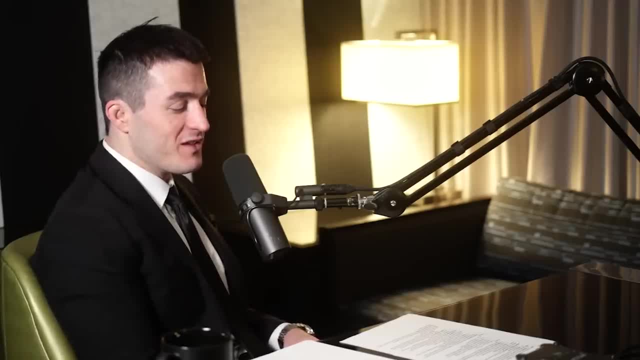 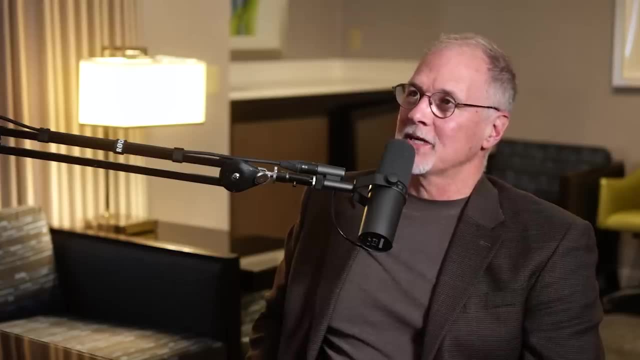 So I don't know what question I'm asking, but should I say what or who? I guess who is Big Dog? What is Big Dog? Well, I'll say, to address the meta question, We don't try to draw hard lines. 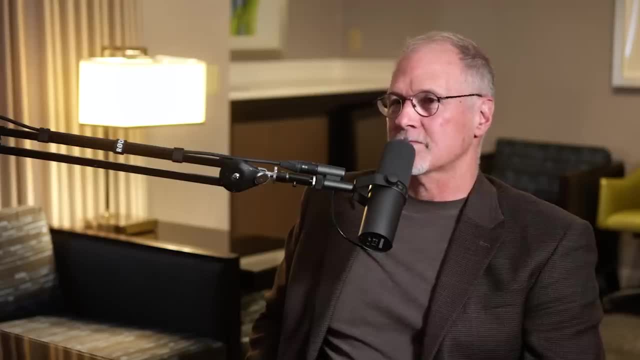 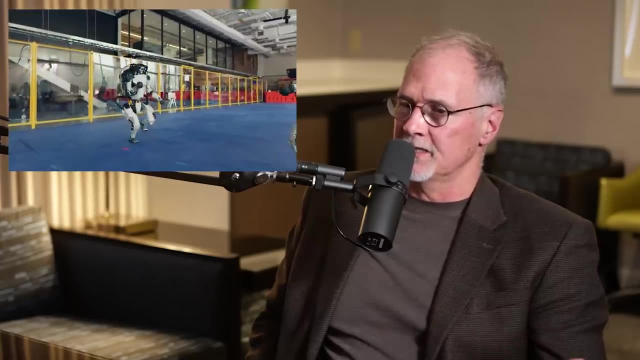 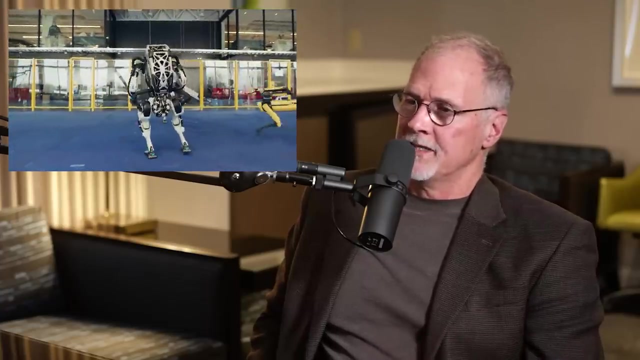 We don't try to draw hard lines around it being an it or a him or a her. um, it's okay, right, People? I think part of the magic of these kinds of machines is, by nature, of their organic movement, of the of their dynamics. we tend to want to identify with them. 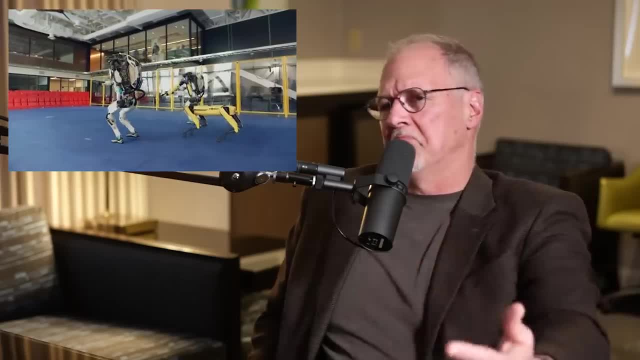 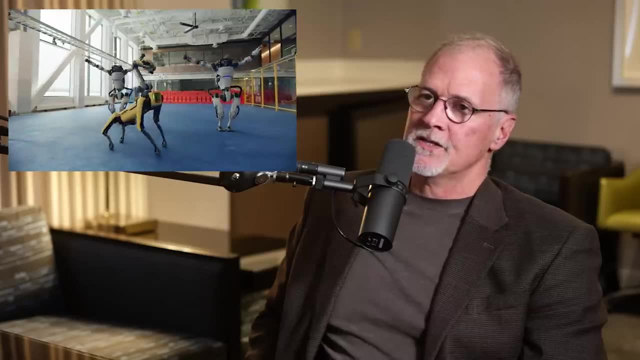 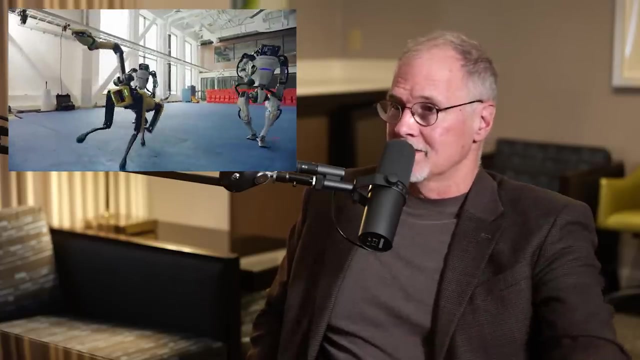 We, we tend to look at them and sort of attribute maybe feeling to that, because we've only seen things that move like this, that were alive, And so, um, this is an opportunity. It means that you could have feelings for a machine, and you know people have feelings for their cars. 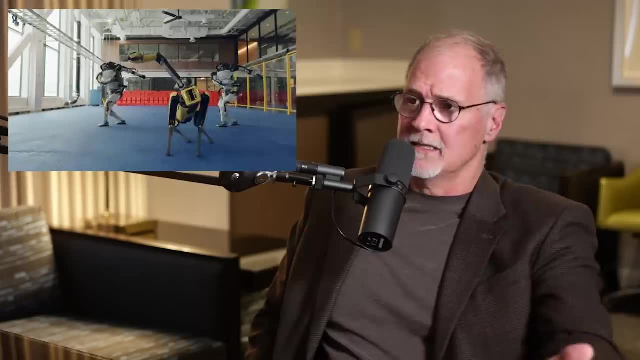 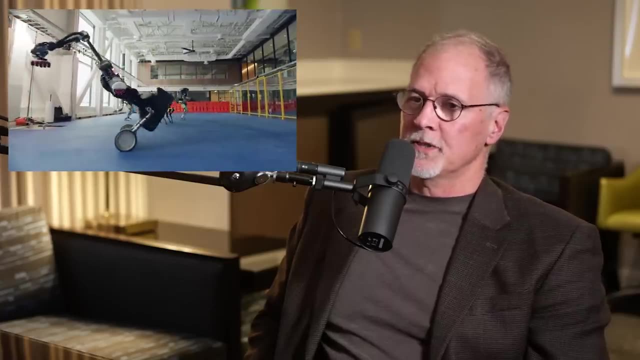 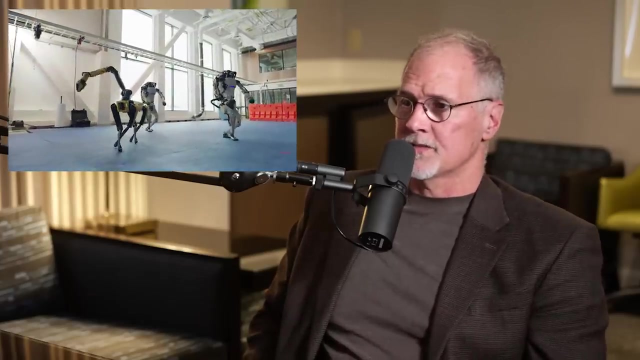 You know they get attracted to them, attached to them. So that's inherently could be a good thing, as long as we manage what that interaction is, So we don't put strong boundaries around this and ultimately think it's a benefit. but it's also can be a bit of a curse, because I think 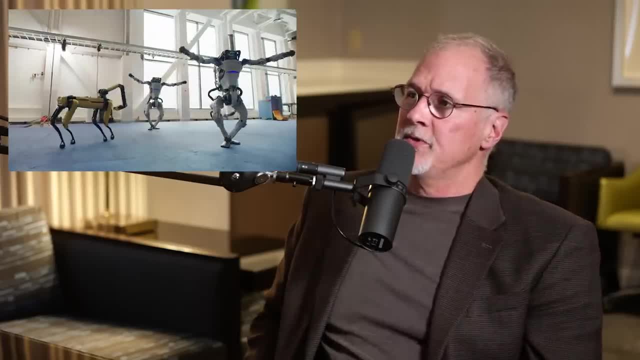 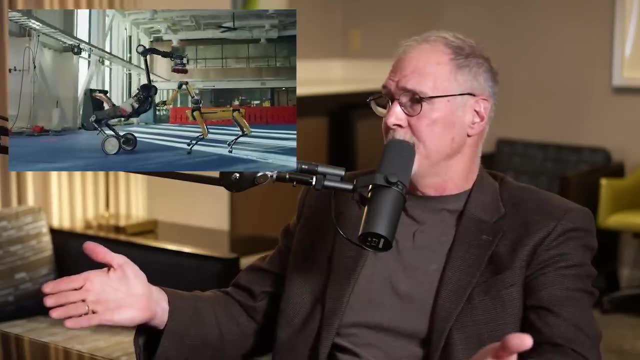 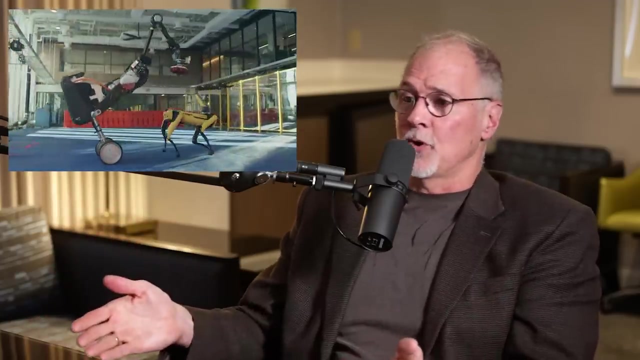 People look at these machines and they attribute a level of intelligence that the machines don't have. Why? Because, again, they've seen things move like this, that we're living beings which are intelligent, And so they want to attribute intelligence to the robots. that isn't appropriate yet, even though they move like an intelligent being. 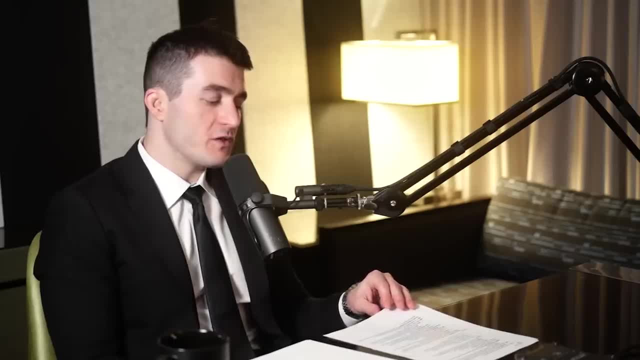 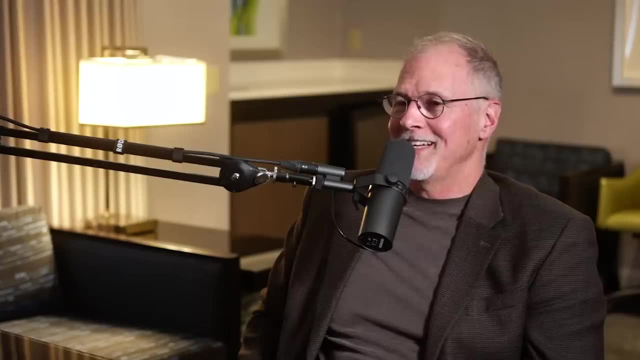 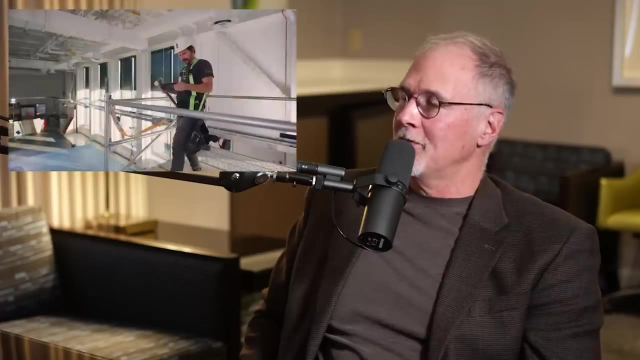 But you try to acknowledge that the anthropomorphization is there, and try to first of all acknowledge that it's there. Yeah, Yeah, Yeah, And have a little fun with it. You know our our most most recent video. it's just kind of fun, you know to to to look at the robot. 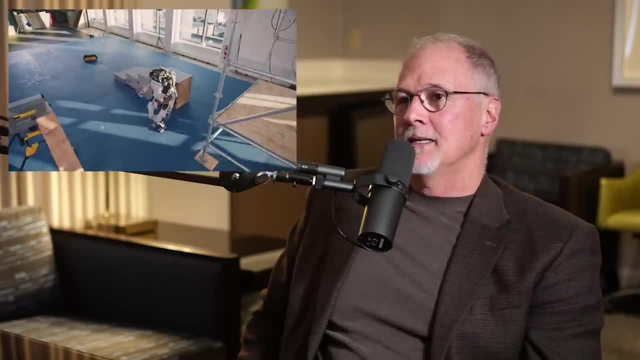 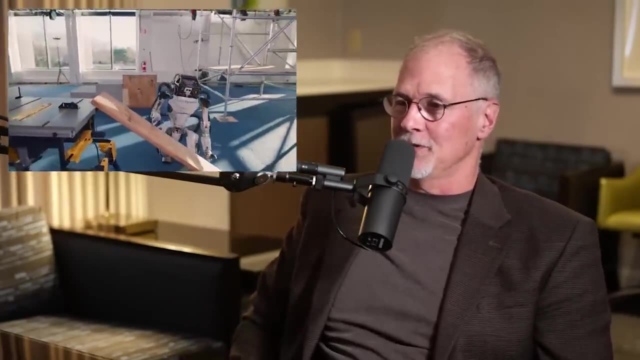 We started off the the video with Atlas um kind of looking around for where the bag of tools was, Cause the guy up on the scaffolding says: send me some tools. Atlas has to kind of look around and see where they are. 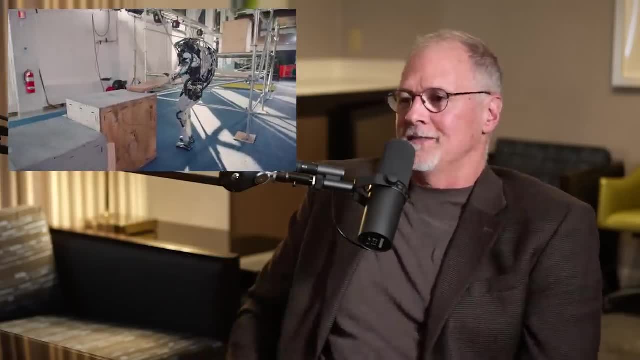 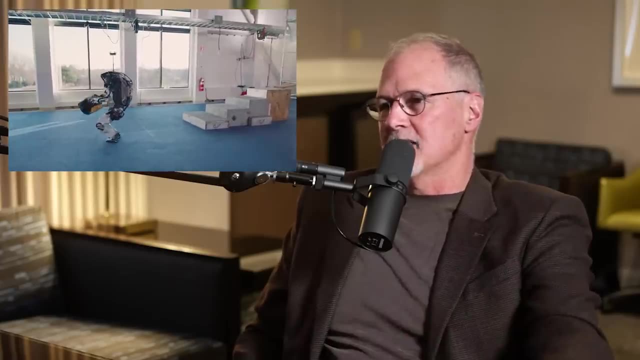 And there's a little personality there. that is fun, It's entertaining, It makes our jobs interesting And I think in the long run Can enhance interaction between humans and robots that in a way that isn't available to machines that don't move that way. 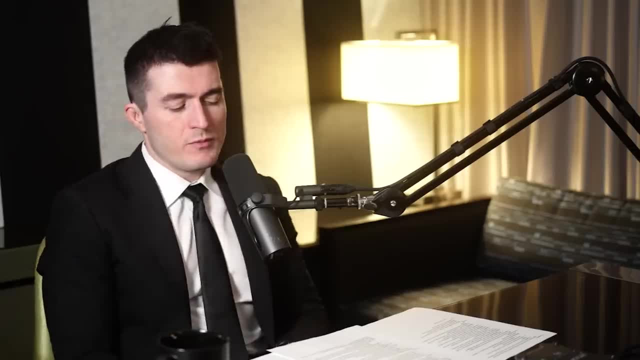 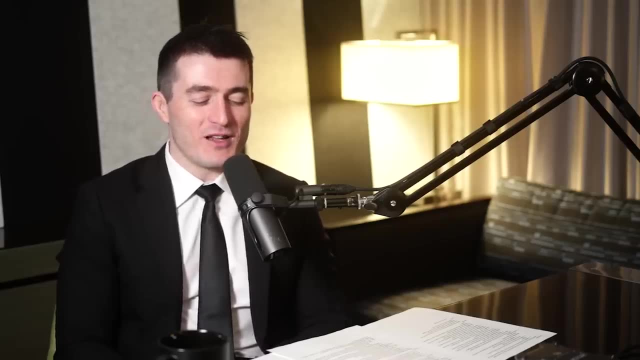 This is something to me personally is very interesting. I've been um. I happen to have a lot of legged robots. I hope to have a lot of spots in my possession Um. I'm interested in celebrating robotics and celebrating companies. 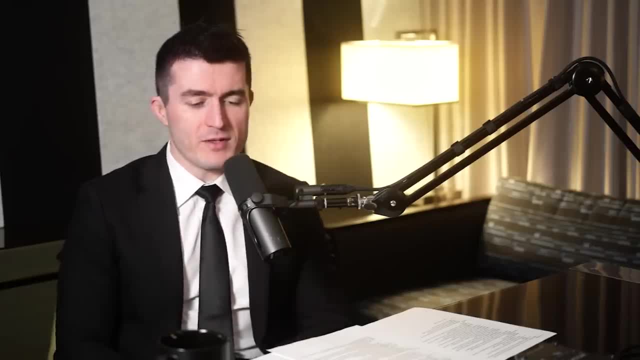 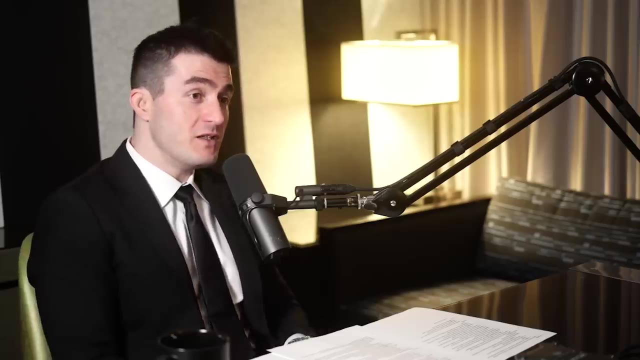 And I also don't want to companies that do incredible stuff like Boston dynamics And I. there's a Um- you know I'm a little crazy- and you say you don't want to. you, you want to align, you want to help the company, because I ultimately want, uh, a company that Boston dynamics to succeed. 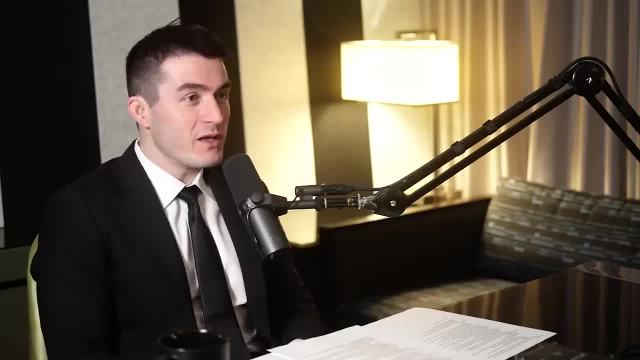 And part of that we'll talk about. you know, success kind of requires making money, And so the kind of stuff I'm particularly interested in may not be the thing that makes money in the short term. I can make an argument that it will in the longterm, but the kind of stuff I've been playing with is 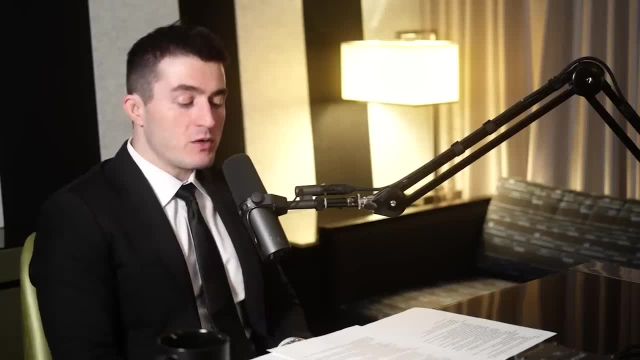 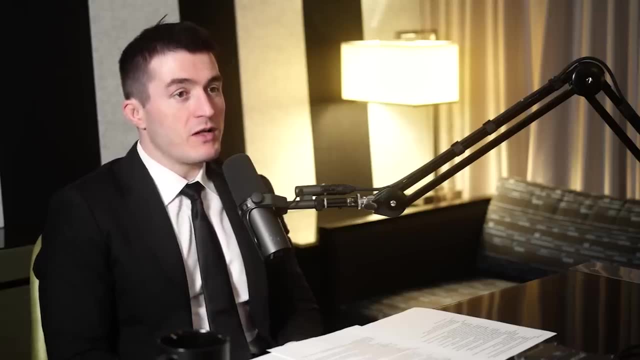 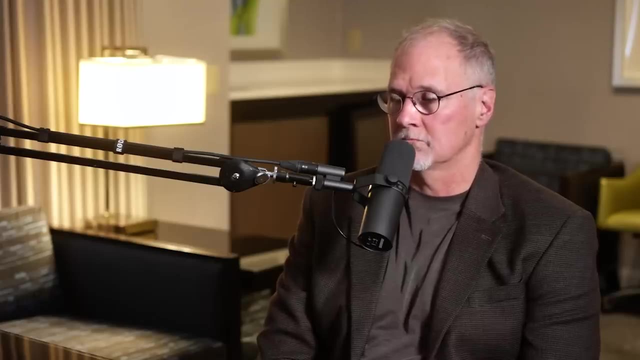 A robust way of uh having the quadrupeds, the robot dogs, communicate emotion with their body movement, the same kind of stuff you do with a, with a dog, but not not hard-coded, uh, but in a robust way- and be able to communicate excitement or fear, uh, boredom, all this kinds of stuff. 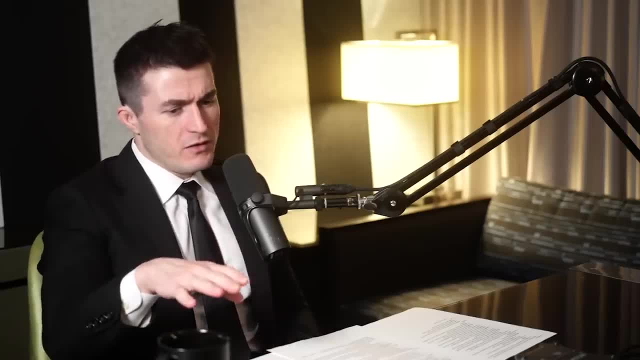 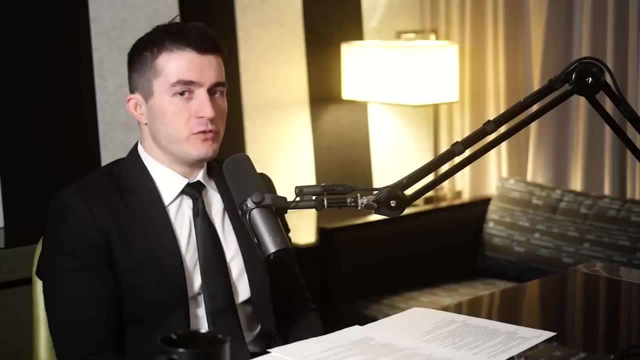 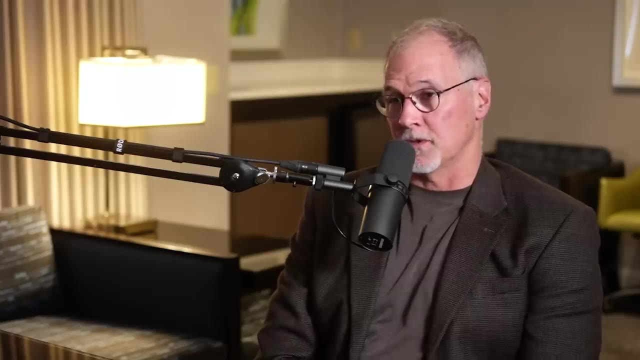 Uh, and I think, as a base layer of function, of behavior, to add on top of a robot, I think that's a really powerful way, uh, to To make the robot more usable for humans, for whatever. I think it's going to be really important and, um, it's a thing we're we're beginning to pay attention to. 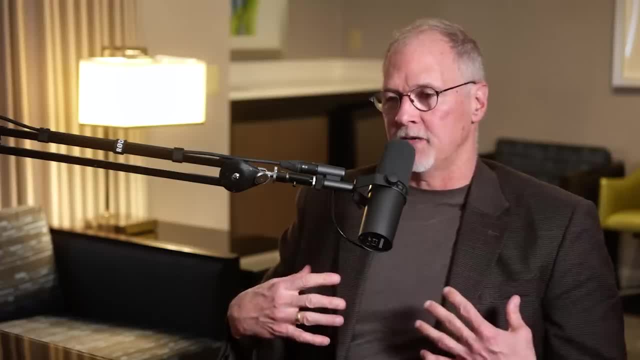 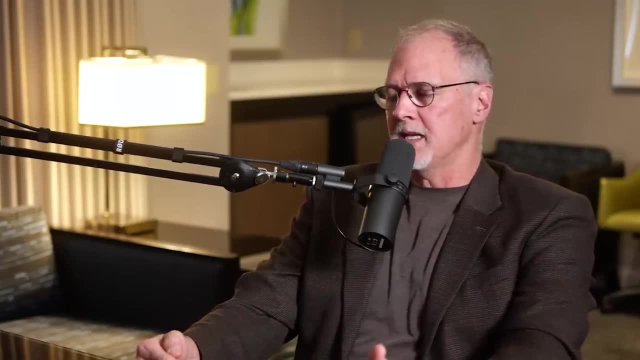 Um, we really want to start a differentiator, for the company has always been. we really want the robot to work, We want it to be useful. uh, making it work at first meant the the legged locomotion really works, It can really get around and it doesn't fall down. 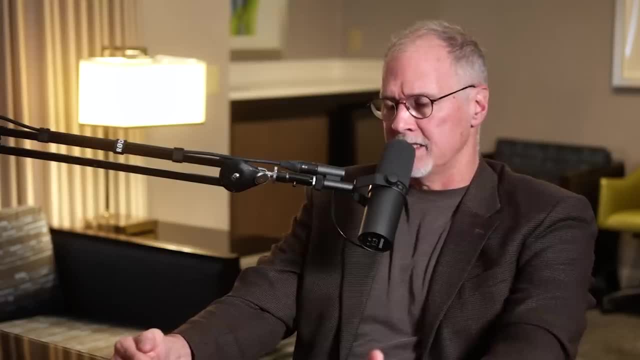 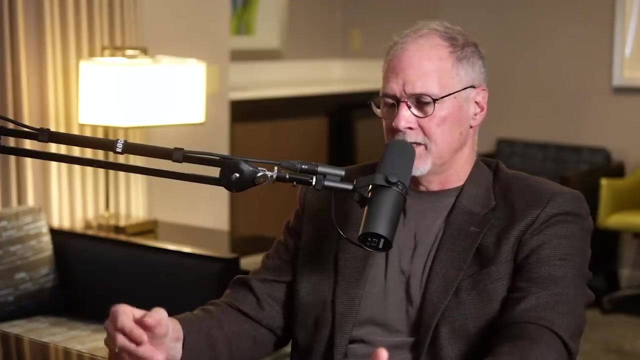 And um, but beyond that, now It needs to be a useful tool And our customers are, for example, factory owners, people who are running a process manufacturing facility, and the robot needs to be able to get through this complex facility in a reliable way, you know, taking, taking measurements. 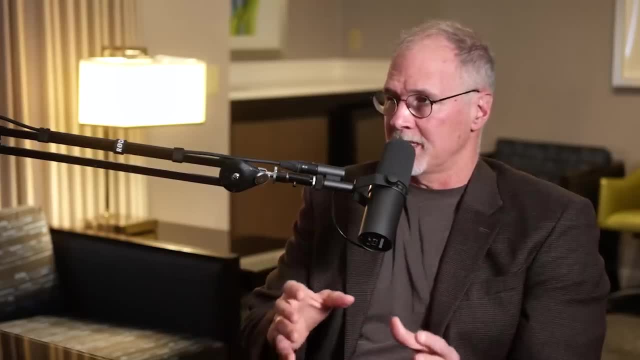 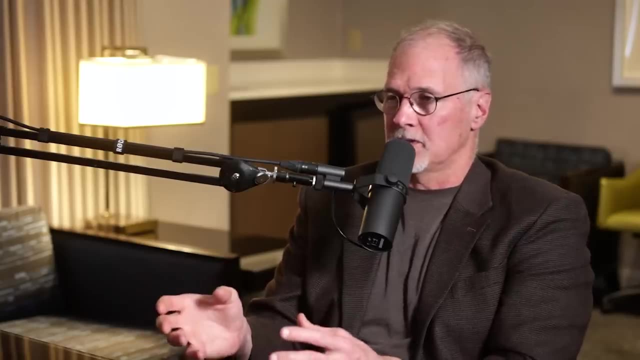 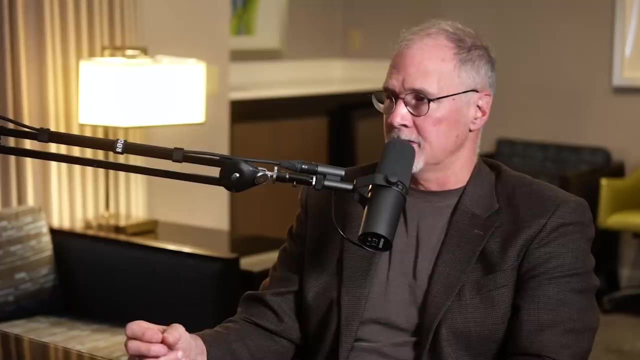 We need for people who are operating those robots to understand what the robots are doing. If the robot gets into, needs help or or you know is in trouble or something, it needs to be able to communicate And a physical indication of some sort, uh to so that a person looked at the robot and goes, oh, I know what that's that robot's doing. 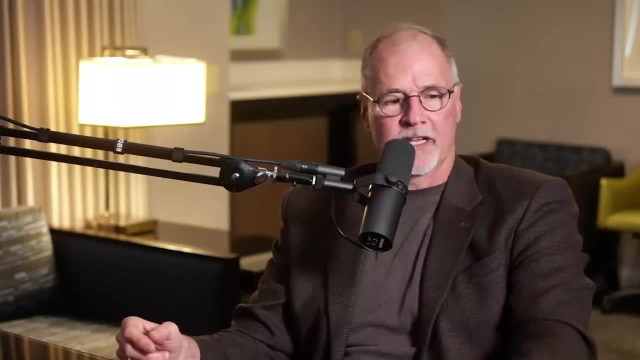 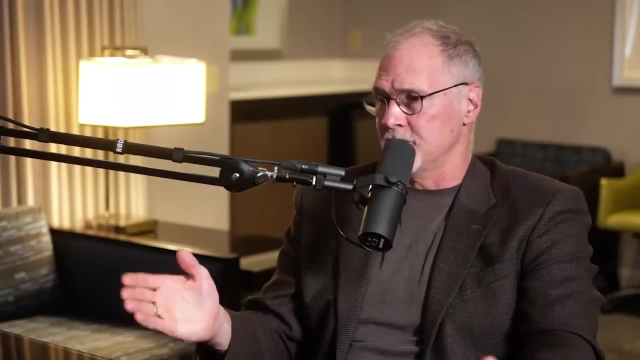 The robot's going to go take measurements of my uh vacuum pump with its thermal camera. You know you want to be able to indicate that And we're even just the robots um about to turn. you know in front of you and maybe indicate that it's going to turn. 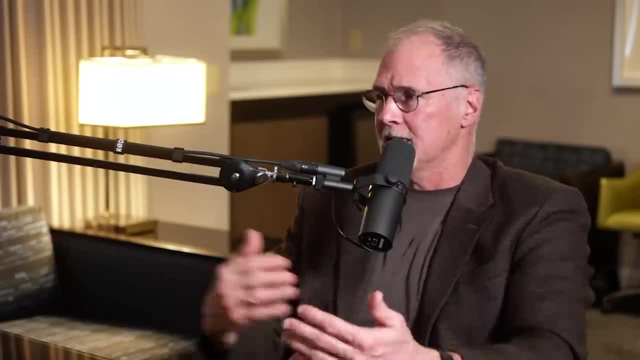 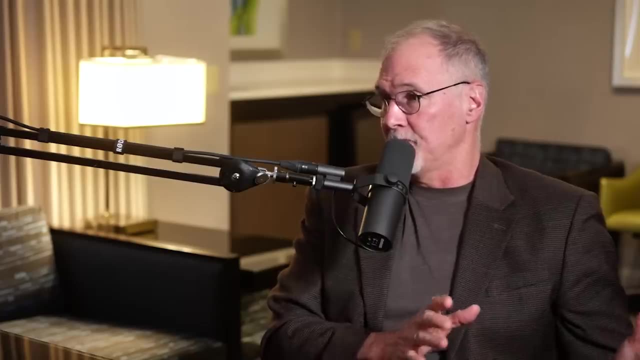 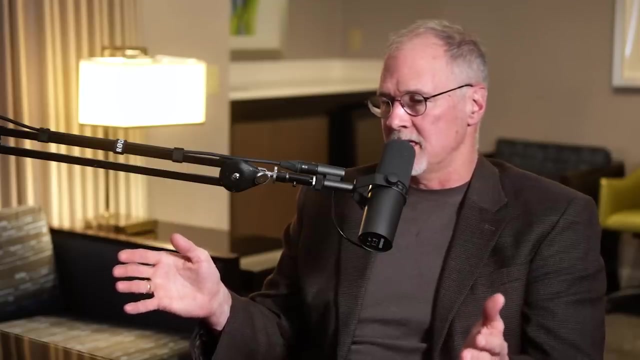 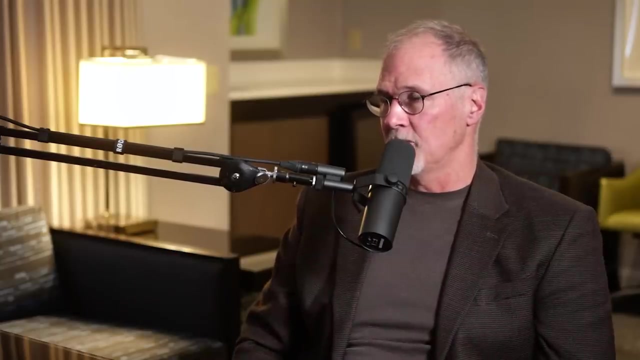 And so you sort of see and can anticipate its motion. So these, this kind of communication is going to be Becoming more and more important. It wasn't sort of our starting point, Um, you know, but now the, the robots are really out in the world and you know we have about a thousand of them out with with customers right now, this layer of physical indication, I think, is going to become more and more important. 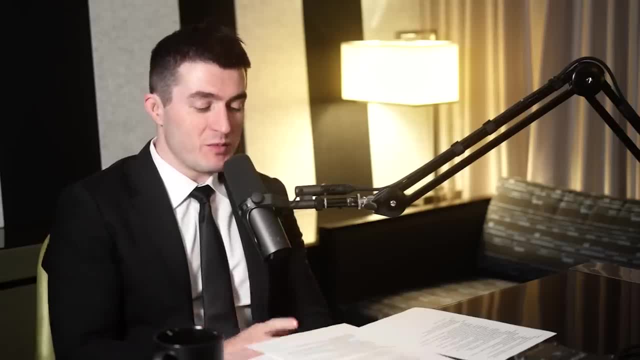 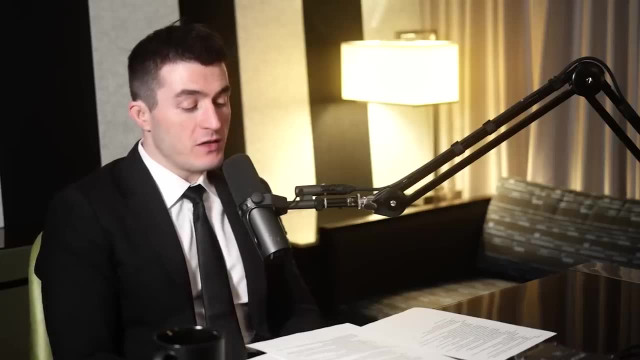 We'll talk about where it goes, cuz there's a lot of interesting possibilities. but if you can return back to the origins of Boston dynamics with so the the more research, the R And D side, before we talk about how to build robots at scale, 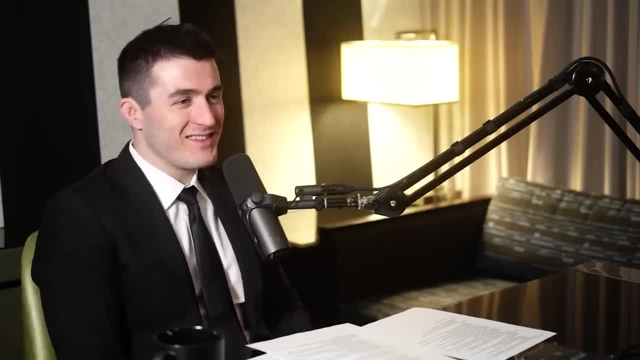 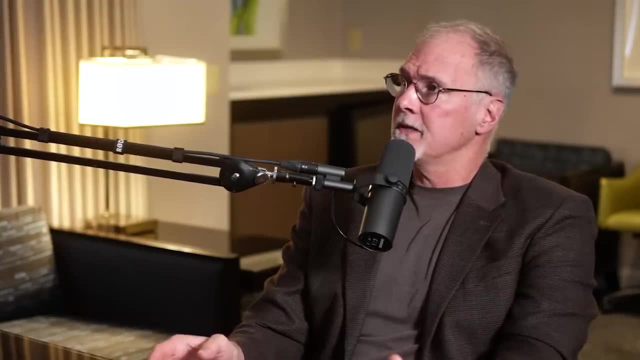 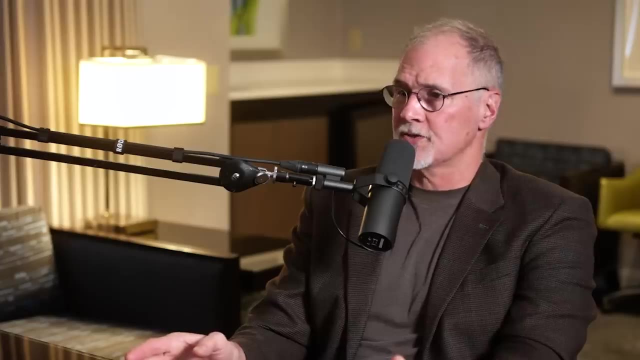 So big dog. so, um, who's big dog? So the company started in 1992 and in um, probably uh, uh, 2003,, I believe, is when we uh took a contract from dark. So basically 10 years, 11 years, um, we weren't doing robotics. 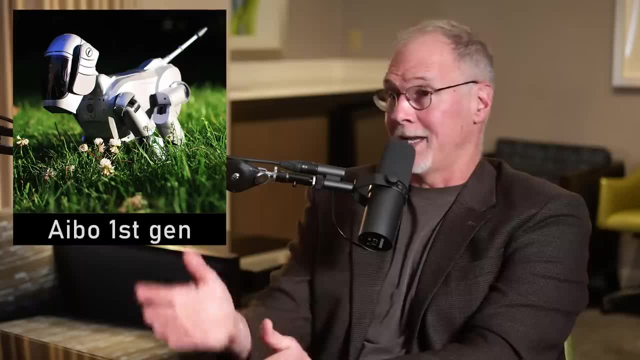 We did A little bit of robotics with Sony. Uh, they had uh IBO. they had the their IBO robot. We were developing some software for that. that kind of got us a little bit involved with robotics again. 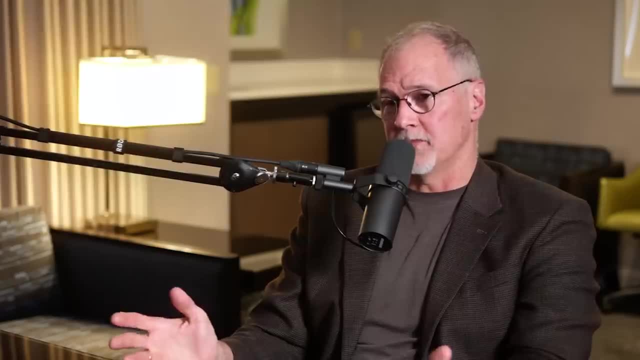 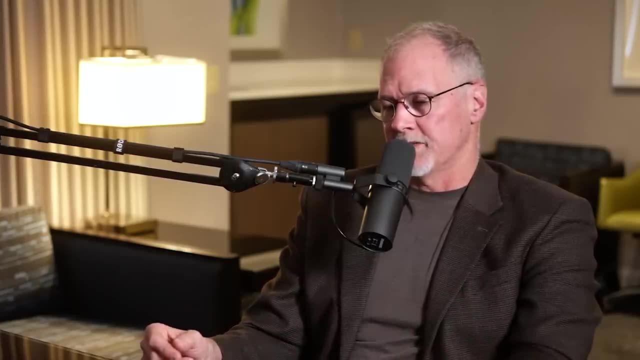 Then there's this opportunity to do a DARPA contract where they wanted to build a robot dog And uh, we, we won a contract to to build that, And so that was the genesis of big dog, and uh, it was a quadruped. 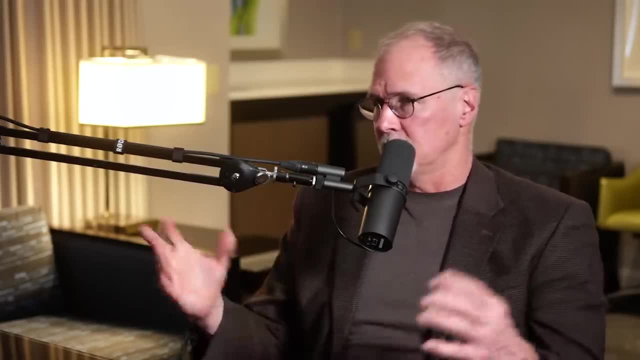 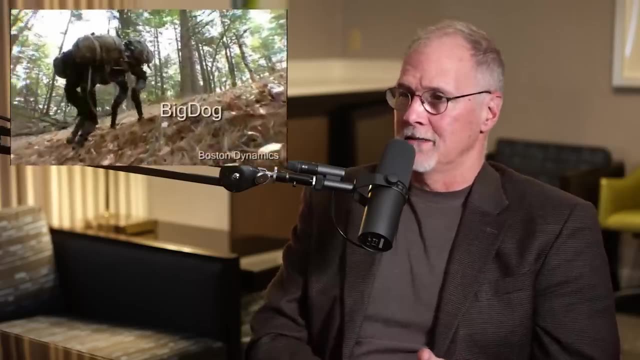 And it was the first time we built a robot that had everything on board that you could Actually take the robot out into the wild and operate it. So it had onboard power plant, It had onboard computers, It had, uh, hydraulic actuators that needed to be cooled. 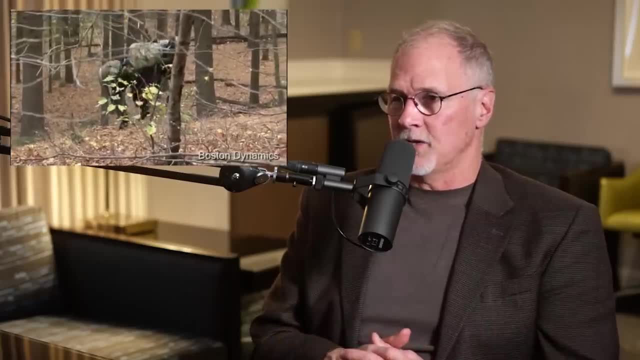 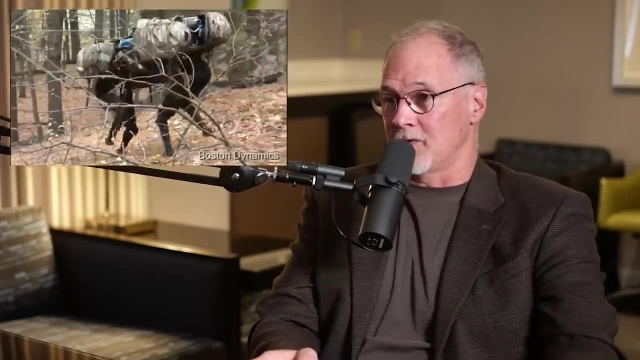 So we had cooling systems built in, everything integrated into the robot, And, uh, that was a pretty rough start, right? So it was. it was 10 years that we were not a robotics company, We were a simulation company, and then we had to build a robot in about a year. 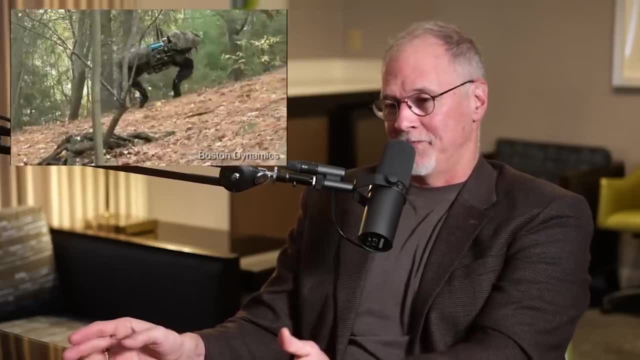 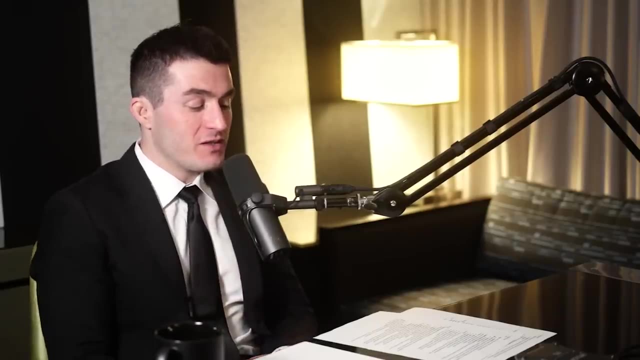 So that was a little bit of a rough transition. Um, I mean, well, can you just comment on the roughness of that transition, Cause, uh, big dog, I mean, this is just big, uh, quadruped four legs robot. 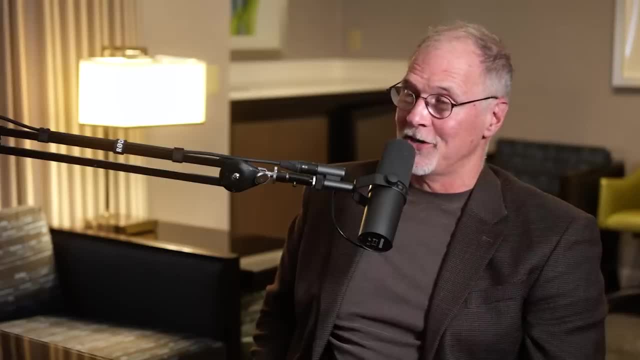 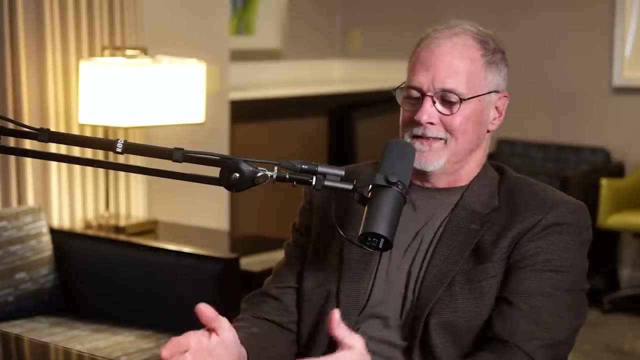 We, we built a few different versions of them, but the first one, the the very earliest ones, you know it didn't work very well and we would take them out And it was hard to get. you know, uh, you know a go-kart engine driving a hydraulic pump. 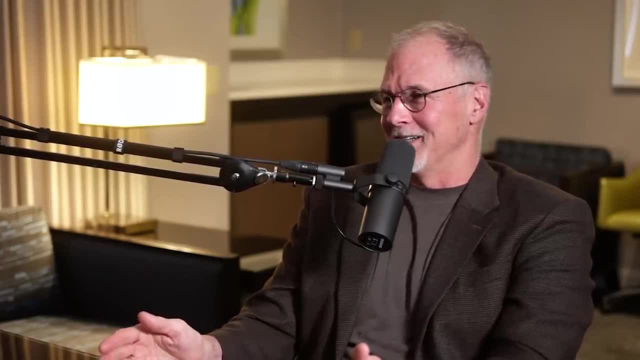 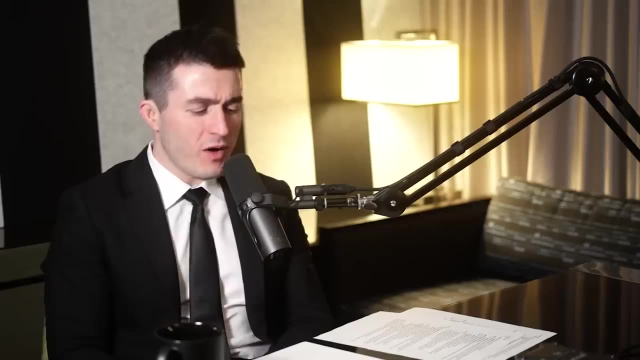 Oh, is that what it was? And and you know, uh, having that all work, Uh, while trying to get, you know, the robot to stabilize itself. And so, what was the power plant? What was the engine? 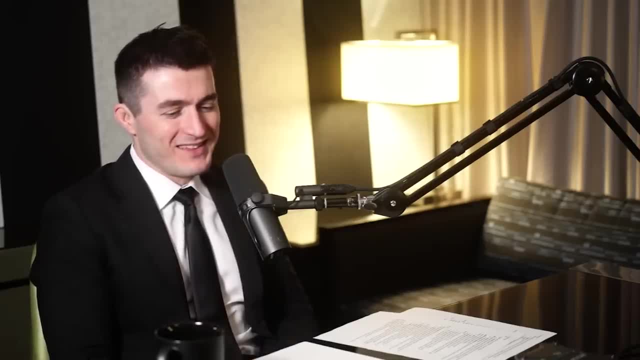 It seemed like- uh- my vague recollection, I don't know. It felt very loud and aggressive and, uh, kind of thrown together, That's what it kind of absolutely was Right, We weren't trying to design the best robot hardware at the time. 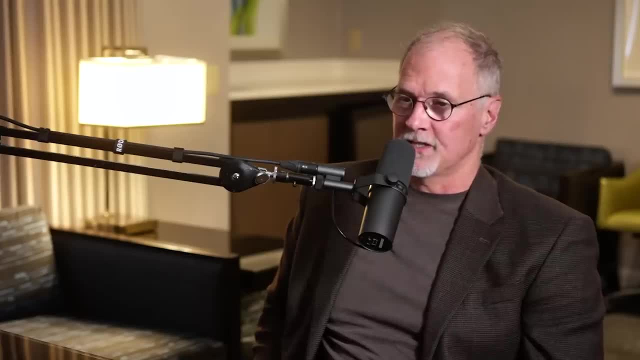 And, um, we wanted to buy an off the shelf engine, And so many of the early Versions of big dog had literally go-kart engines or something like that. Usually it's like a gas powered two stroke engine, And the reason why it was two stroke is two stroke engines are lighter weight, but they're 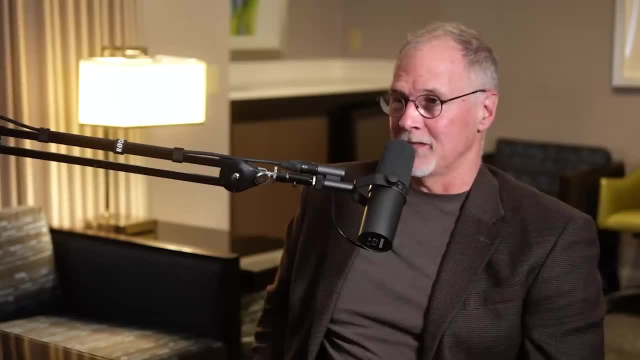 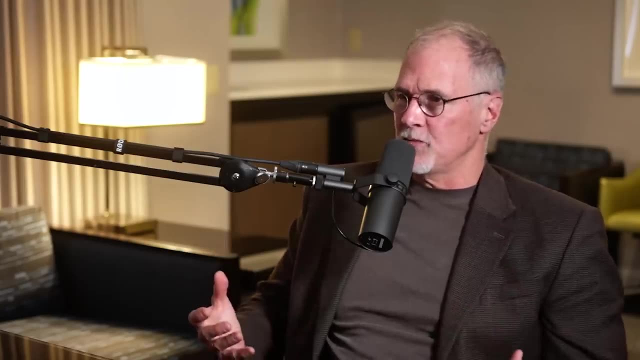 also- and we, we didn't generally- didn't put mufflers on them because we're trying to save the weight and we didn't care about the noise, And so these things were horribly loud. Um, but we're trying to manage weight, because managing weight in a legged robot is always. 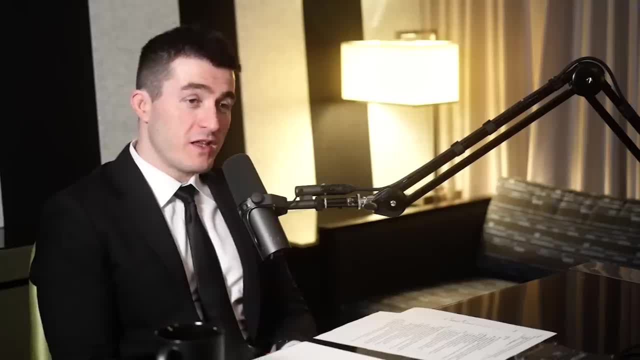 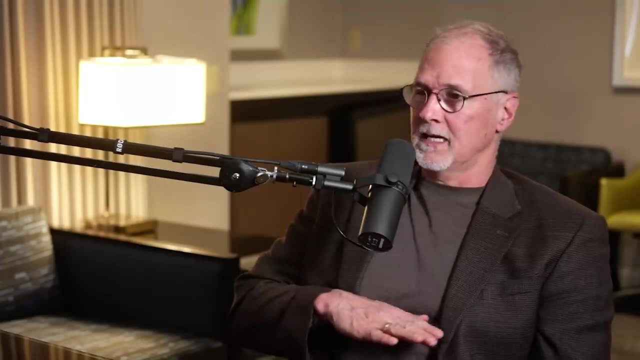 important because it has to carry everything. That said that That thing was big. Well, I've seen the videos. Yeah, I mean the, the, the early versions you know, stood about I don't know. belly high, chest high. 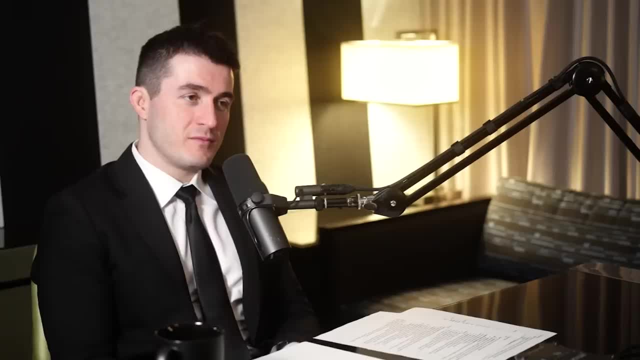 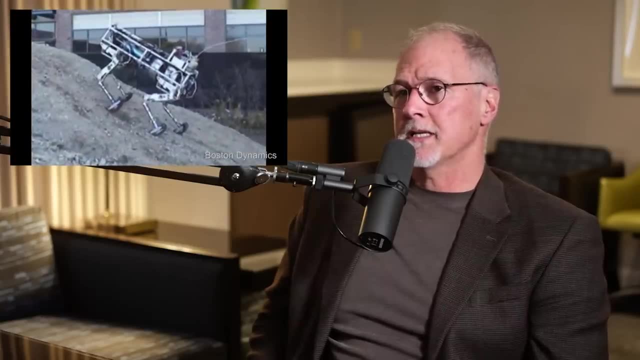 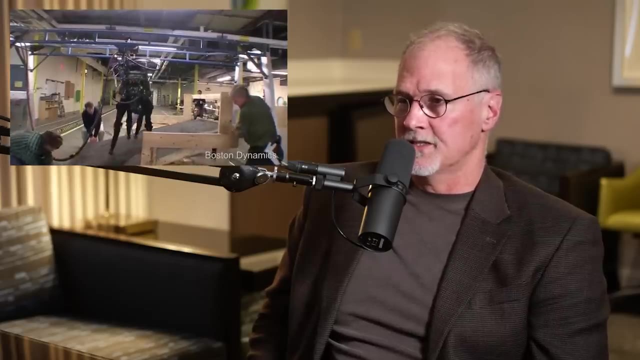 Um, you know, they probably weighed maybe a couple of hundred pounds but, you know, over the course of probably five years, uh, we were able to get that robot um to really manage a remarkable level of rough terrain. So, you know, we started out with just walking on the flat and then we started walking on rocks. 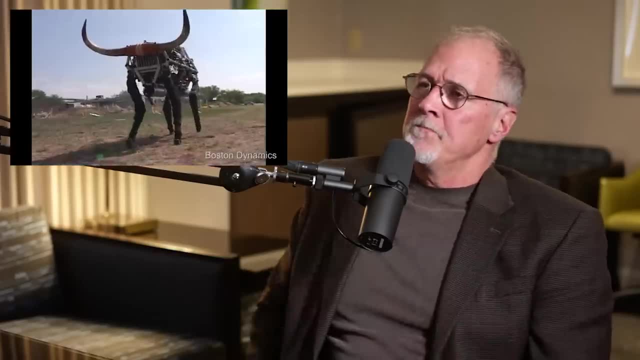 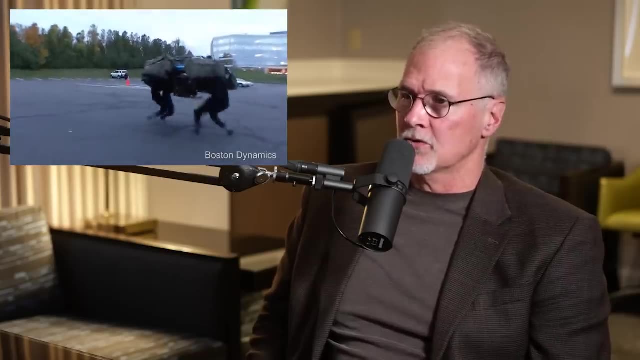 And then inclines, and then mud, and then slippery mud. And you know, by the end of that program we were convinced that legged locomotion and a robot could actually work. because, you know, going into it, we didn't, we didn't know that. 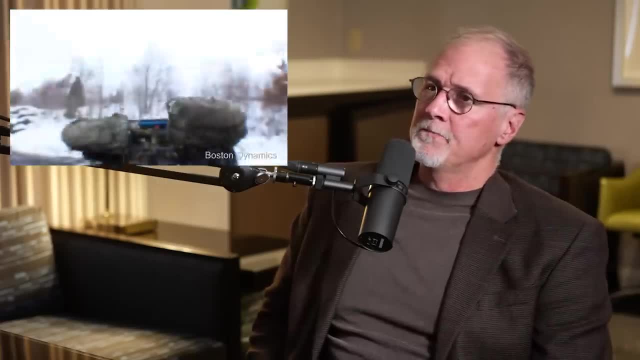 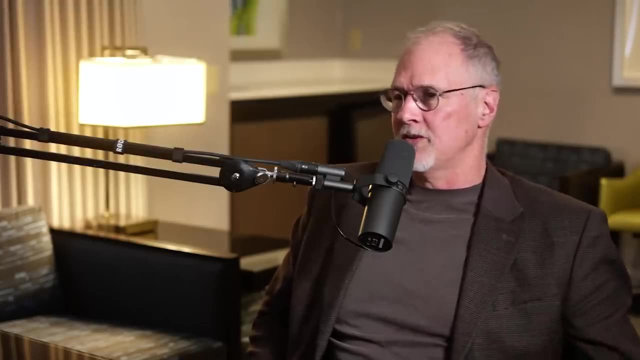 We had built quadrupeds at at MIT, but they were. they used a giant hydraulic pump. you know, in the lab they use a giant computer. that was in the lab. They're always tethered to the lab. This was the first time, something that was sort of self-contained. 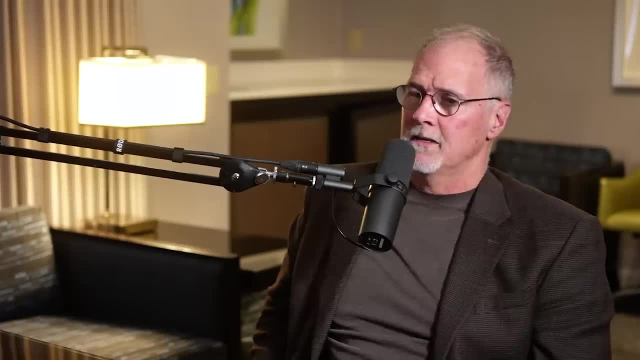 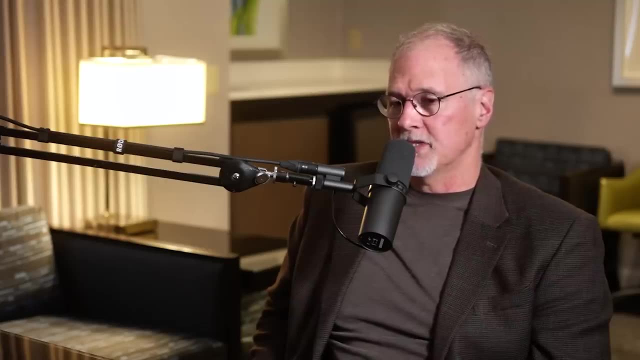 You know, um walked around in the world, um, and and, balanced but, and, and. the purpose was to prove to ourself that the legged locomotion could really work, And so um big dog really cut that open for us. 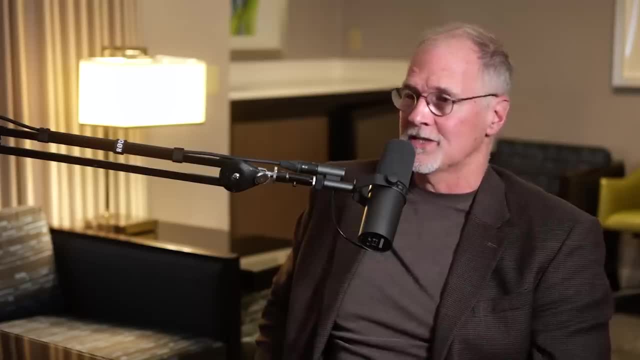 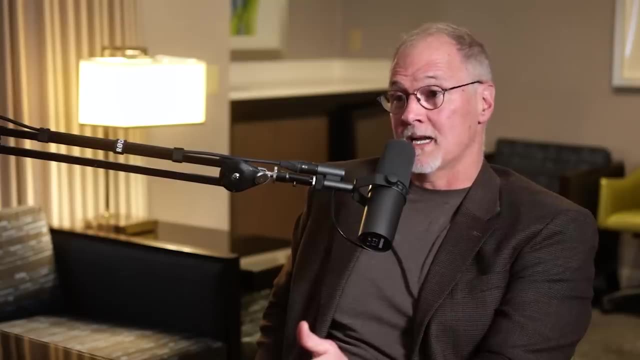 And it was the beginning of what became a whole series of robots. So once, once, we showed to DARPA that you could make a legged robot that could work. there was a period at DARPA where robotics got really hot and there was lots of different programs. 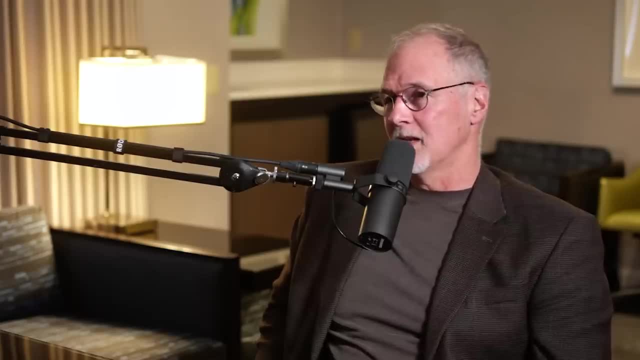 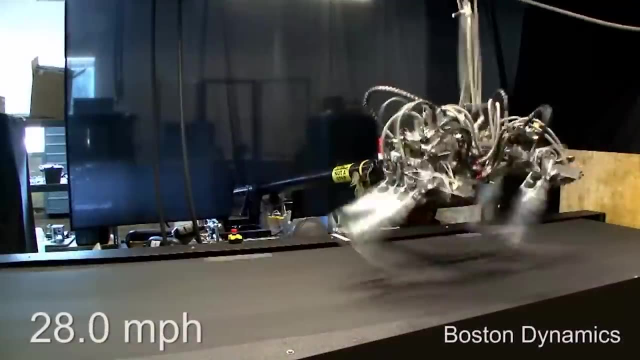 And, um you know, we were able to build other robots. We built other programs. We built quadrupeds to hand, like LS3, designed to carry heavy loads. We built Cheetah, which was designed to explore what are the limits to how fast you can run. 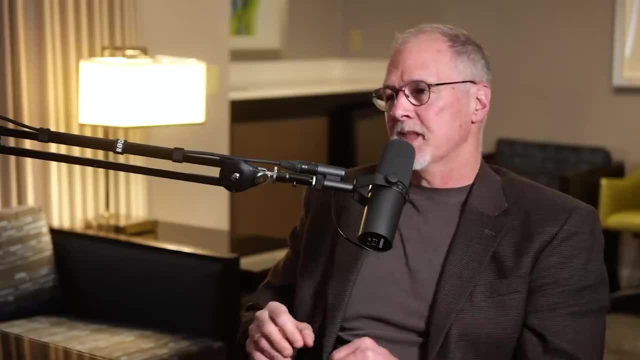 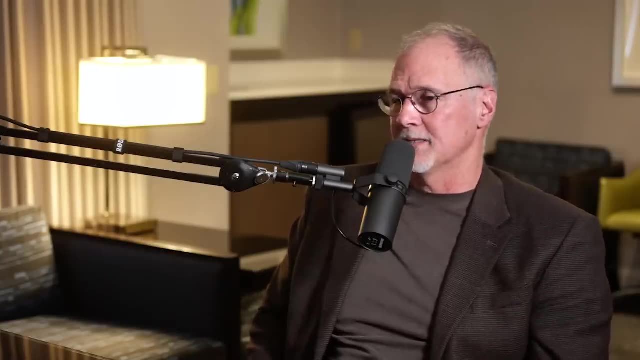 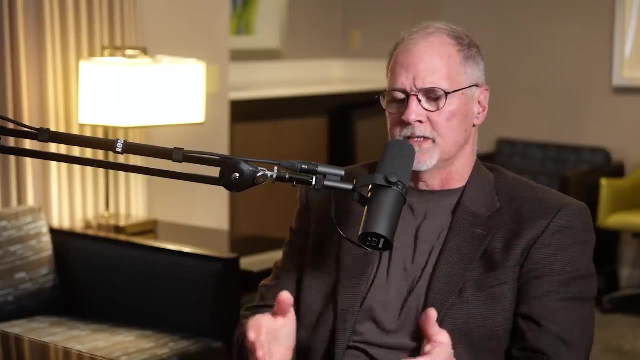 You know, we, we began to build sort of a portfolio of machines and software that led us build not just one robot but a whole family of robots To push the limits in all kinds of directions, Yeah, And to discover those principles. you know, you asked earlier about the art and science of a legged locomotion. 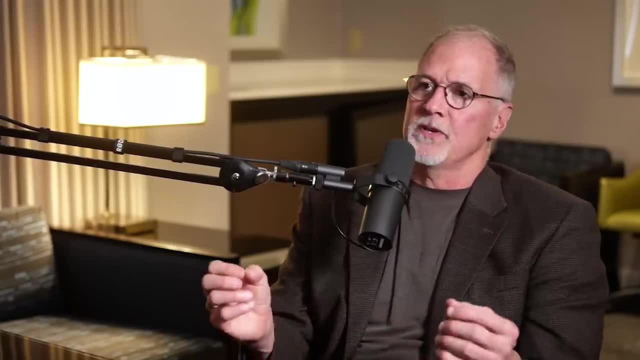 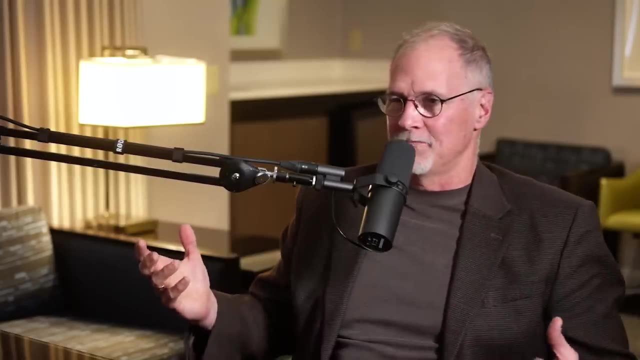 We were able to develop principles of legged locomotion so that we knew how to build a small legged robot or a big one. So the leg leg length, you know, was now a parameter that we could play with. Payload was a parameter we could play with. 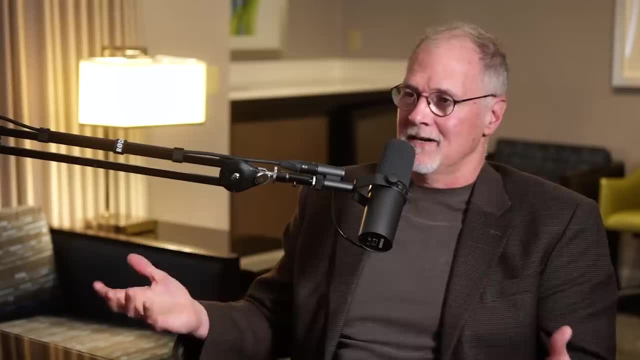 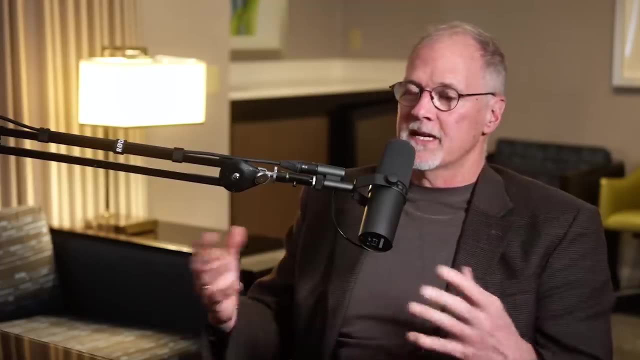 So we built the LS3, which was an 800 pound robot designed to carry a 400 pound payload, And we we learned the design rules, basically developed the design rules. How do you scale different robot systems to you know their terrain to their. 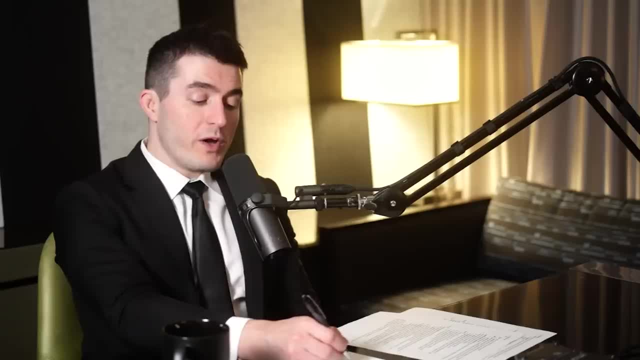 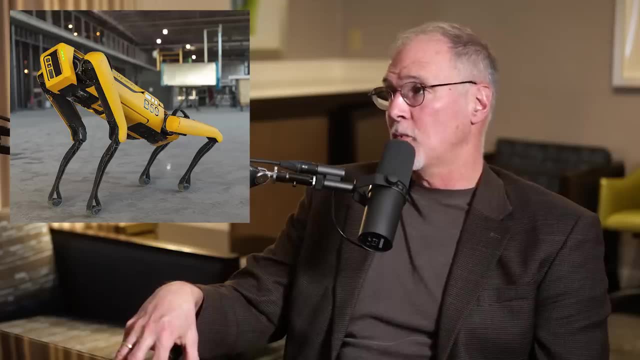 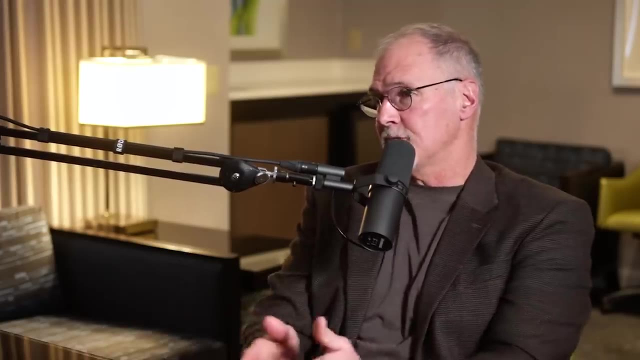 Walking speed to their payload. So when uh was spot born Around 2012 or so, So again almost 10 years into sort of a run with DARPA where we built a bunch of different quadrupeds- We had a sort of a different thread where we started building humanoids. 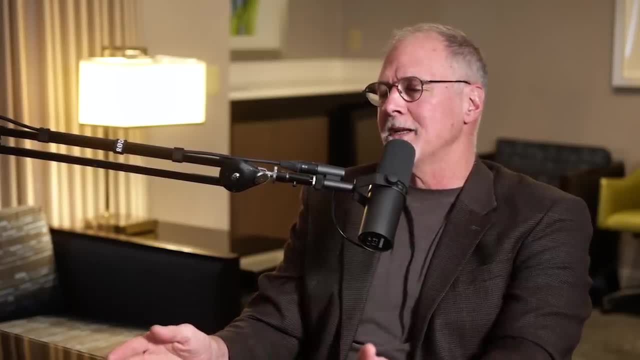 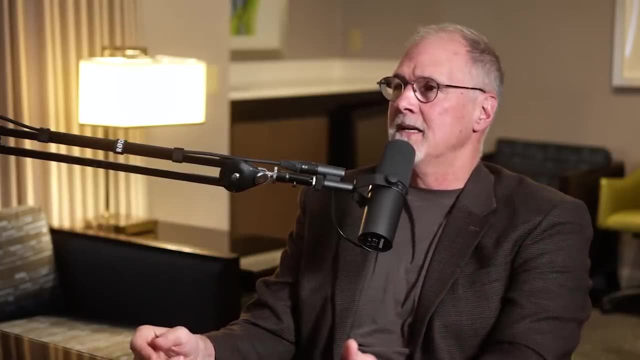 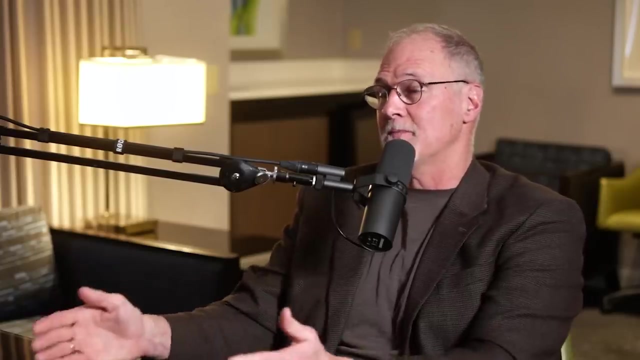 Um, we, we, we saw that probably an end was coming where the government was going to kind of Back Off from a lot of robotics investment and, uh, in order to maintain progress, we just deduced that, well, we probably need to sell ourselves to somebody who wants to continue to invest in this, this area. 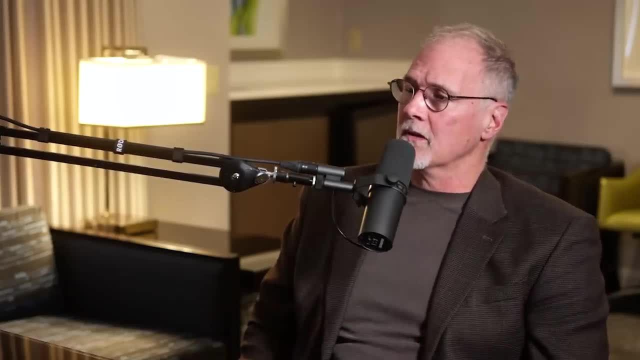 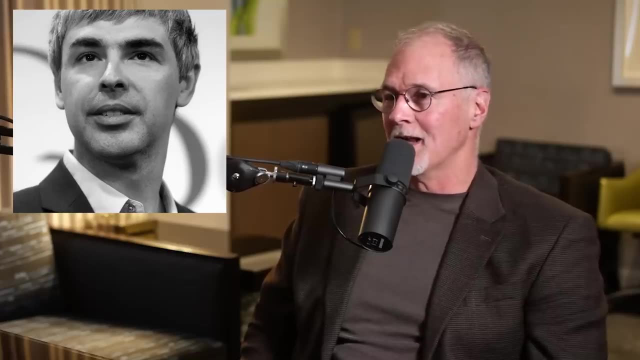 And that was Google. And so, um, uh, at Google, we would meet regularly with Larry page, and Larry just started asking us: you know well what's your product going to be, And you know the logical thing. 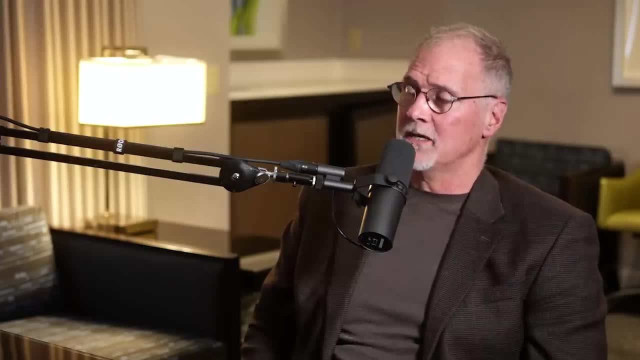 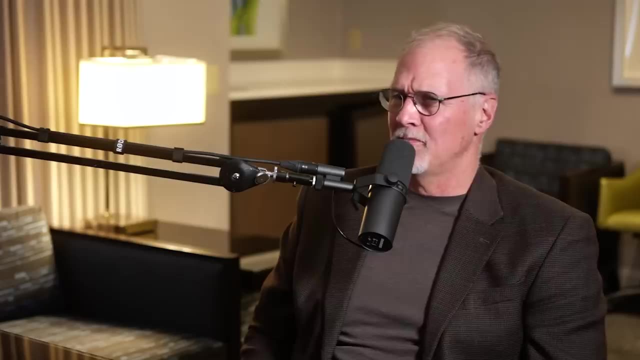 The thing that we had the most history with, that we wanted to continue developing, was a quadruped, but we knew it needed to be smaller. We knew it couldn't have a gas engine. We we thought it probably couldn't be hydraulically actuated. 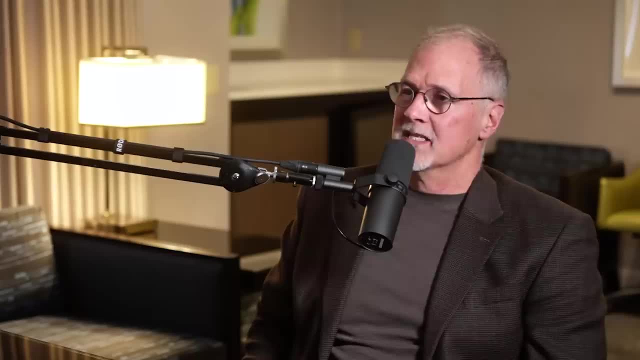 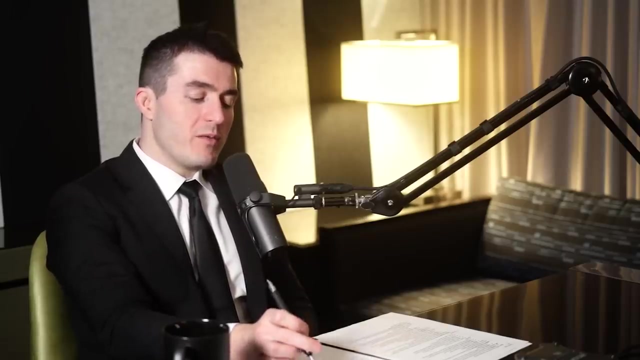 So that began the process of exploring if we could migrate to a smaller electrically actuated um robot, And that was really the genesis of spot. So not a gas engine and the actuators are electric. Yes, So can you maybe comment on what it's like um at Google with working with Larry page, having those meetings and thinking of what will a robot look like that could be built at scale? 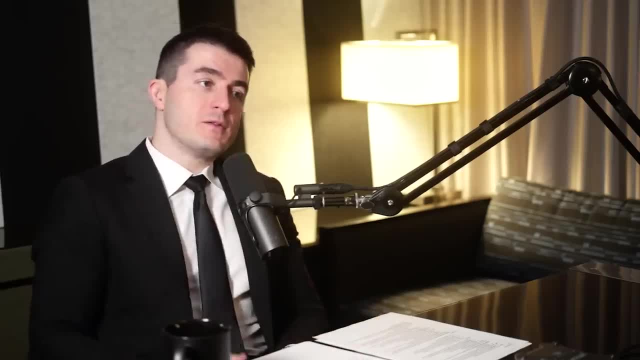 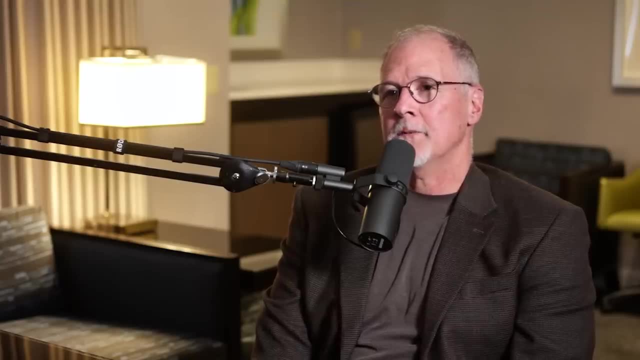 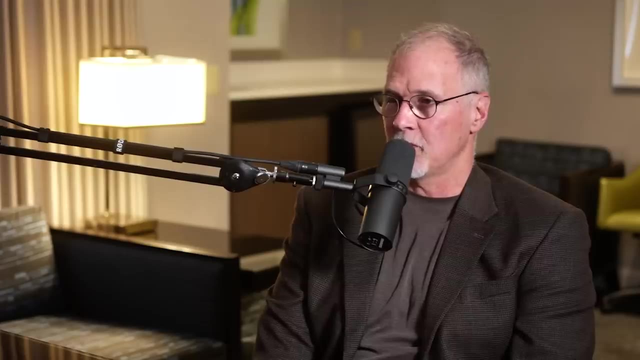 What like starting to think about a product? Larry always liked the the toothbrush test. He wanted products that you used every day. Um, what they really wanted was, you know, a consumer level product, Something that would work in your house. 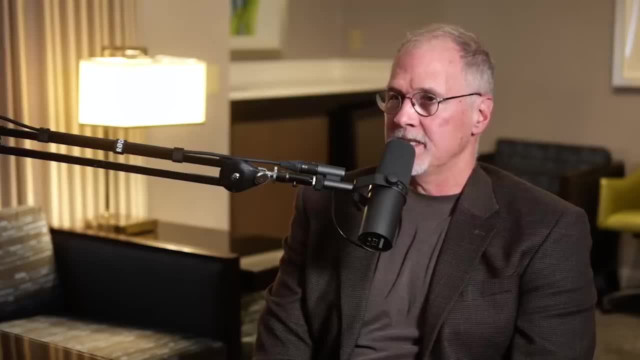 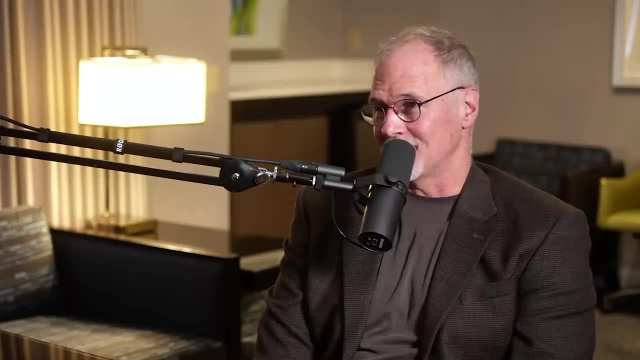 We didn't think that was the right next thing to do because to be a consumer level, product cost is going to be very important, Probably needed to cost a few thousand dollars. And we were. we were building these machines that cost hundreds of thousands of dollars, maybe a million dollars, to build. 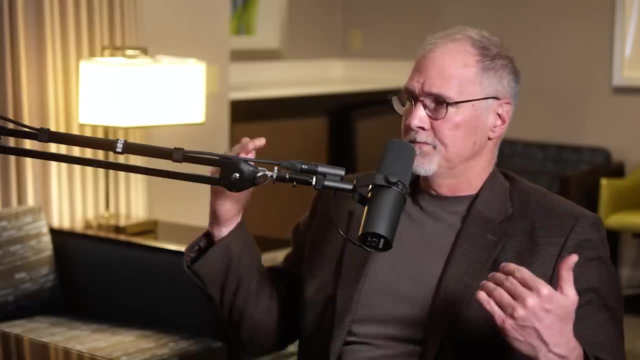 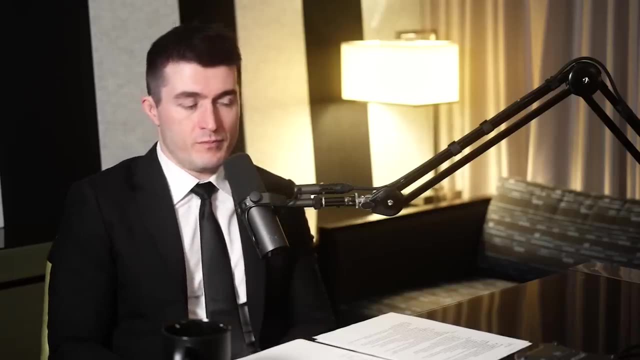 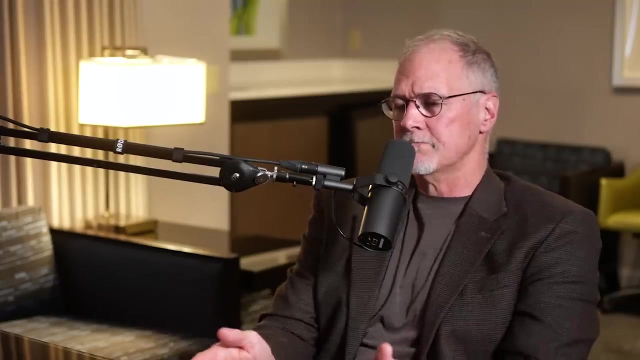 Of course we were only building a two, but but we didn't see how to get all the way to this consumer level product in a short amount of time In a short amount of time. And he suggested that we. we make the robots really inexpensive, and part of our philosophy has always been: build the best hardware. 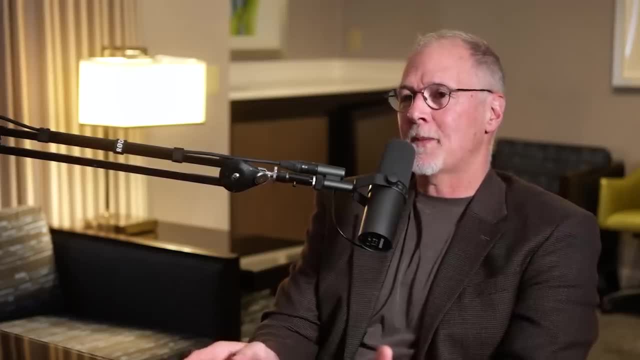 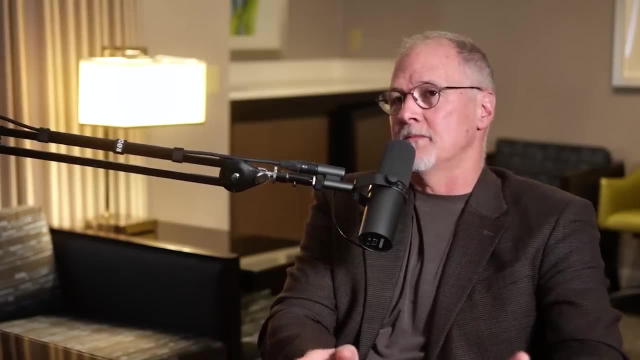 You can make, make the machine operate well, so that you're trying to solve- you know, discover the- the hard problem that you don't know about. Don't don't make it harder by by building a crappy machine. basically, build the best machine you can. 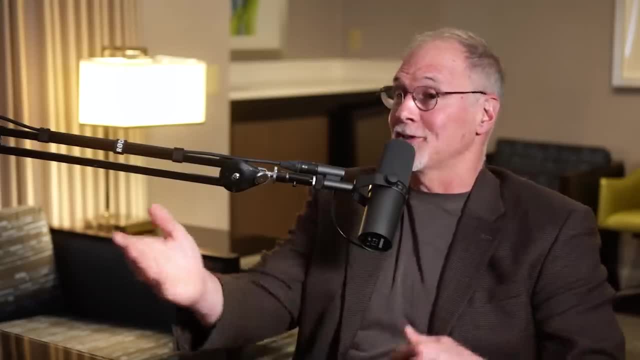 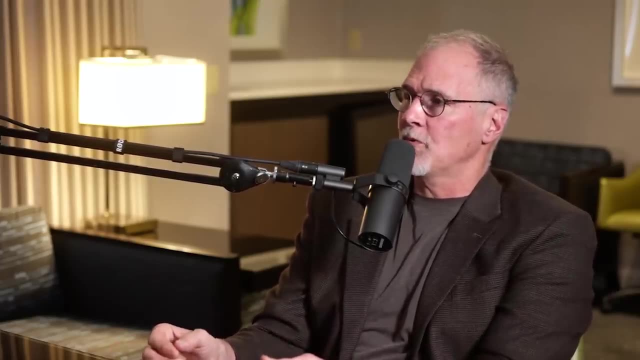 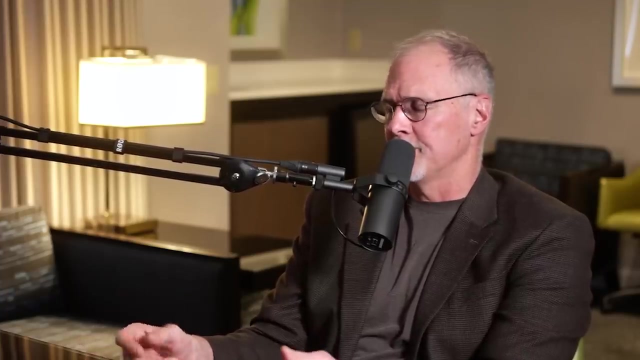 There's plenty of hard problems to solve There That are going to have to do with, you know, under actuated systems and balance, And so we wanted to build these high quality machines still, And we thought that was important for us to continue learning about really what was the important parts of that- make robots work. 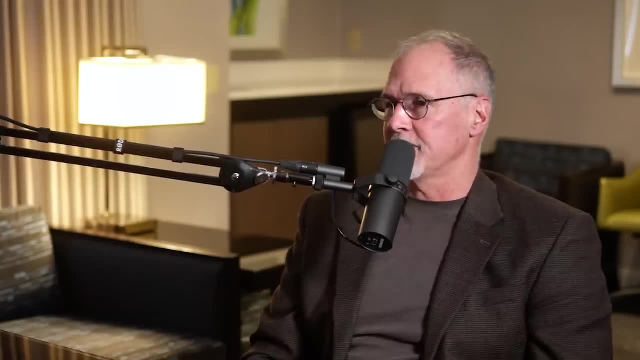 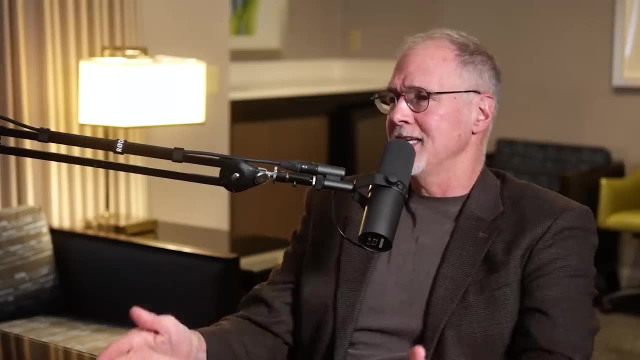 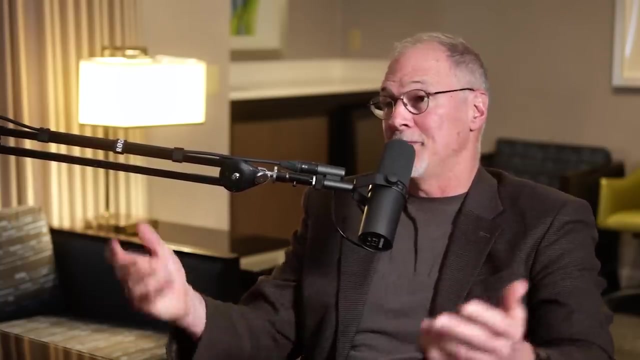 Um and so there was a little bit of a philosophical difference there that we and and so, ultimately, that's why we're building robots for the industrial sector now, because the industry Can afford a more expensive Machine, because you know, their productivity depends on keeping their factory going. 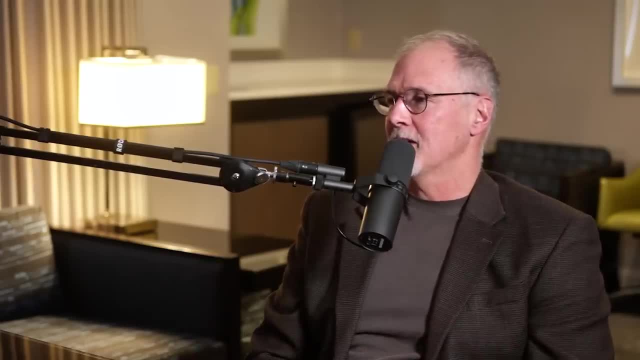 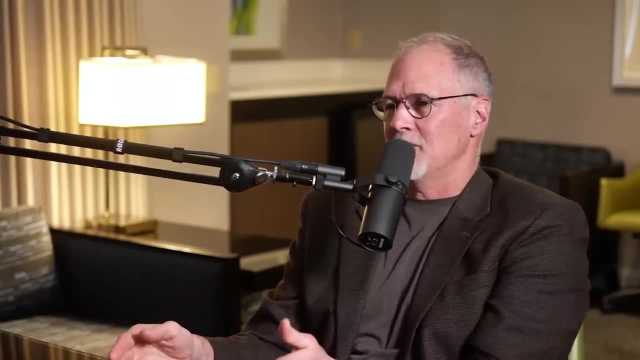 And so if spot costs you know um a hundred thousand dollars or more, that's not such a big expense to them, Whereas at the consumer level no one's going to buy a robot like that, And I think we might eventually get to a consumer level product that will be that cheap. 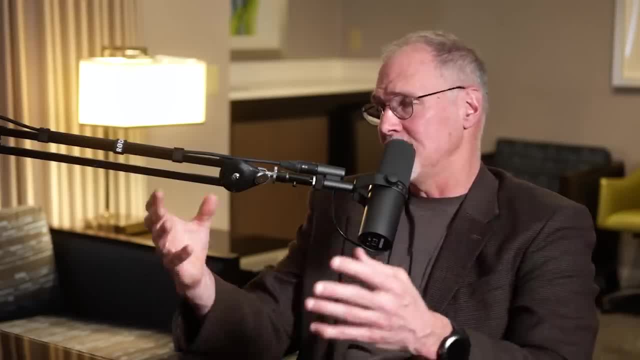 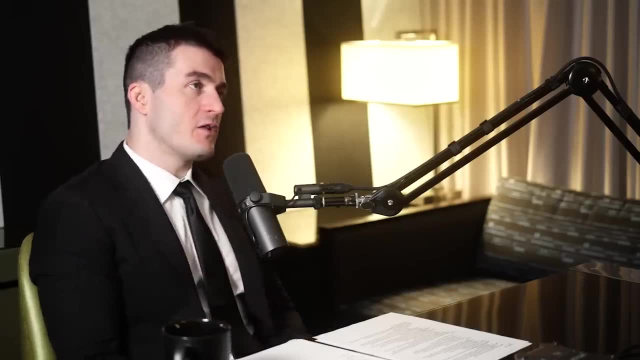 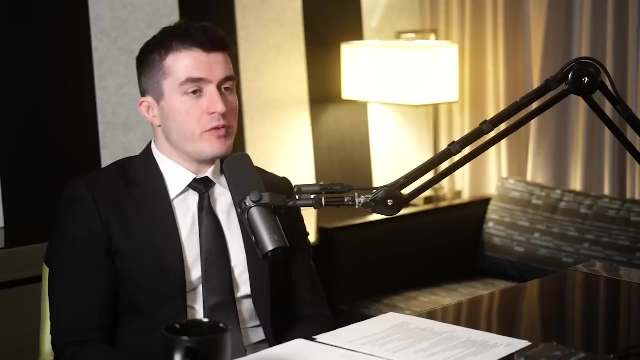 But I think the path to getting there needs to go through these really nice machines so that we can then learn how to simplify. Okay, So what can you say to the almost the engineering challenge of bringing down cost of a robot? So that presumably when you try to build the robot at scale, that also comes into play when you're trying to make money on a robot even in in the industrial setting. 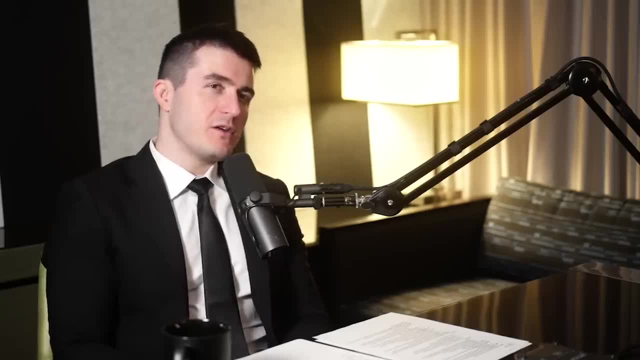 But how interesting, how challenging uh of of a thing is that, in particular probably new to an R and D company. Yeah, I'm glad you brought that last part, The transition from an R and D company to a commercial company. 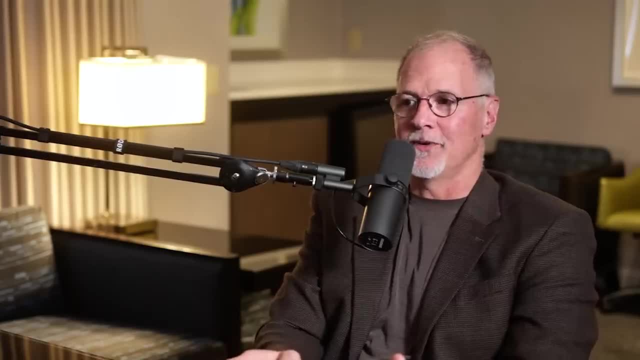 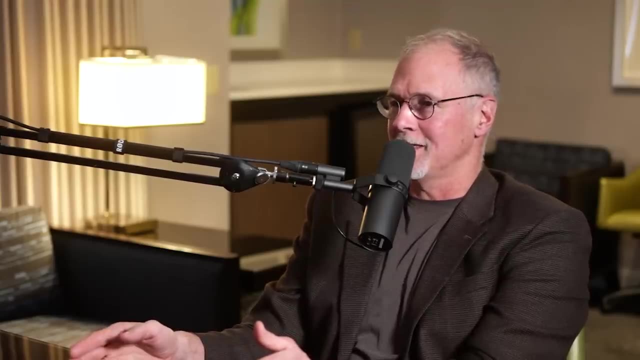 That's the thing you worry about. you know cause you've got these engineers who love hard problems, who want to figure out how to make robots work, And you don't know if you have engineers that want to work on the quality and reliability and costs that is ultimately required. 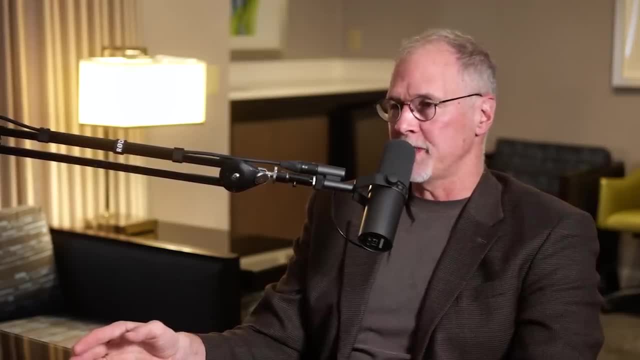 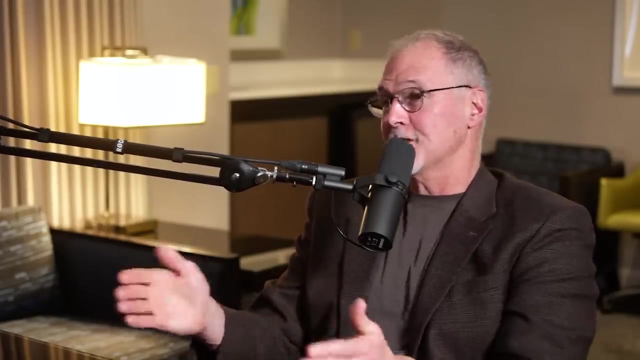 Um, and indeed you know we have brought on a lot of new people who are inspired by those problems, but but the big takeaway lesson for me is we have good people. We have, We have engineers who want to solve problems and and the quality and cost and manufacturability is just another kind of problem. 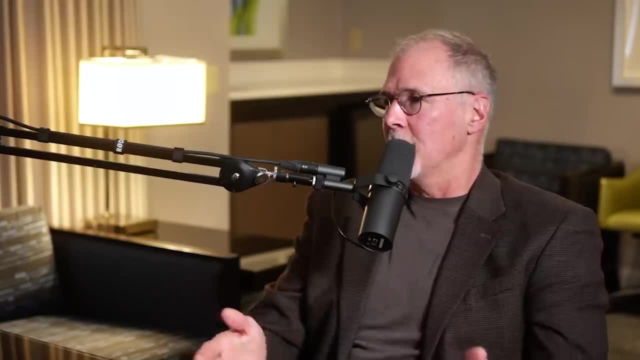 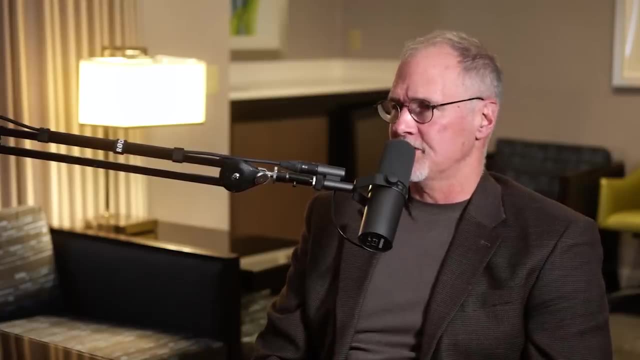 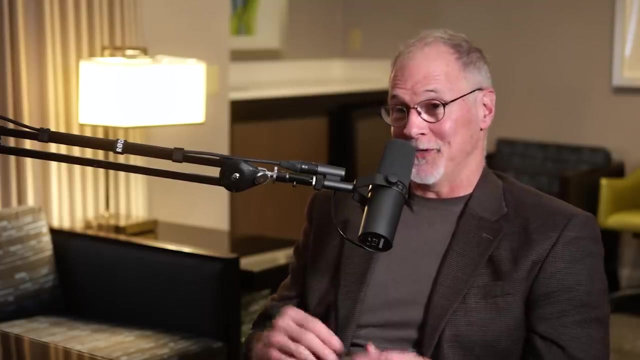 And because they're so invested in what we're doing they're interested in, and we'll go work on on those problems as well, And so I think we're managing that transition very well. In fact, I'm really pleased that I mean, uh, it's a huge undertaking, by the way, right. 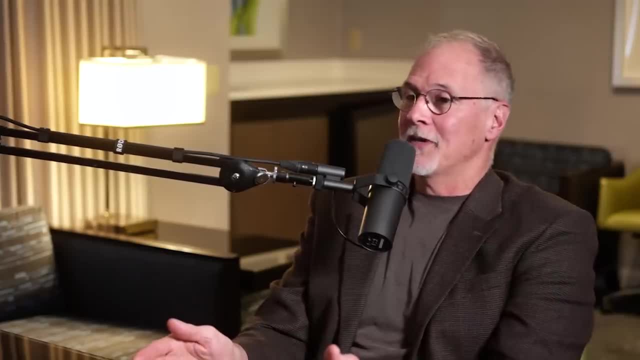 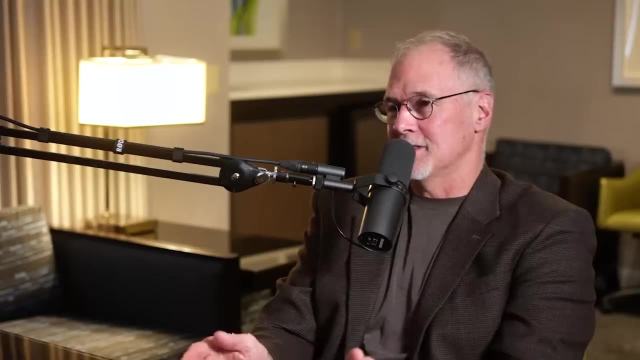 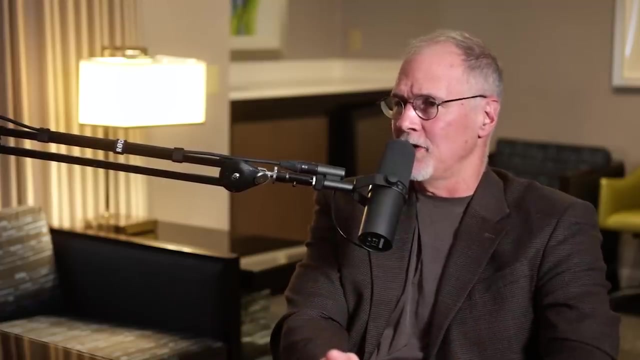 So you know, even having to get Reliability to where it needs to be, We have to have fleets of robots that we're just operating 24, seven in our offices to go find those rare failures and eliminate them. It's a just a totally different kind of activity than the research activity where you get it to work. 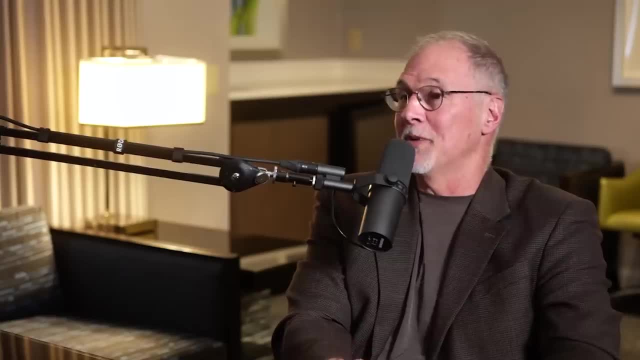 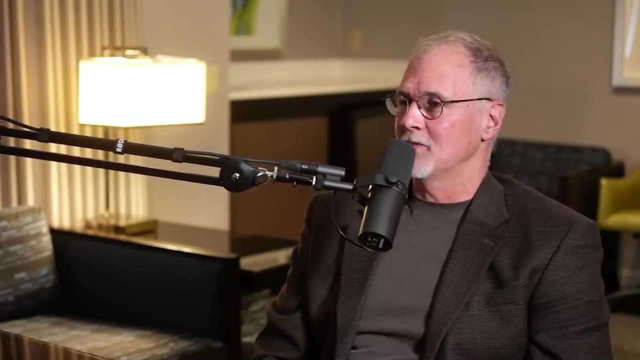 You know the one robot you have to work in a repeatable way. you know, at the, at the high stakes demo, it's just very different, Um, but I think we're making remarkable progress, I guess. So one of the cool things that got a chance to. 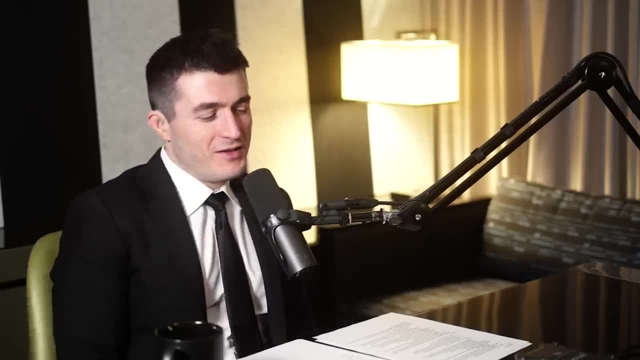 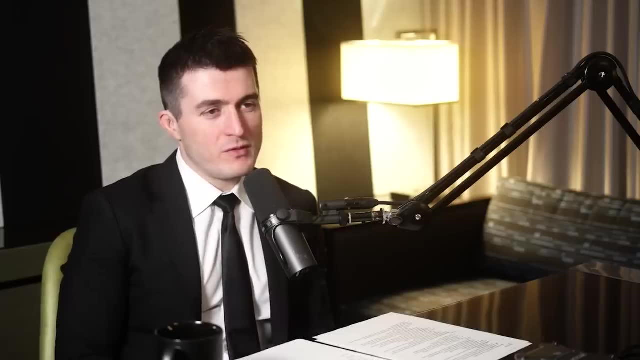 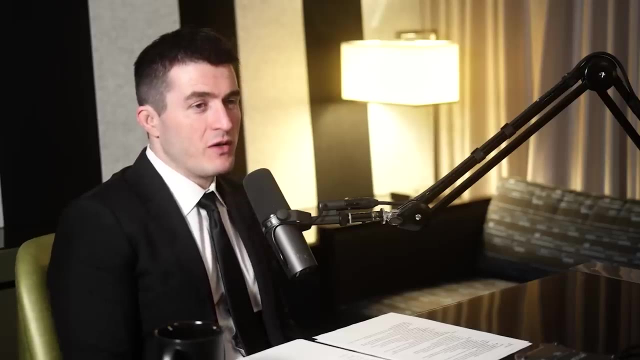 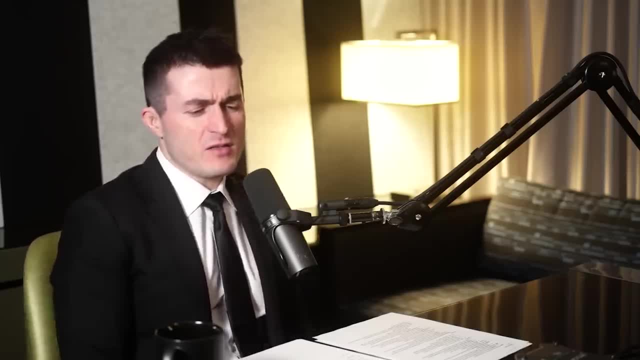 Yeah, Yeah, Yeah, Yeah, For a brief moment of time, but the just to have. I just, I just remember there's like a there's a spot robot, just uh, had like a cowboy hat on and was just walking randomly. 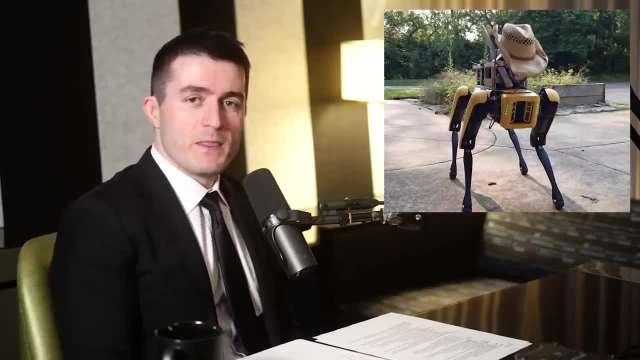 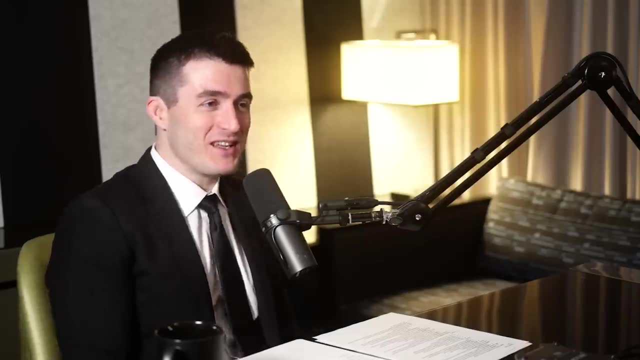 for whatever reason, I don't even know, but there's a kind of a sense of sentience to it because it doesn't seem like anybody was supervising it. It was just doing its thing. I'm going to stop way short of the sentience. 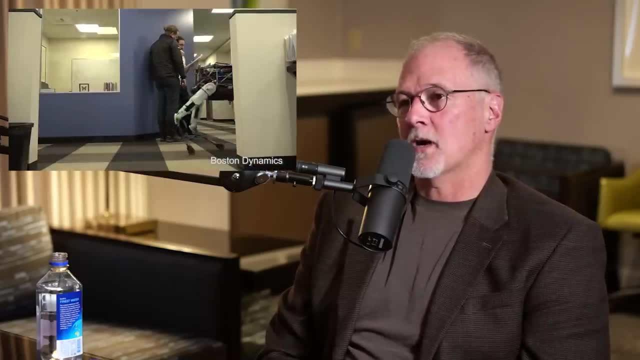 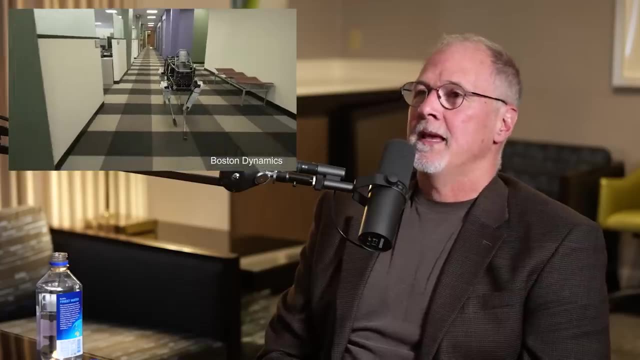 Um, it is the case that if you come to our office you know today, and walk around the hallways, um, you're going to see a dozen robots. It's just kind of walking around all the time And that's really a reliability test for us. 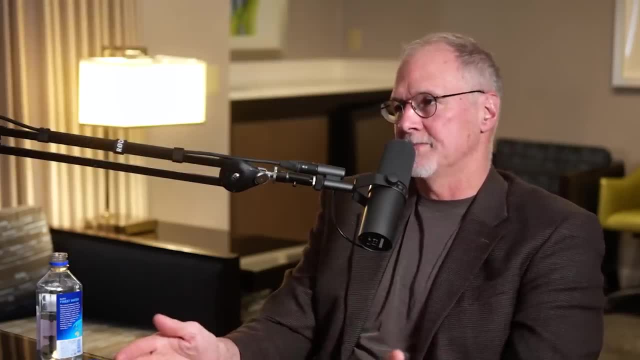 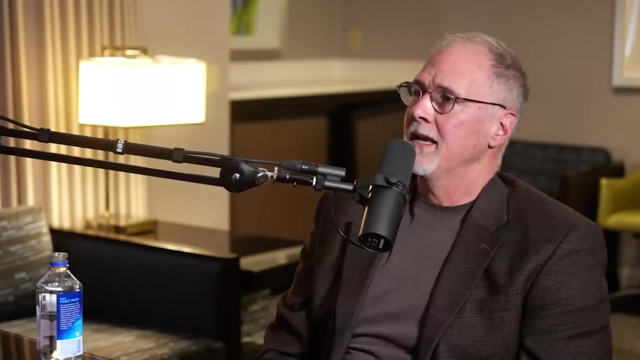 So we have these robots programmed to do autonomous missions: get up off their charging dock, walk around the building, collect data at a few different places and go sit back down, And we want that to be a very reliable process, because that's what somebody who's running 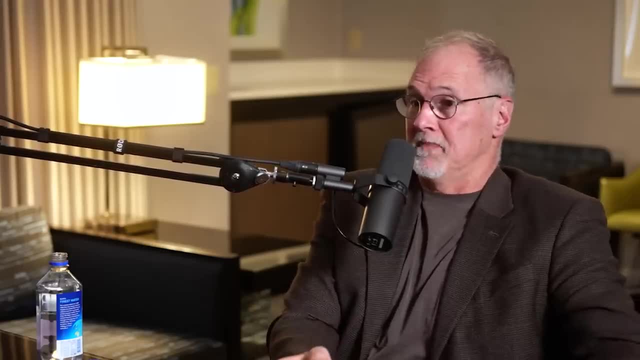 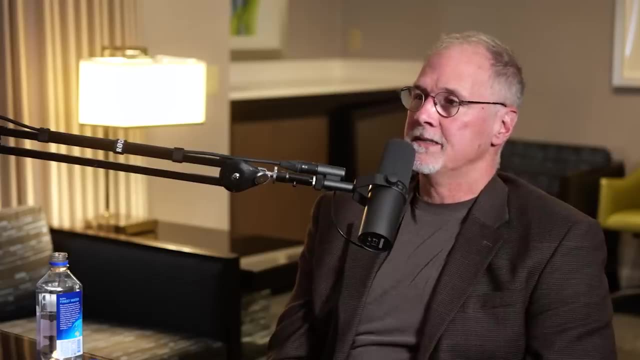 a- uh, a brewery, a factory. that's what they need the robot to do, And so we have to. we have to dog food our own robot, We have to test it in that way, And um so, on a weekly basis, we have robots that are accruing something like um 1500. 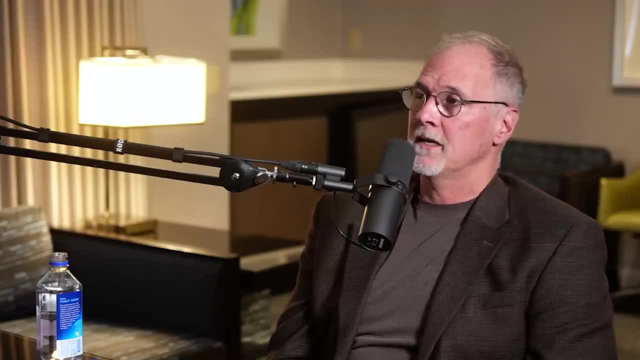 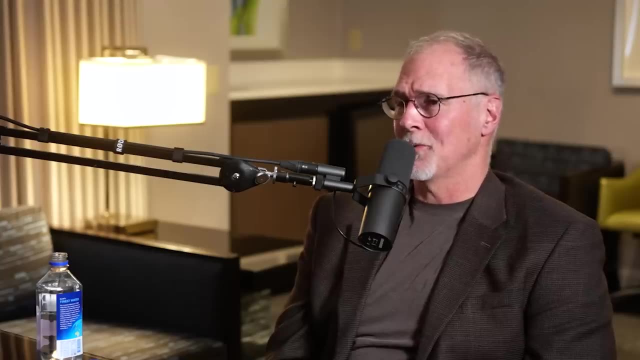 or maybe 2000 kilometers of walking and, uh you know, over a thousand hours of operation every week, And that's something that almost I don't think anybody else in the world can do, because a you have to have a fleet of robots to just accrue that much information. 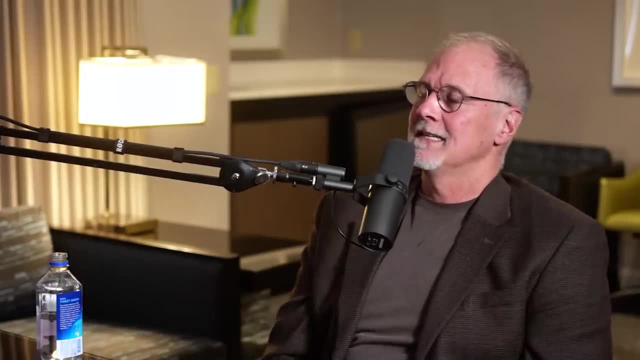 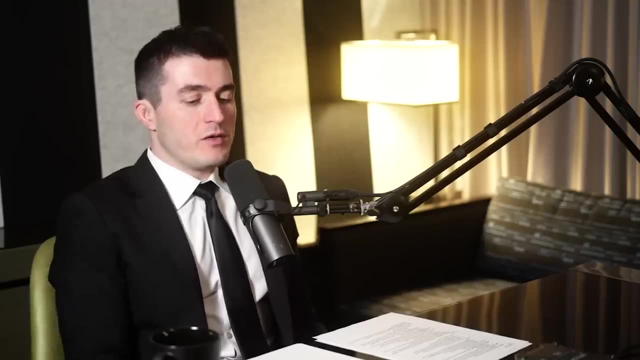 You have to be willing to dedicate it to that test And uh, So that's, but that's essential. That's how you get the reliability. That's how you get it. What about some of the cost cutting from the, from the manufacturer side? 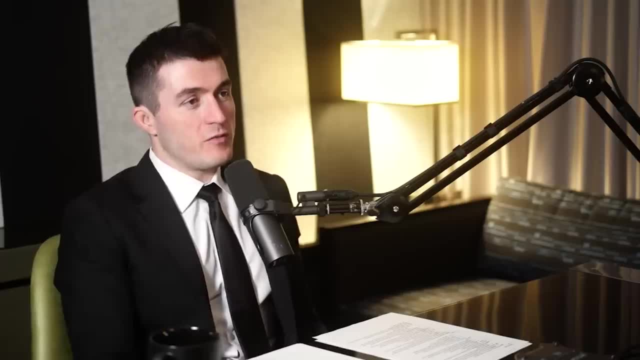 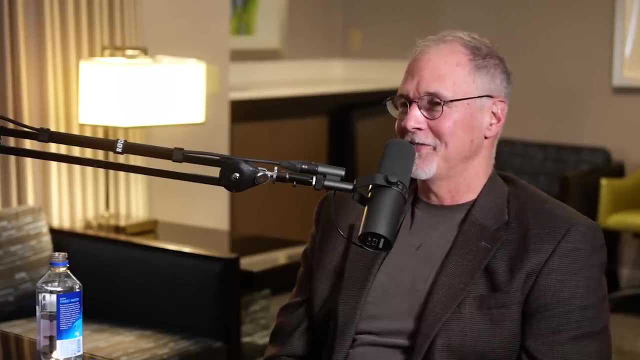 What? what have you learned from the manufacturer side of the transition from R and D? And we're still, we're still learning a lot there. Um, we're learning how to cast parts and sell instead of mill it all out of you know. 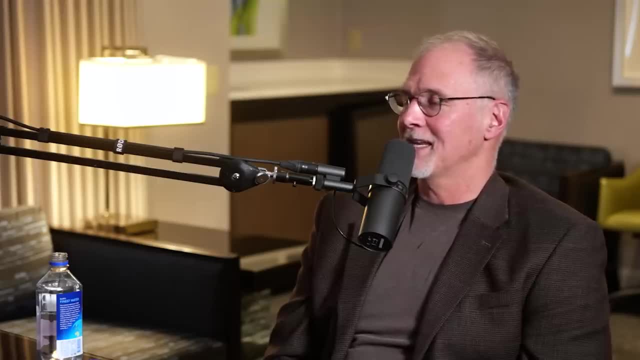 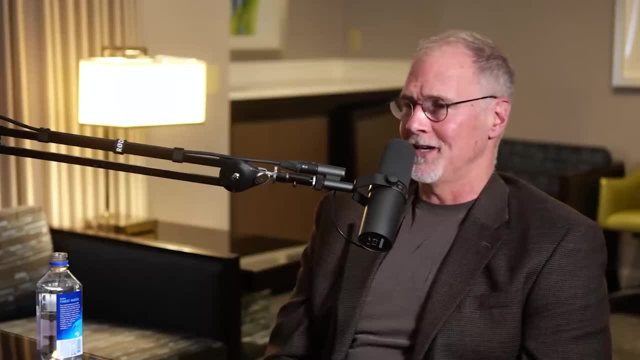 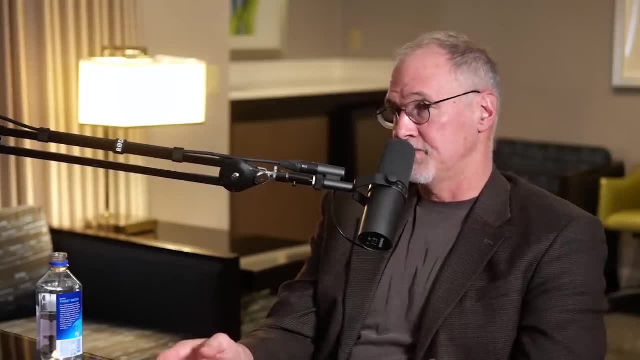 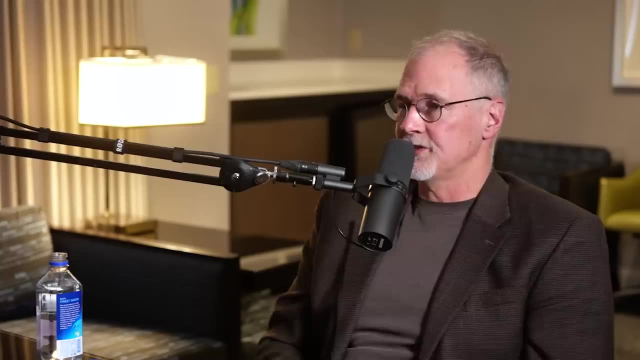 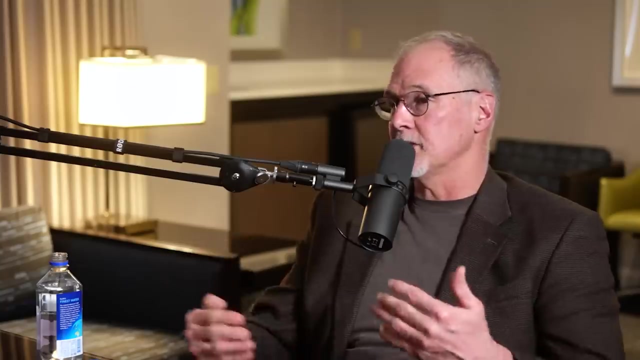 Um, we've, we've set up a manufacturing facility in Wolf M- It's about a mile from our headquarters- and we're doing final assembly and tests of both spots and stretches. you know, at that factory And um, and it's hard because, to be honest, we're still iterating on the design of the 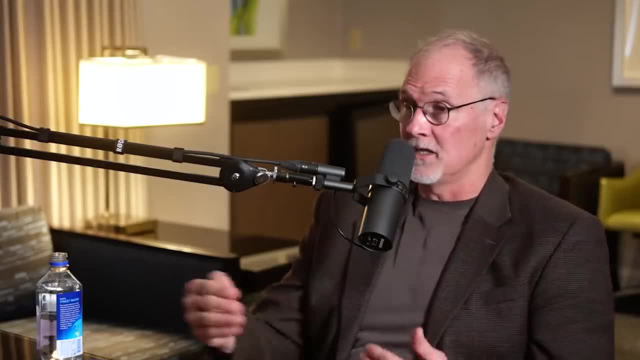 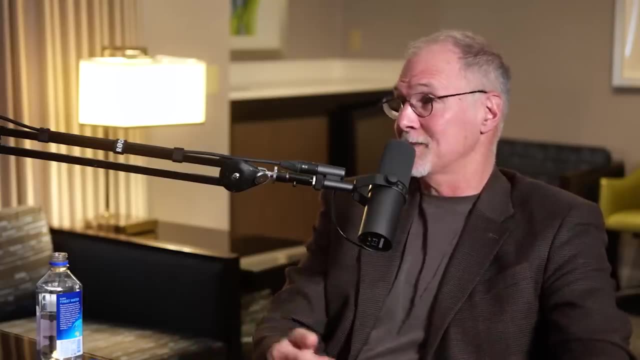 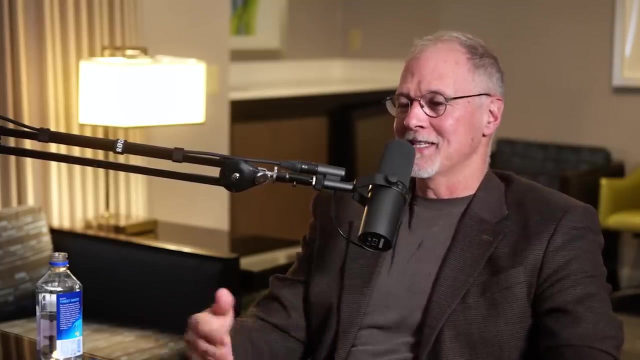 robot. As we find failures from these reliability tests, we need to go engineer changes- Yeah, changes, and those changes need to now be propagated to the manufacturing line. and that's a hard process, especially when you want to move as fast as we do, and that's been challenging and it makes 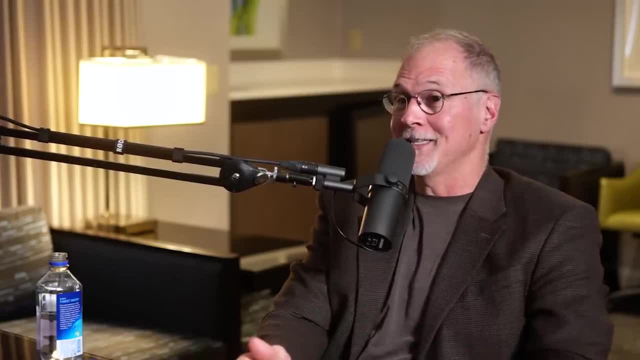 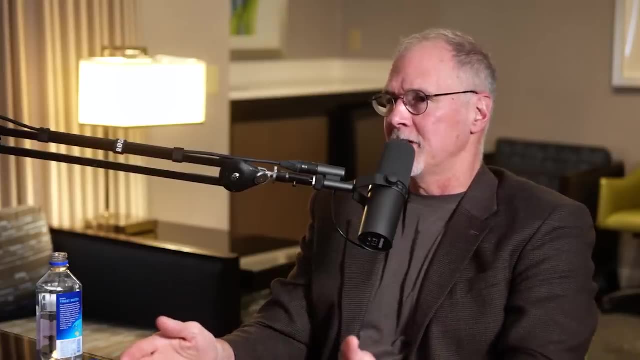 it. you know, the folks who are working supply chain, who are trying to get the cheapest parts, for us kind of requires that you buy a lot of them to make them cheap and then we go change the design from underneath them. they're like: what are you doing? and so you know getting everybody on the 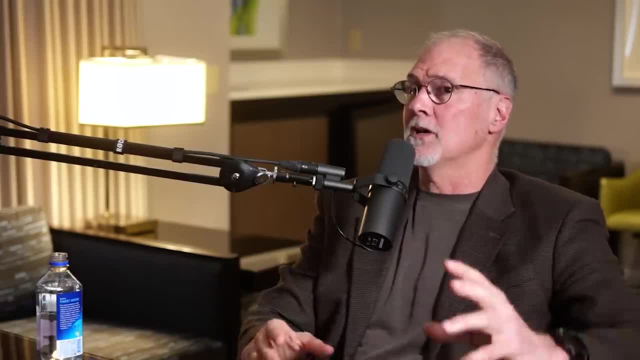 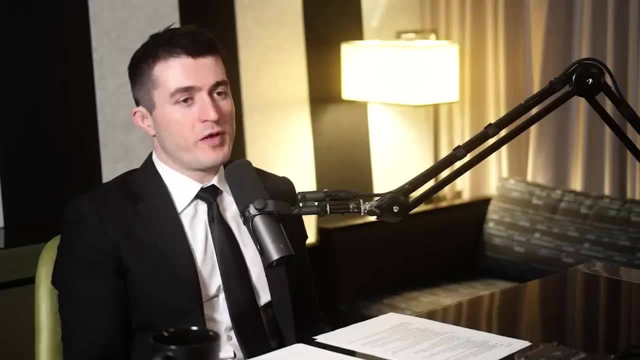 same page here that it? yep, we still need to move fast, but we also need to try to figure out how to reduce cost. that's one of the challenges of of this migration we're going through and over the past few years, challenges to the supply chain. i mean, i'm imagining you've been a part of a bunch. 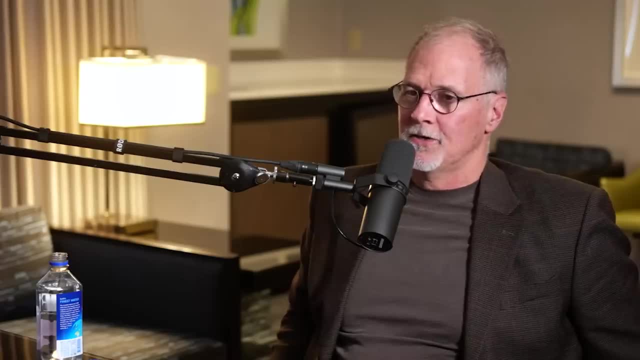 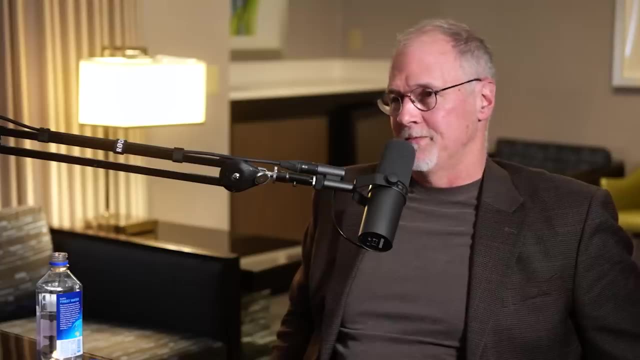 of stressful meetings. yeah, things got more expensive and harder to get, and yeah, so it's. it's all been a challenge. is there still room for simplification? oh, yeah, much more. and you know, these are really just the first generation of these machines. we're already thinking about what the next generation of spots going to look like. 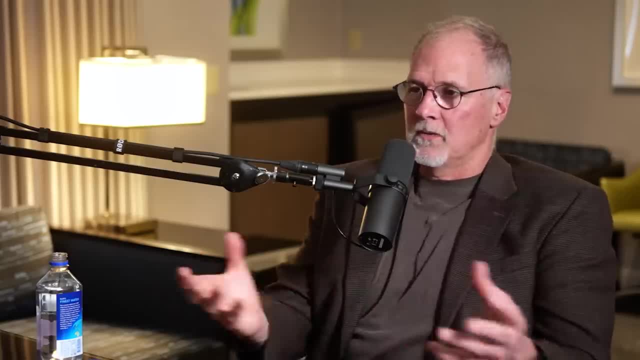 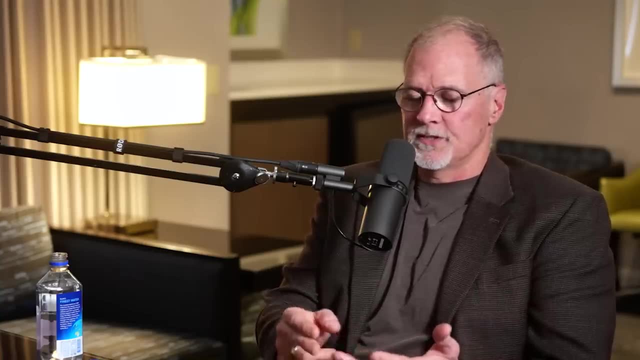 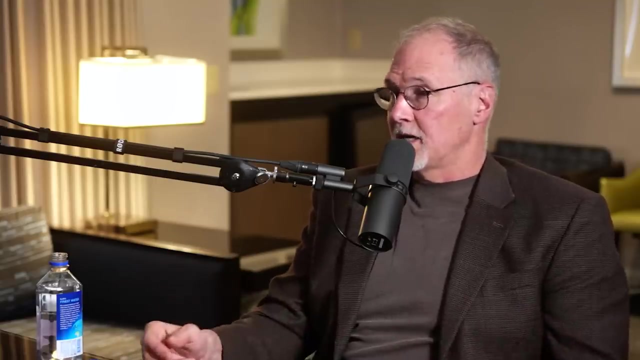 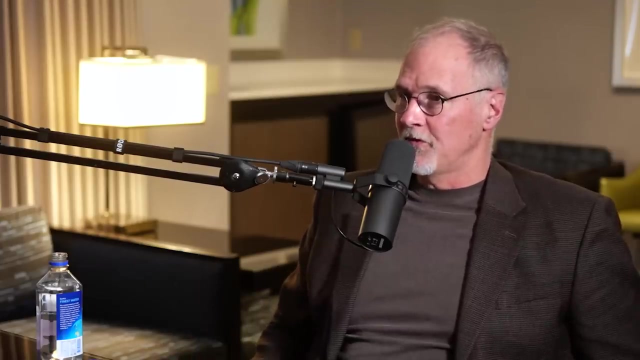 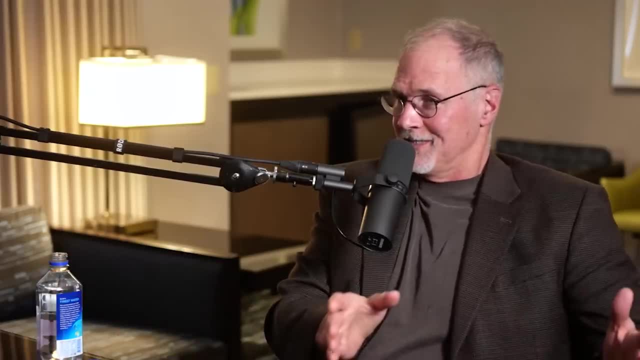 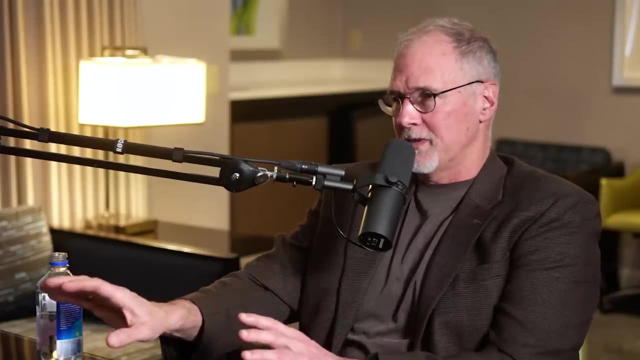 we're going to be able to do that, and that's the difference between the general purpose machine, or the platform, versus the purpose-built machine. and so, even though even in the factory we'd still like the robot to do lots of different tasks, if it's, if we really knew on day one that 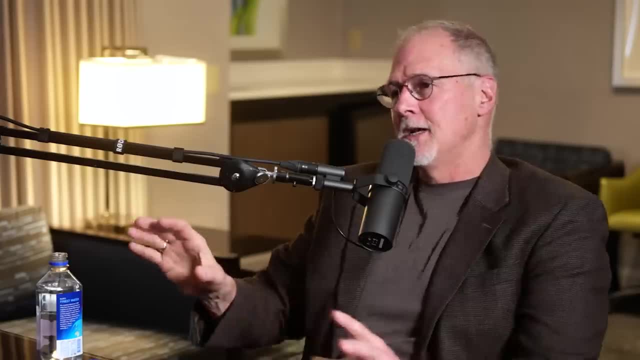 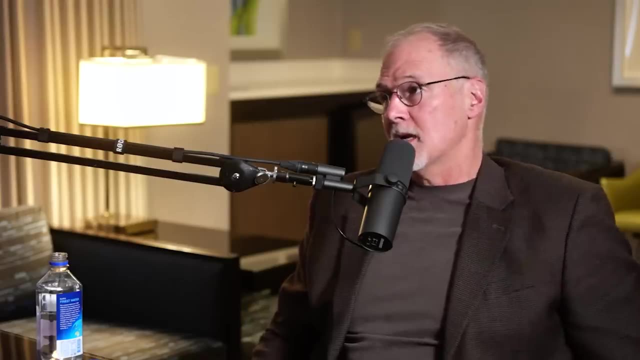 we're going to be operating in a factory with these three sensors in it. we would have it all integrated in a package that would be easier, more less expensive and more reliable. so we're contemplating building, you know, a next generation of that machine. so we should mention that the 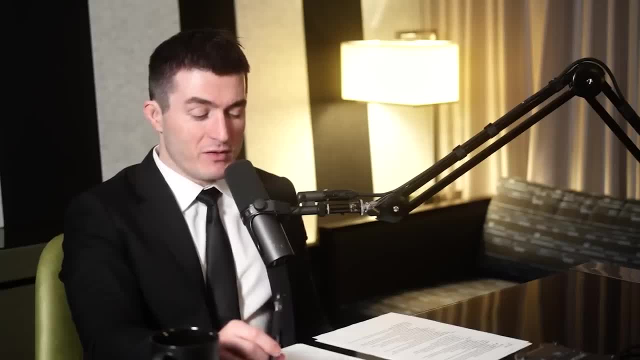 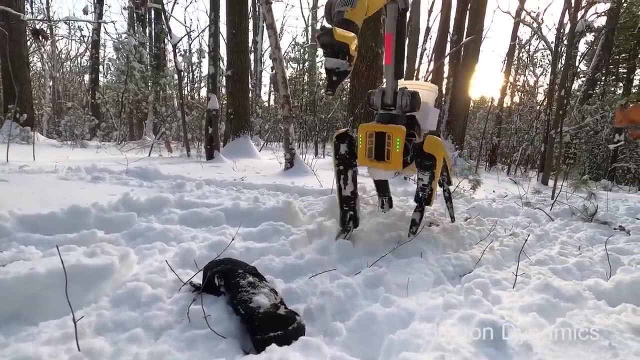 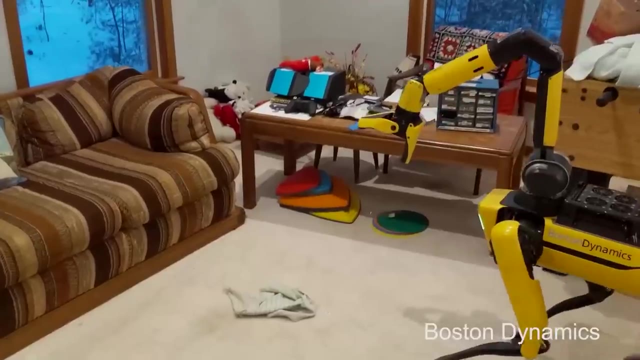 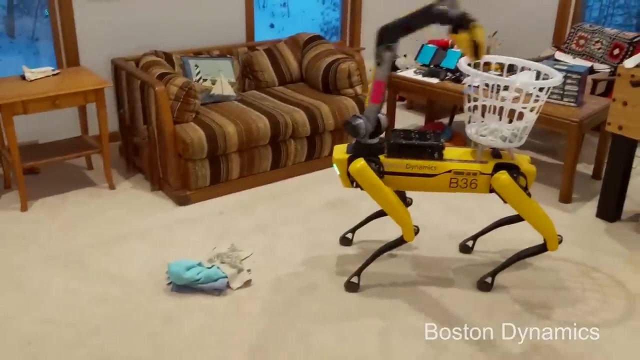 so spot. for people who somehow are not familiar: uh, so it's a yellow robotic dog and um has been featured in many dance videos. uh, it also has gained an arm. so what can you say about the arm? that spot has bought the challenges of this design and the manufacturer of it. we think the future of 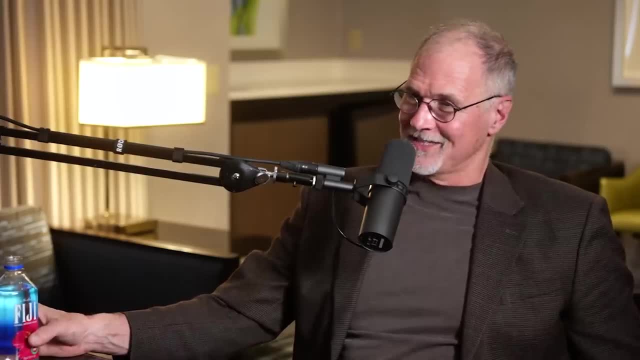 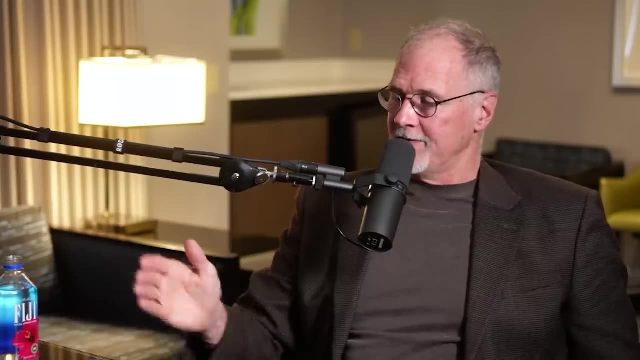 mobile robots is mobile manipulation. that's where you know, in the past 10 years it was getting mobility to work, getting the legged locomotion to work. if you ask what's the hard problem in the next 10 years, it's getting a mobile robot to do. 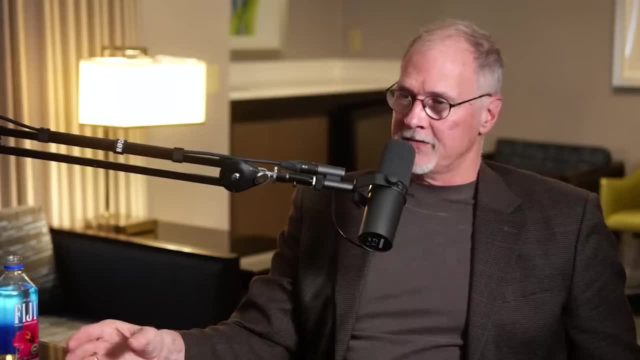 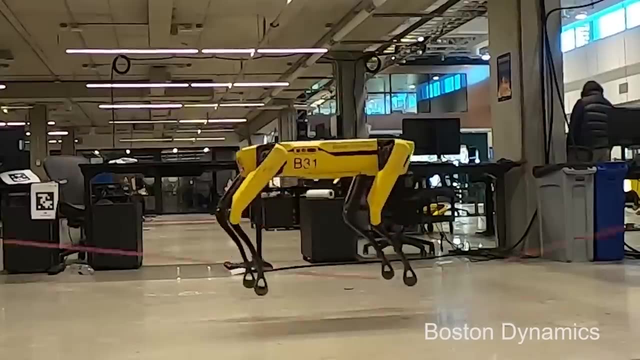 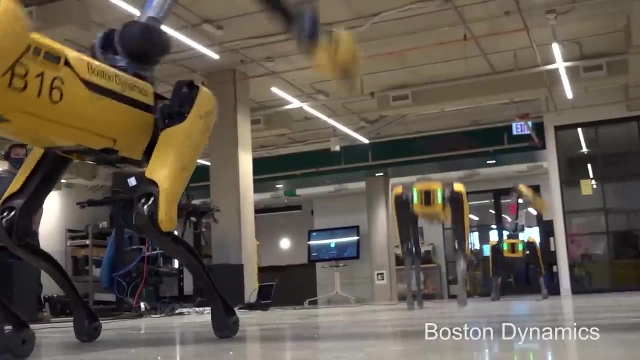 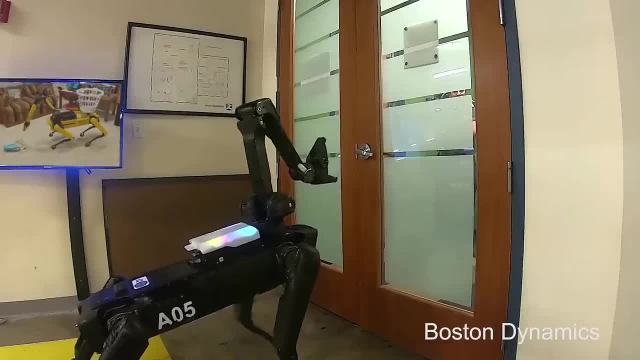 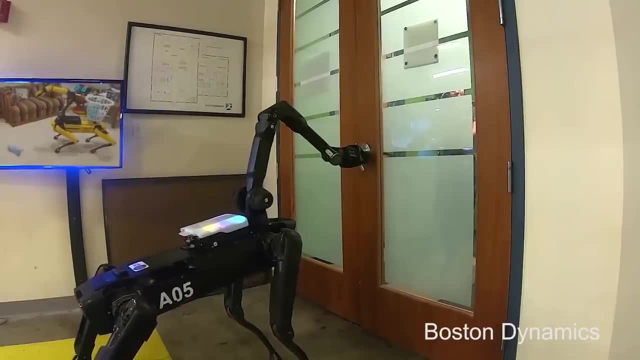 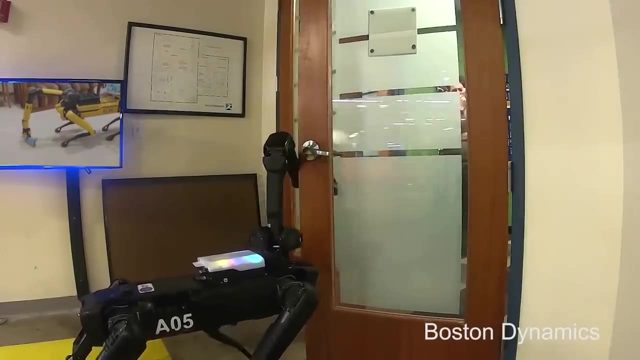 um, it has, you know, several motors and actuators and sensors. it has a camera in the end of its hand. so, you know, you can sort of see something, the- and the robot will control the motion of its hand to go pick it up autonomously. so, in the same way, the robot walks and balances, managing its own foot. 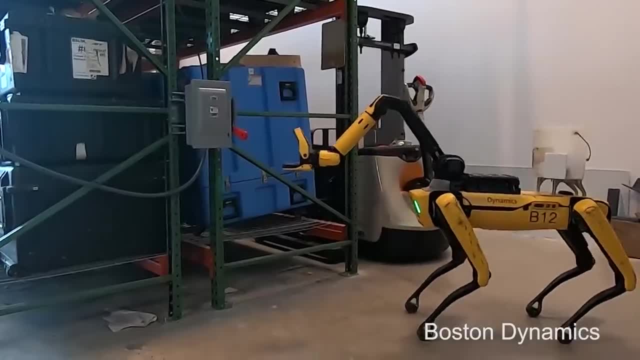 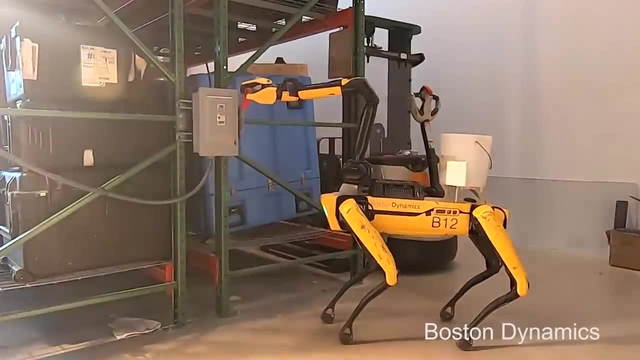 placement to stay balanced. we want manipulation to be mostly autonomous, where the robot you indicate: okay, go grab that bottle, and then the robot will just go do it. you're going to be able to use the camera in its hand and then sort of closing in on that um the grasp, but it's, it's a. 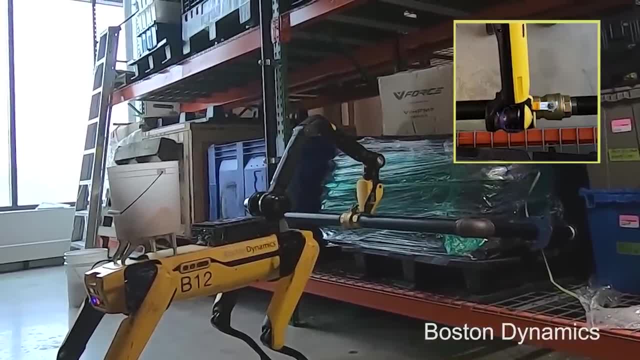 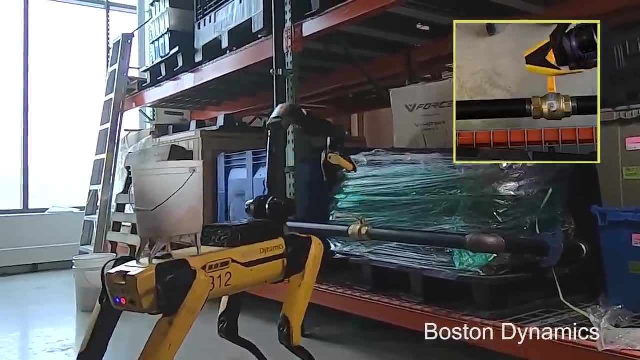 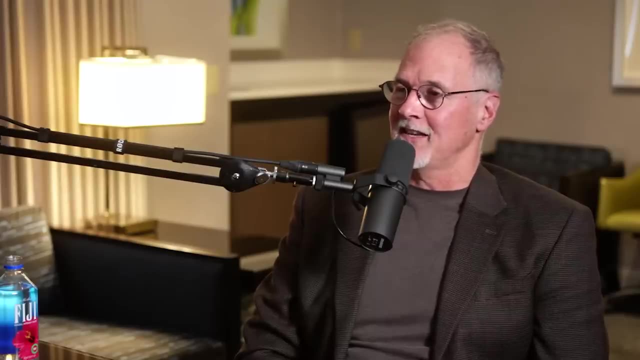 whole nother complex robot on top of a complex legged robot, and so, and of course we made it the hand look a little like a head, you know, because again we want it to be sort of identifiable. in the last year, um, a lot of our sales have been people who already have a robot now buying an arm. 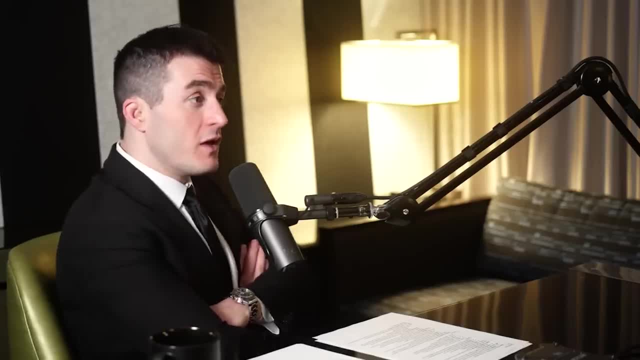 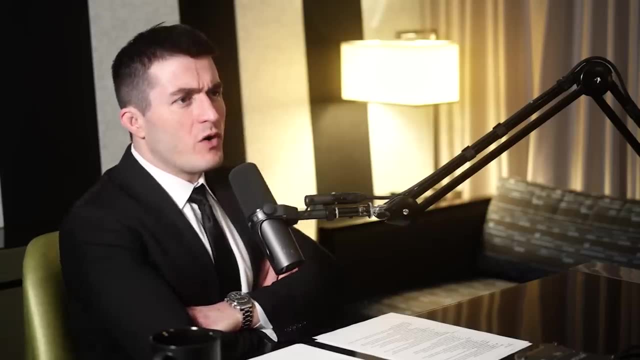 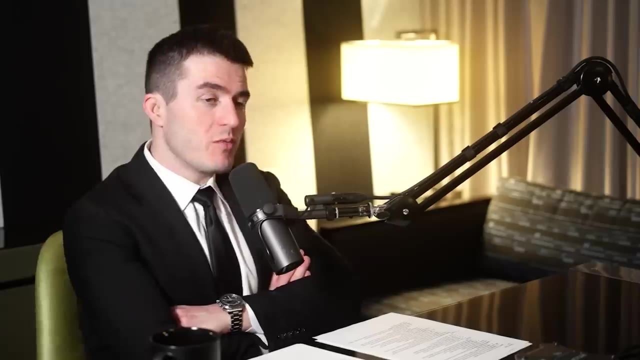 to add to that robot. oh, interesting, and so the, the arm is for sale. oh yeah, oh yeah, it's an option. what's the? what's the interface? like to work with the arm? like, is it pretty? so are they designed primarily, i guess, just ask that question in general about robots from boston dynamics. is it designed to be easily? 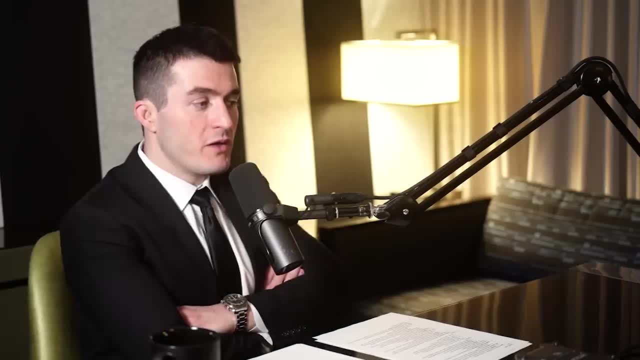 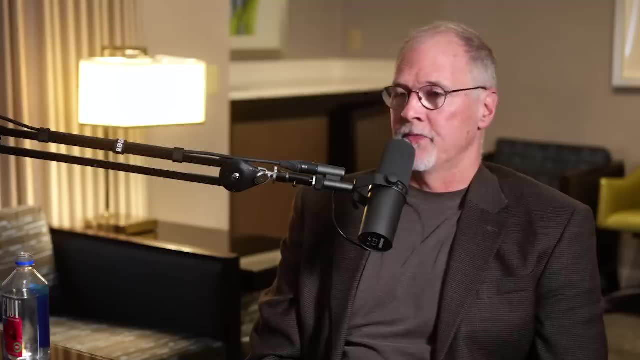 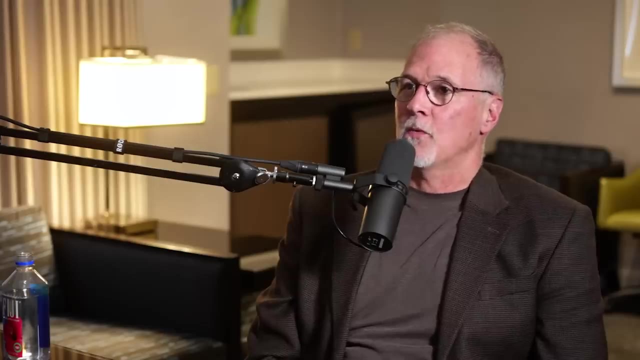 and efficiently operated remotely by a human being, or is there also the capability to push towards autonomy? we want both uh. in the next version of the software that we release, uh, which will be version 3.3, we're going to offer the ability of if you have an autonomous mission for the robot. 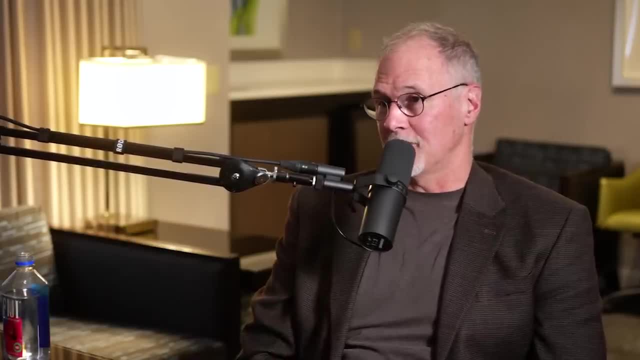 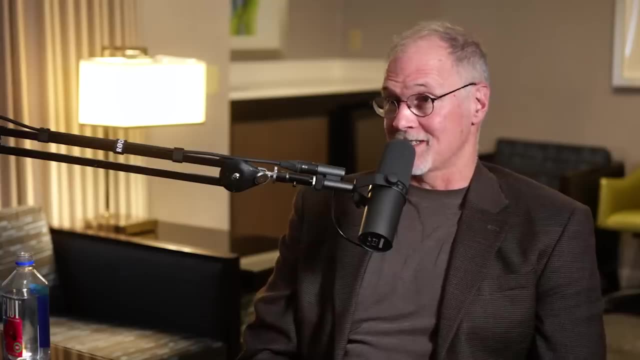 we're going to include the option that it can go through a door, which means it's going to have to have an arm and it's going to have to use that arm to open the door, and so that'll be an autonomous manipulation task that just you can program easily. uh, with the robot strictly through, you know we. 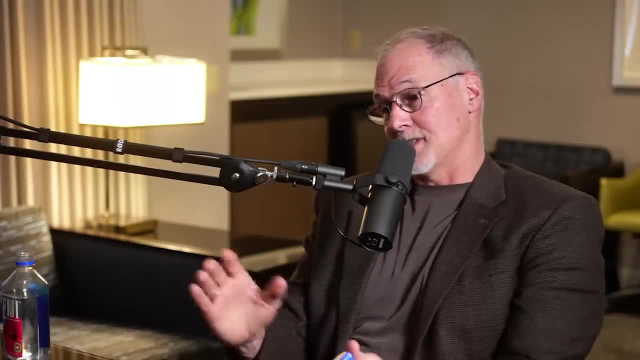 have a tablet interface and we're going to have to use that arm to open the door and so that'll be an autonomous manipulation task and so on the tablet, you know you sort of see the, the view that spot sees. you say there's the door handle. you know the hinges are on the left and it opens in. 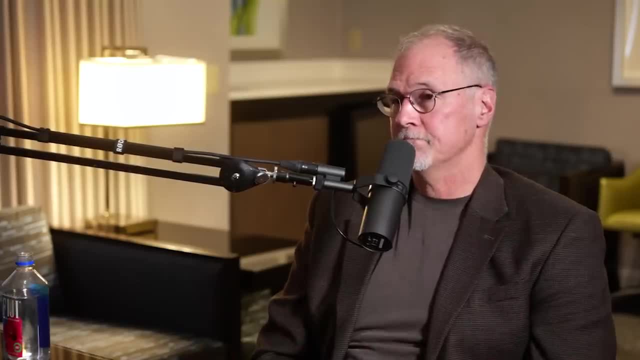 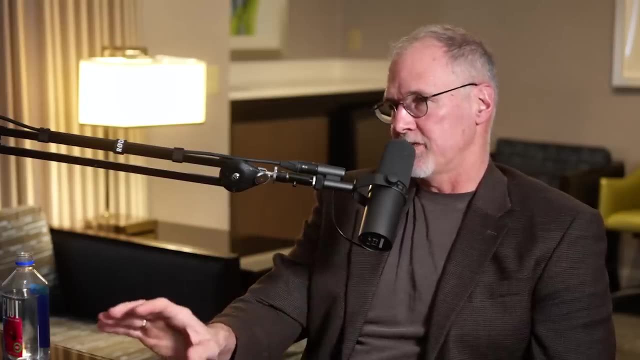 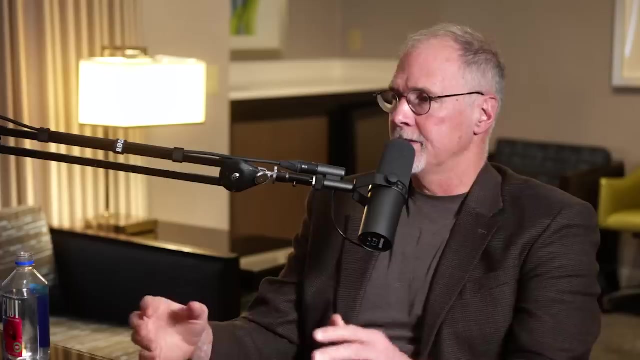 the rest is up to you take care of it. so it just takes care of everything. yeah, so we, we want, and for a task like opening doors, you can automate most of that, and we've automated a few other tasks. uh, we had a customer who had a, um, a high powered breaker switch. essentially it's an electric. 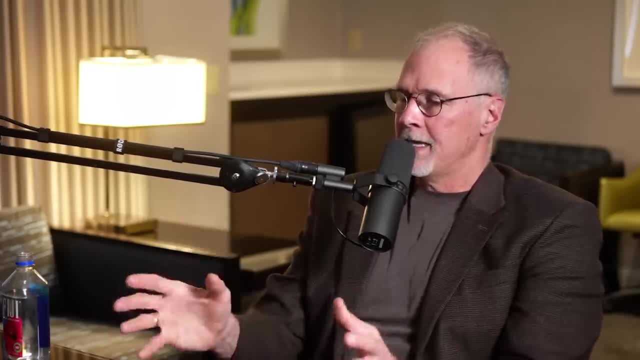 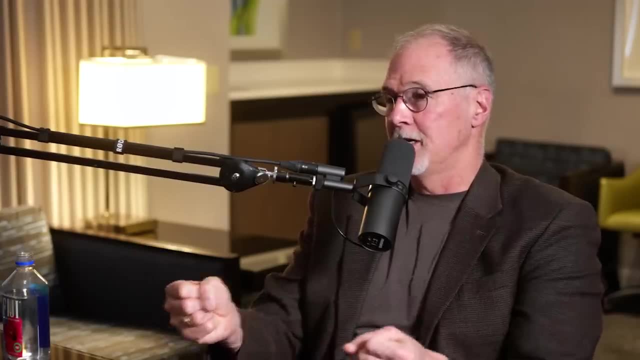 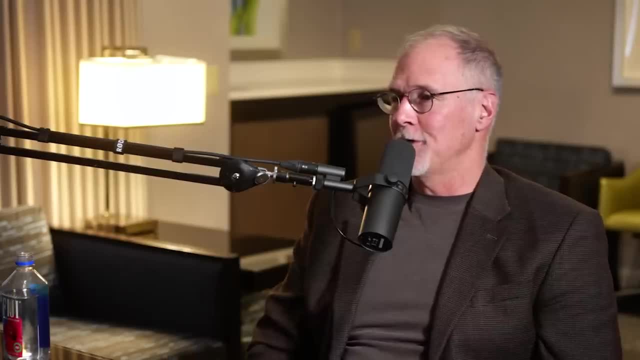 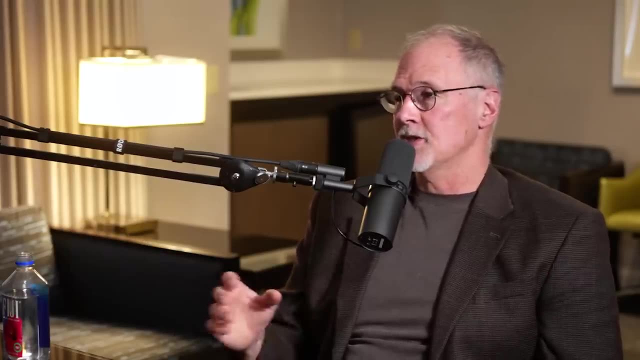 disconnect this breaker switch. well, as you can imagine, there's, you know, hundreds or thousands of amps and volts involved in this breaker switch and it's a dangerous event because occasionally you'll get what's called an arc flash. as you just do this, disconnect the power, the sparks jump. 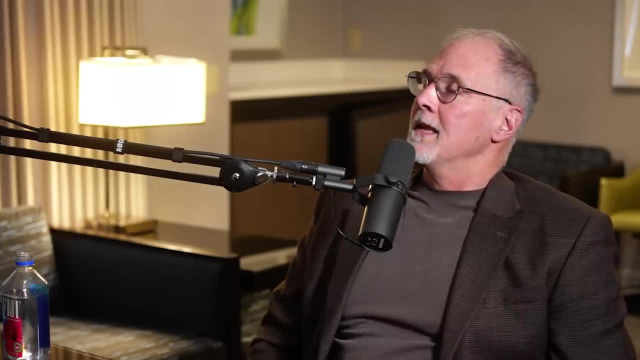 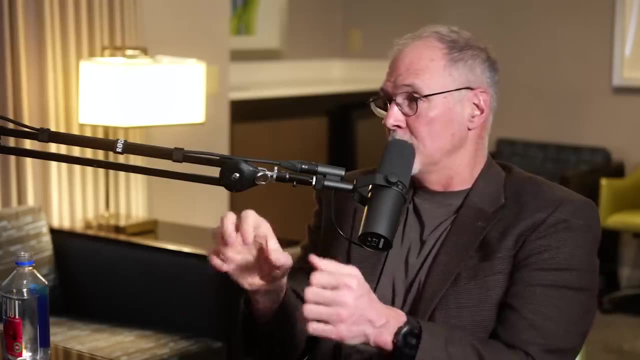 across and people die and they're going to have to do something about it and they're going to have to be doing this, and so, uh, ontario power generation used our spot and and the arm through the interface to to operate this, this disconnect- um, that's right- in an interactive way, and they 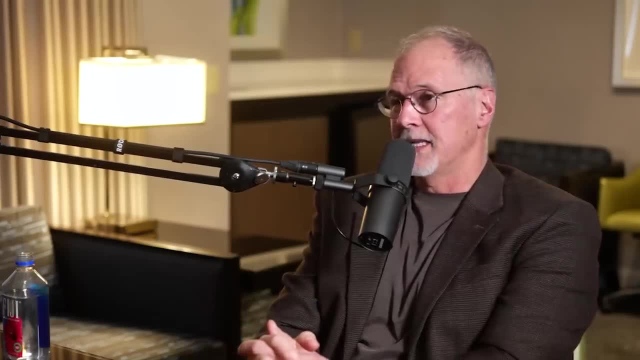 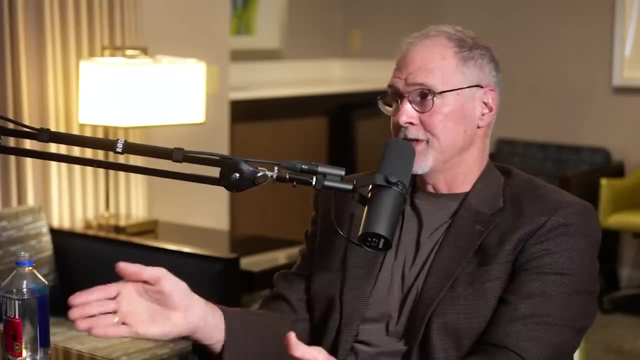 showed it to us and we were so excited about it and said: you know, i bet we can automate that task. and so we we got some examples of that breaker switch and i believe in the next generation of software. now we're going to deliver back to ontario power generation. 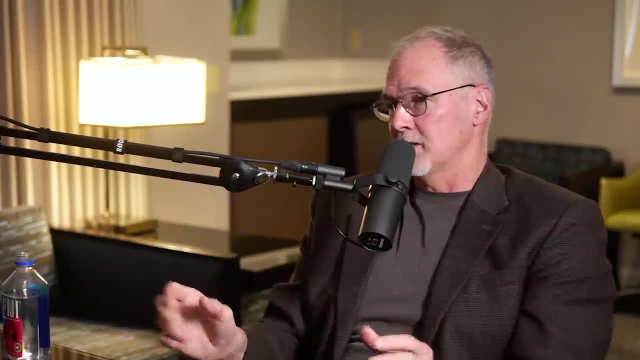 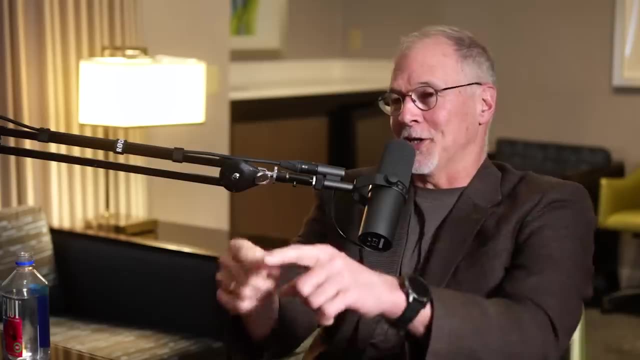 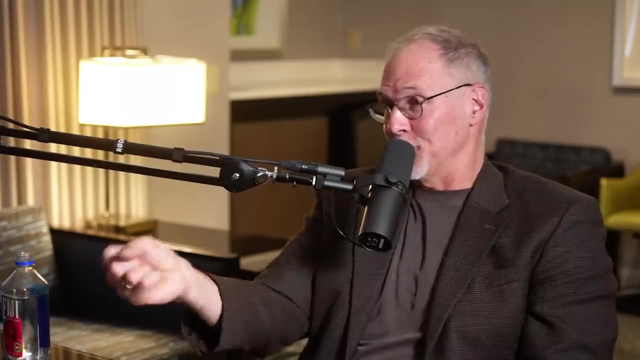 they're going to be able to just point the robot at that breaker. they'll be. they'll indicate that's the switch. there's sort of two actions you have to do. you have to flip up this little cover, press a button, then get a ratchet, stick it into a socket and literally unscrew this giant breaker. 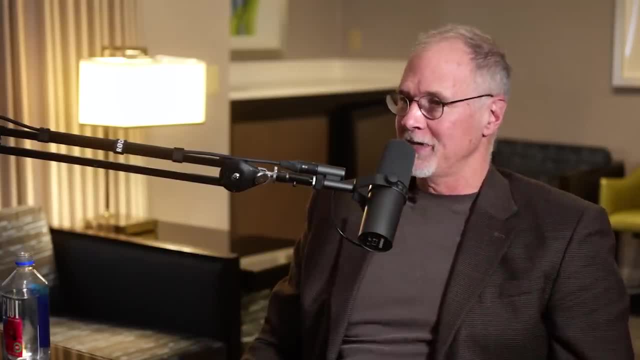 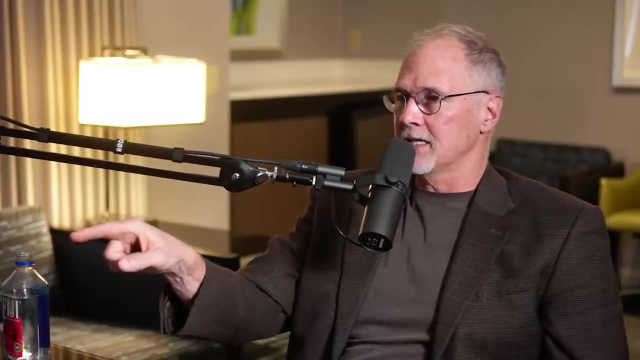 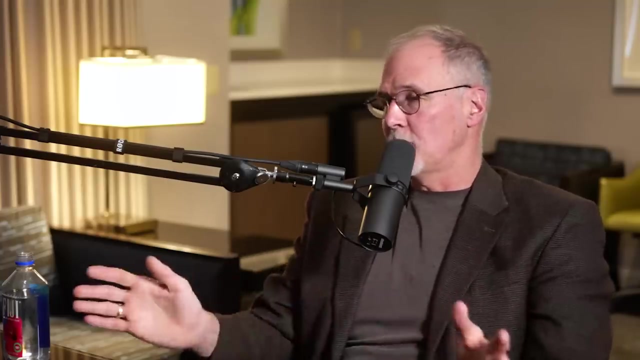 switch. so there's a bunch of different tasks and we basically automated them so that the human says you're going to put your tool and you're going to open it up, and so you can remotely sort of indicate this on the tablet, and then the robot just does everything in between and it does. 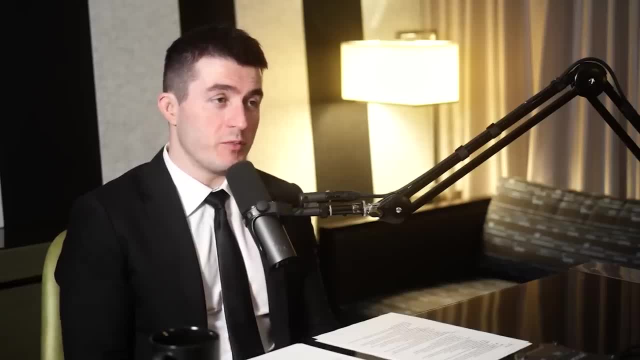 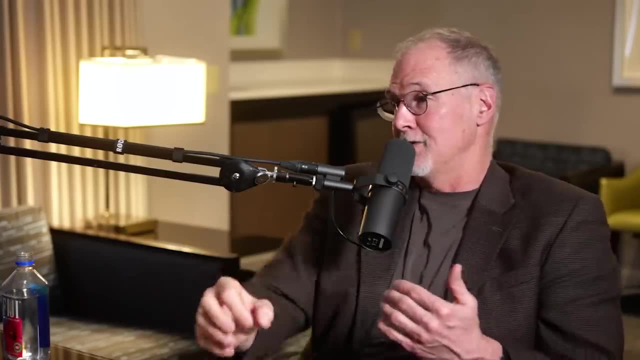 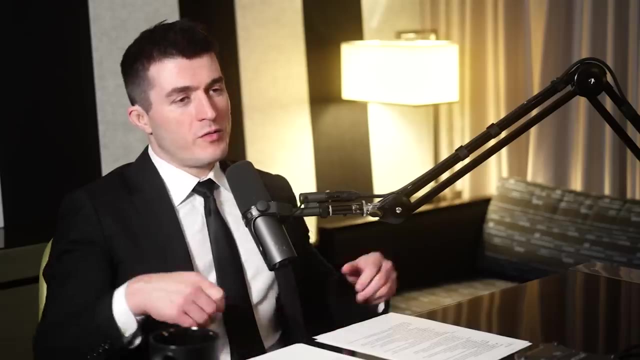 everything, all the coordinated movement of all the different actuators, that includes the body maintains its balance, it walks itself, you know, into position, so it's within reach, and the arm is in a position where it can do the whole task, so it manages the whole body. so how does one become? 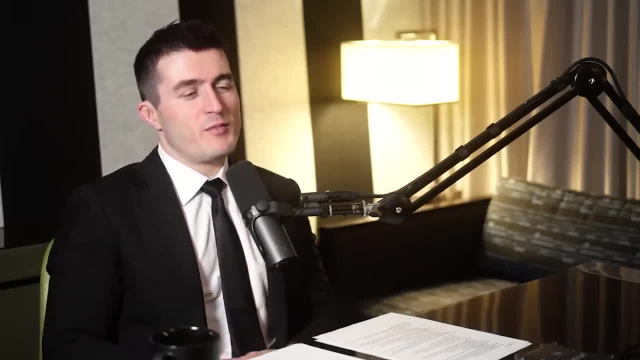 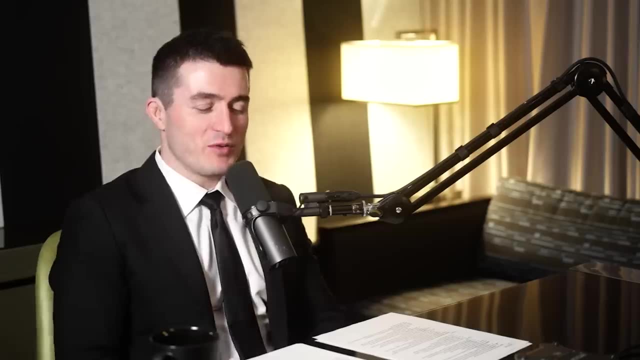 a big enough customer to request features, because i personally want a robot that gets me a beer. i mean that has to be like one of the most requests. i suppose in the industrial setting that's a non-alcoholic beverage of picking up objects and bringing the objects to you. we love working with customers who have 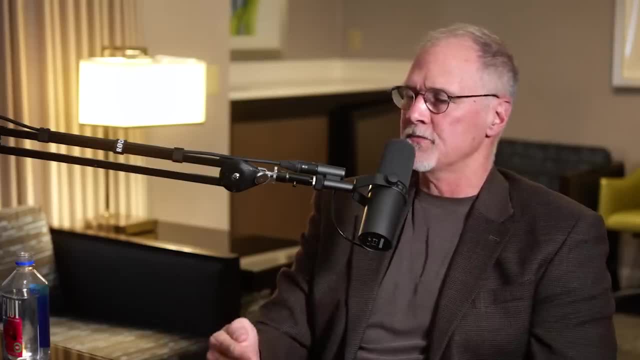 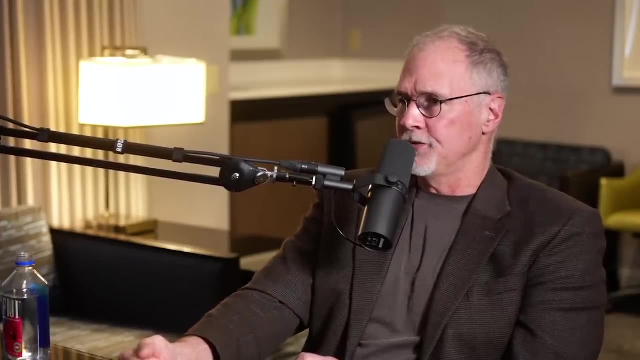 challenging problems like this and and this one in particular, because we felt like what they were doing. a- it was a safety feature. b- we saw that the robot could do it because they they tele-operated it the first time. probably took them an hour to do it the first time. 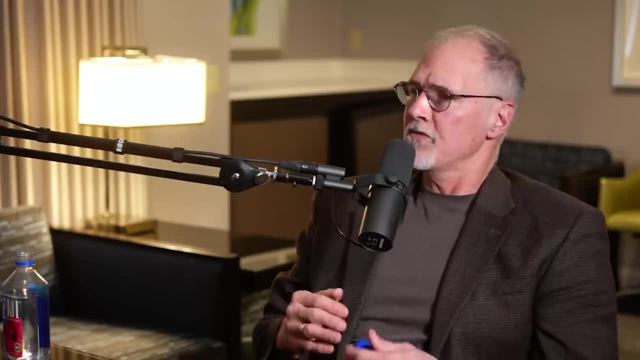 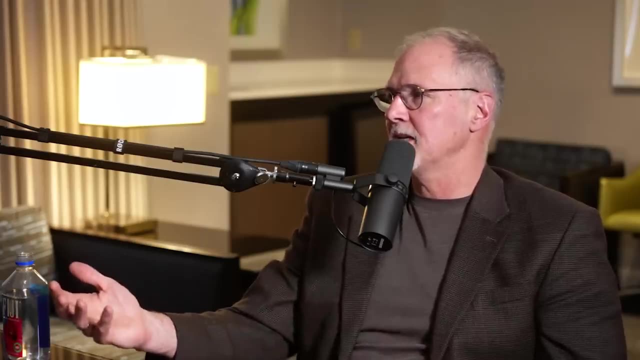 right. but the robot was clearly capable and we thought, oh, this is a great problem for us to work on, to figure out how to automate a manipulation task. and so we took it on, not not because we were going to make a bunch of money from it in selling the robot back to them, but because it motivated us. 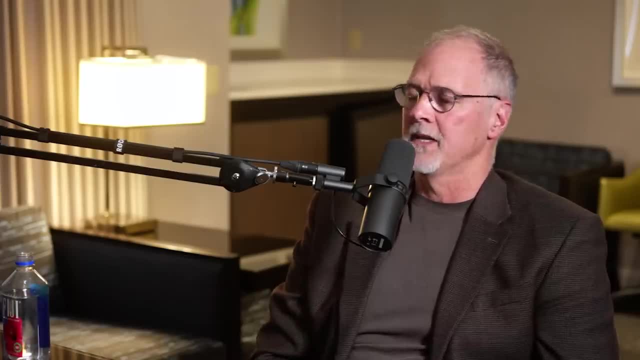 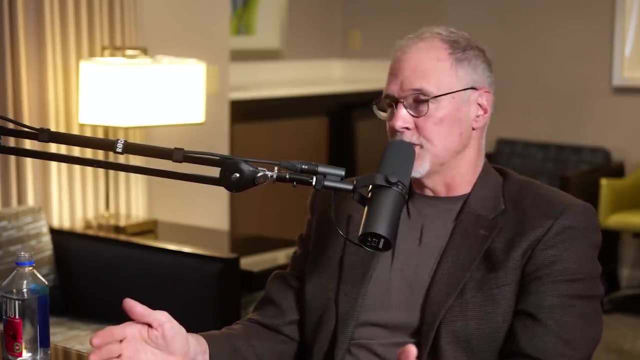 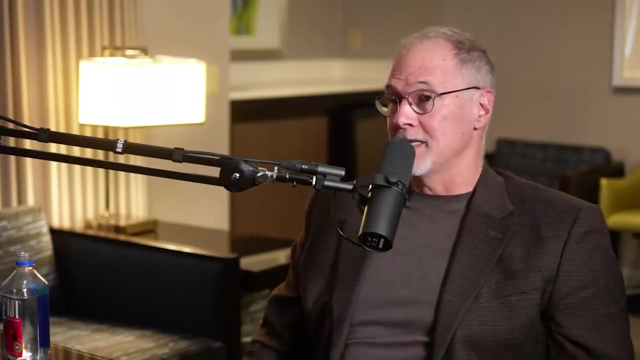 to go solve what we saw as the next logical step. but many of our customers, in fact, uh, we, we try to our bigger customers, typically ones who are going to run a utility or a factory or something like that. we take that kind of direction from them and if they're, especially if they're going to buy 10 or 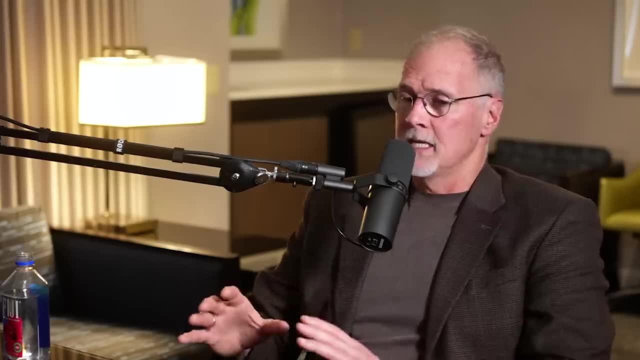 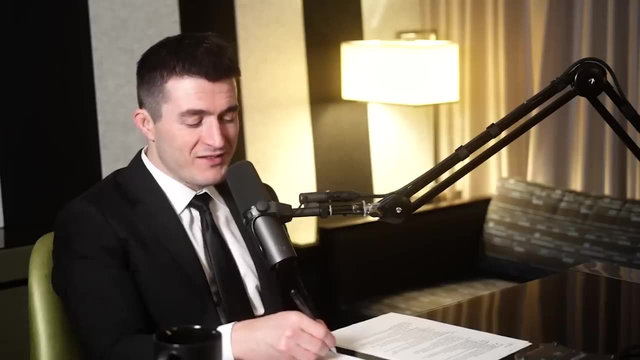 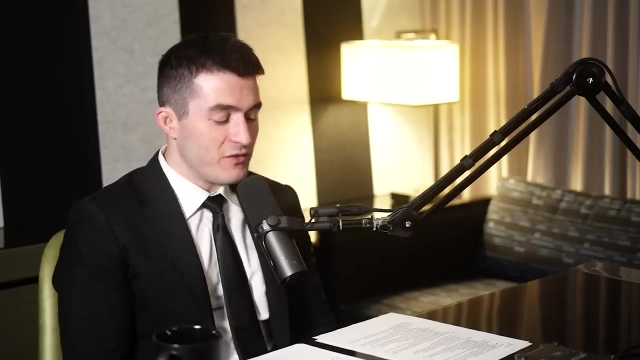 20 or 30 robots and they say: i really need it to do this. well, that's exactly the right kind of problem that we want to be working on. yeah, and so, note to self, buy 10 spots and aggressively push for beer manipulation. i think it's fair to say it's notoriously difficult to make a lot of money. 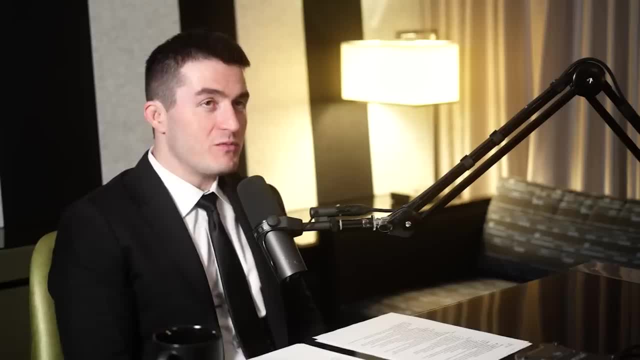 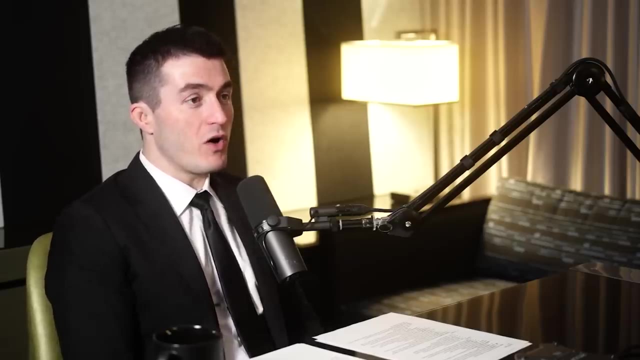 as a robotics company. uh, how can you make money as a robotics company? can you speak to that? it seems that a lot of robotics companies fail. it's difficult to build robots. it's difficult to build robots at a low enough cost where customers, even the industrial setting, want to purchase them, and it's difficult to build robots that 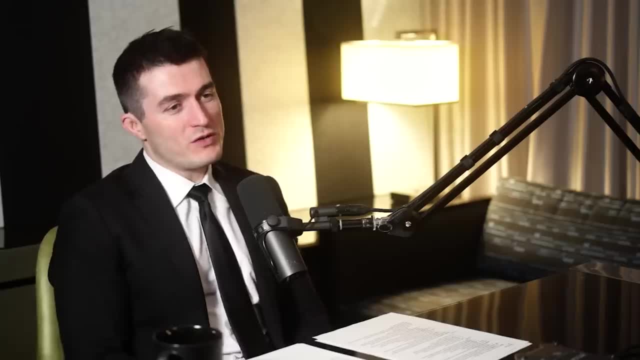 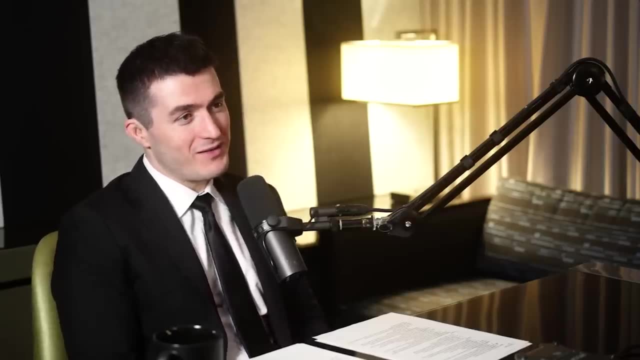 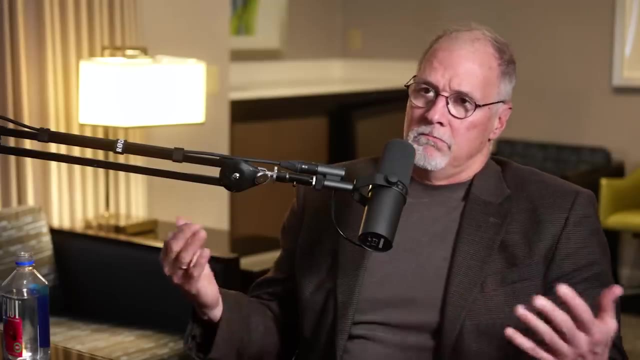 are useful, sufficiently useful. so what can you speak to? and boston dynamics has been been uh successful for many years of finding a way to make money well in the early days. of course you know the money we made was from doing contract r&d work and we made money, but you know we weren't. 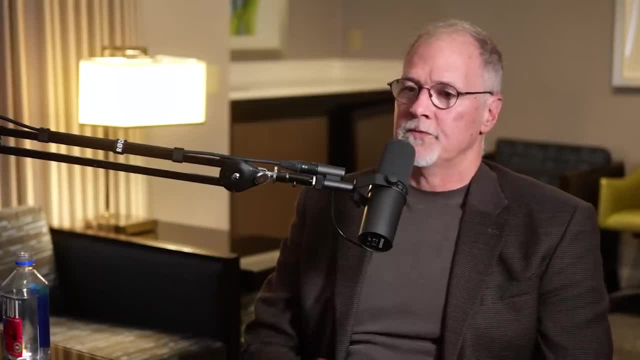 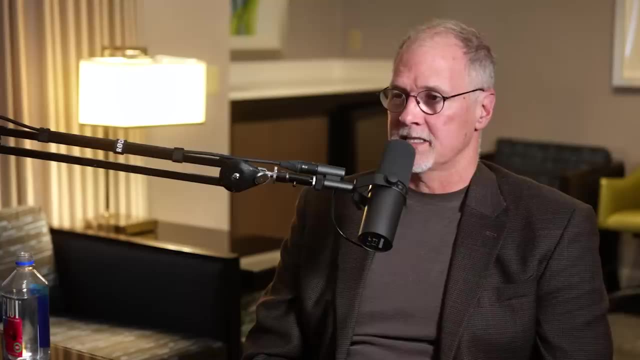 growing and we weren't selling a product. and then we went through several owners who, you know, had a vision of not only developing advanced technology but eventually developing products, and so both- you know- google and softbank, and now hyundai, you know- had that vision and were willing to. 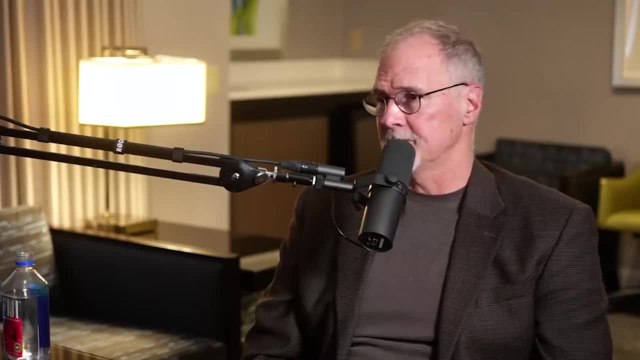 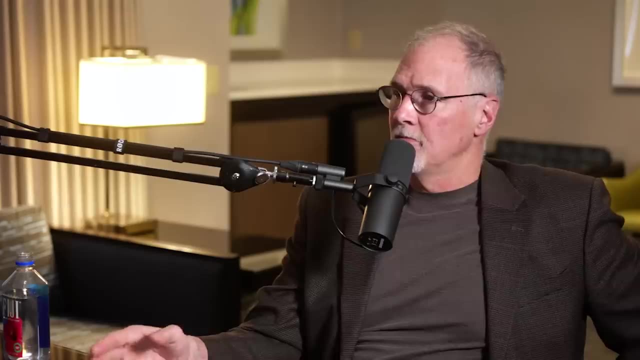 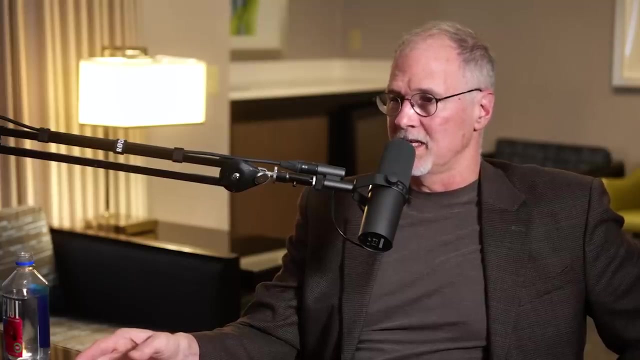 you know, provide, uh, that investment. um, now, our discipline is that we need to go find applications that are broad enough that you could imagine selling thousands of robots, because it doesn't work if you don't sell thousands or tens of thousands of robots, if you only sell hundreds. 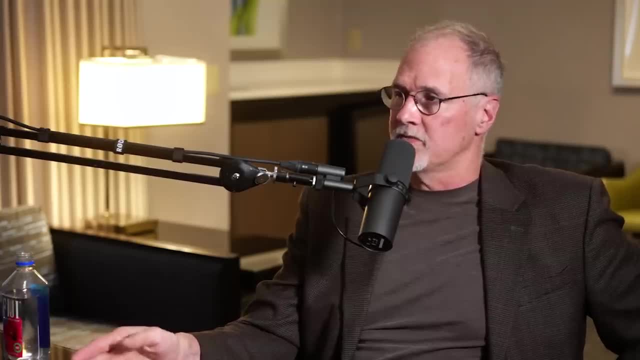 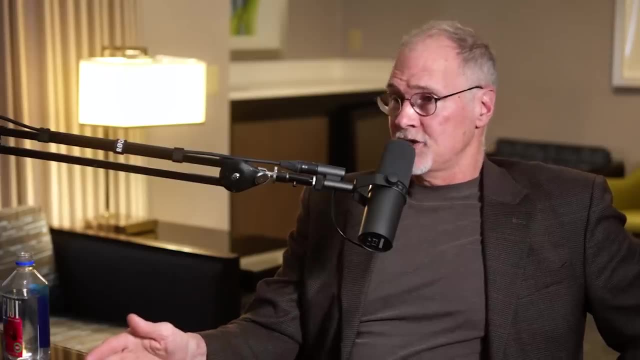 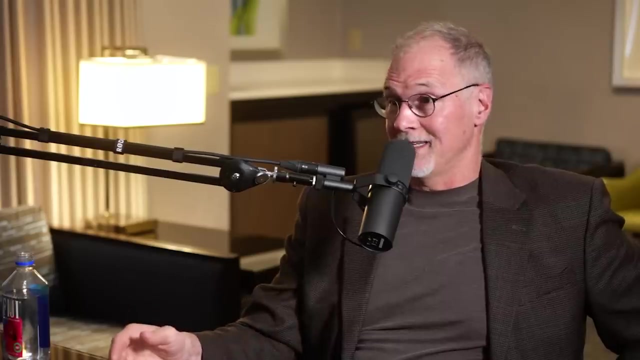 the, you will commercially fail, and that's where most of the small robot companies have died. um, and- and that's a challenge, because you know a, you need to field the robots. they need to start to become reliable and, as we've, as we've said, that takes time and investment to get there. 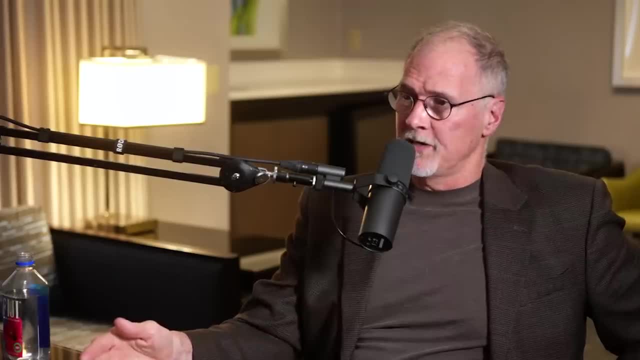 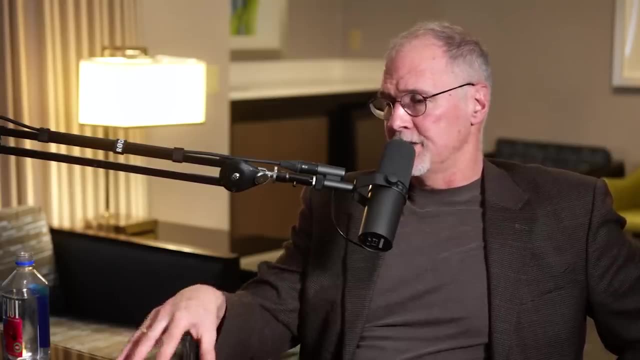 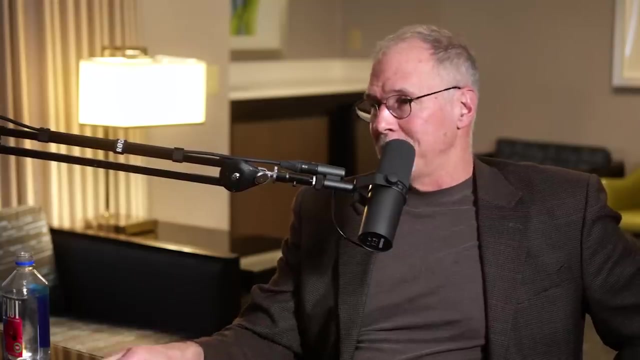 and so it really does take visionary investment to get there. but we, we believe that we are going to make money in this uh industrial monitoring space because you know if a, if a chip fab, if the line goes down because a vacuum pump failed, someplace that can be in a. 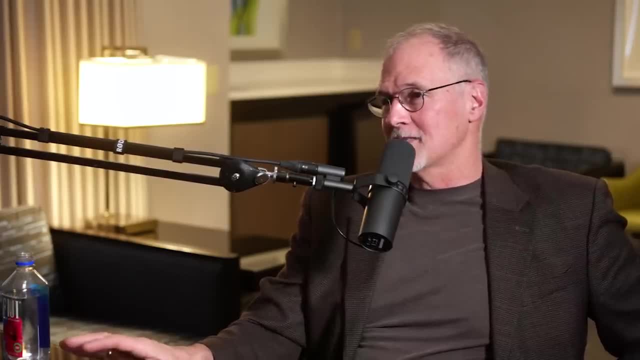 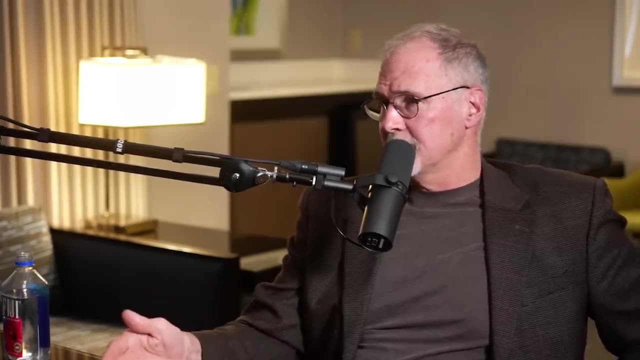 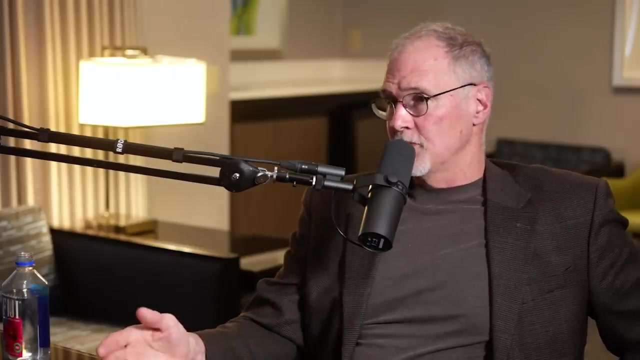 very expensive process. it can be a million dollars a day in lost production. maybe you have to throw away some of the product along the way, and so the robot, if you can prevent that by inspecting the factory every single day, maybe every hour if you have to. there's a real return on investment. 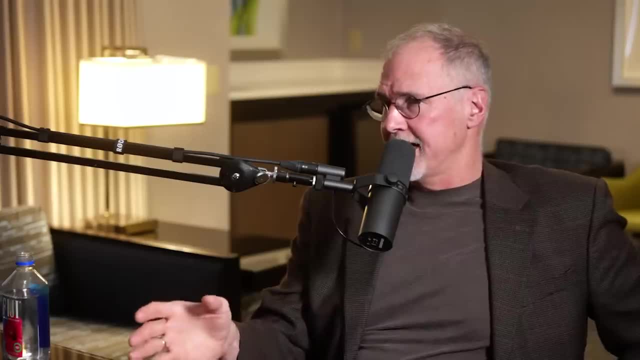 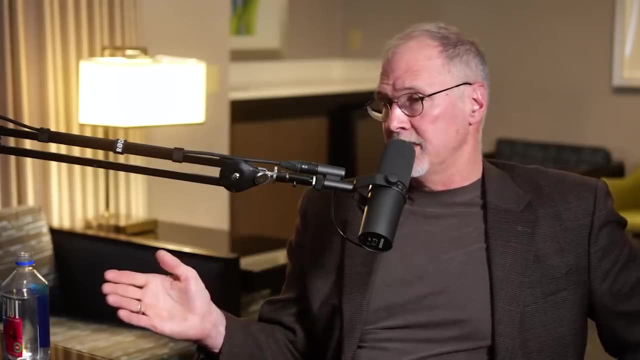 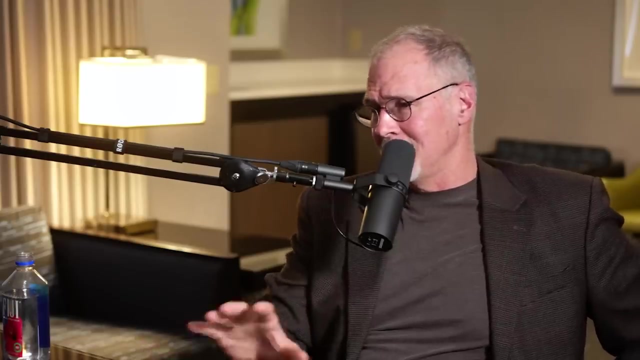 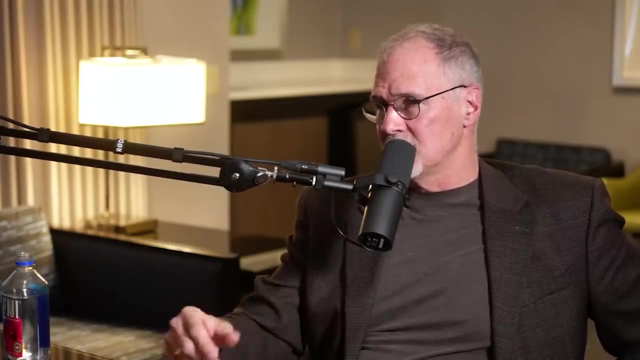 there, but there needs to be a critical mass of this task, and and we're focusing on a few that we believe are ubiquitous in the industrial production environment, and that's using a thermal camera to keep things from overheating, using an acoustic imager to find compressed air leaks, using visual cameras to read gauges measuring vibration. these are standard. 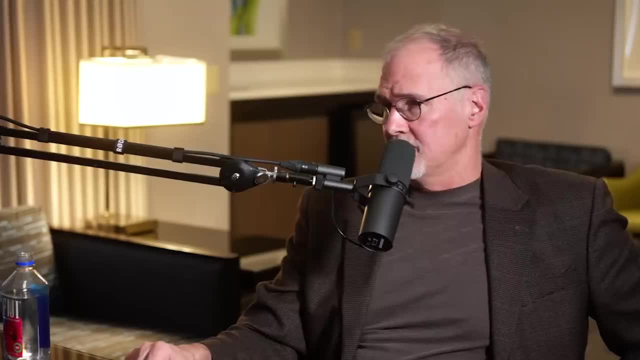 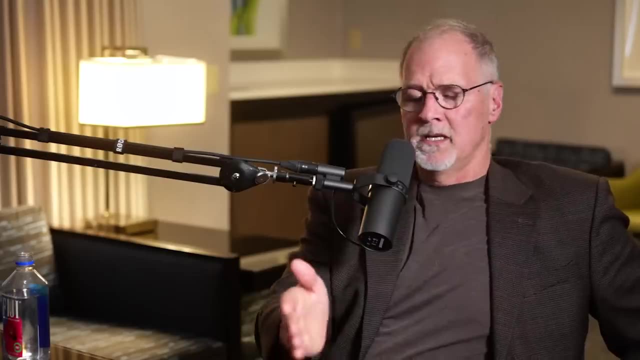 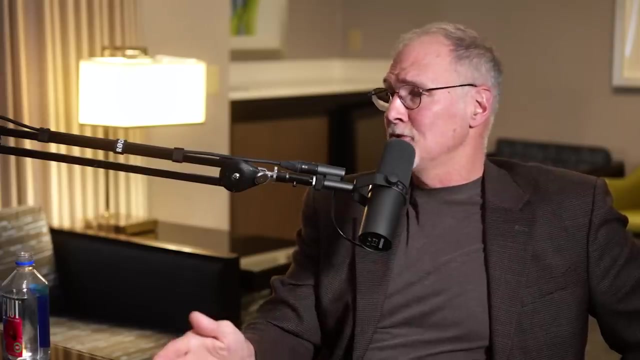 things that you do to prevent unintended shutdown of a factory, and this. this takes place in a beer factory. we're working with a b in dev. it takes place in chip fabs- you know we're working with global foundries. it takes place in electric utilities and nuclear power plants, and 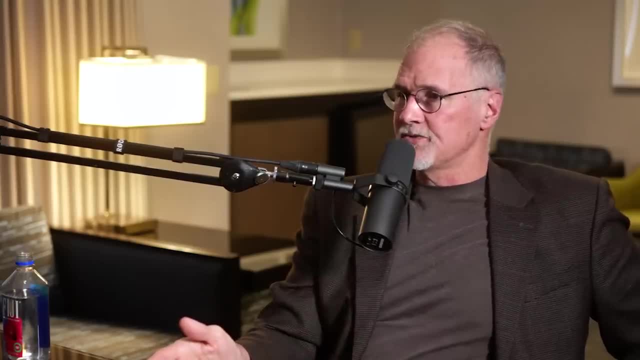 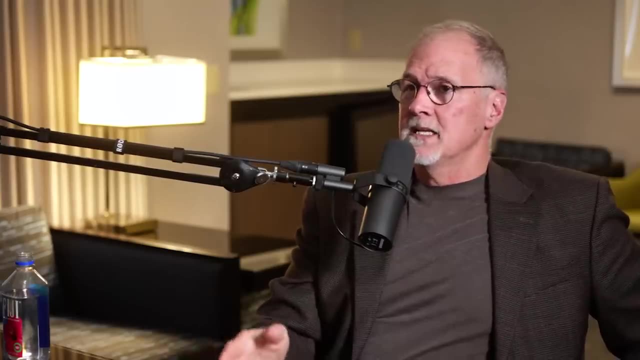 so the same robot can be applied in all of these industries and, and, as i said, we have about- actually it's 1100 spots out now to really get- uh, you know- profitability, we need to be at a thousand a year, maybe, maybe fifteen hundred a year, you know, for that space. and so we're working with a lot of the 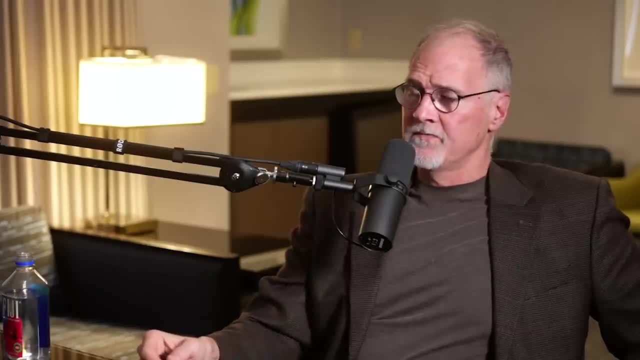 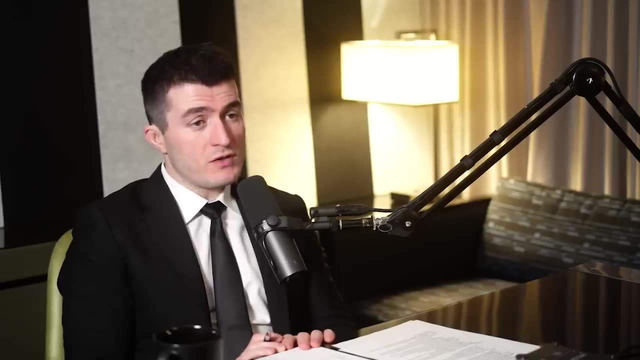 sort of part of the business. so it still needs to grow, um, but, but we're on a good path so i think that's totally achievable. so the application should require the crossing that thousand robot barrier. it really should. yeah, i want to mention, you know, our second robot, uh, stretch, yeah tell. 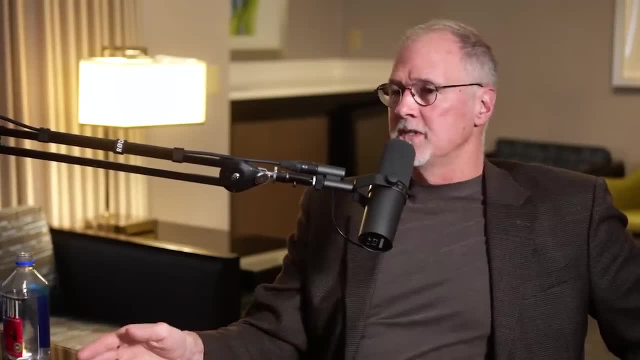 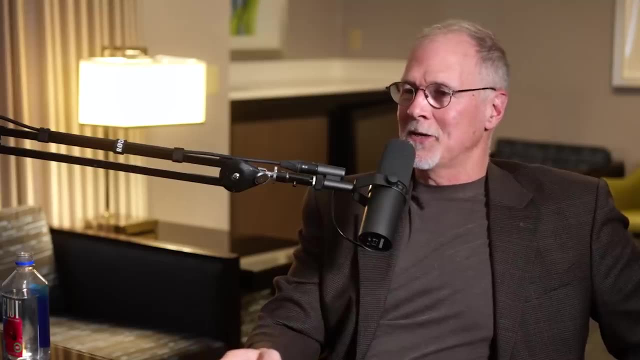 me about stretch. what's stretch? whose stretch stretch started differently than spot? you know, spot we built because we had decades of experience building quadrupeds. we just we had it in our blood- Quadruped product. but we had to go figure out what the application was And we actually discovered. 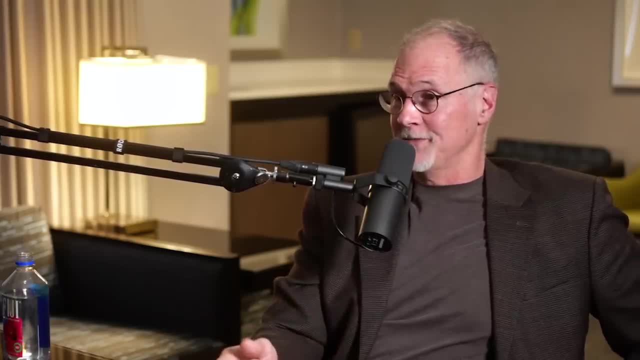 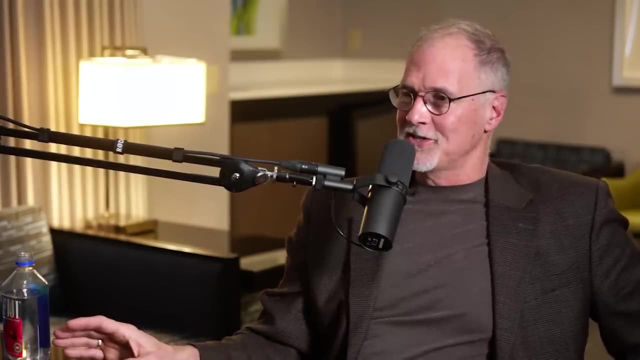 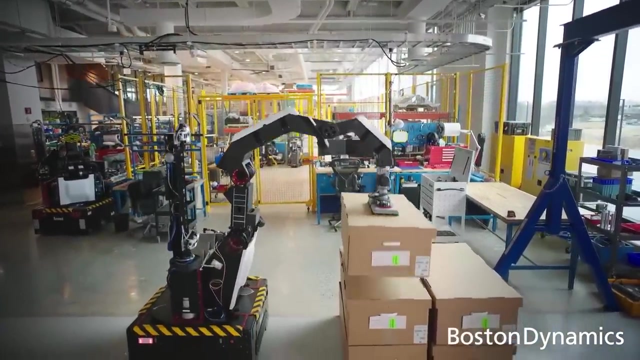 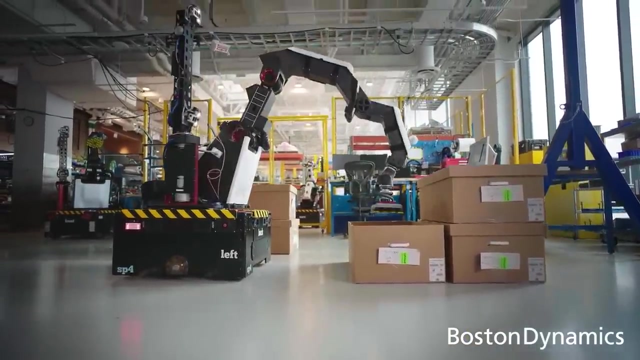 this factory patrol application, basically preventative maintenance, by seeing what our customers did with it. Stretch is very different. We started knowing that there was warehouses all over the world. There's shipping containers moving all around the world full of boxes that are mostly being moved by hand. By some estimates we think there's a trillion boxes. 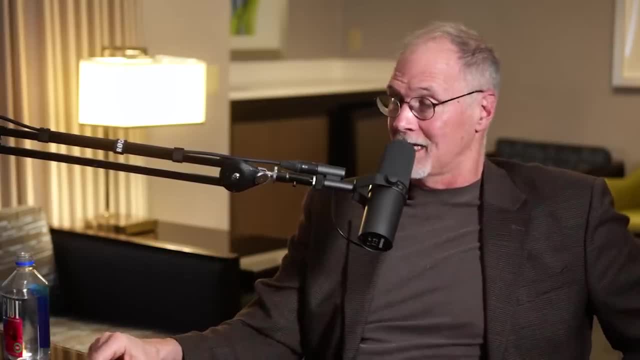 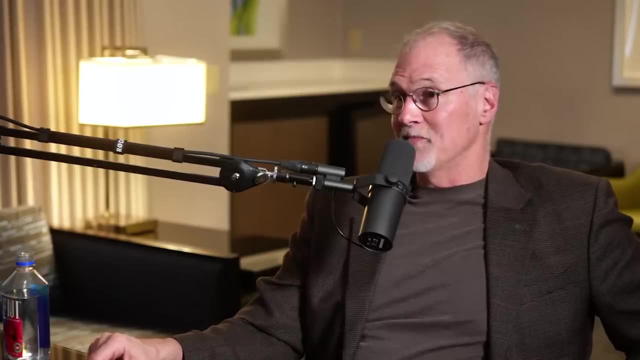 cardboard boxes shipped around the world each year and a lot of it's done manually. It became clear early on that there was an opportunity for a mobile robot in here to move boxes around, And the commercial experience has been very different between Stretch and with Spot. 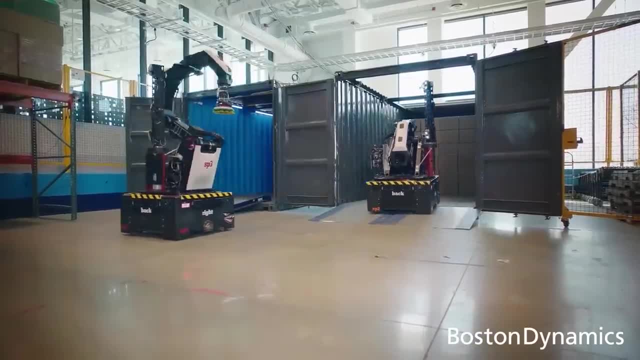 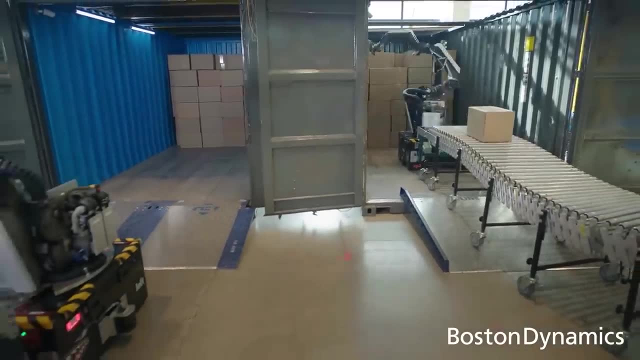 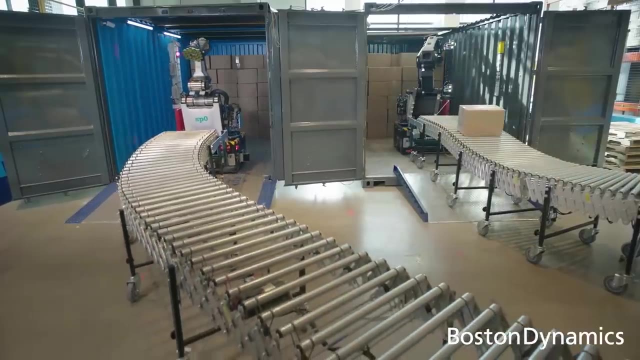 As soon as we started talking to people- potential customers- about what Stretch was going to be used for, they immediately started saying, oh, I'll buy that robot. In fact, I'm going to put in an order for 20.. Right now, we just started shipping the robot in January after several years of development. 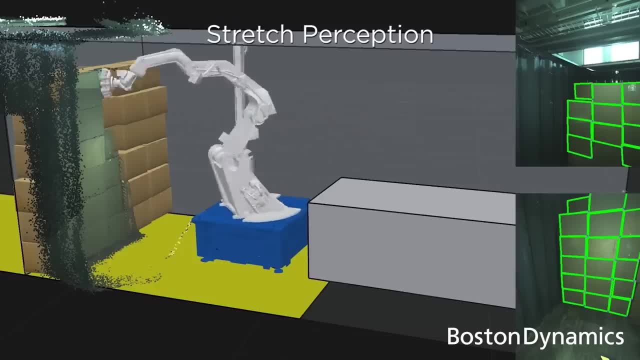 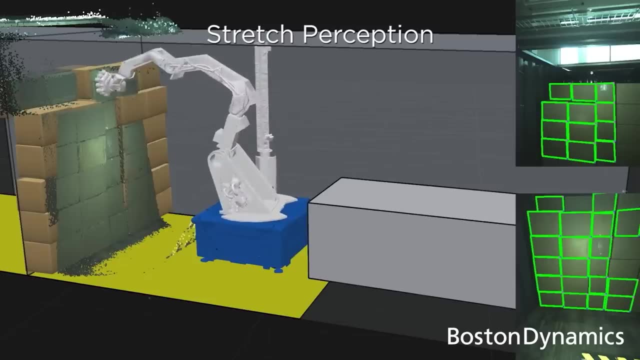 Of this year, Of this year. So our first deliveries of Stretch to customers were DHL and Maersk in January. We're delivering to Gap right now And we have about seven or eight other customers, all who've already agreed in advance to buy between 10 and 20 robots, And so we've already. 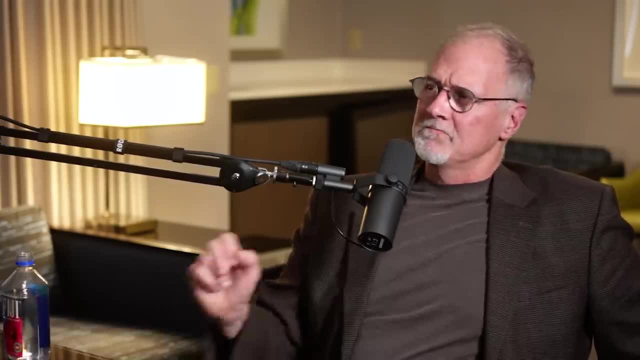 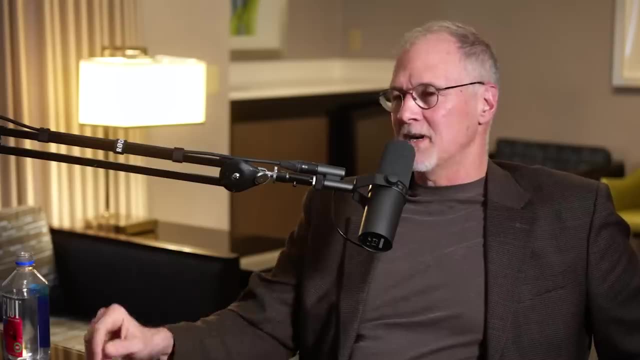 got commitments for a couple hundred of these robots. This one's going to go right. It's so obvious that there's There's a need, And we're not just going to unload trucks, We're going to do any box-moving task in the warehouse, And so it too will be a multi-purpose robot, And we'll eventually have 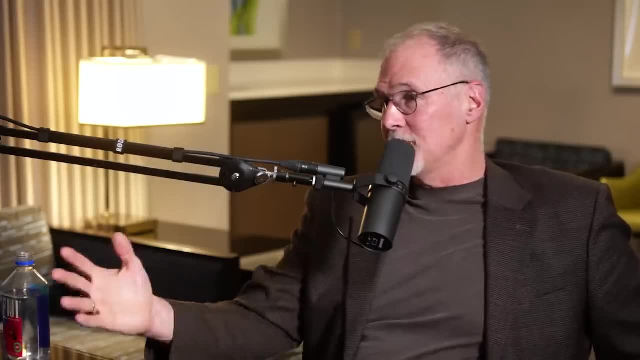 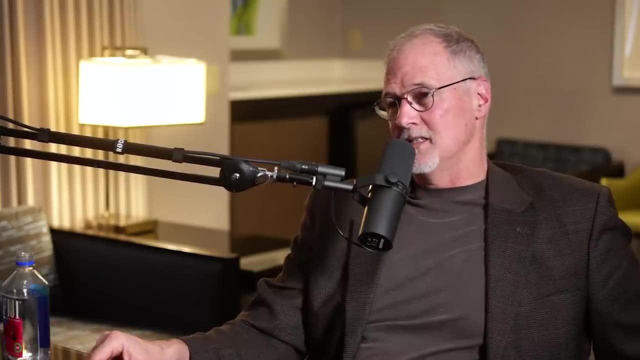 it doing palletizing or depalletizing or loading trucks or unloading trucks. There's definitely thousands of robots. There's probably tens of thousands of robots of this in the future, So it's going to be profitable. Can you describe what Stretch looks like? 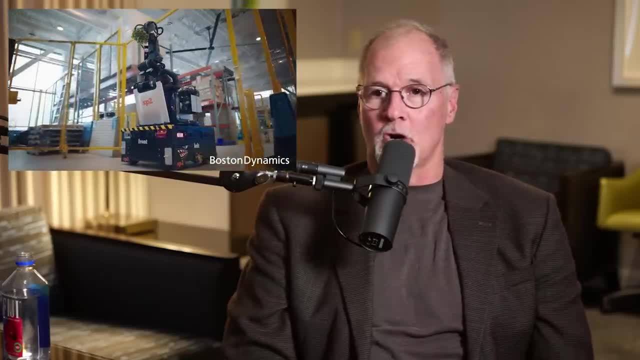 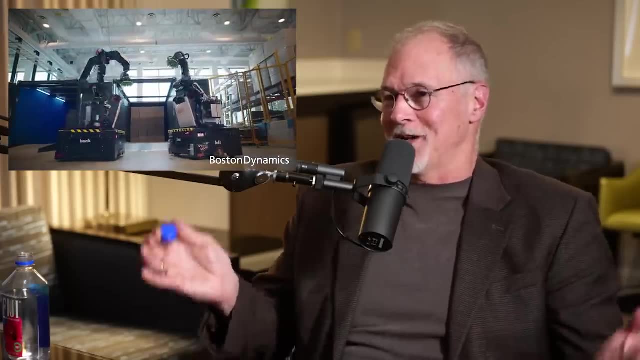 It looks like a big, strong robot arm on a mobile base. The base is about the size of a pallet, And we want it to be the size of a pallet because that's what lives in warehouses, right: Pallets of goods sitting everywhere. So it needed to be able to fit in. 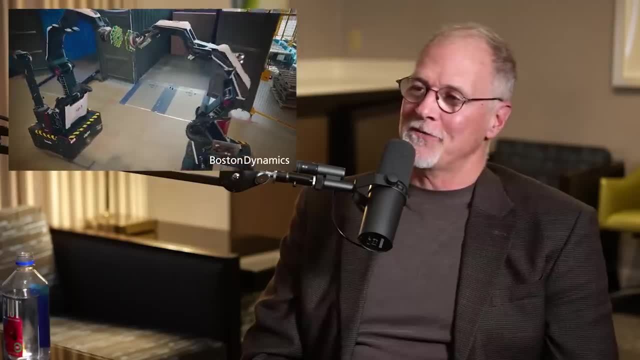 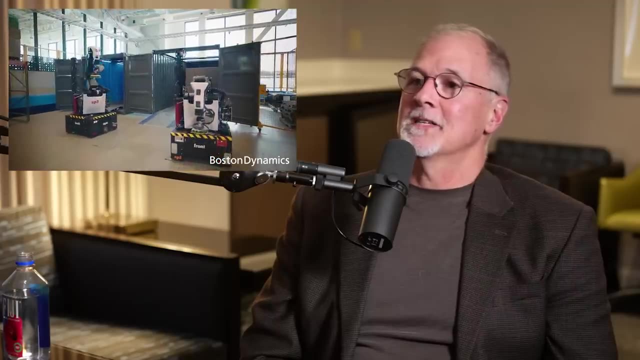 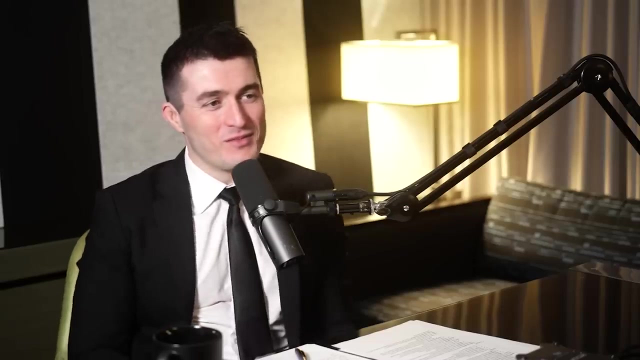 that space. It's not a legged robot. It's not a legged robot, And so it was our first. It was actually a bit of a commitment from us, a challenge for us to build a non-balancing robot, To do the much easier problem, But to do a well. 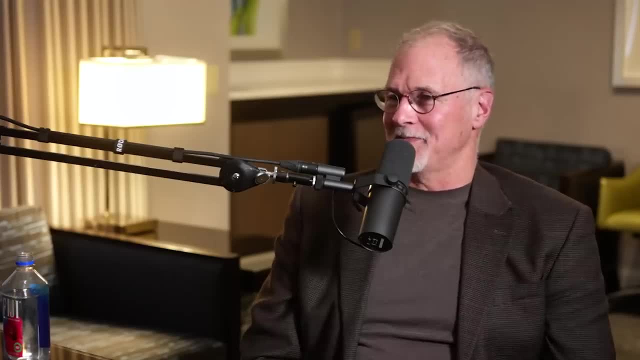 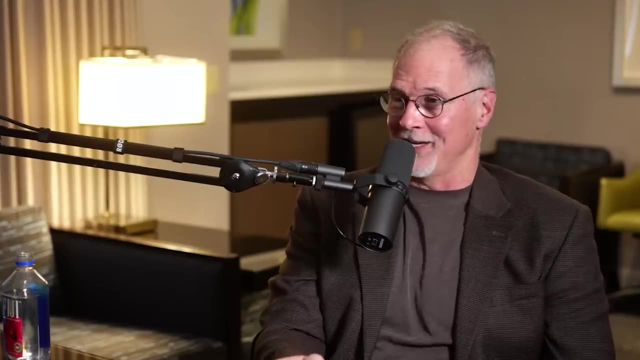 Because it wasn't. It wasn't going to have this balance problem And in fact, the very first version of the logistics robot we built was a balancing robot And that's called Handle. And there's, That thing was epic. Oh, it's a beautiful machine. 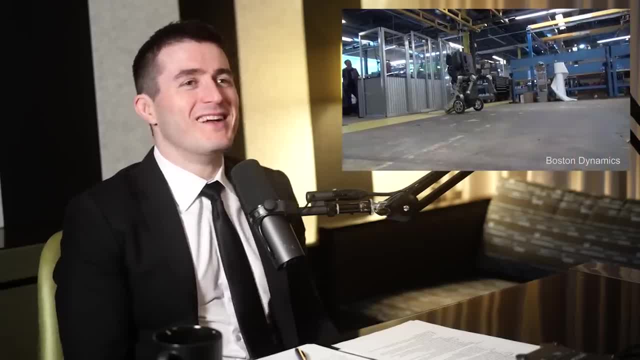 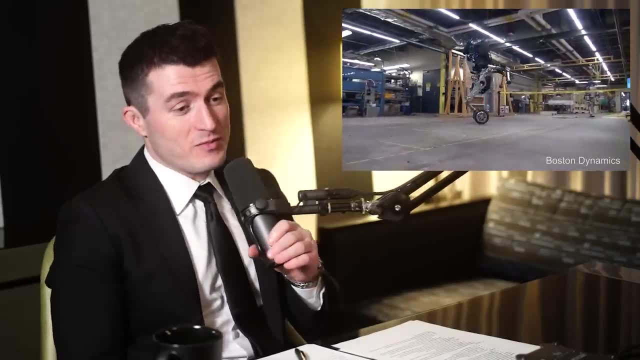 It's an incredible machine. So it was. I mean it looks epic, It looks like out of the sci-fi movie of some sort. I mean just, Can you actually just linger on the design of that thing, Because that's another leap into something you probably haven't. 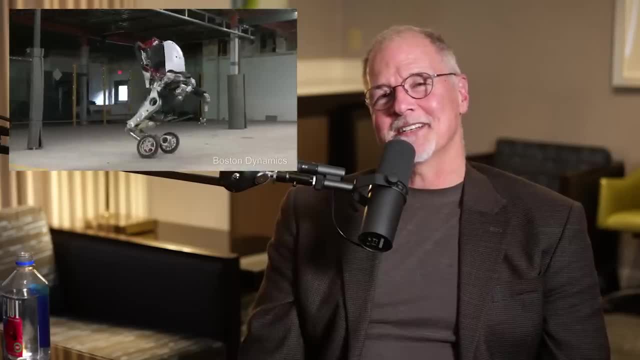 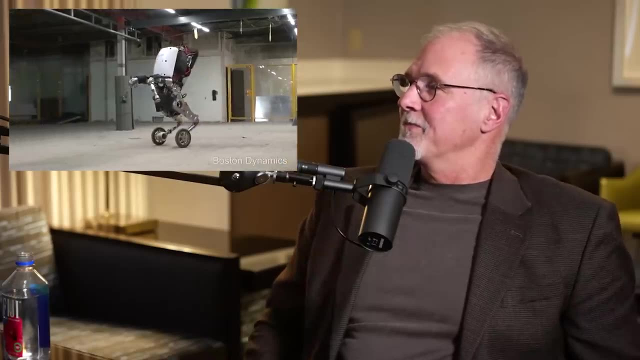 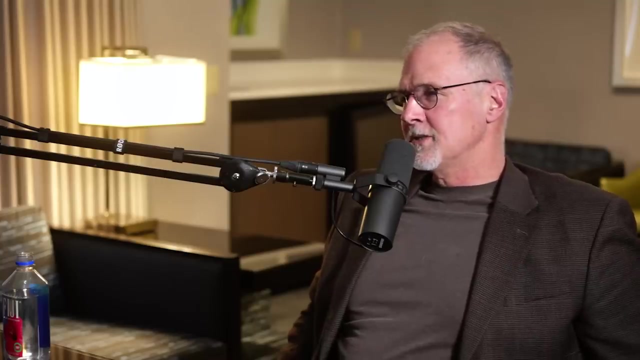 That's a different kind of balancing, Yeah, So let me. I love talking about the history of how Handle came about, Because it connects all of our robots actually. So I'm going to start with Atlas. When we had Atlas getting fairly far along, we wanted to understand. I was telling you earlier. 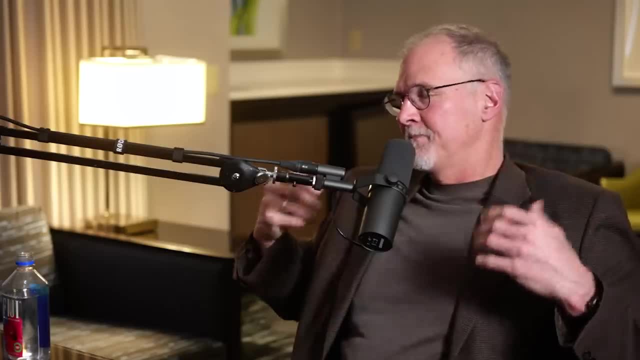 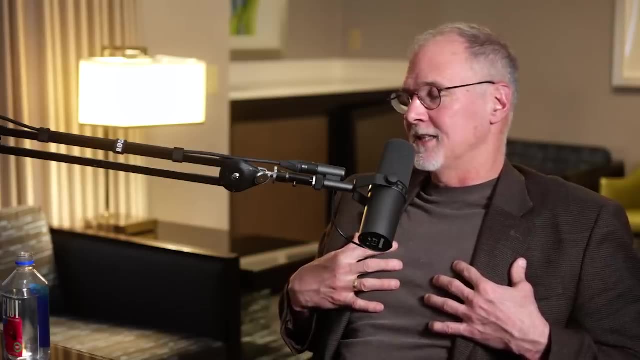 the challenge of the human form is that you have this mass up high, And balancing that inertia, that mass up high, is its own unique challenge. And so we started trying to get Atlas to balance, standing on one foot, like on a balance beam. 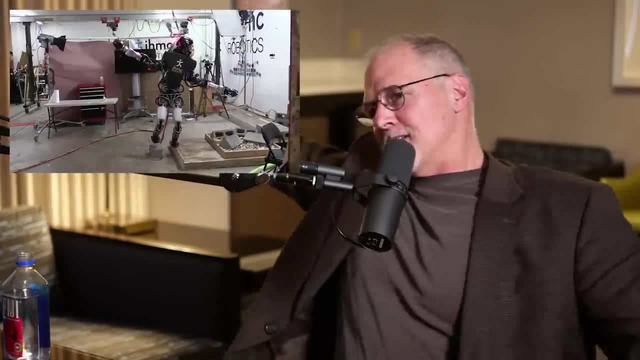 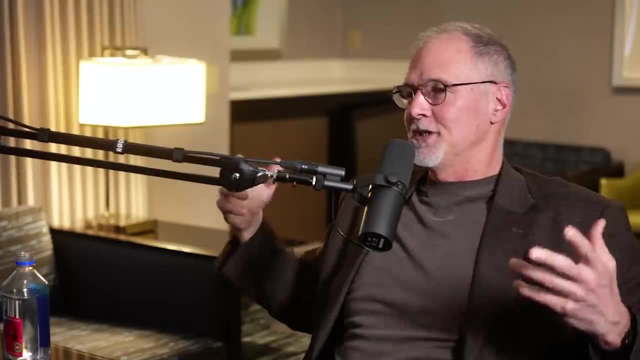 using its arms like this- And you can do this, I'm sure I can do this right- Like if you're walking a tightrope, How do you do that balance? So that's sort of controlling the inertia, controlling the momentum of the robot. We were starting to figure that out on Atlas. 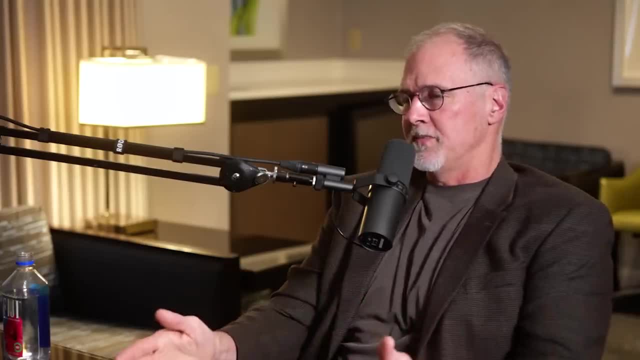 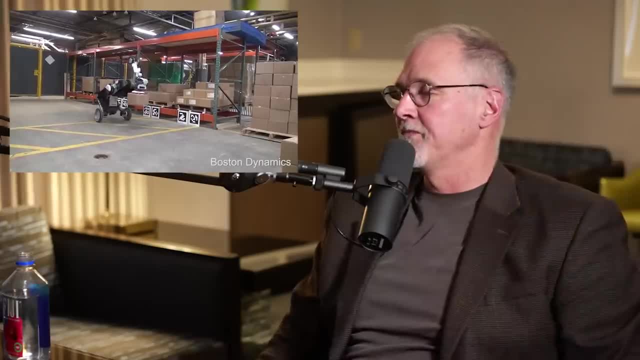 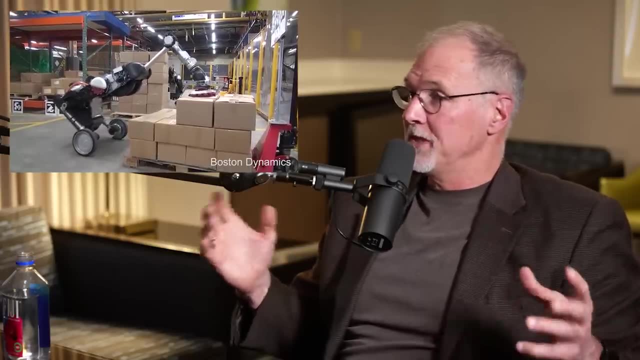 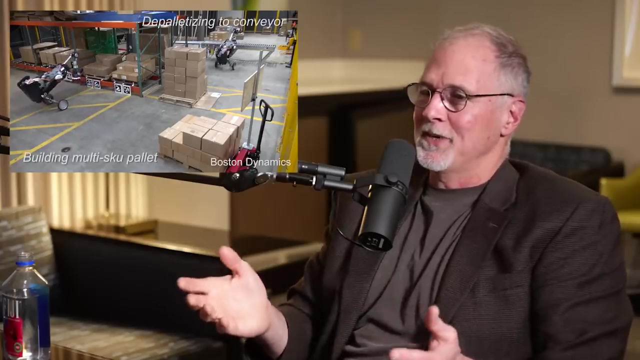 arm so it could reach a box at the top of a truck And it was going to. It needed yet another counterbalance, a big tail, to help it balance while it was using its arm. So the reason why this robot sort of looks epic- some people said it looked like an ostrich or maybe an ostrich. 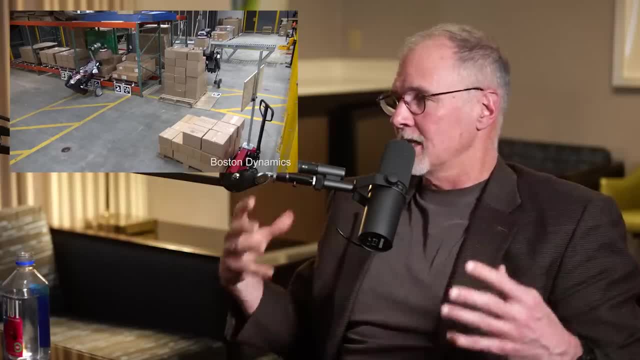 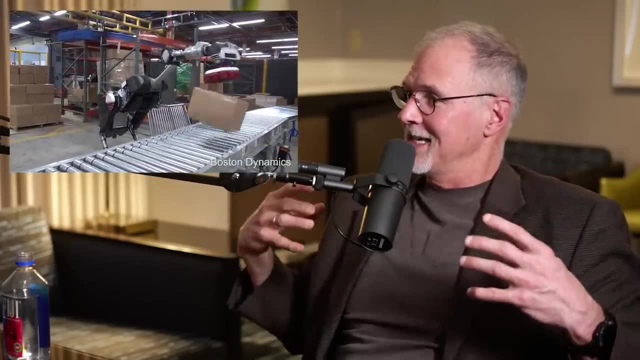 moving around was the wheels, the legs. It has legs so it can extend its legs, So it's wheels on legs. We always wanted to build wheels on legs. It had a tail and it had this arm And they're all moving simultaneously and in coordination to maintain balance. 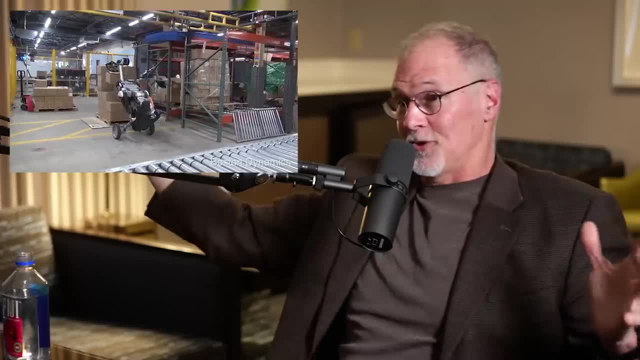 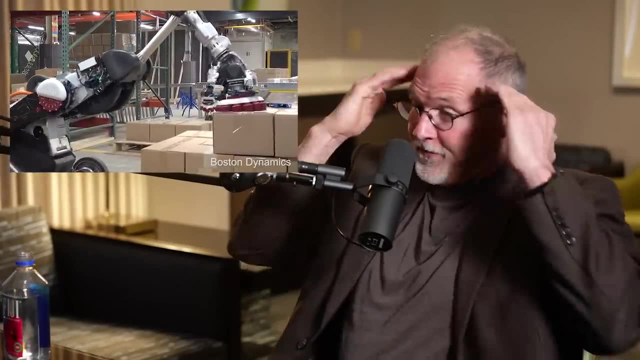 because we had figured out the mathematics of doing this momentum control, how to maintain that balance, And so part of the reason why we built this two-legged robot was we had figured this thing out, We wanted to see it in this kind of machine and we thought, maybe this kind of 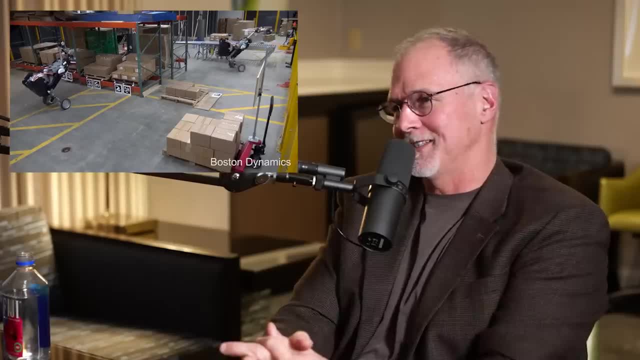 machine would be good in a warehouse, And so we built it. And it's a beautiful machine. It moves in a graceful way. It's a beautiful machine. It's a beautiful machine. It's a beautiful machine. It moves in a graceful way like nothing else we've built. But it wasn't the right machine for. 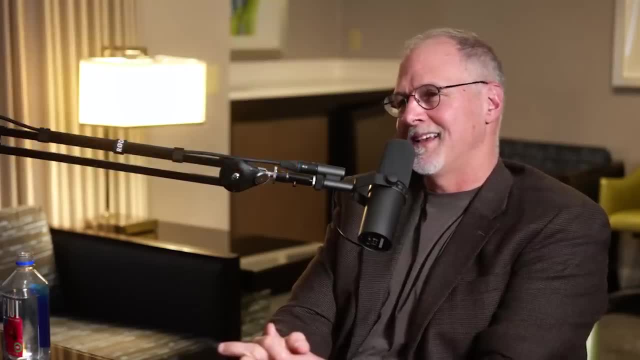 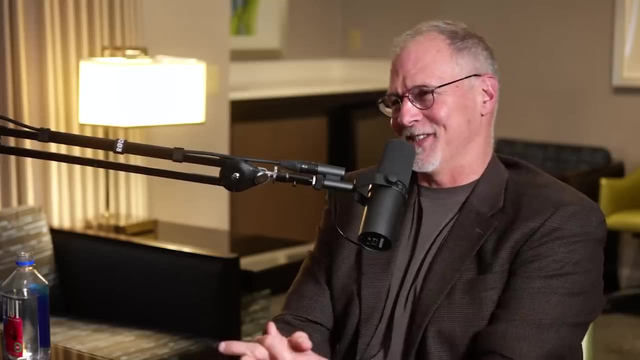 a logistics application. We decided it was too slow and couldn't pick boxes fast enough. basically, And it was doing beautifully with elegance. It did beautifully, but it just wasn't efficient enough. So we let it go. Yeah, But I think we'll come back to that machine eventually. 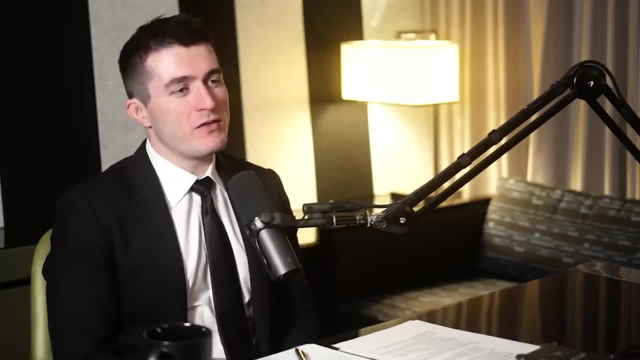 The fact that it's possible, the fact that you showed that you could do so many things at the same time in coordination, and so beautifully. there's something there That was a demonstration of what is possible. Basically, we made a hard decision and this was. 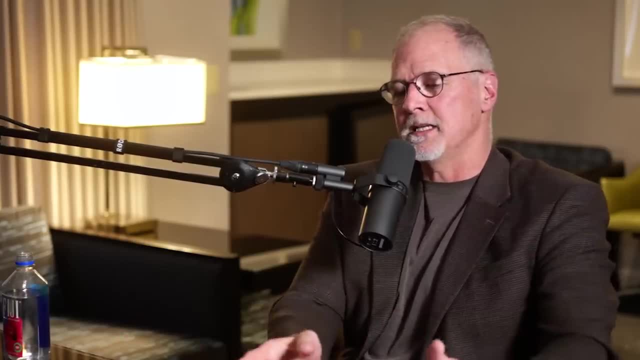 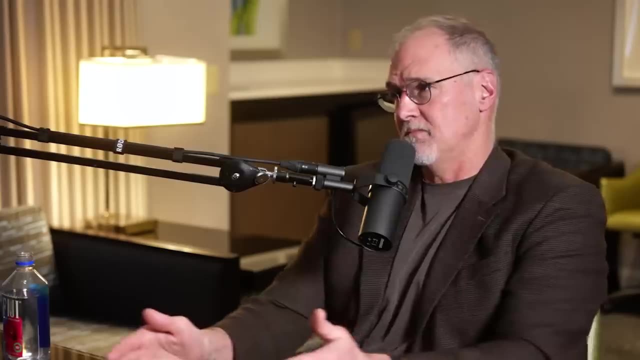 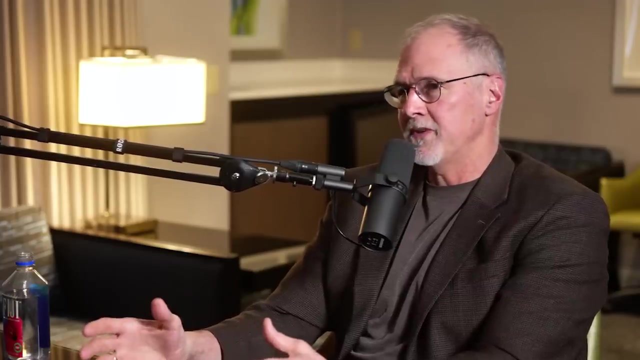 really kind of a hard-nosed business decision. It indicated us not doing it just for the beauty of the mathematics or the curiosity. but no, we actually need to build a business that can make money in the long run, And so we ended up building Stretch, which has a big heavy base with a giant. 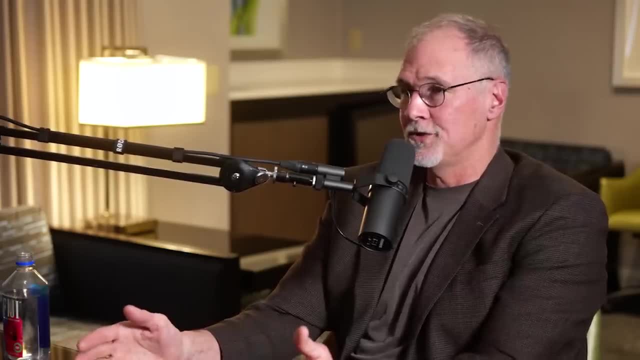 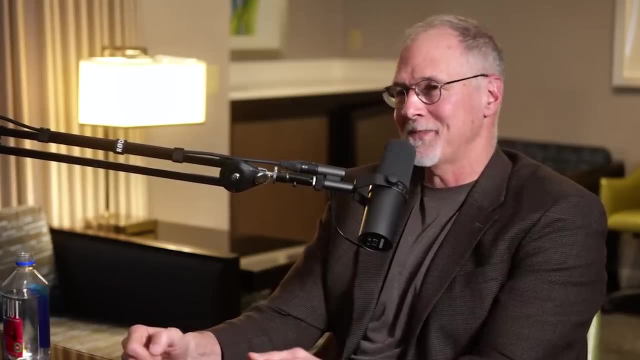 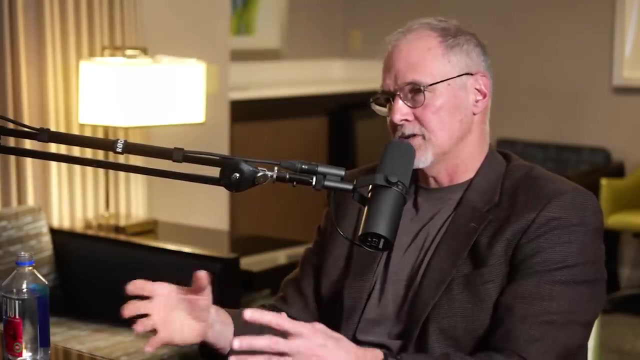 battery in the base of it that allows it to run for two shifts, 16 hours worth of operation, And that big battery sort of helps it stay balanced right, So you can move a 50-pound box around with its arm and not tip over. It's omnidirectional: It can move in any direction. 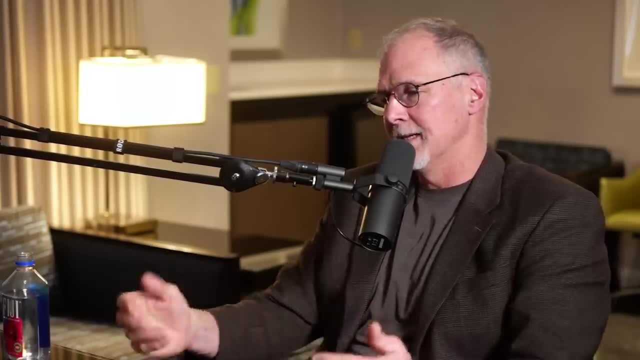 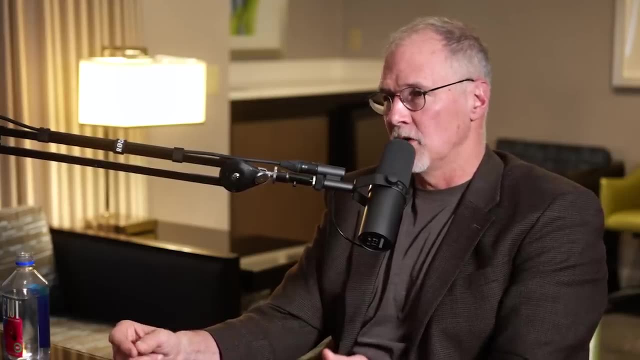 So it has a nice suspension built into it so it can deal with gaps or things on the floor and roll over it. But it's not a balancing robot. It's a mobile robot arm that can work to carry or pick or place a box up to 50 pounds anywhere in the warehouse. 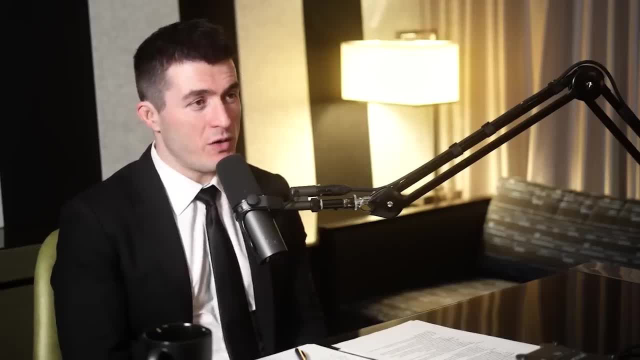 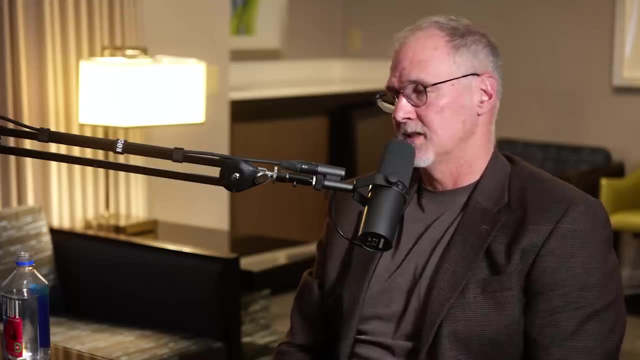 Take a box from point A to point B anywhere. Yeah, Palletize, depalletize. We're starting with unloading trucks because there's so many trucks and containers where goods are shipped and it's a brutal job. In the summer it can be. 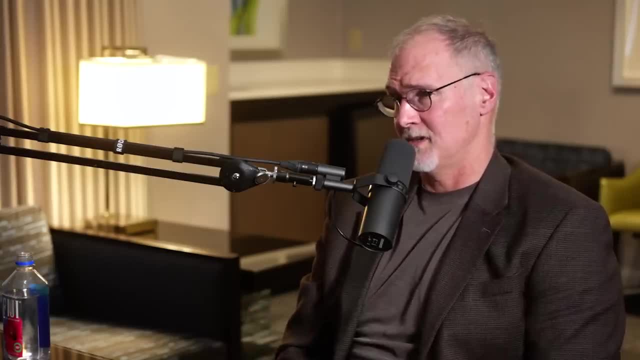 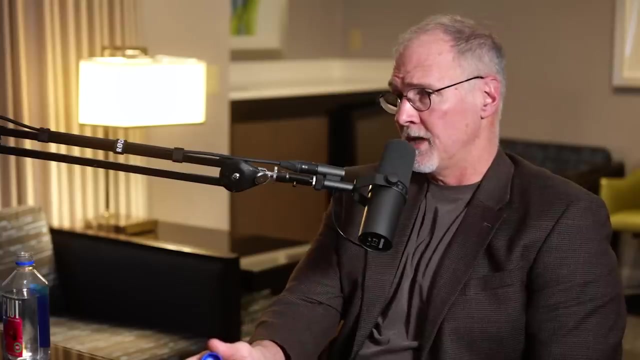 120 degrees inside that container. People don't want to do that job And it's backbreaking labor, right. Again, these can be up to 50-pound boxes, And so we feel like this is a productivity enhancer And for the people who used to do that job- unloading trucks- they're actually operating. 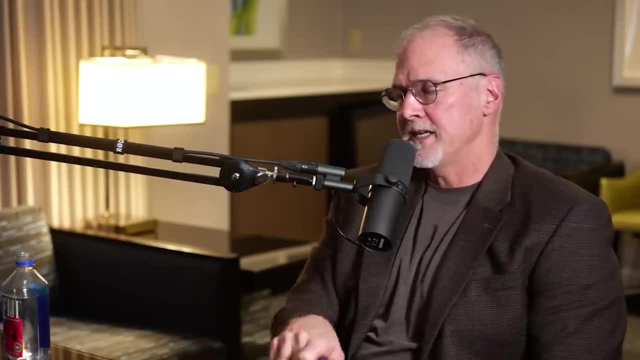 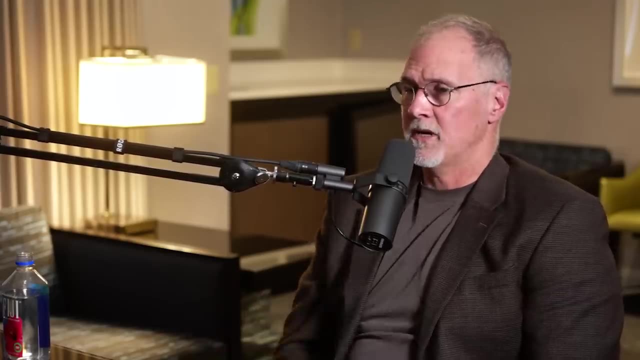 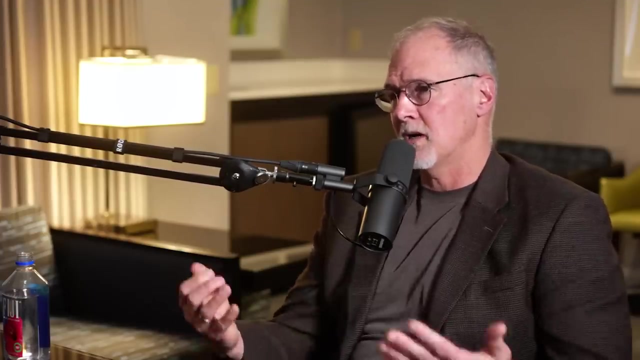 the robot now, And so by building robots that are easy to control and it doesn't take an advanced degree to manage, you can become a robot operator. And so, as we've introduced these robots to both DHL and Maersk and Gap, the warehouse workers who were doing that manual labor are now the 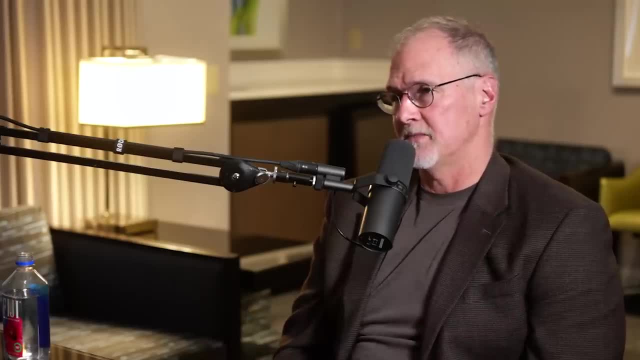 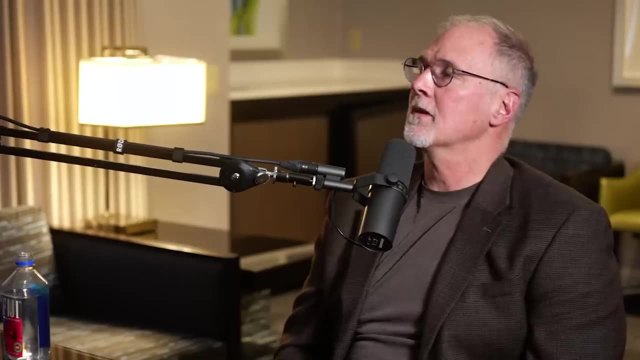 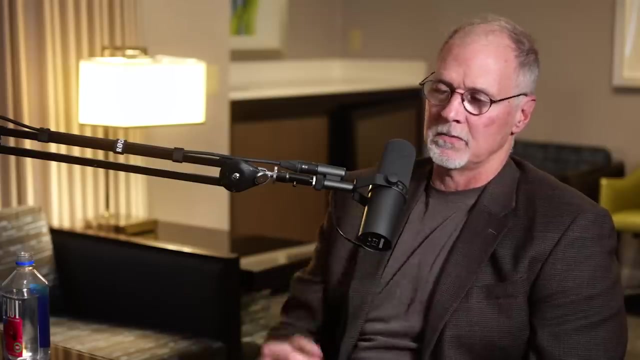 robot operators, And so we see this as ultimately a benefit to them as well. Can you say how much of a benefit to them? Can you say how much Stretch costs? Not yet, But I will say that when we engage with our customers, they'll be able to see a return on. 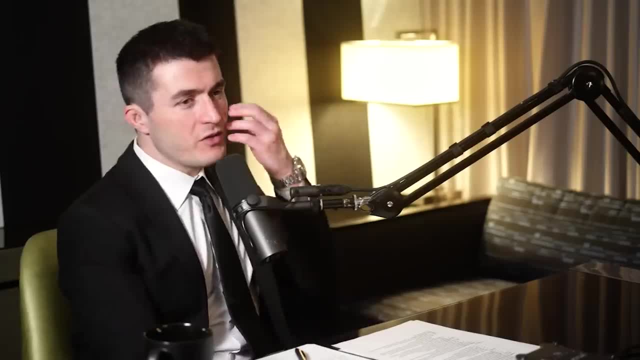 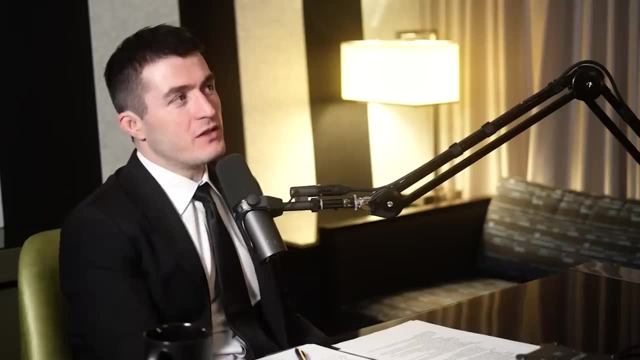 investment in typically two years. Okay, So that's something that you're constantly thinking about. how? Yeah, And I suppose you have to do the same kind of thinking with Spot. So it seems like with Stretch the application is directly obvious. 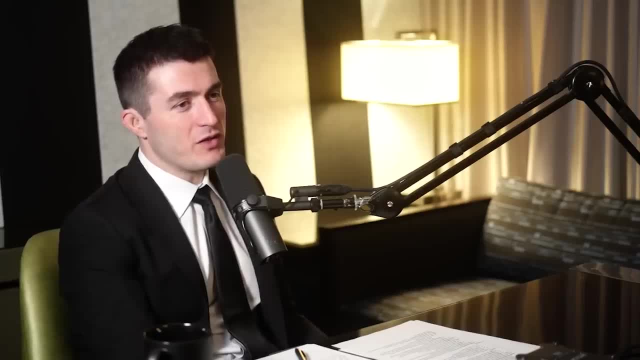 Yeah, it's a slam dunk. Yeah, And so you have a little more Flexibility. Well, I think we know the target, We know what we're going after. Yeah, And with Spot, it took us a while to figure out what we were going after. 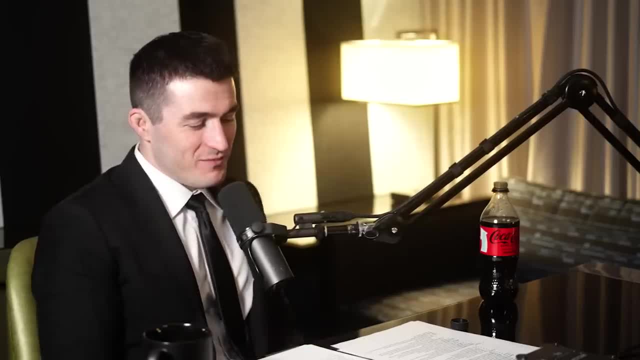 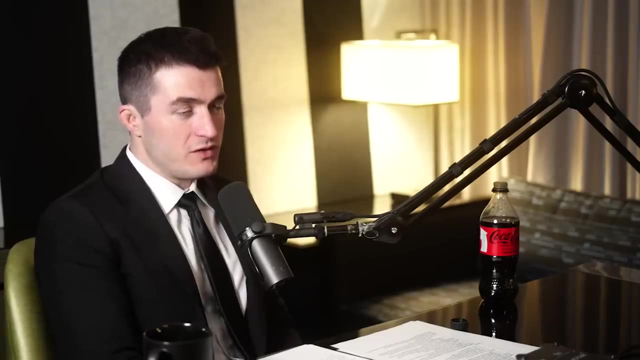 Well, let me return to that question about maybe the conversation you were having a while ago with Larry Page, maybe looking to the longer future of social robotics, of using Spot to connect with human beings, perhaps in the home. Do you see a future there, If we were to sort of hypothesize, or? 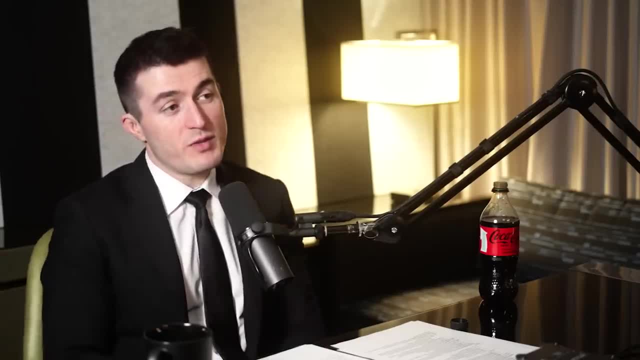 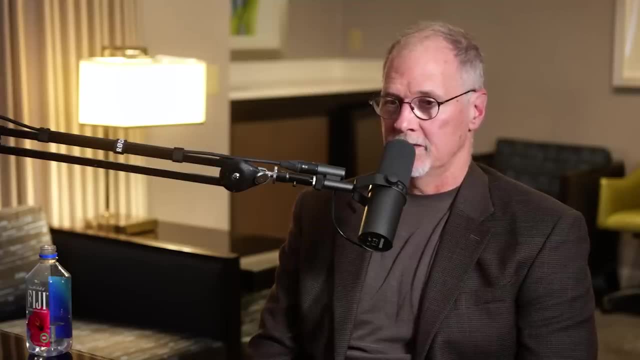 dream about a future where Spot-like robots are in the home as pets, as social robots. We definitely think about it And we would like to get there. We think the pathway to getting there is, you know, likely through these industrial applications and then mass manufacturing, You know. 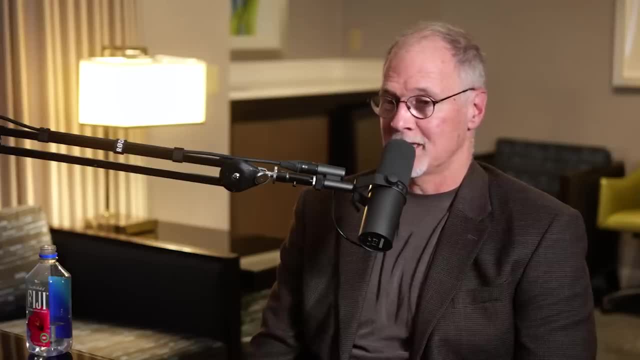 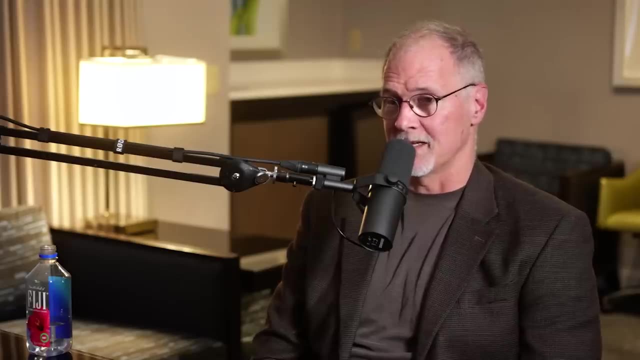 let's figure out what: how to mill, how to build the robots, how to make the software so that they can really do a broad set of skills That's going to take real investment to get there. Performance first, right Yeah. 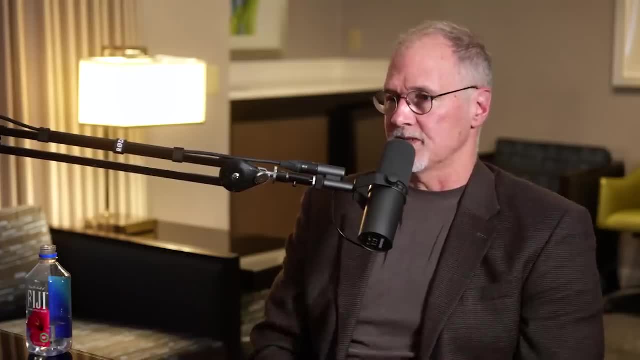 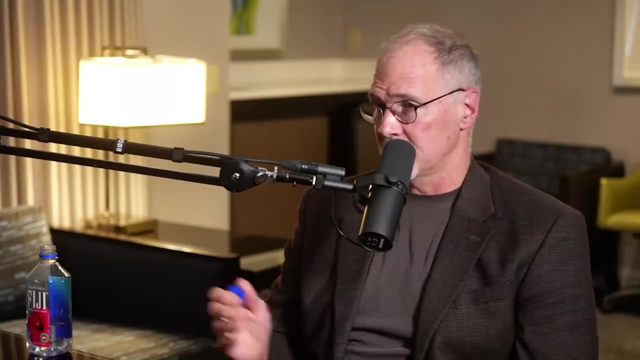 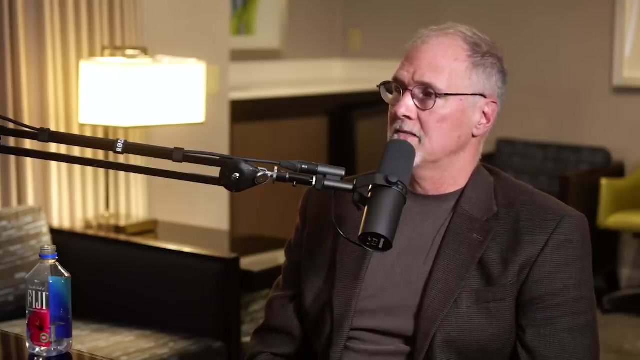 A principle of the company has always been really make the robots do useful stuff, And so you know the social robot companies that tried to start someplace else by just making acute interaction. mostly they haven't survived, And so we think the utility really needs to come. 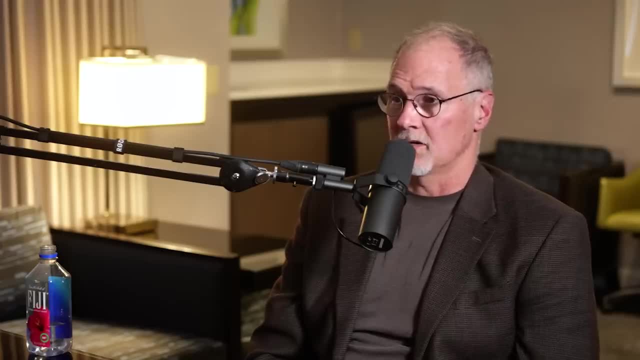 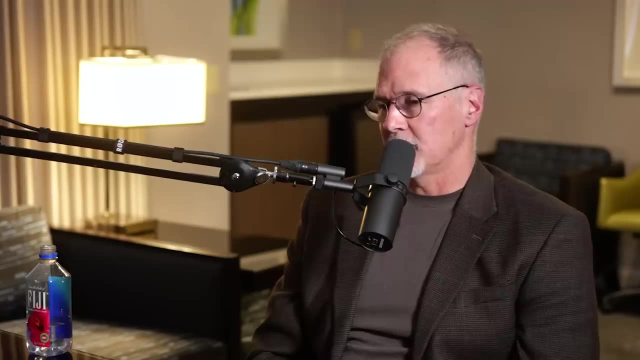 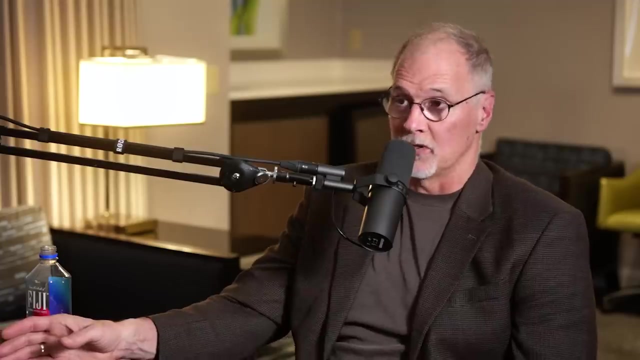 first, And that means you have to solve some of these hard problems. And so to get there, we're going to go through the design and software development in industrial, and then that's eventually going to let you reach a scale that could then be addressed to a commercial, consumer level market, And so 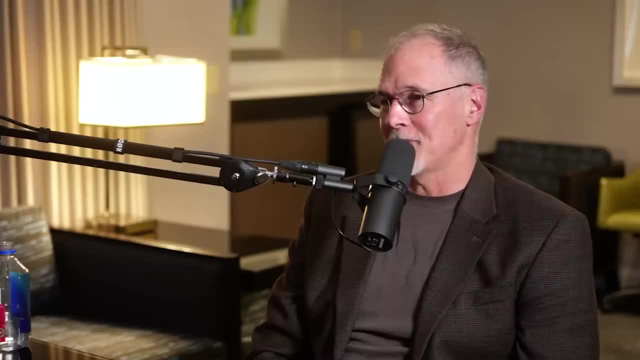 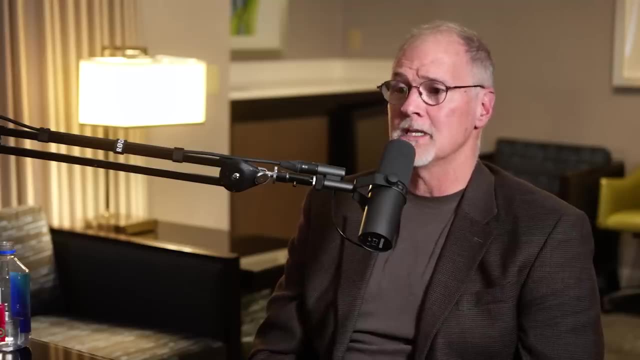 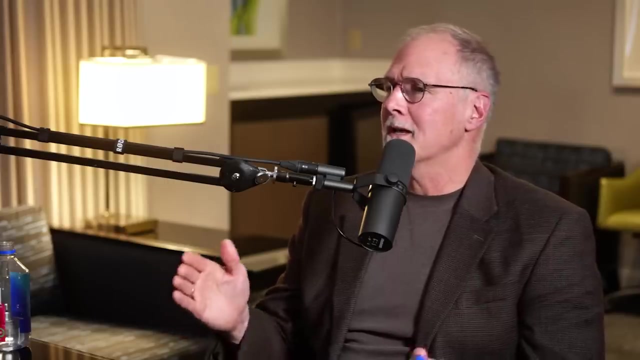 yeah, maybe we'll be able to build a smaller spot with an arm that could really go get your beer for you. But there's things we need to figure out still: how to safely really safe, And if you're going to be interacting with children, you, you better be safe And right now we, we count on a. 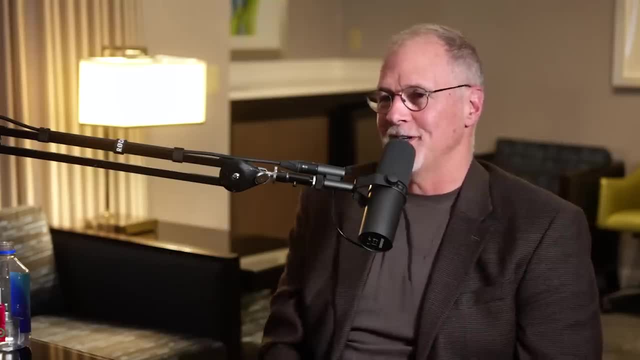 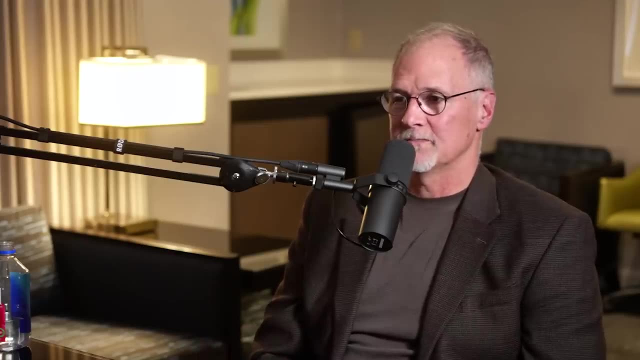 a little bit of standoff distance between the robot and people so that you don't pinch a finger, you know in the robot. so you've got a lot of things you need to go solve before you jump to that consumer level product. well, there's a kind of trade-off in safety because it feels like in the 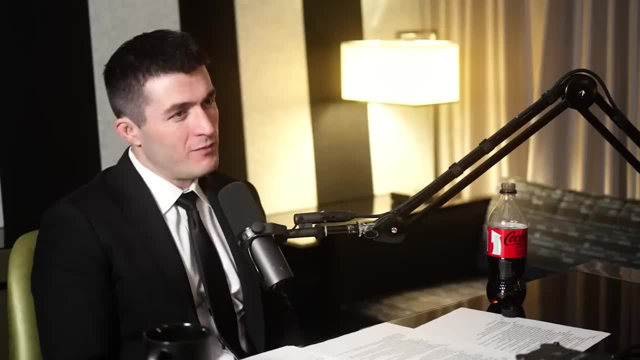 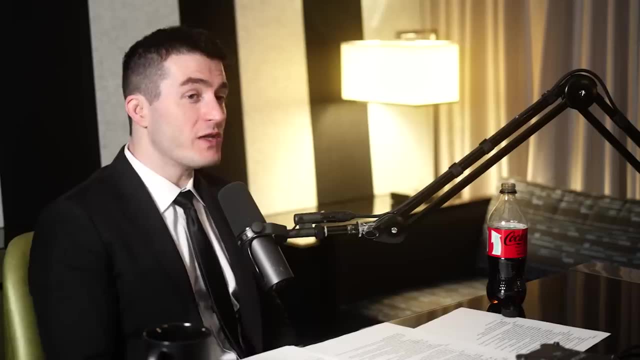 home. you can fall like you're. you don't have to be as good at like. you're allowed to fail in different ways, in more ways, as long as it's safe for the humans. so it just feels like an easier problem to solve because it feels like in the factory you're not allowed to fail. 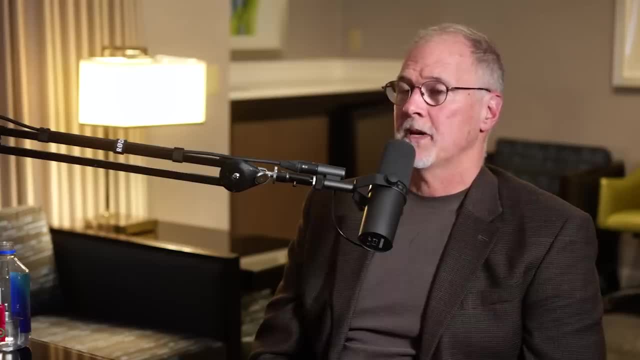 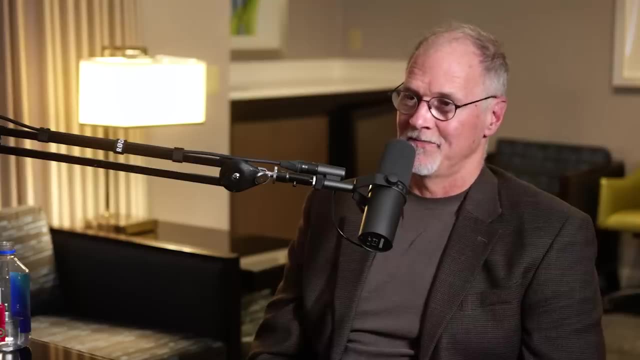 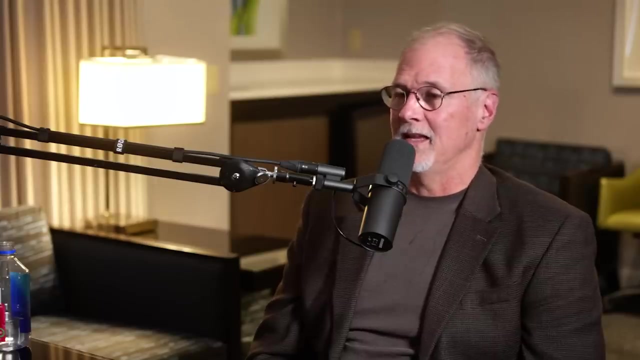 that may be true, um, but i also think the variety of things a consumer level robot would be expected to do will also be quite broad. yeah, they're going to want to get the beer and know the difference between the beer and a coca-cola, or my snack and or. 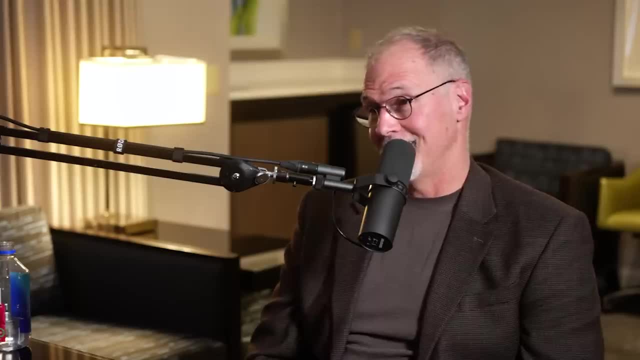 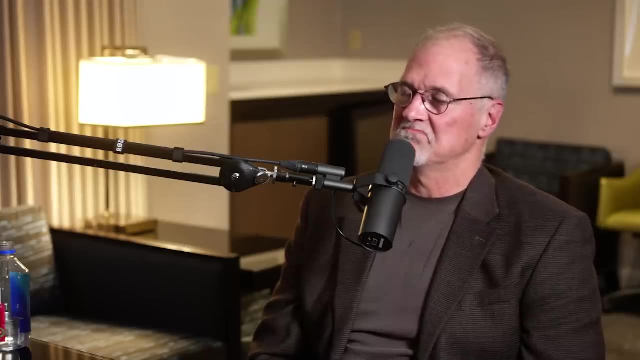 or you know, they're all going to want you to clean up the dishes- uh, you know- from the table without breaking them. those are pretty complex tasks, and so there's there's still work to be done there. so, to push back on that, here's my application. i think they'll be very interesting. 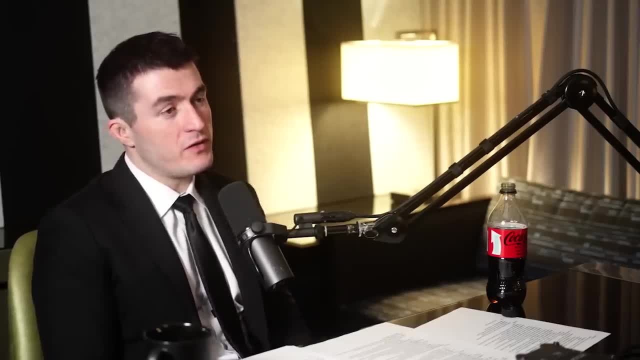 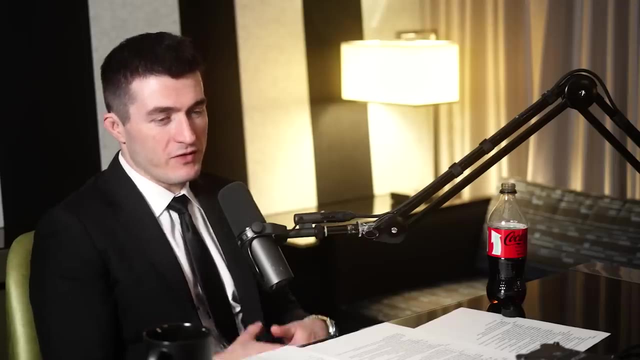 i think the application of being a pet, a friend, so like no tasks, just be cute, because i not cute. not cute like the dog is more. a dog is more than just cute. a dog is a friend, is a companion. there's something about just having interacted with them and maybe because 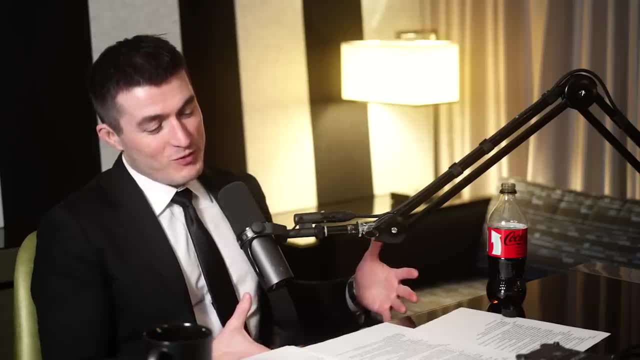 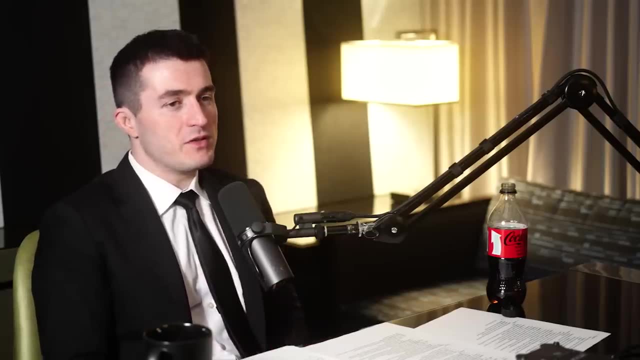 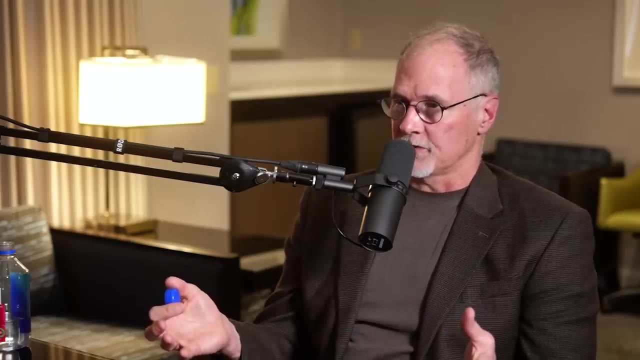 i'm hanging out alone with the robot dogs a little too much, but like there's a, there's a connection there and it feels like that connection is not should not be disregarded. no, it should not be disregarded. robots that can somehow communicate through their physical gestures: are you're going? 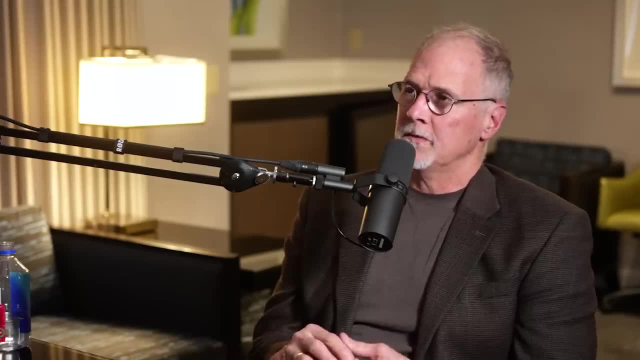 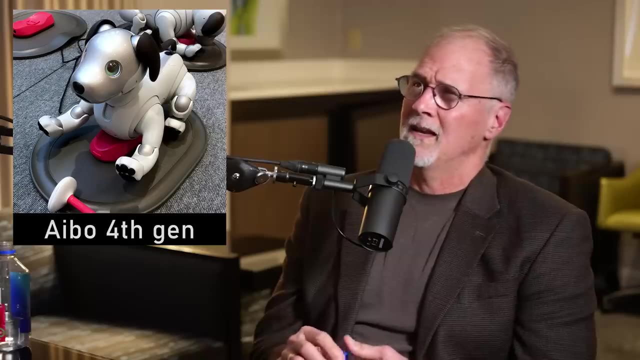 to be more attached to in the long run. do you remember i ibo the sony ibo. yeah, i ibo, ibo, ibo, ibo. they sold over a hundred thousand of those, maybe a hundred and fifty thousand, you know what probably wasn't considered a successful product for them. they suspended that eventually and then they. 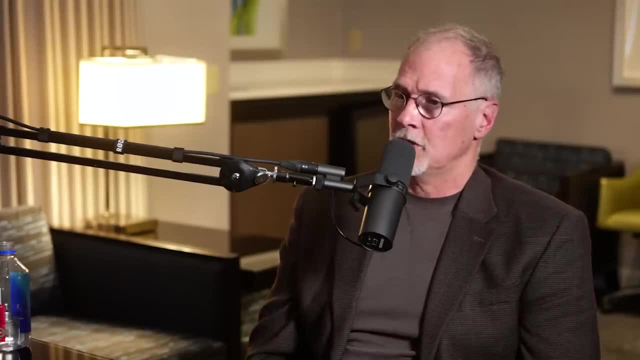 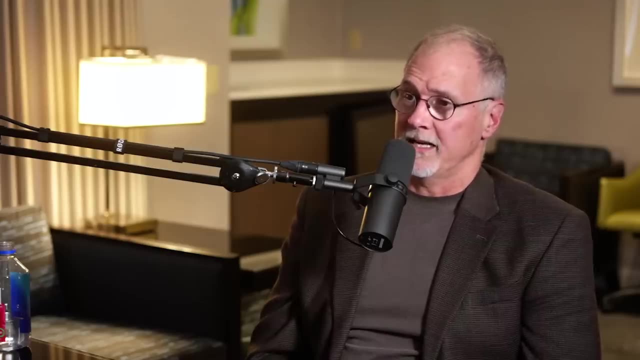 brought it back. so he brought it back and people definitely, you know, treated this as a, as a pet, as an, as a companion. um, and i think that will come around again- um, will you get away without having any other utility, maybe in a world where we can really 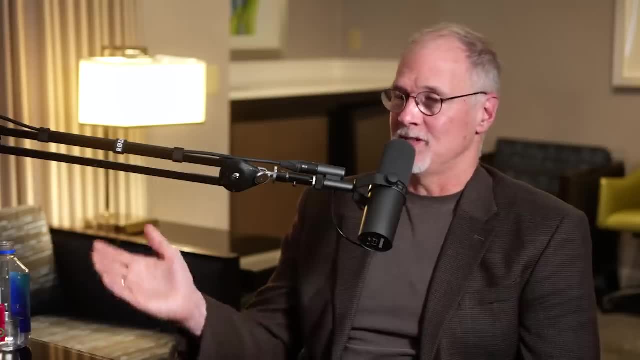 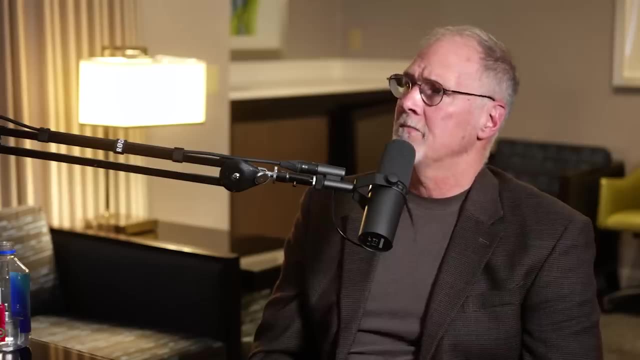 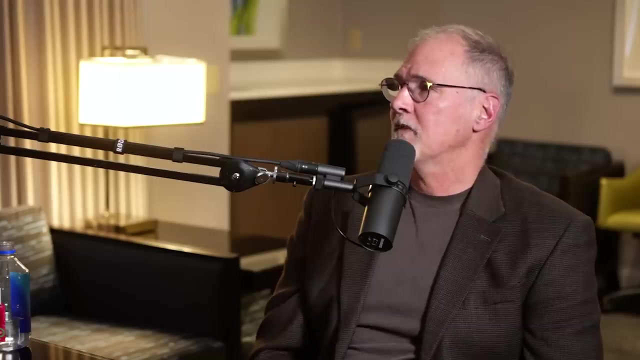 talk to our simple little pet because you know, chat, gpt or some other generative ai has made it possible for you to really talk in what seems like a meaningful way. maybe that'll open the social robot up again. um, that's probably not a path we're going to go down because again we're 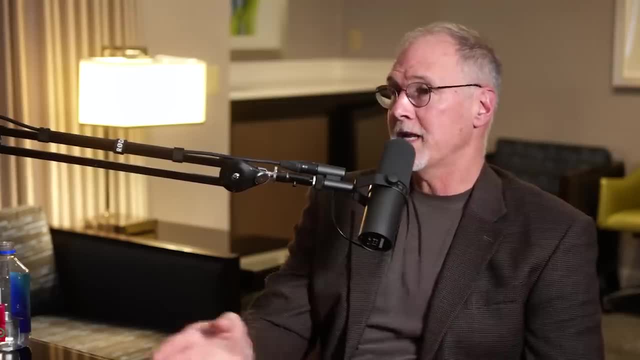 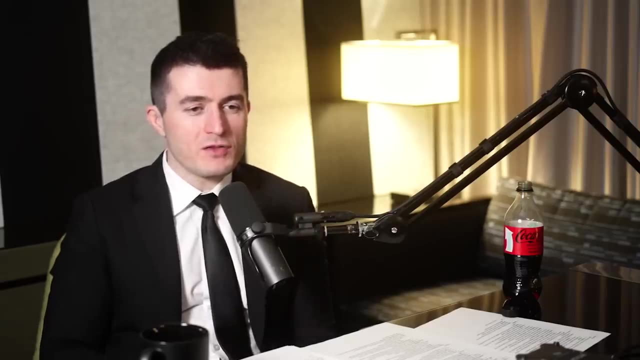 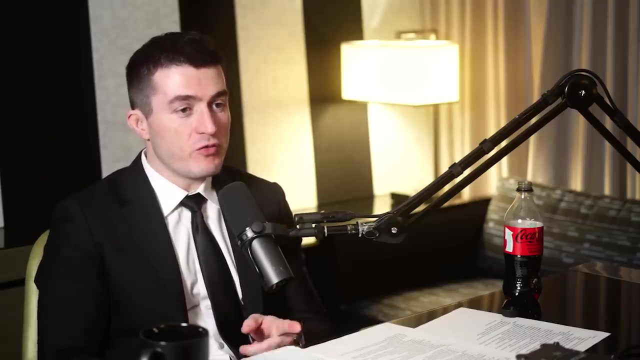 so focused on performance and utility. we can add those other things also, but we really want to start from that foundation of utility. i think, yeah, but i i also want to predict that you're wrong on that. so, which is that the very path you're taking, which is creating a great robot platform, will very easily take a leap to adding. 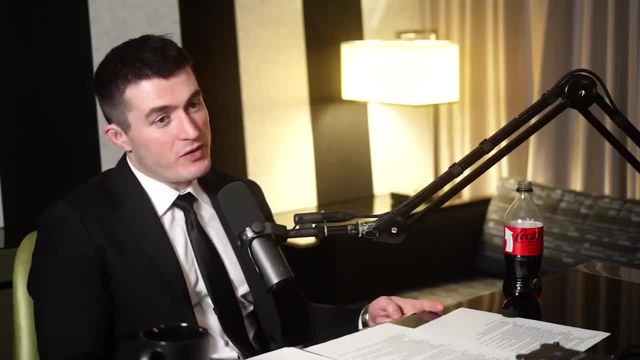 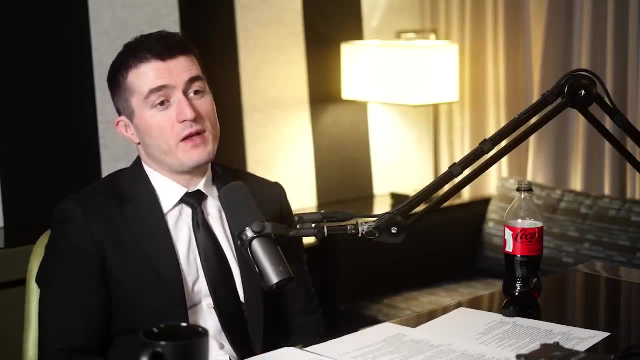 a chat gpt, like capability, maybe gpt5, and there's just so many open source alternatives. you could just plop that on top of spot. and because you have this robust platform and you're figuring out how to mass manufacture it and how to make it work, you're going to have to figure out how to. 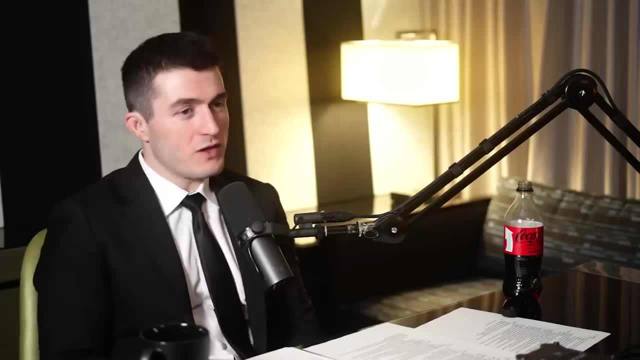 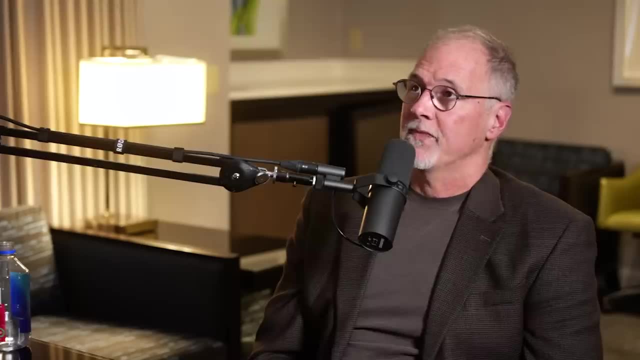 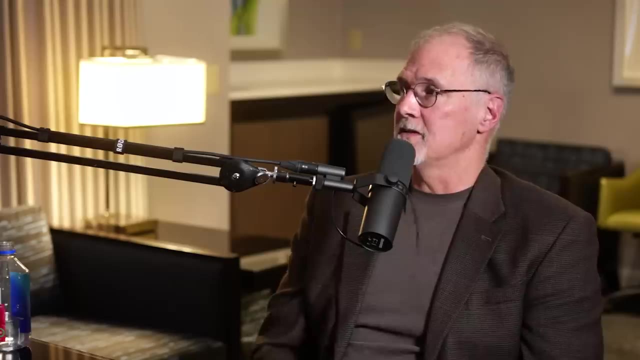 drive the cost down and how to make it, you know, reliable, all those kinds of things. it'll be a natural transition to where, just adding chad gpt. i do think that being able to verbally converse, or even converse through through gestures, you know, part of part of these learning models is 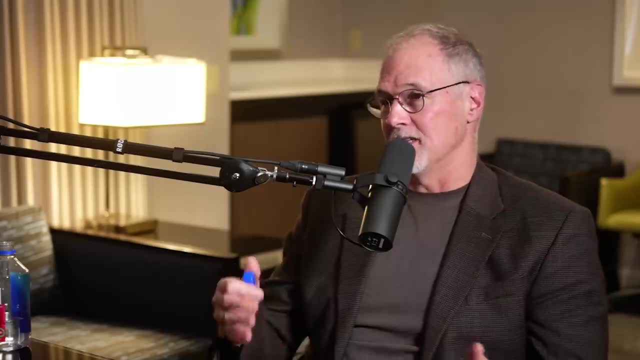 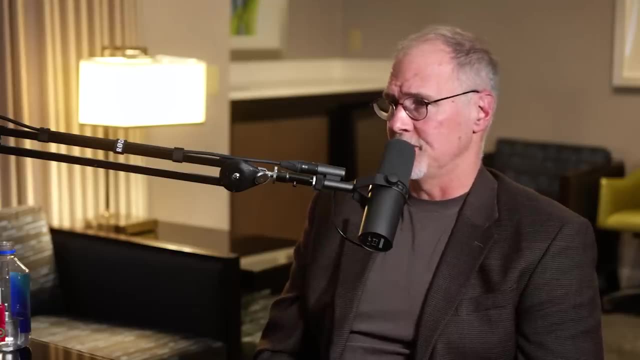 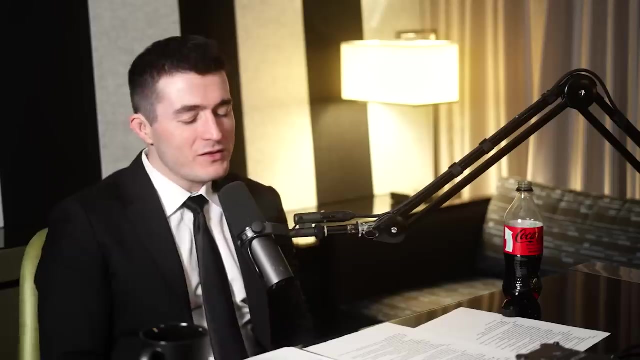 that you know. you can now look at video and image imagery and associate- you know intent with that. those will all help in the communication between robots and people, for sure, and that's going to happen obviously more quickly than any of us were expecting. i mean, what else do you want from life? a friend to get your beer and then just talk? 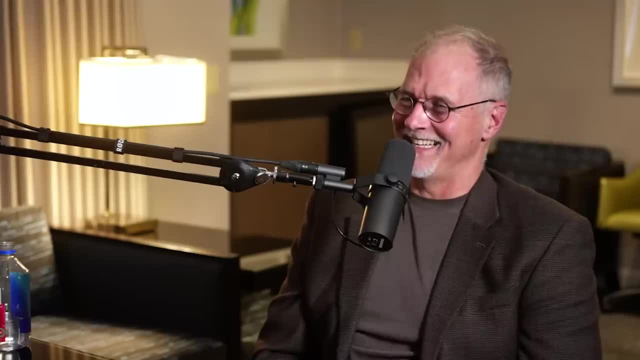 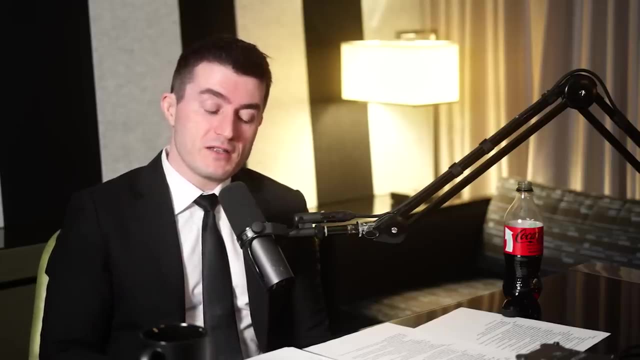 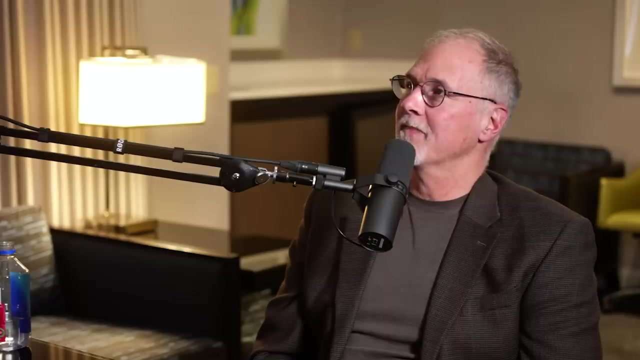 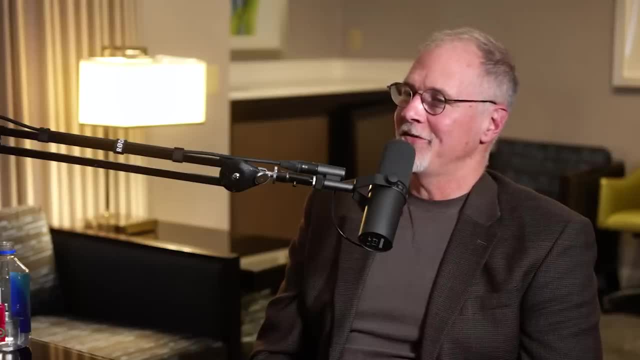 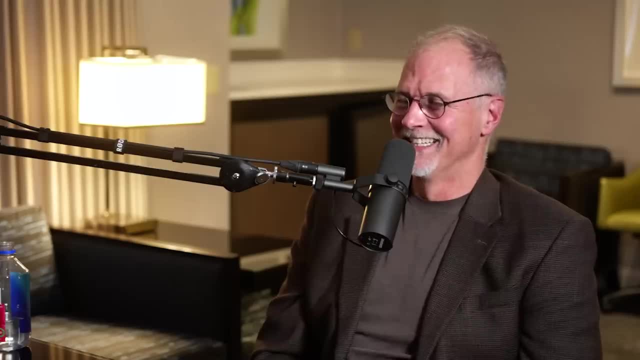 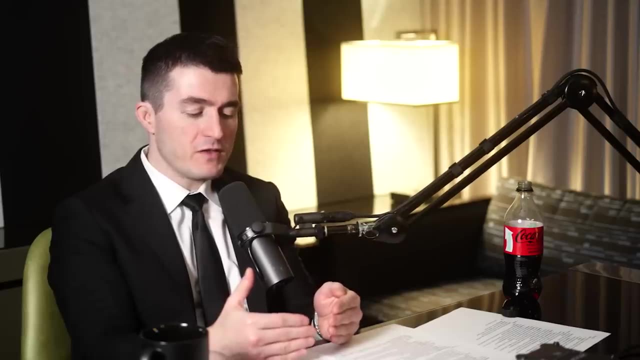 of joint, like memory of, yeah, having witnessed, hey, that that's what friendship, that's what connection, that's what love is in. in many cases, some of the deepest friendships you have is having gone through a difficult time together and having a shared memory of an amazing time. 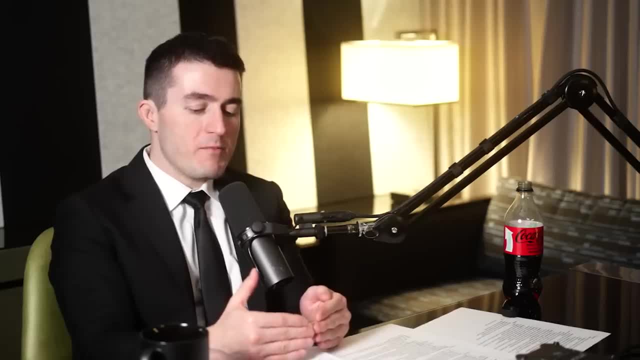 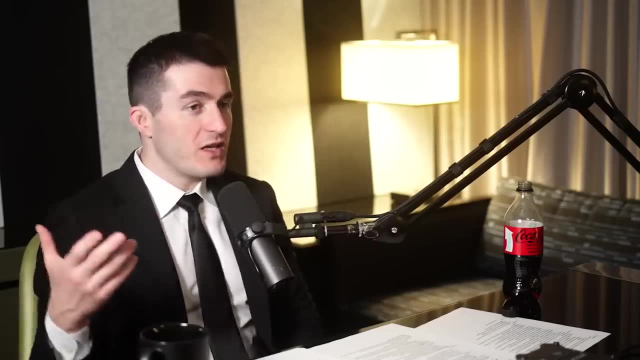 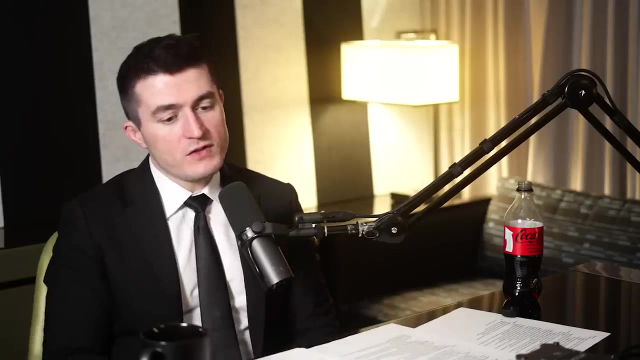 or a difficult time and kind of that memory, creating this like foundation based on which you can then experience the world together. The silly, the mundane stuff of day to day is somehow built on a foundation of having gone through some shit in the past, And the current systems are not personalized in that way. 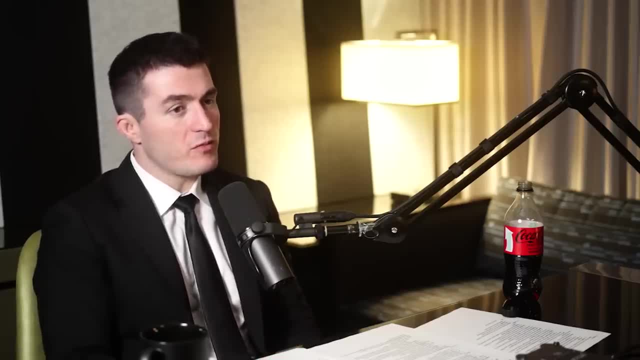 But I think that's a technical problem, not some kind of fundamental limitation. So combine that with an embodied robot like Spot, which already has magic in its movement. I think it's a very interesting possibility of where that takes us. But of course you have to build that on top of a company. 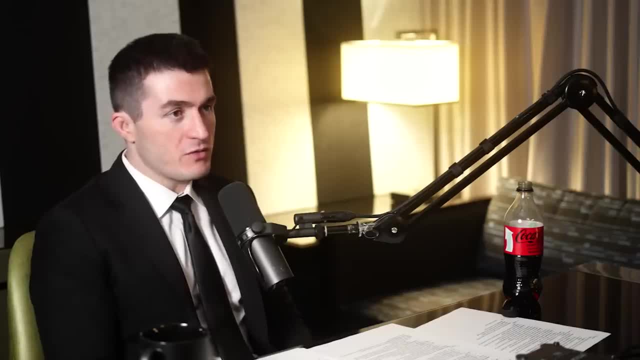 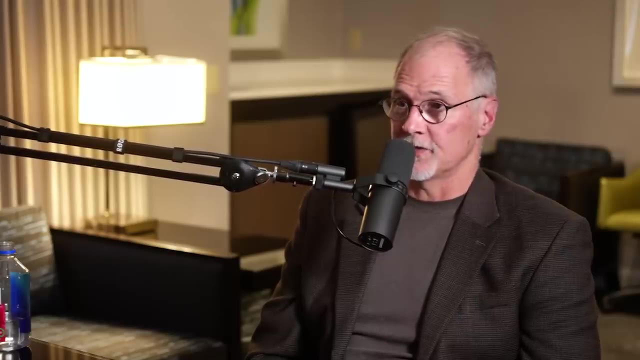 that's making money with real application, with real customers and with robots that are safe and work and reliable and manufactured scale. And I think we're in a unique position in that, Because of our investors, primarily Hyundai, but also SoftBank- still owns 20% of us. 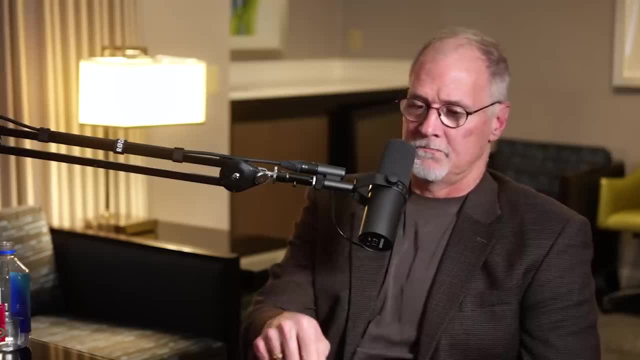 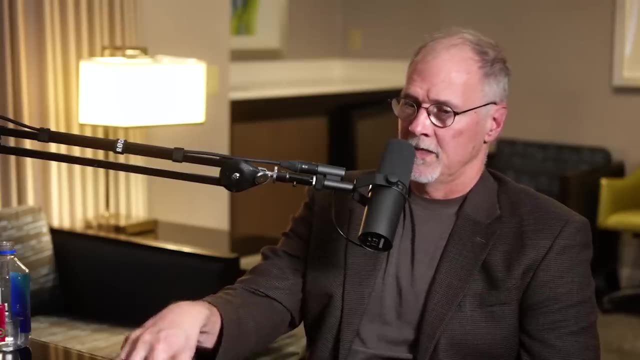 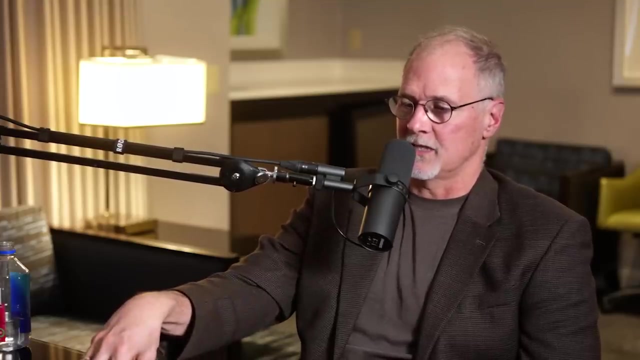 They don't. They're not totally fixated on driving us to profitability as soon as possible. That's not the goal. The goal really is a longer term vision of creating you know what does mobility mean in the future. How is this mobile robot technology going to influence us? 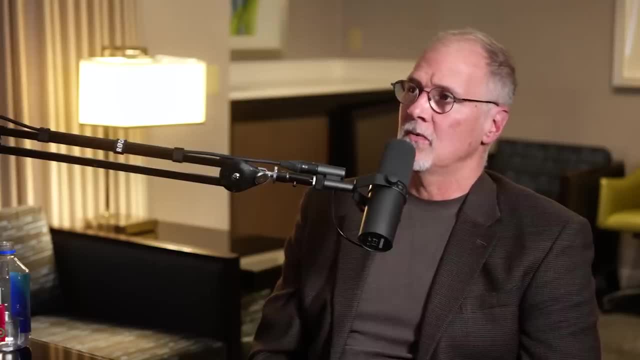 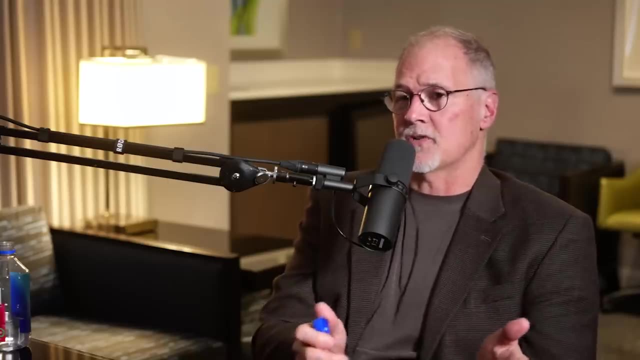 And can we shape that? And they want both, And so we are, as a company, are trying to strike that balance between let's build a business that makes money. I've been describing that to my own team as self-destination, If I want to drive my own ship. 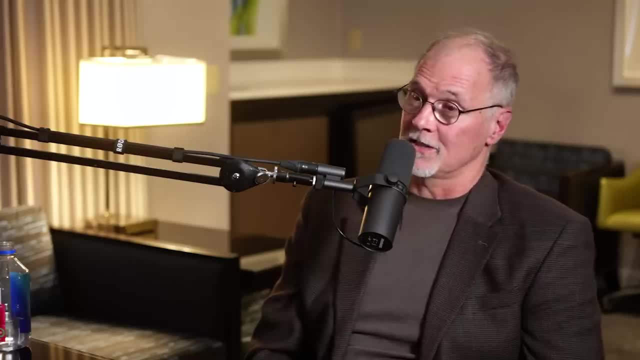 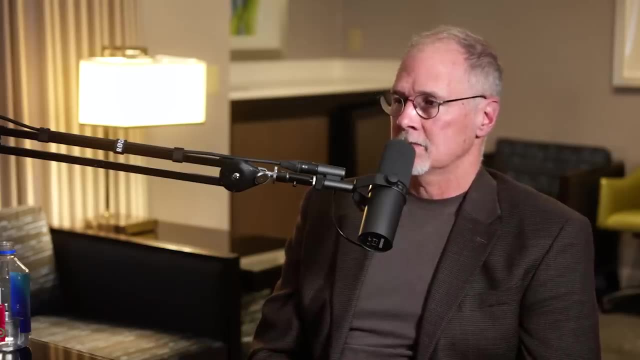 we need to have a business that's profitable in the end, Otherwise somebody else is going to drive the ship for us. So that's really important. But we're going to retain the aspiration that we're going to build the next generation of technology. 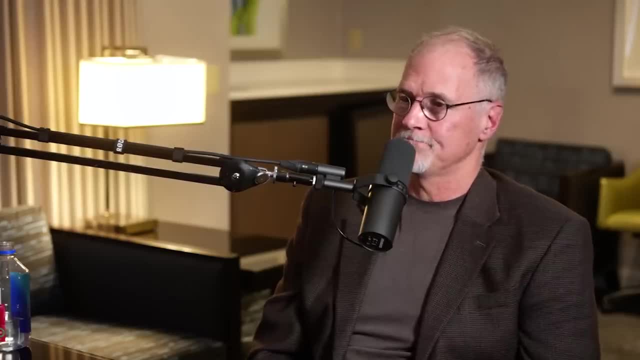 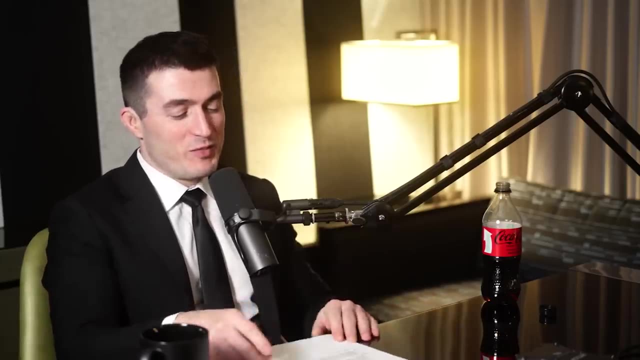 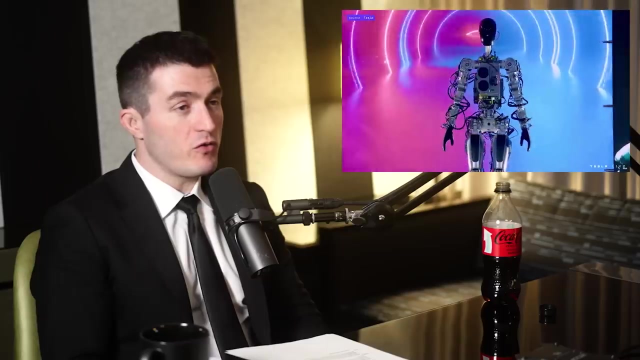 at the same time, And the real trick will be if we can do both. Speaking of ships, let me ask you about a competitor And somebody who's become a friend. So Elon Musk and Tesla have announced they've been in the early days of building a humanoid robot. 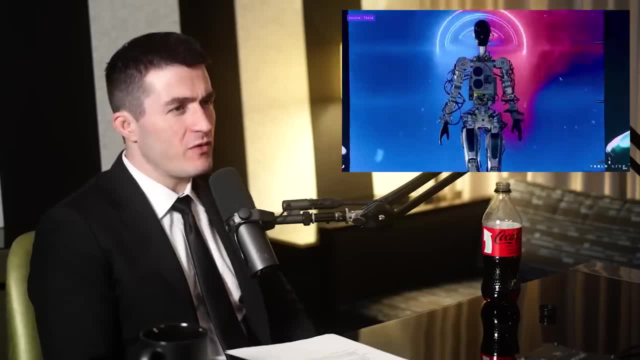 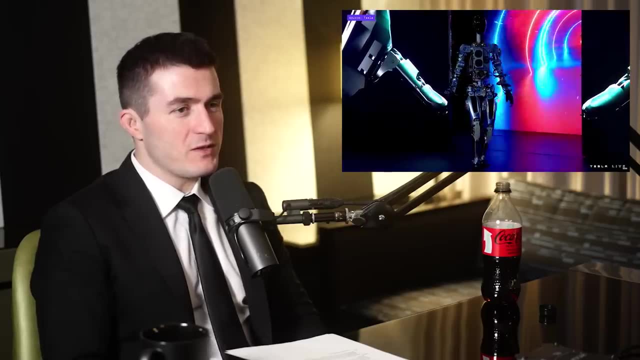 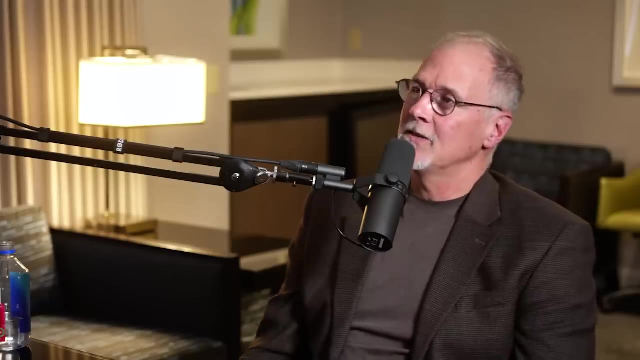 How does that change the landscape of your work? So there's sort of from the outside perspective, it seems like. well, from a fan, As a fan of robotics, it just seems exciting. It's very exciting, right. When Elon speaks, people listen. 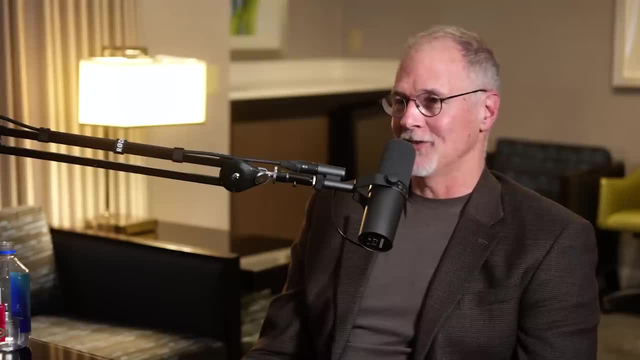 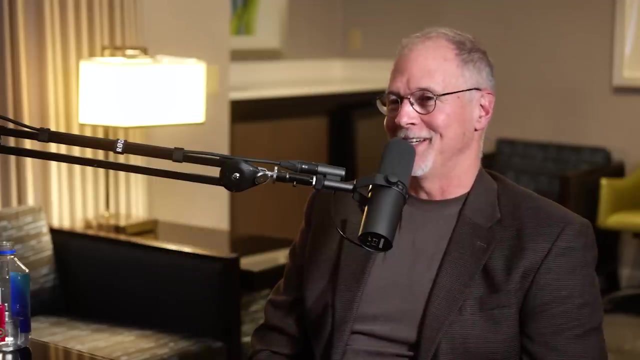 And so it suddenly brought a bright light onto the work that we'd been doing for over a decade, And I think that's only going to help, And, in fact, what we've seen is that, in addition to Tesla, we're seeing a proliferation of robotic companies arise now. 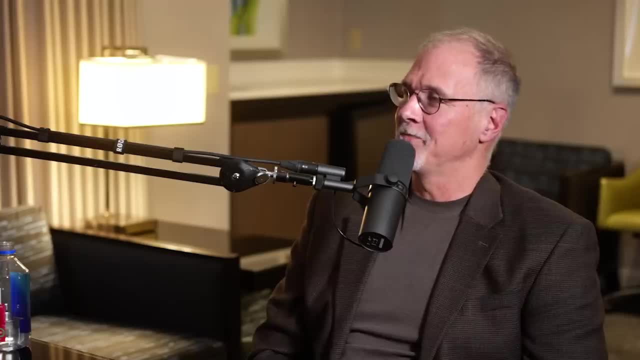 Including humanoid. Yes, Oh, wow, Yeah. And interestingly, many of them, as they're raising money, for example, will claim whether or not they have a former Boston Dynamics employee on their staff as a criteria. Yeah, that's true. 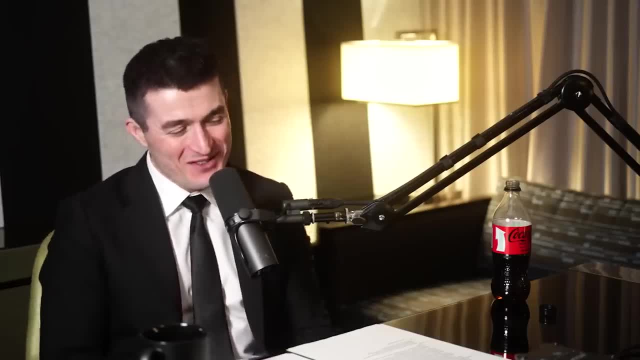 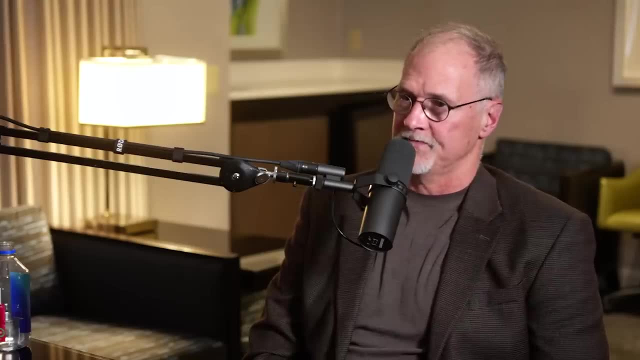 I would do that as a company, yeah for sure. And shows you're legit- Yeah, So you know what It has brung, a tremendous validation to what we're doing, and excitement And competitive juices are flowing. you know the whole thing. 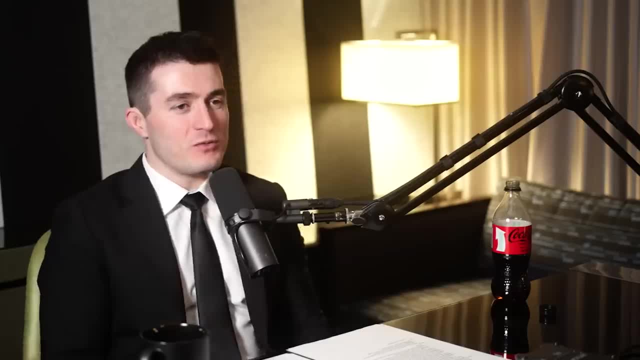 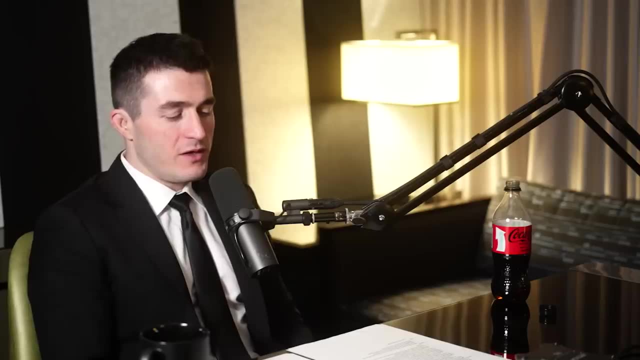 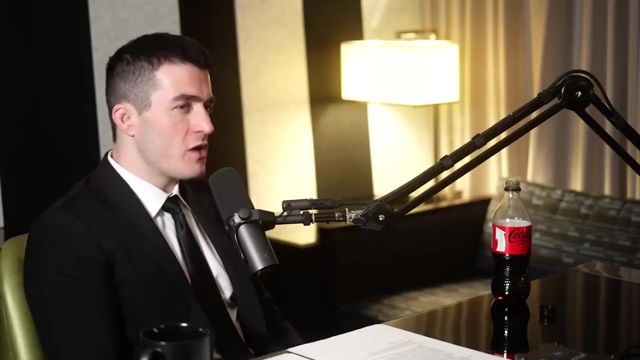 So it's all good. Elon has also kind of stated that. you know, maybe he implied that the problem is solvable in the near term, which is a low-cost humanoid robot that's able to do. that's a relatively general use. 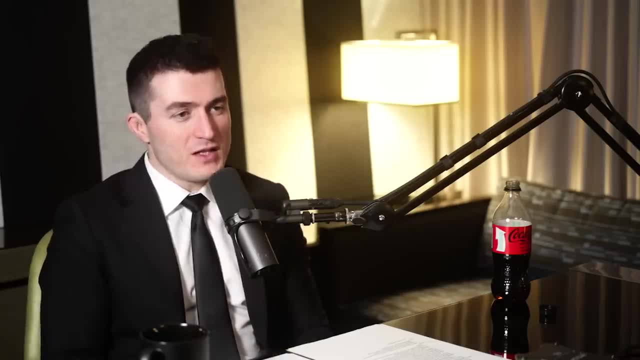 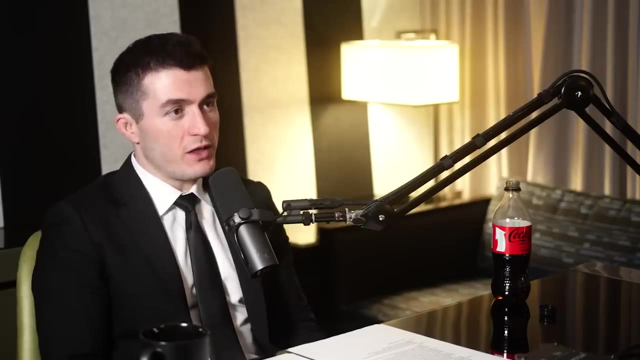 in this case robot. So I think Elon is known for sort of setting these kinds of incredibly ambitious goals, maybe missing deadlines, but actually pushing not just the particular team he leads but the entire world to like accomplishing those. Do you see Boston Dynamics? 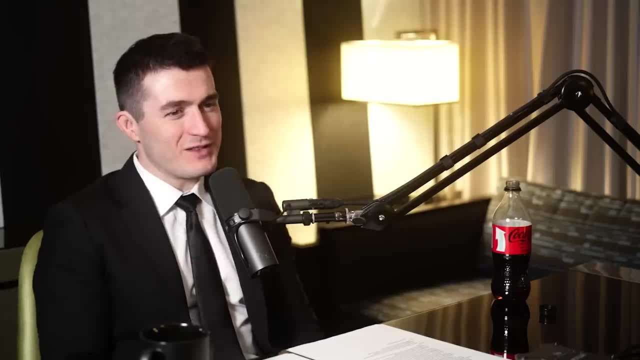 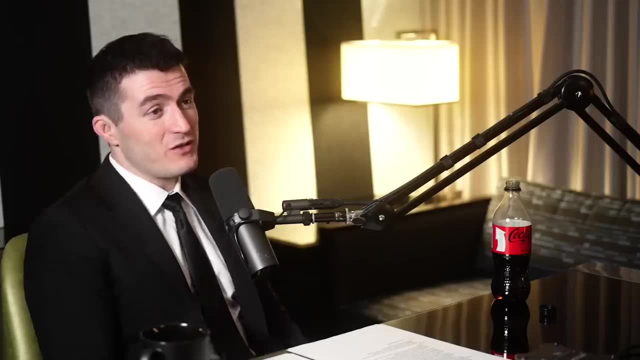 in the near future being pushed in that kind of way, Like this excitement of competition, kind of pushing out Atlas maybe to do more cool stuff, trying to drive the cost of Atlas down perhaps? Or I mean, I guess I want to ask. 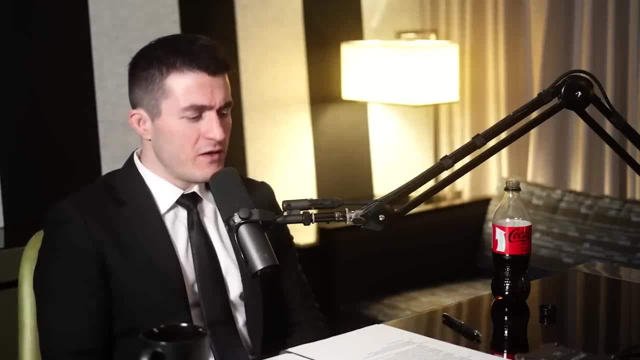 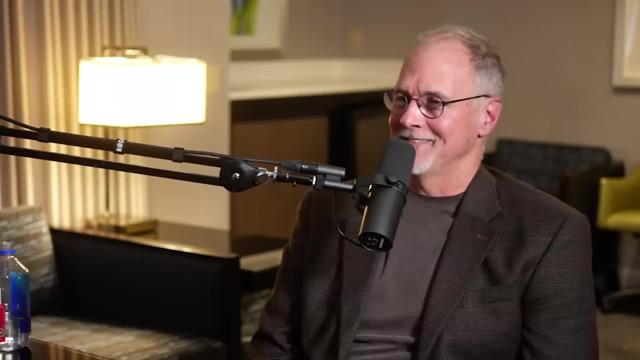 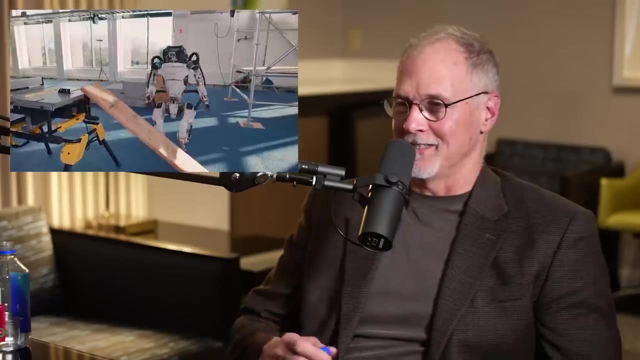 if there's some kind of exciting energy in Boston Dynamics due to this little bit of competition. Oh yeah, definitely. When we released our most recent video of Atlas, you know- I think you'd seen it- the scaffolding and throwing the box of tools around. 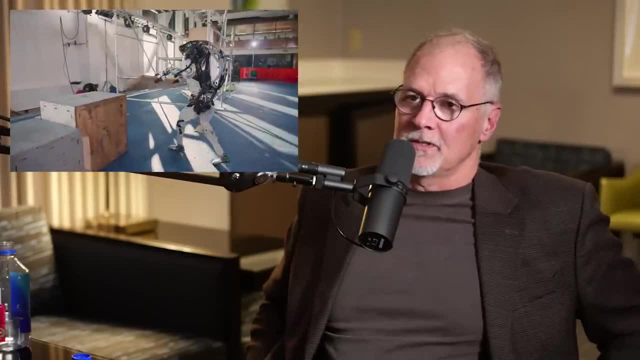 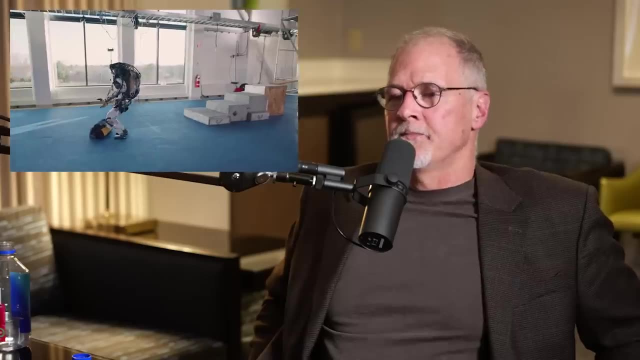 and then doing the flip at the end. We were trying to show the world that not only can we do this parkour mobility thing, but we can pick up and move heavy things, Because if you're going to work in a manufacturing environment, that's what you've got to be able to do. 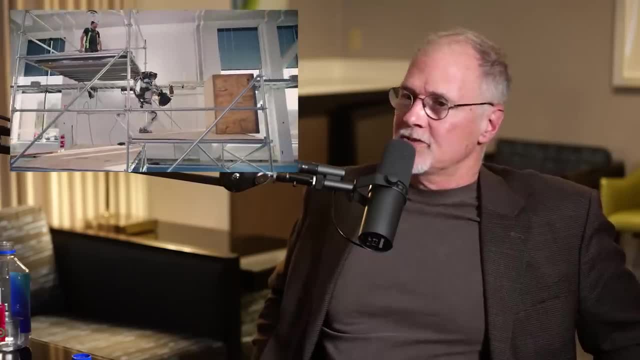 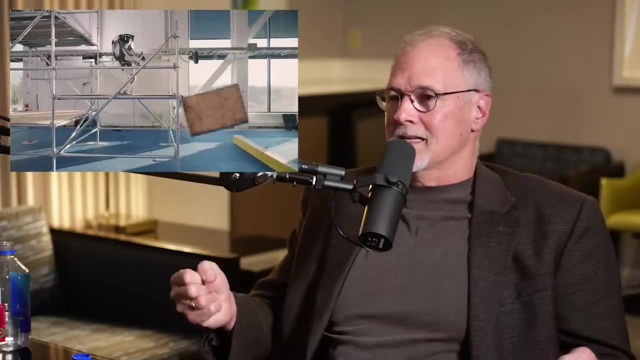 And for the reasons I explained to you earlier, it's not trivial to do so. You know, changing the center of mass. you know, by picking up a 50-pound block. you know, for a robot that weighs, I don't know, 150 pounds. 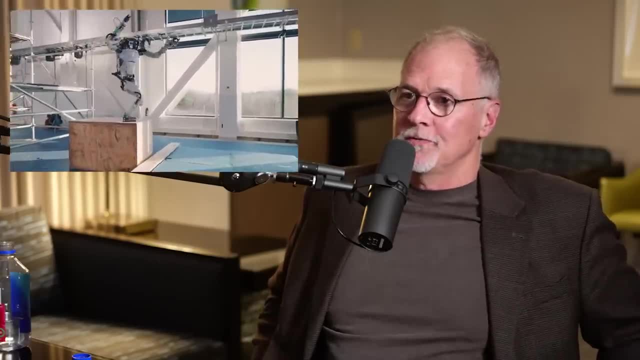 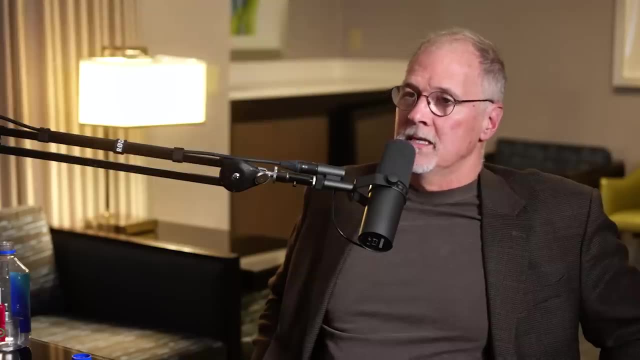 that's a lot to accommodate. So we're trying to show that we can do that And so it's totally been energizing. You know, we see the next phase of Atlas being more dexterous hands that can manipulate and grab more things. 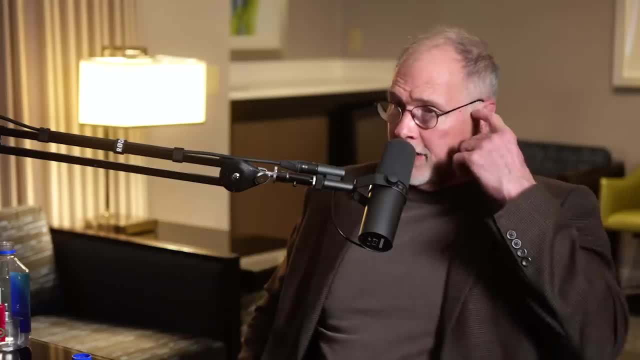 that we're going to start by moving big things around that are heavy and that affect balance. And why is that? Well, really tiny, dexterous things probably are going to be hard. Well, really tiny, dexterous things probably are going to be hard. 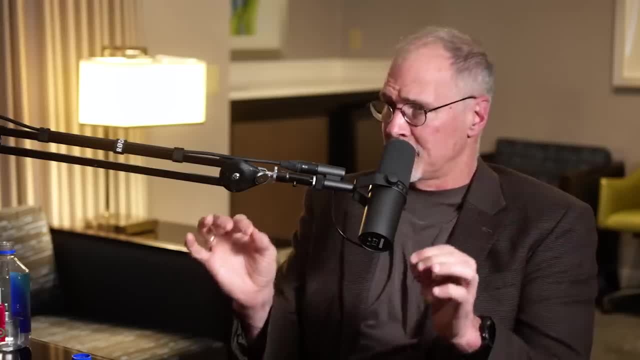 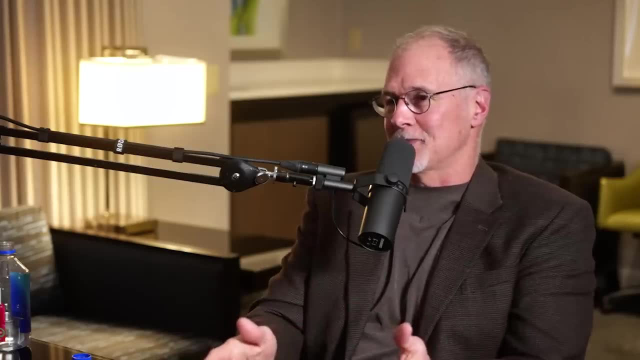 There's so little support in the right place and, you know, maybe you could go build a special-purpose robot arm, you know, for stuffing chips into electronics boards. But we don't really want to do really fine work like that. I think more coursework. 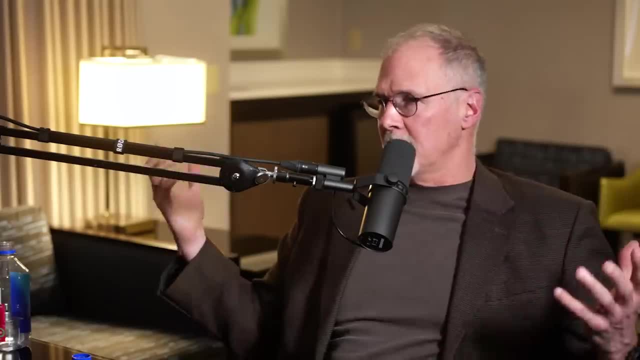 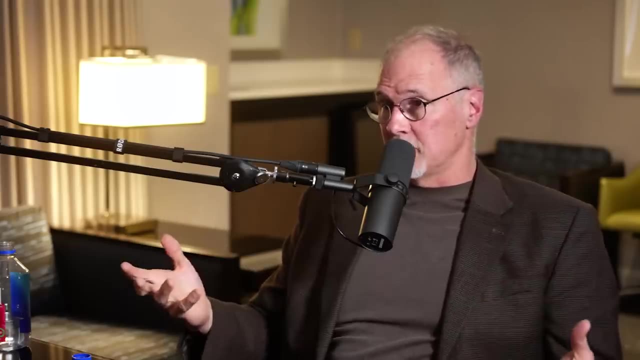 where you're using two hands to pick up and balance an unwieldy thing, maybe in a manufacturing environment, maybe in a construction environment. those are the things that we think robots are going to be able to do with the level of dexterity. 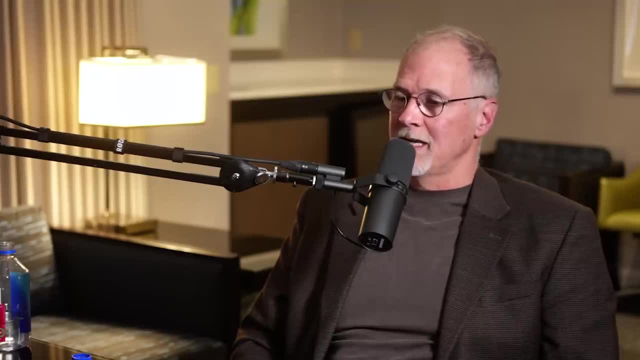 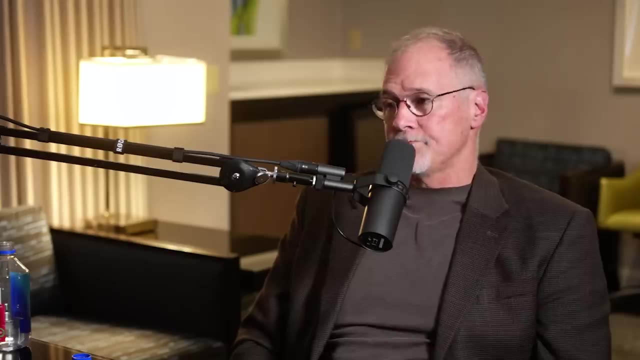 that they're gonna have in the next few years And that's where we're headed. And I think- and Elon has seen the same thing right- He's talking about using the robots in a manufacturing environment. We think there's something very interesting there. 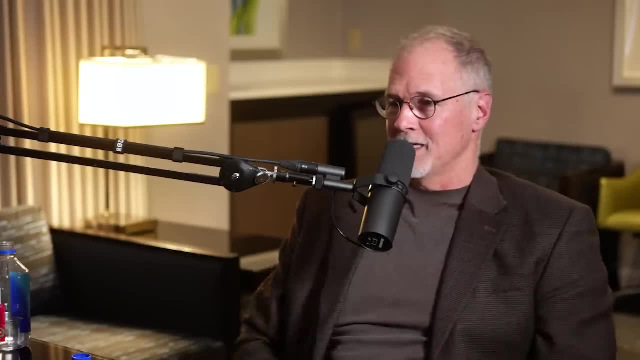 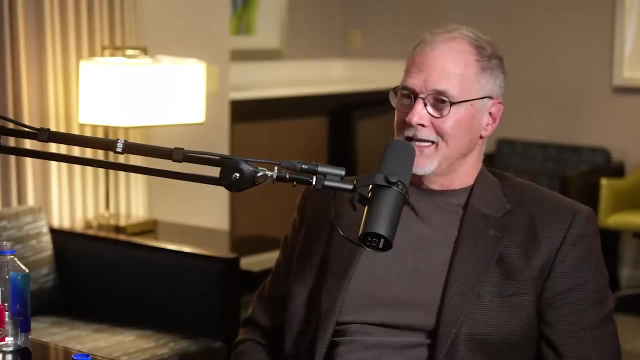 about having this a two-armed robot, Because when you have two arms, you can transfer a thing from one hand to the other, you can turn it around, you can reorient it in a way that you can't do it if you just have one hand on it. 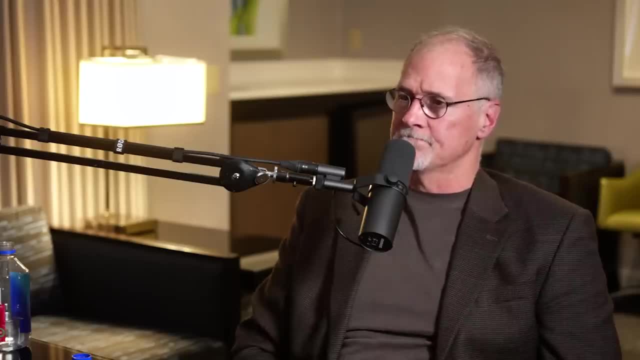 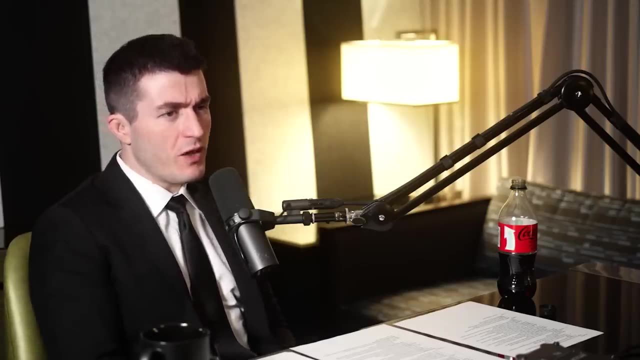 And so there's a lot that extra arm brings to the table. So I think, in terms of mission you mentioned, Boston Dynamics really wants to see what's the limits of what's possible, And so the cost comes second Or it's a component, but first figure out. 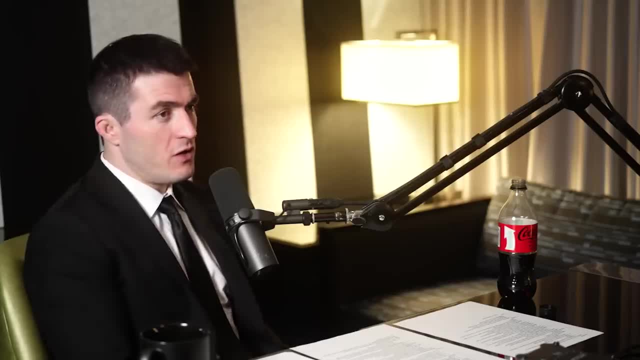 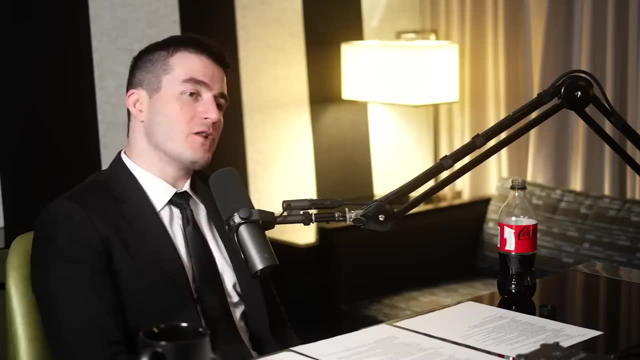 what are the limitations? I think with Elon, he's really driving the cost down. Is there some inspiration, some lessons you see there, of the challenge of driving the cost down, especially with Atlas, with a humanoid robot. Well, I think the thing that he's certainly been learning. by building car factories is what that looks like. and scaling By scaling you can get efficiencies that drive costs down very well, And the smart thing that they have in their favor is they know how to manufacture. they know how to build electric motors. 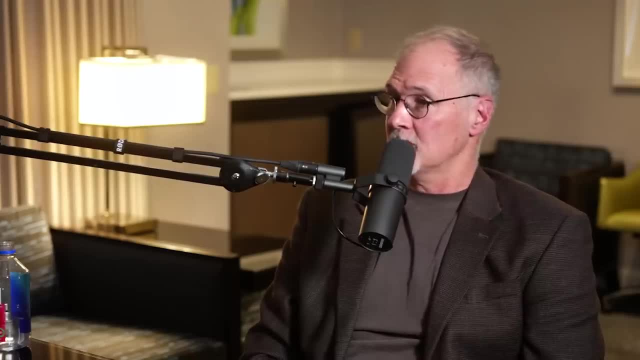 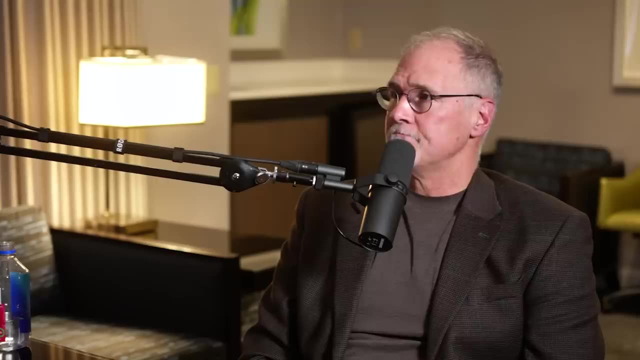 they know how to build computers and vision systems. So there's a lot of overlap between modern automotive companies and robots. But hey, we have a modern robotic- I mean the automotive company- behind us as well, So bring it on. Who's doing pretty well, right? 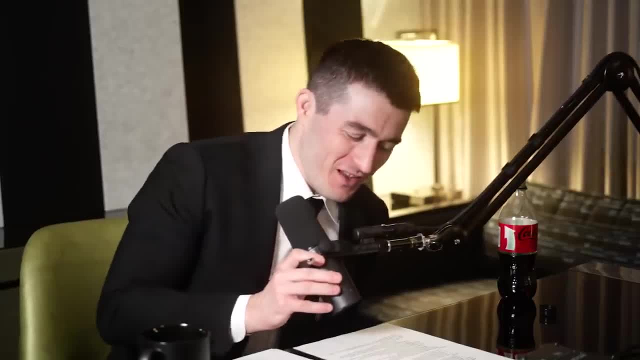 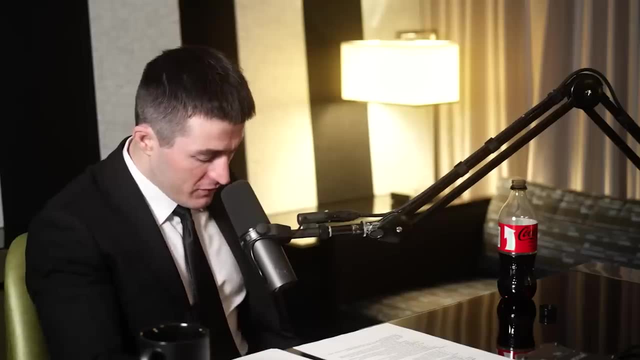 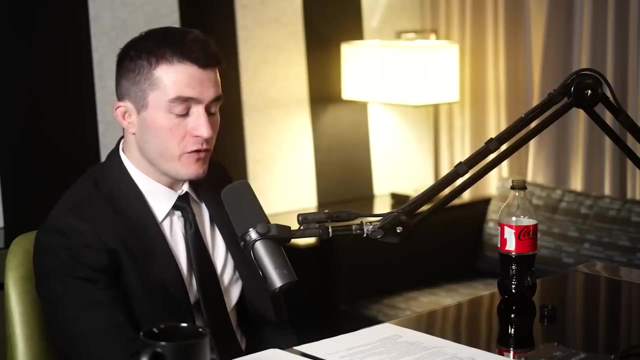 The electric vehicles from Hyundai are doing pretty well. I love it. So how much? so? we've talked about some of the low level controls, some of the incredible stuff that's going on and basic perception, But how much do you see currently and in the future of Boston Dynamics? 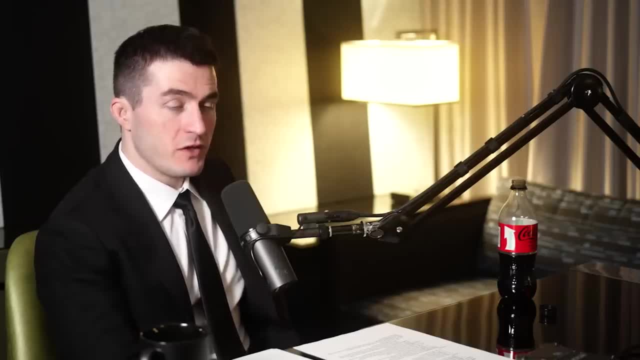 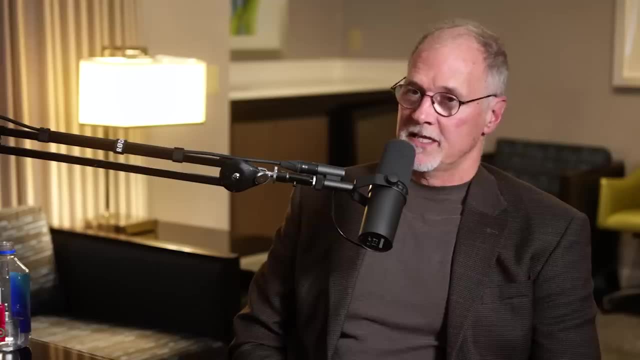 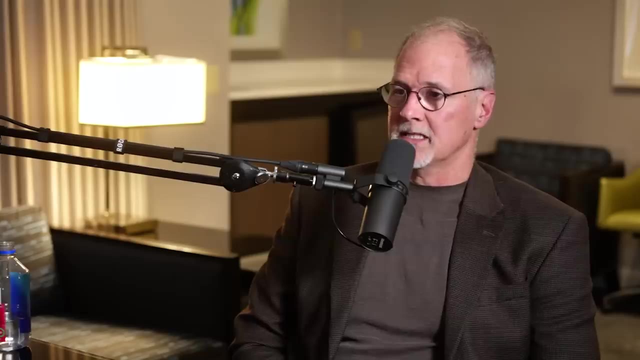 sort of more high-level machine learning applications. Do you see customers adding on those capabilities or do you see Boston Dynamics doing that in-house? Some kinds of things we really believe are probably going to be more broadly available, maybe even commoditized. You know, using a machine learning. 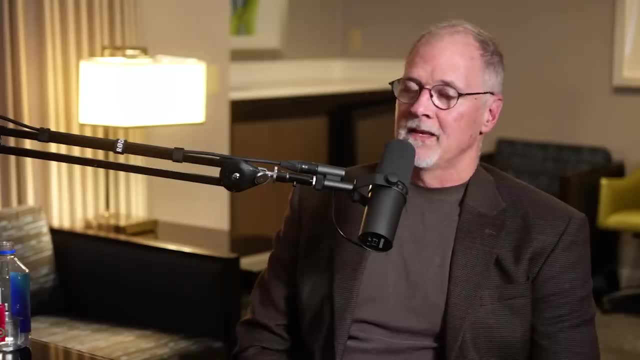 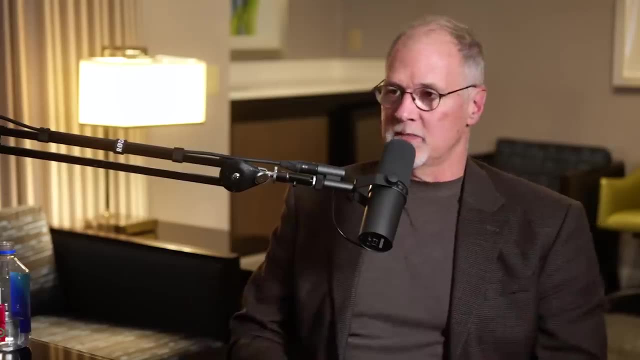 like a vision algorithm so a robot can recognize something in the environment. That ought to be something you can just download Like. I'm going to a new environment and I have a new kind of door handle or piece of equipment I want to inspect. 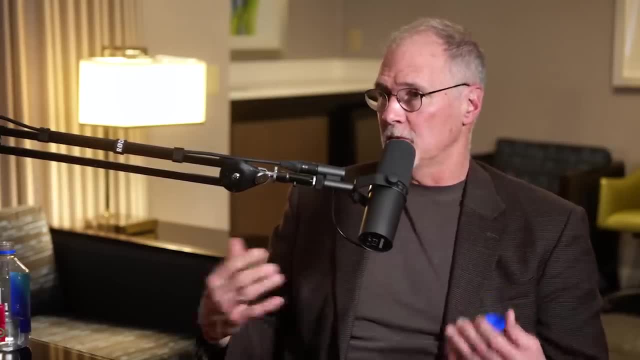 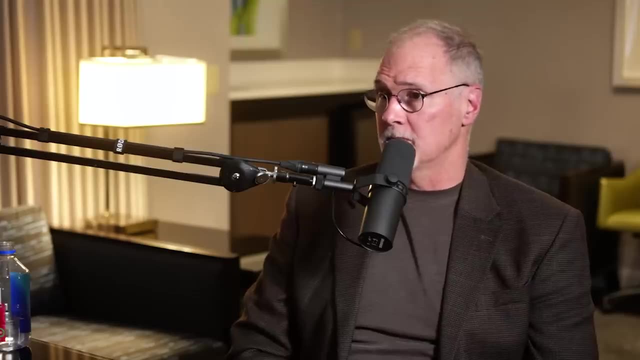 You ought to be able to just download that, And I think people besides Boston Dynamics will provide that- And we've actually built an API that lets people add these vision algorithms to Spot, And we're currently working with some partners who are providing that. 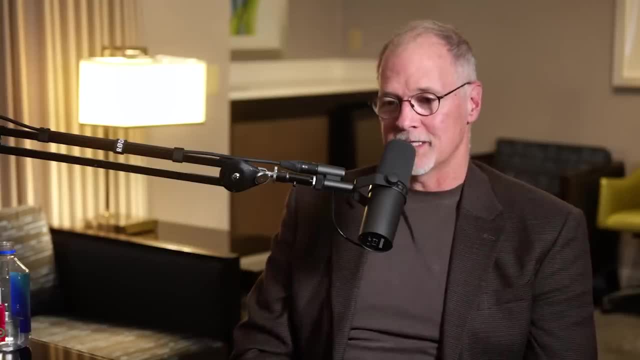 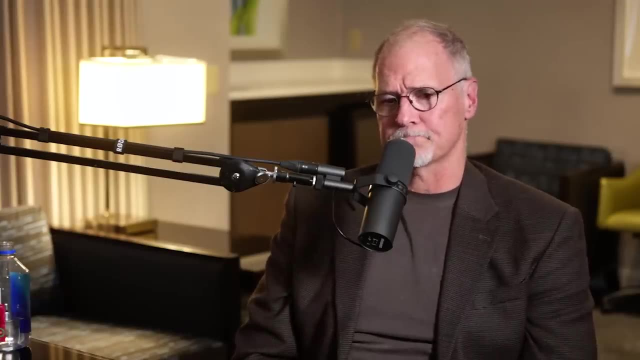 Levitas is an example of a small provider who's giving us software for reading gauges, And actually another partner in Europe, Reply, is doing the same thing. So we see that We see, ultimately, an ecosystem of providers doing stuff like that. 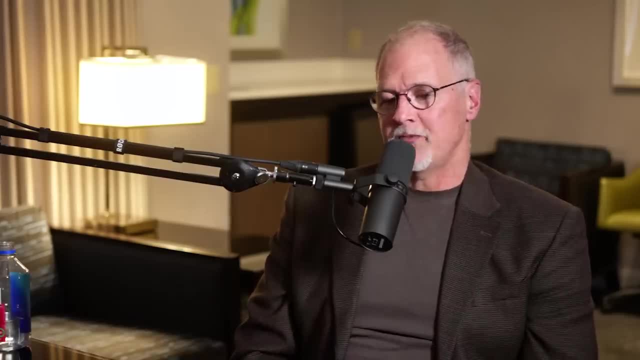 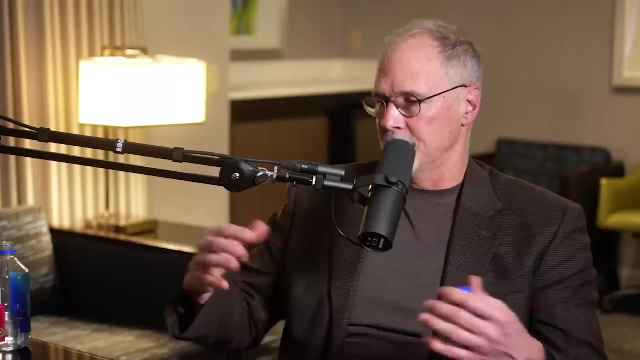 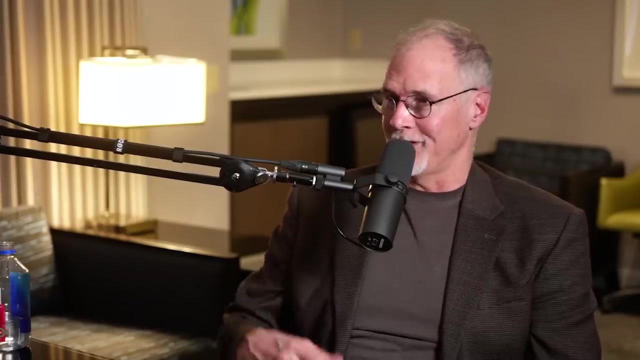 And I think, ultimately you might even be able to do the same thing with behaviors. So this technology will also be brought to bear on controlling the robot, the motions of the robot, And you know we're using reinforcement learning to develop. 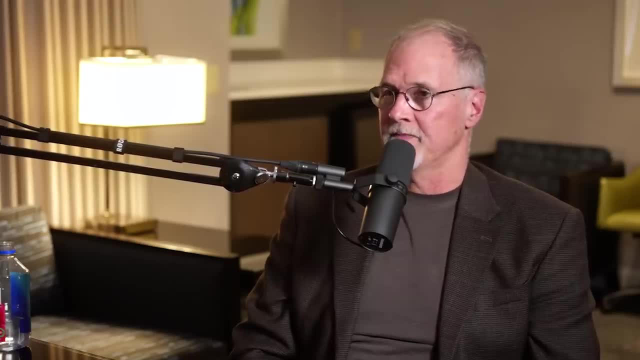 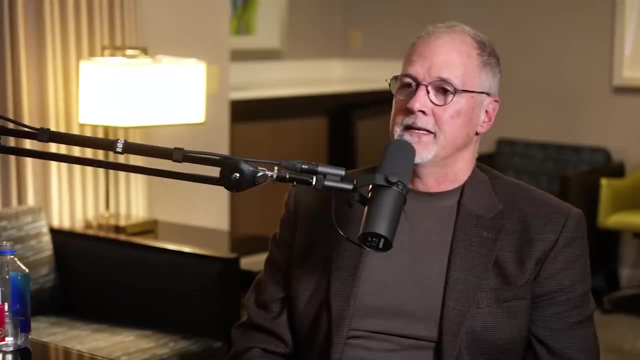 you know algorithms for both locomotion and manipulation, And ultimately this is going to mean you can add new behaviors to a robot you know quickly, And that could potentially be done outside of Boston Dynamics Right now. that's all internal to us. 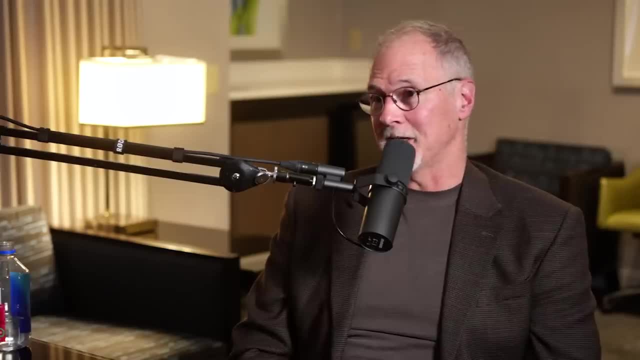 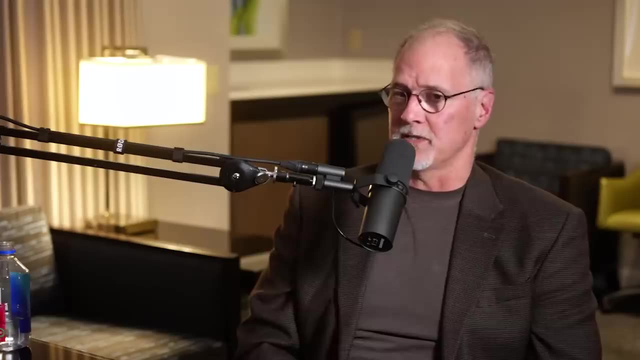 I think you need to understand at a deep level. you know the robot control to do that, But eventually that could be outside. But it's certainly a place where these approaches are going to be brought to bear In robotics. So reinforcement learning is part of the process. 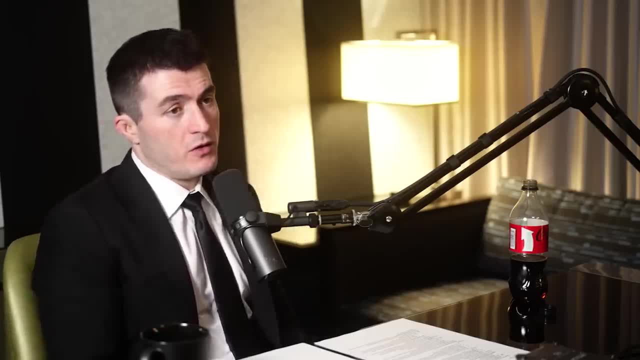 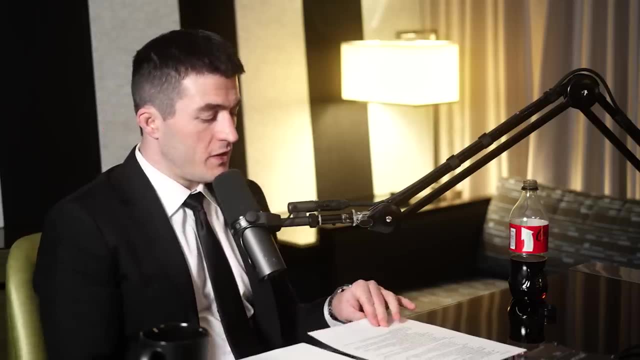 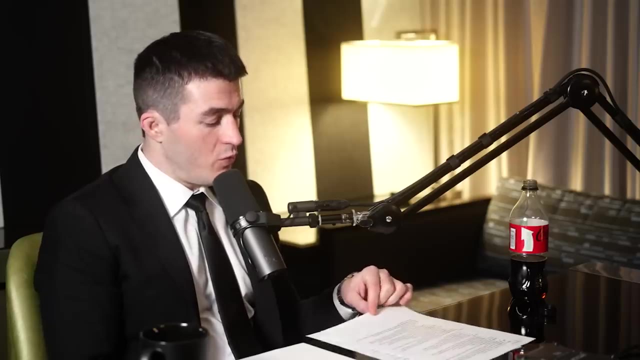 So you do use reinforcement learning? Yes, So there's increasing levels of learning with these robots? Yes, And that's for both for locomotion, for manipulation and for perception. Yes, Well, what do you think in general about all the exciting advancements? 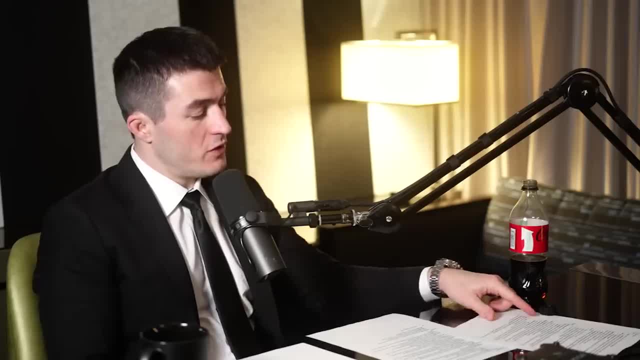 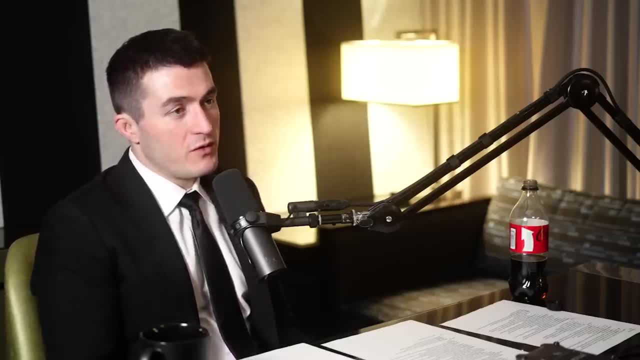 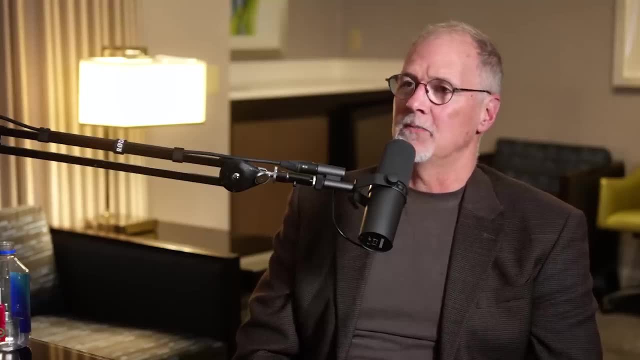 that are being provided to the players through the large language models that are being provided to the players, like GPT-4.. like GPT-4. Like everybody else, we're all you know. I'm surprised at how much, how far they've come. 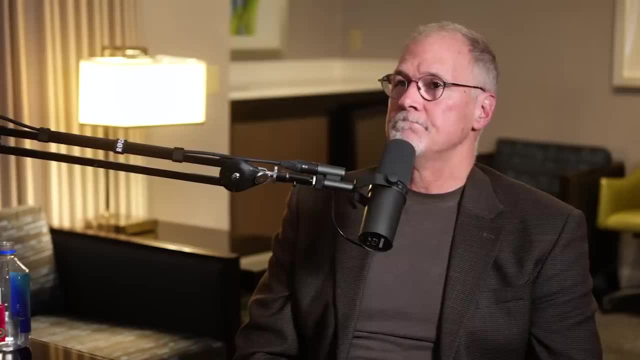 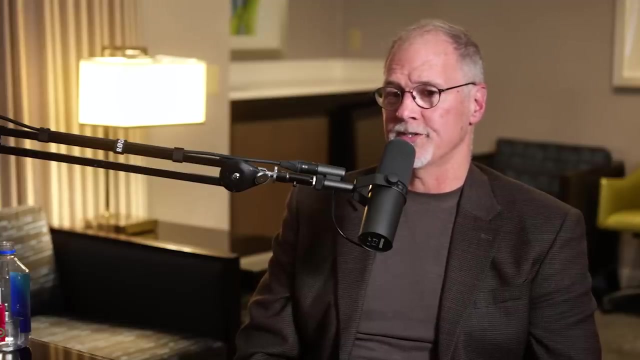 I'm a little bit nervous about the. there's anxiety around them, obviously, for I think good reasons right that disinformation is a curse, that's an unintended consequence of social media that could be exacerbated with these tools. So if you use them to deploy disinformation, it could be a real risk. 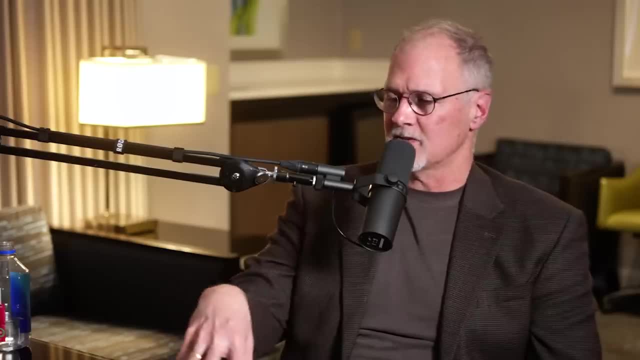 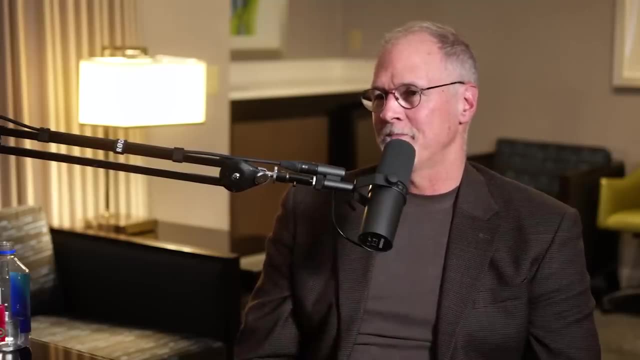 But I also think that the risks associated with these kinds of models don't have a whole lot to do with the way we're going to use them in our robots. If I'm using a robot, I'm building a robot to do a manual task of some sort. 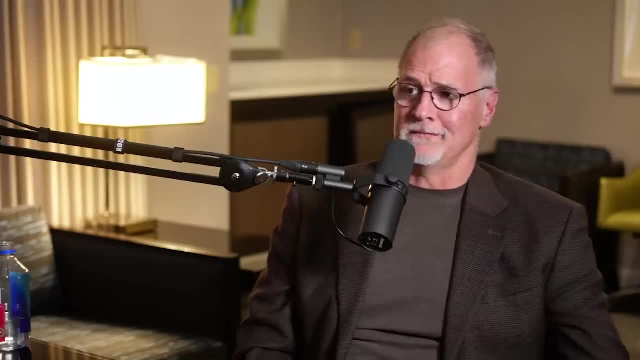 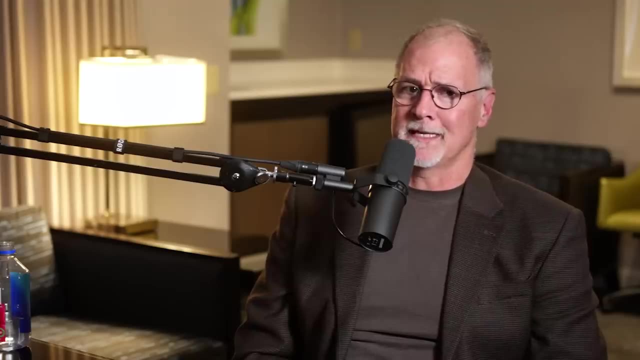 I can judge very easily. is it doing the task I asked it to? Is it doing it correctly? There's sort of a built-in mechanism for judging. is it doing the right thing? Did it successfully do the task? Yeah, physical reality is a good verifier. 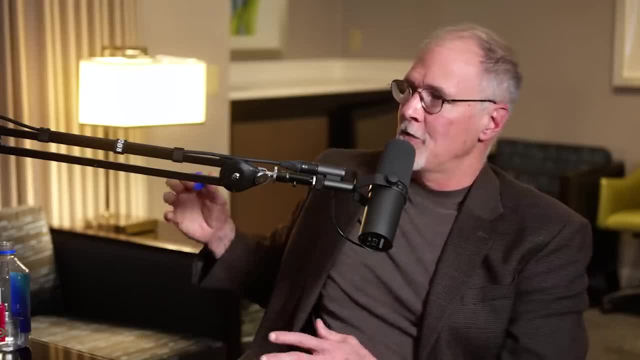 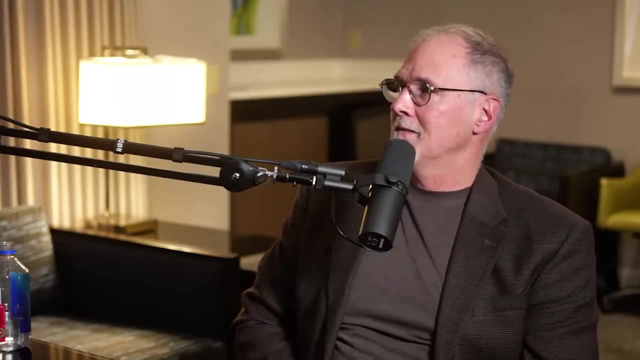 It's a good verifier. that's exactly it, Whereas if you're asking for yeah, I don't know if you're trying to ask a theoretical question in ChatGPT- it could be true or it may not be true, and it's hard to have that verifier. 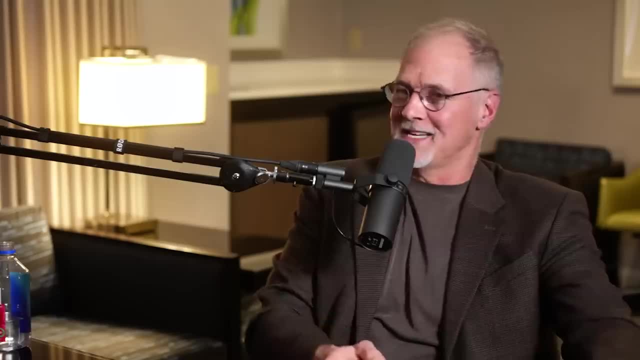 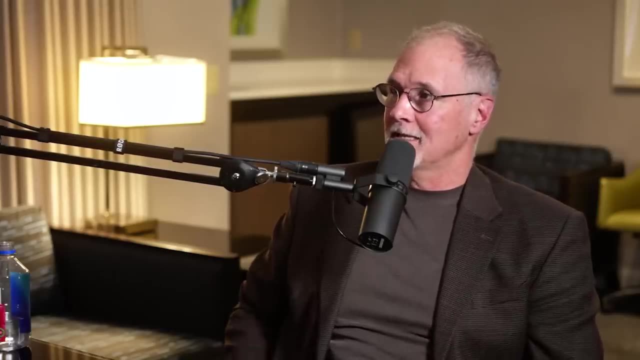 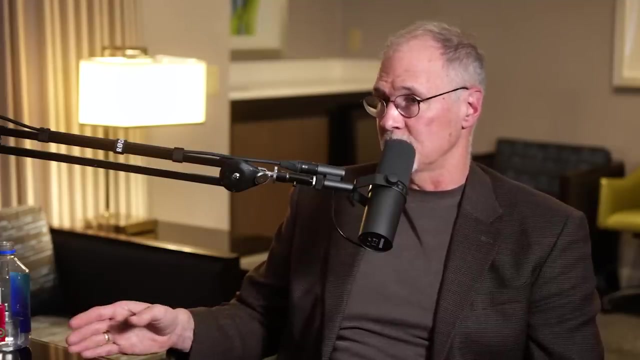 What is that truth that you're comparing against, Whereas in physical reality you know the truth, And this is an important difference, And so I'm not. I think there is reason to be a little bit concerned about you know how these tools- large language models- could be used. 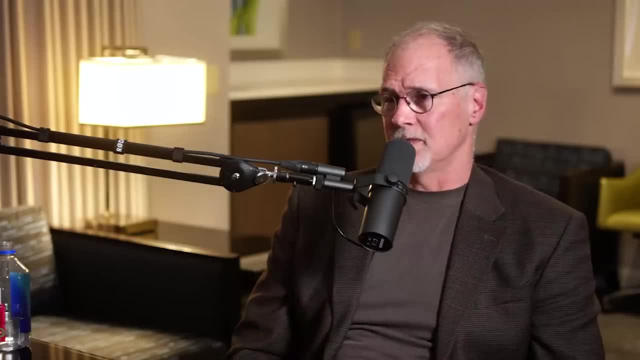 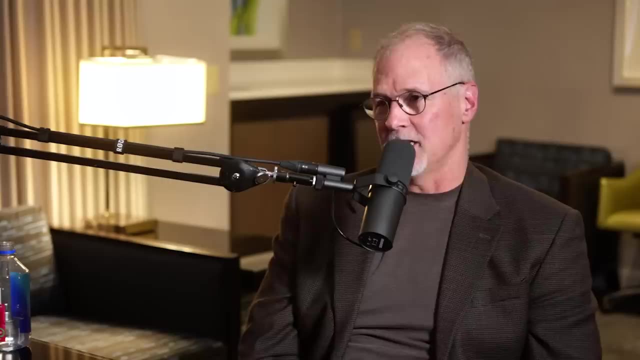 but I'm not. I'm not very worried about how they're going to be used well, how learning algorithms in general are going to be used on robotics. It's really a different application that has different ways of verifying what's going on. 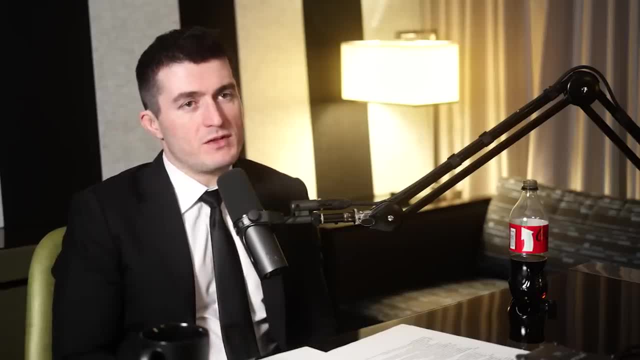 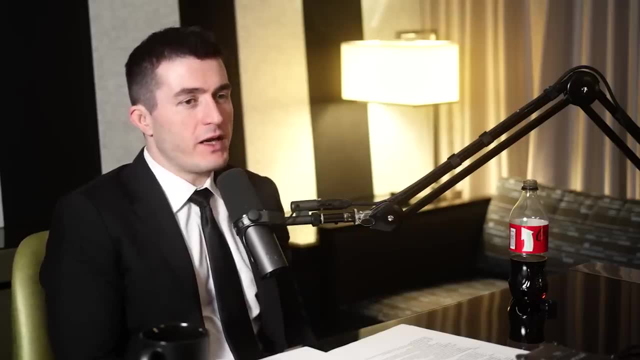 Well, the nice thing about language models is that I ultimately see. I'm really excited about the possibility of having conversations with Spot. Yeah, There's no, I would say, negative consequences to that, but just increasing the bandwidth and the variety of ways. 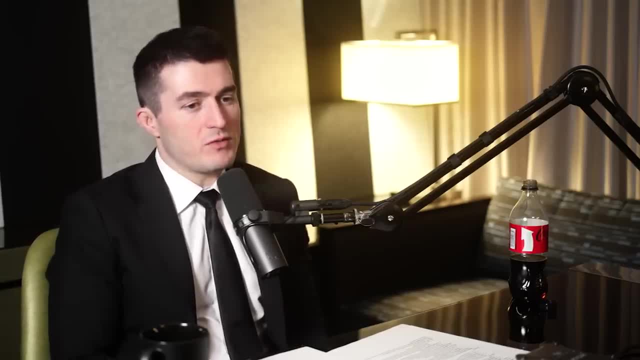 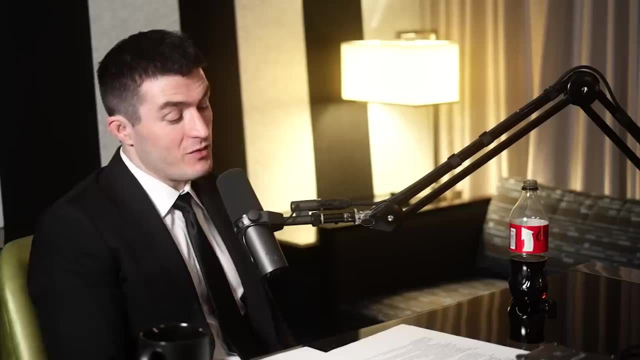 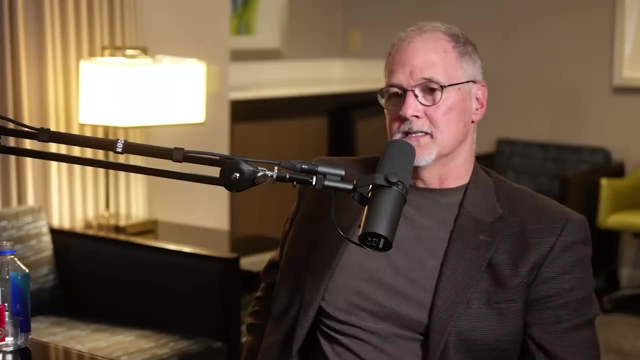 you can communicate With this particular robot, So you could communicate visually, you can communicate through some interface, and to be able to communicate verbally again with the beer and so on. I think that's really exciting. to make that much, much easier, We have this partner, Levitas, that's adding the vision algorithms for gauge reading for us. 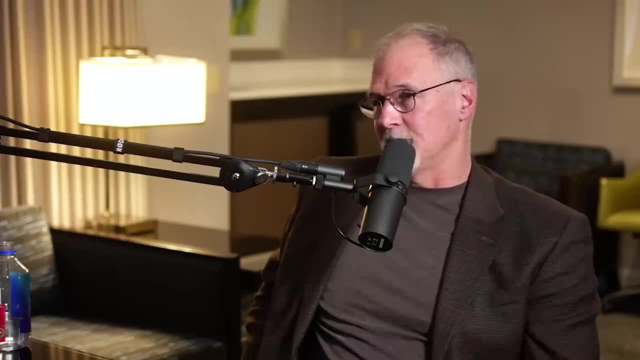 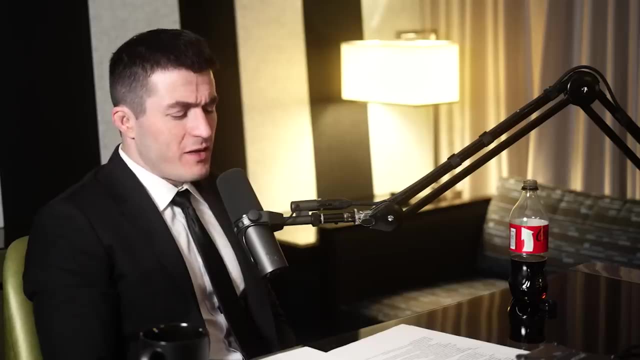 They just just this week I saw a demo where they hooked up, you know, a language tool to Spot and they're talking to Spot to give it commands. I love it. Yeah, Can you tell me about the Boston Dynamics AI Institute? 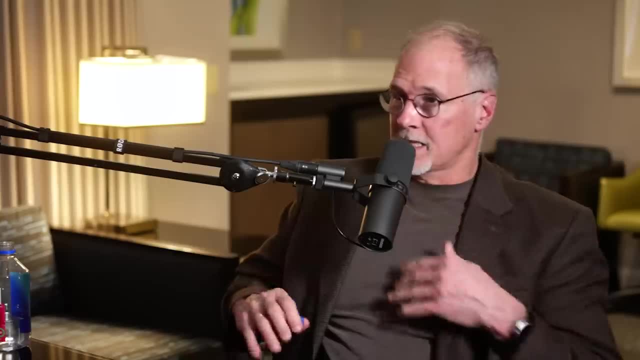 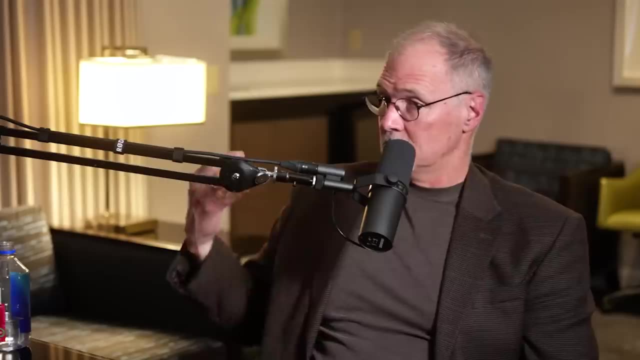 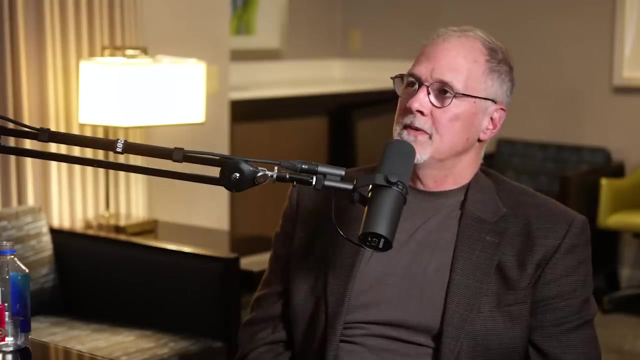 What is it and what is its mission? So it's a separate organization, the Boston Dynamics Artificial Intelligence Institute. It's led by Mark Rayburn, the founder of Boston Dynamics and the former CEO and my old advisor at MIT. Mark has always loved the research, the peer research, without the confinement or demands of commercialization. 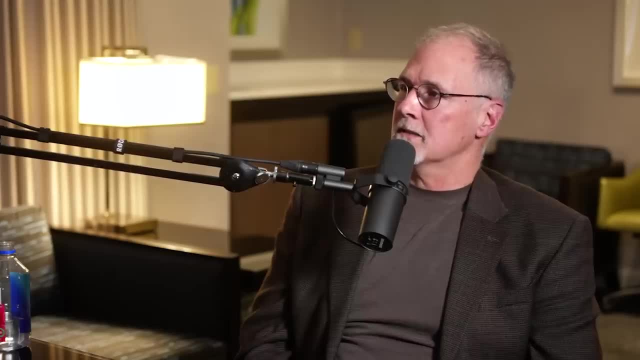 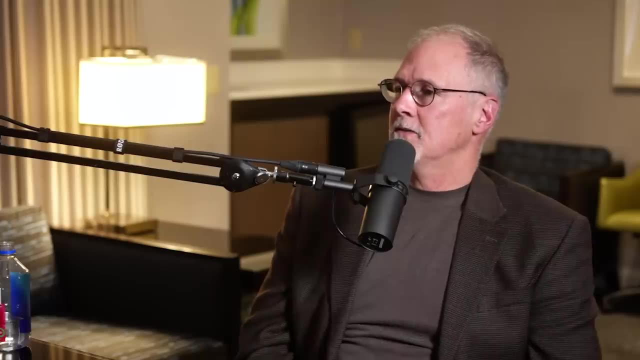 Mm-hmm, And he wanted to continue to, you know, pursue that unadulterated research And so suggested to Hyundai that he set up this institute, and they agree that it's worth additional investment to kind of continue pushing this forefront. 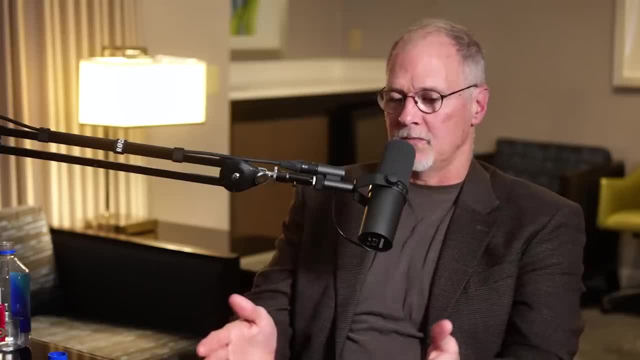 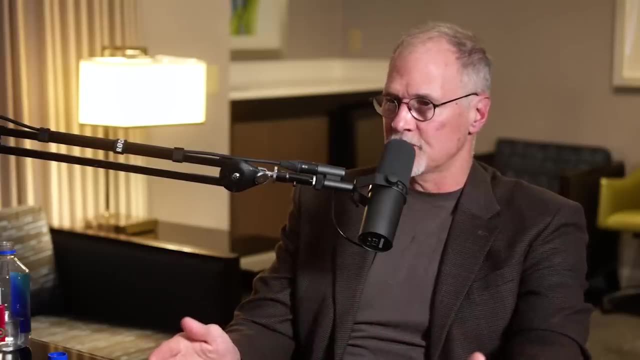 And we expect to be working together where you know Boston Dynamics is going to both commercialize and do research. But the sort of time horizon of the research we're going to do is, you know, in the next, let's say, five years. you know, what can we do in the next five years? 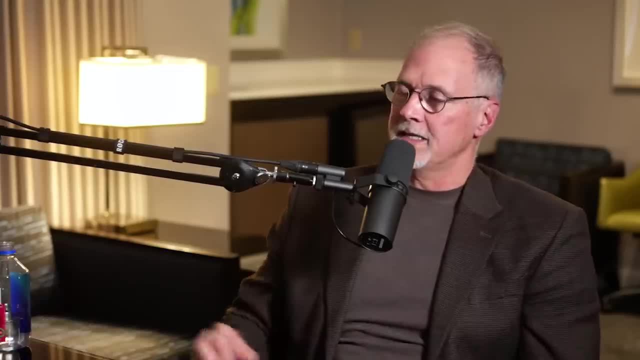 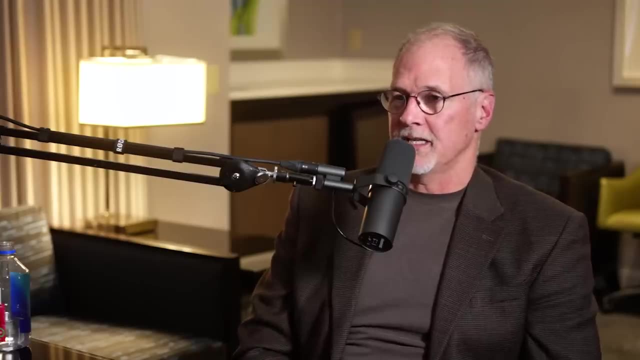 Let's work on those problems And I think the goal of the AI Institute is to work even further out. Certainly you know the analogy of of legged locomotion. again, when we started that that was a multi-decade problem. 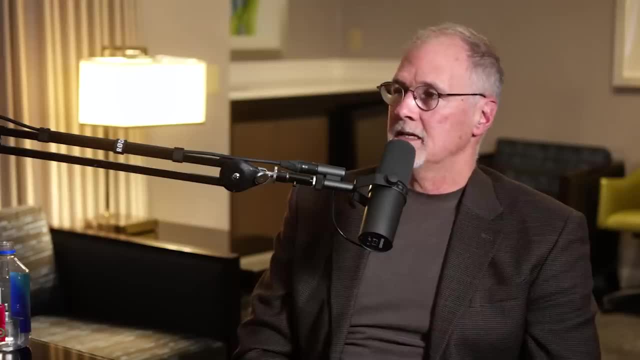 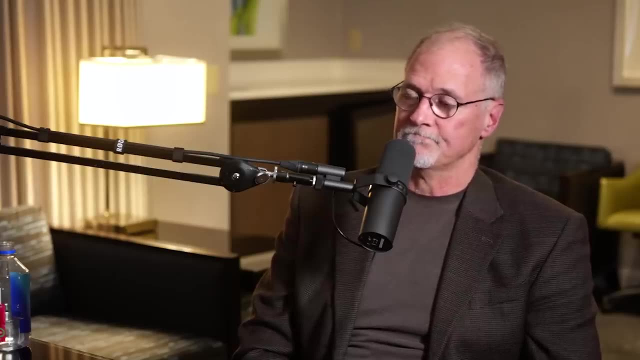 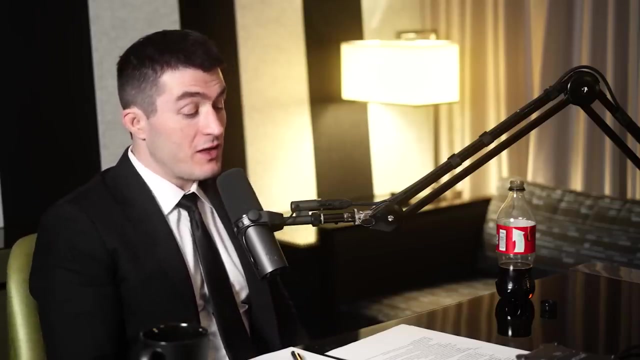 And so I think Mark wants to have the freedom to pursue really hard over the horizon problems, And that's that'll be the goal. The Institute: So we mentioned some of the dangers, of some of the concerns about large language models. That said, you know there's been a long running fear of these embodied robots. 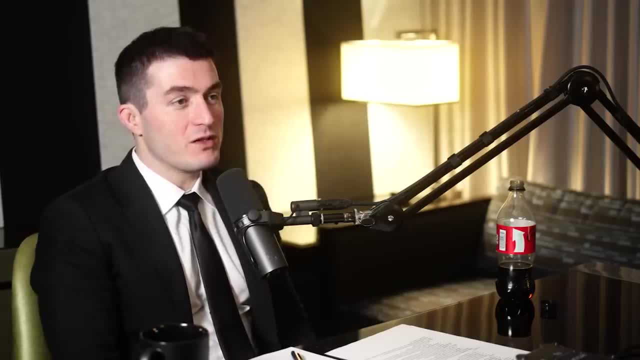 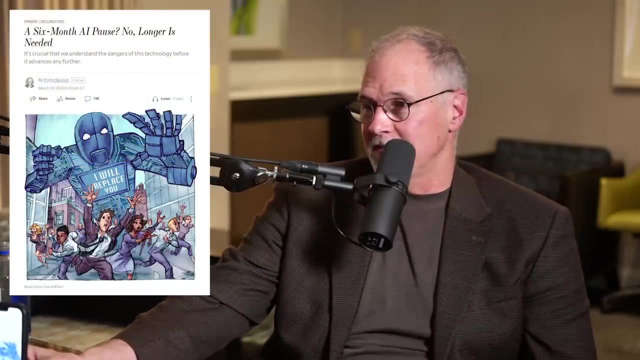 Why do you think people are afraid of legged robots? Yeah, I wanted to show you this, This, so this. this is a Wall Street Journal and this is all about chat. GPT, right, But look at the picture, Yeah. 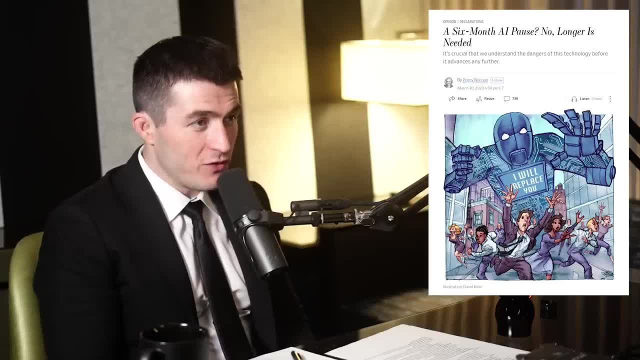 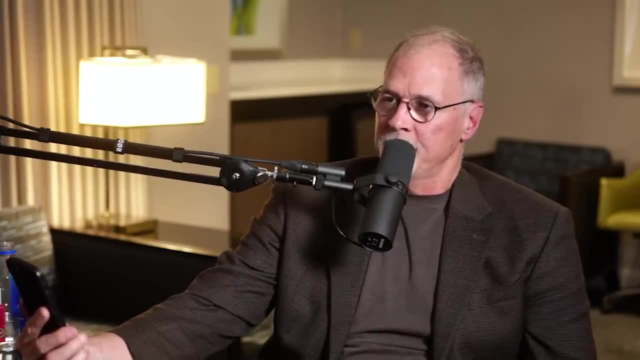 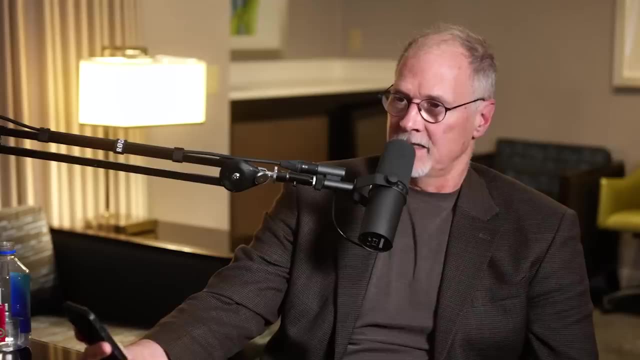 It's a humanoid robot That's saying I will replace. That's saying that looks scary and it says I'm going to replace you. Yeah, And so the humanoid robot is sort of is the embodiment of this chat GPT tool, that there's reason to be a little bit nervous about how it gets deployed. 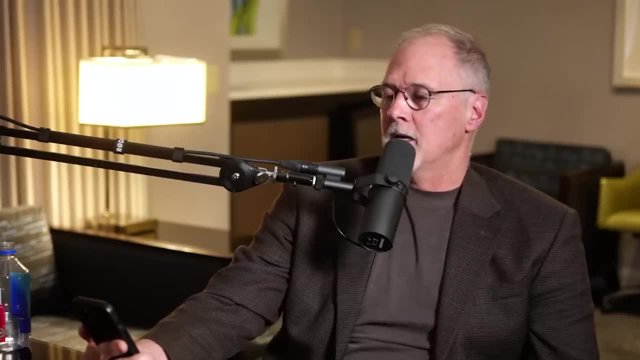 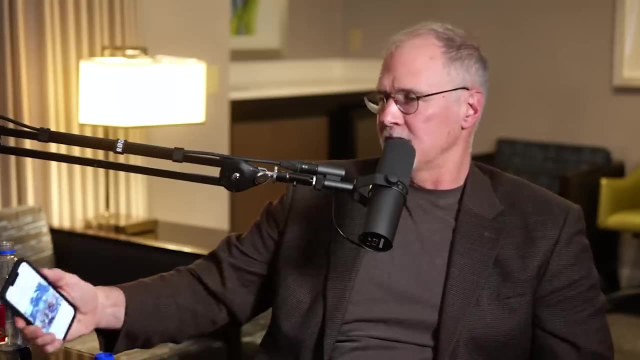 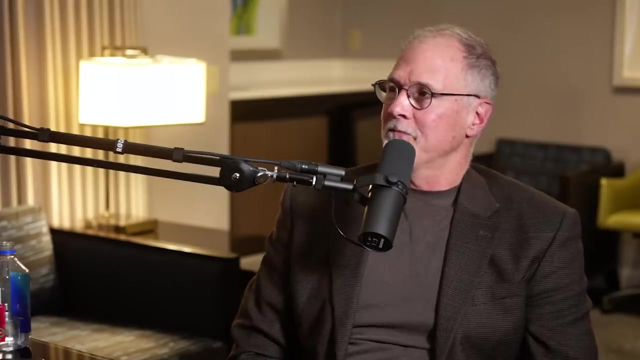 Yeah, So I'm nervous about that connection. It's unfortunate that they chose to use a robot as that embodiment, for, as you and I just said, there's big differences in in This. but uh, people are afraid because we've been taught to be afraid for over a hundred years. 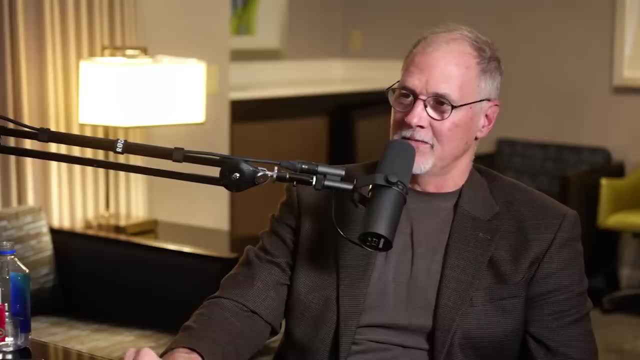 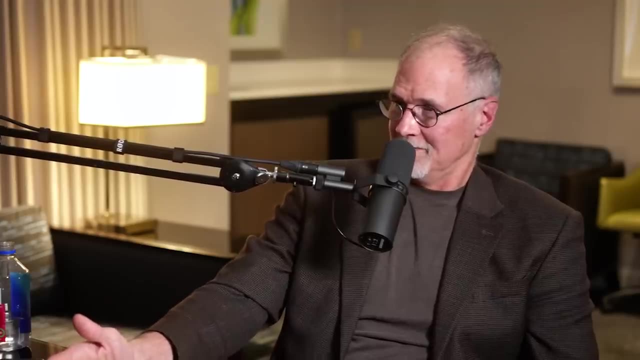 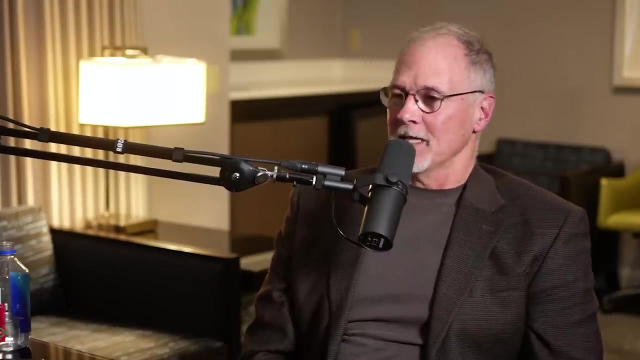 So you know, the word robot was developed by a playwright named Carol Chapek in 1921 to check playwright Rossum's universal robots. And in that first depiction of a robot, the robots took over the end of the story. and you know, people love to be afraid. 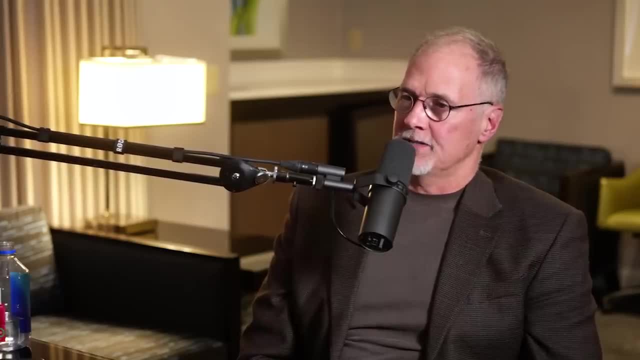 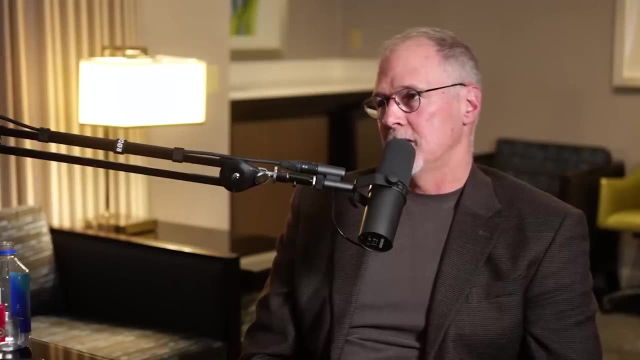 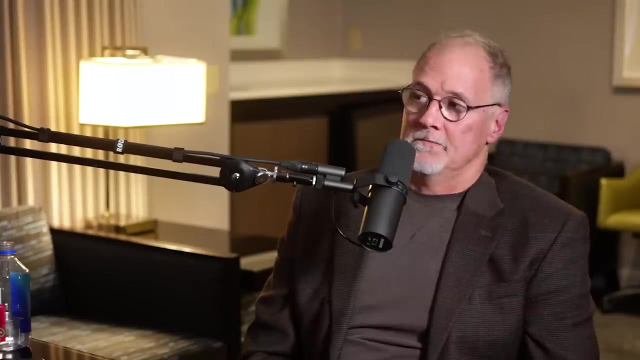 And so we've been entertained by these stories For a hundred years. But I- and I think that's as much why people are afraid as anything else is- we've been sort of taught that this is the logical progression through fiction. Um, I think it's fiction. 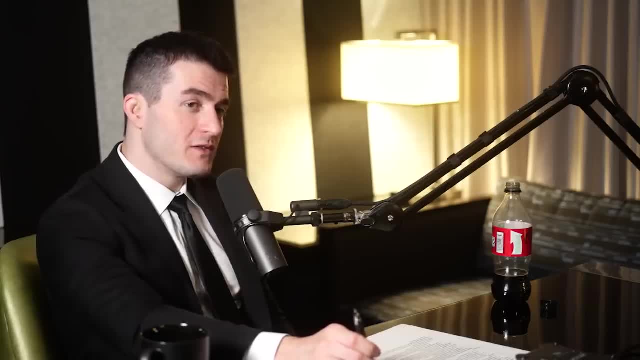 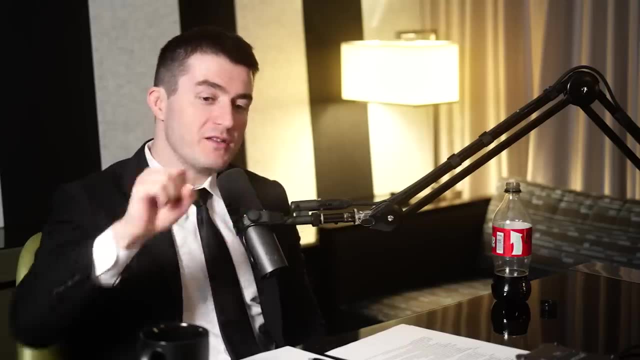 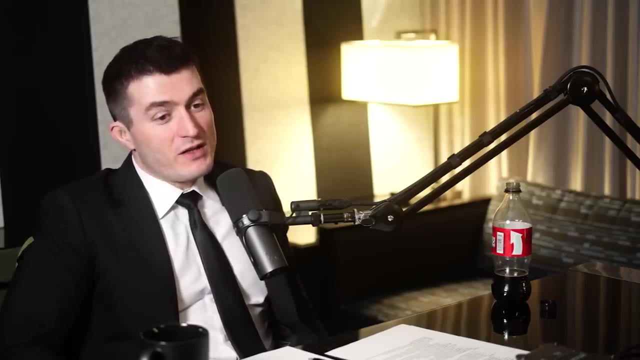 I think, uh, what people more and more will realize, just like you said, that the threat- like say, you have a super intelligent AI embodied in a robot- That's much less Threatening because it's visible, it's verifiable, it's right there in physical reality. 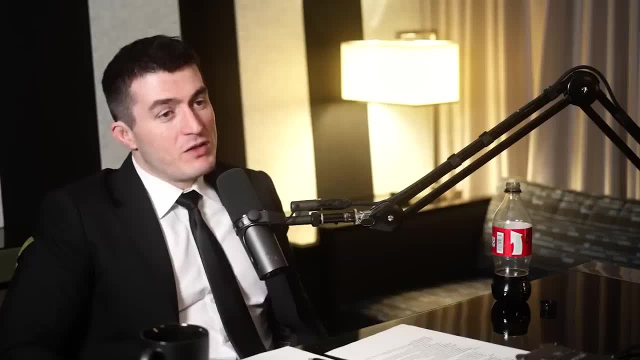 And we humans know how to deal with physical reality. I think it's much scarier, when you have arbitrary scaling of intelligent AI systems in the digital space, that they could, uh, pretend to be human. So robot spot is not going to be pretend. it can pretend it's human all at once. 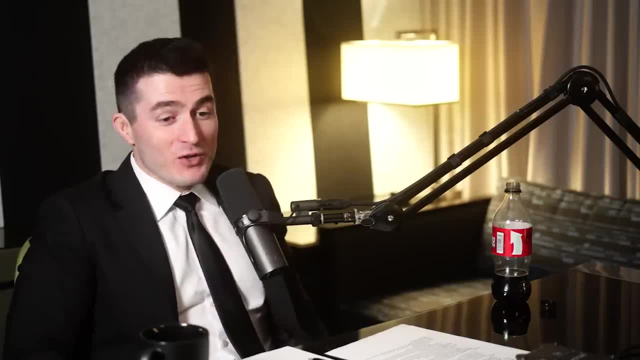 It could tell you. you could put chat GPT on top of it, but you're going to know it's not human Cause. you have a contact with physical reality and you're going to know whether or not it's doing what you asked it to do. 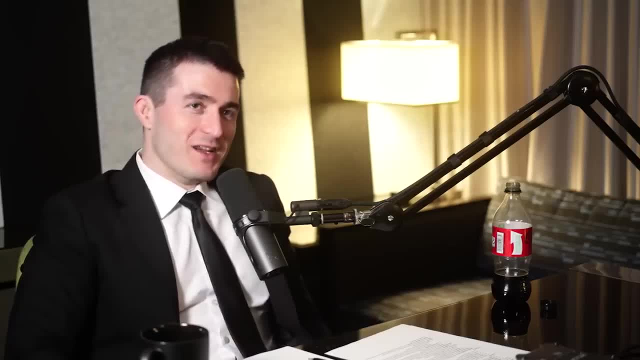 Yeah, Like it's not going to like. if it let, I mean, I'm sure you can start just like a dog uh lies to use. Like I didn't. I wasn't part of tearing up that couch. 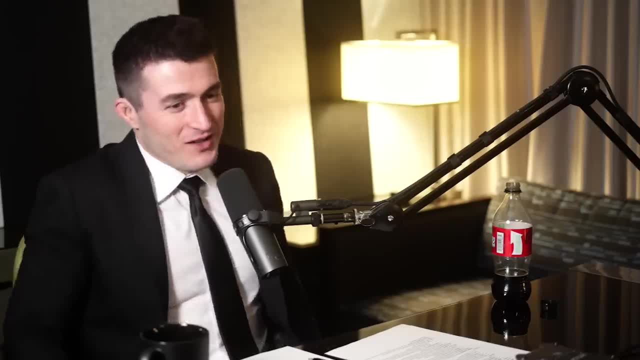 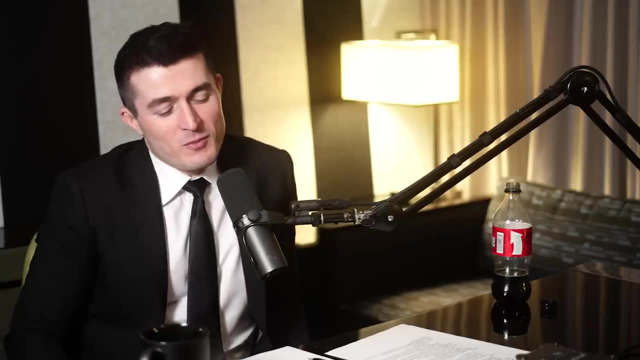 So spot can try to lie that, like you know, it wasn't me that spilled that thing. but you're going to kind of figure it out. eventually It's, but if it happens multiple times, you know, uh, but I think that humanity has figured out how to make machines. 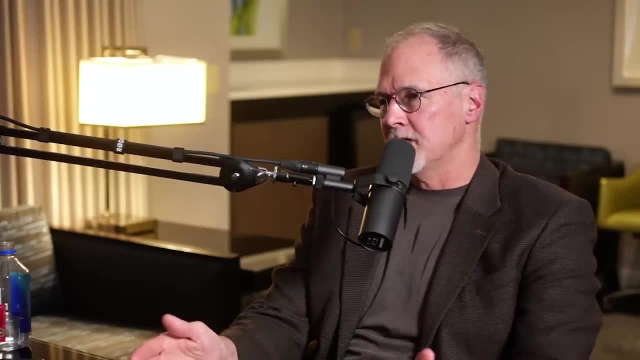 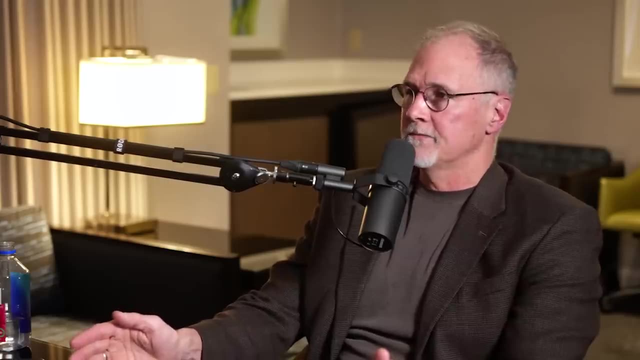 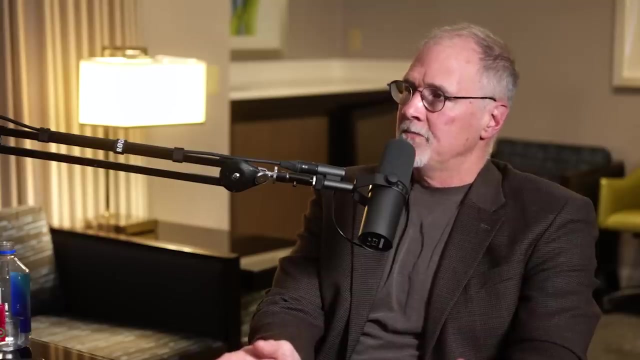 Safe and there's, you know, the regulatory environments and certification uh protocols that we've developed in order to figure out how to make machines safe. We don't know, we and don't have that experience with software that can be propagated worldwide in an instant. 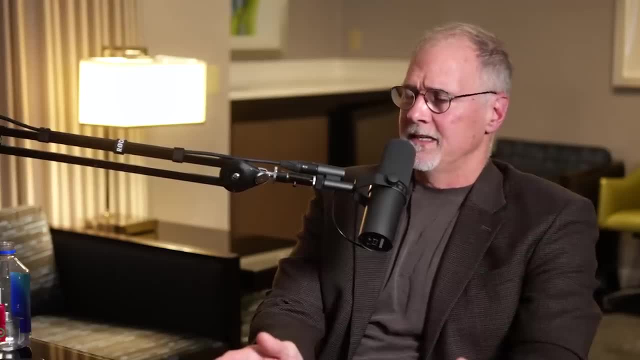 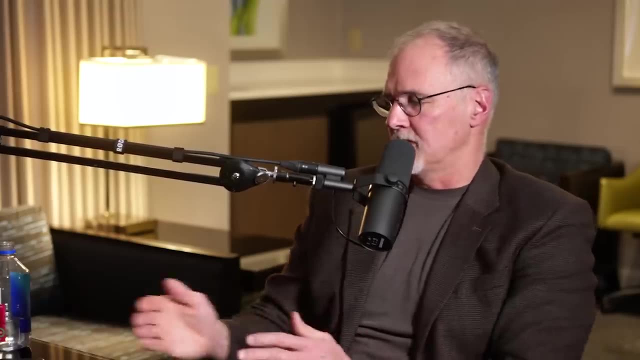 And so I think we needed to develop those protocols and those tools, And so, uh, that's work to be done, but I don't think the fear Of that and that work should necessarily impede our ability to now get robots out, because, again, I think I think we can judge when a robot's being safe. 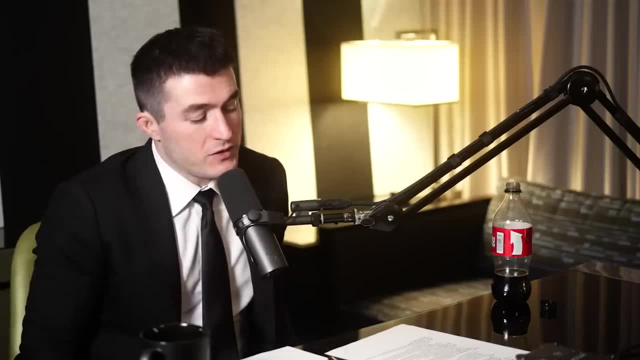 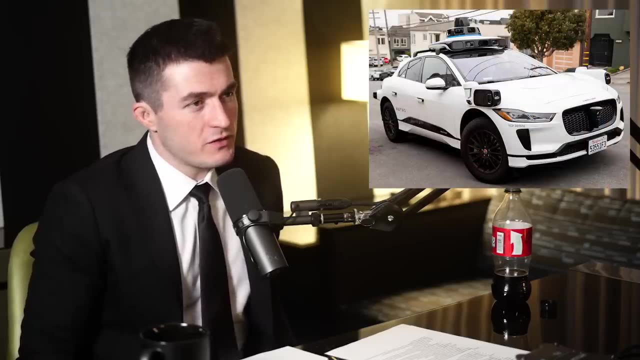 So and again, just like in that image, there's a fear that robots will take our jobs. I just um, I took a ride. I was in San Francisco, I took a ride in the Waymo vehicles and autonomous vehicle. 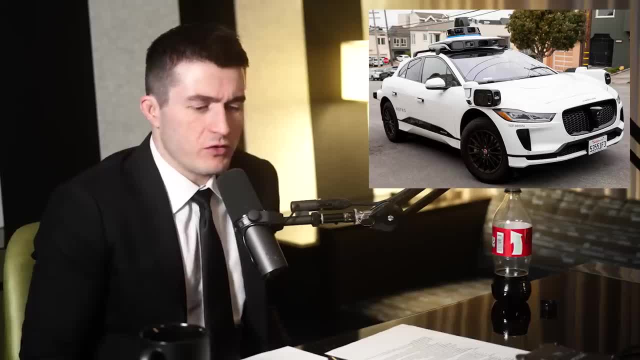 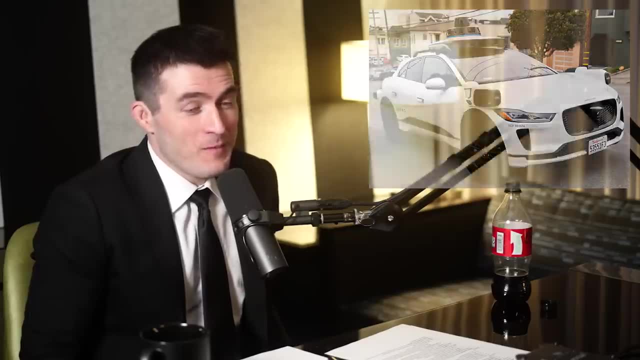 And uh- I've done it several times- They're, uh, they're doing incredible work over there, Uh, but uh, people flicked it off the car. So that's a long story of what the psychology of that is. 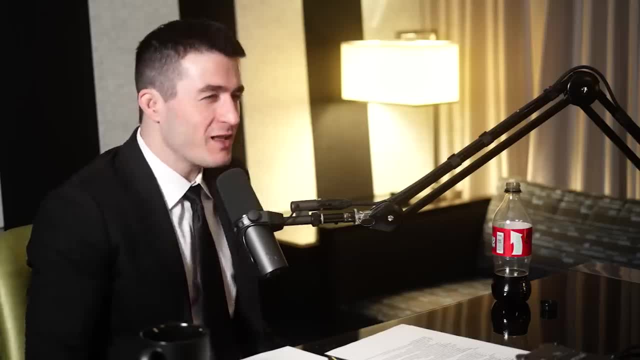 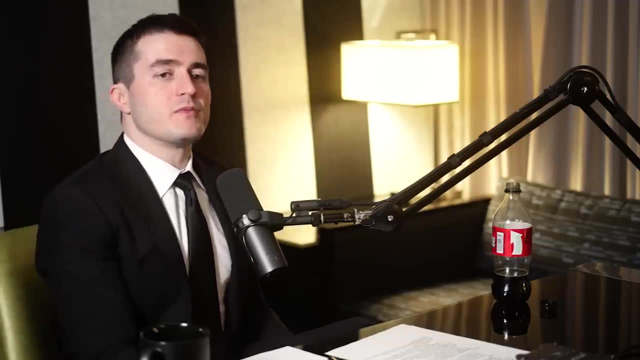 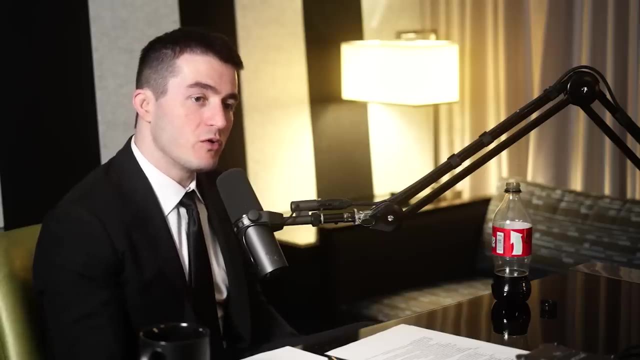 It could be maybe big tech or what, I don't know exactly what they're flicking off, but there is an element of like these robots are taking our jobs or or irreversibly transforming society such that it will have economic impact And the little guy will be: uh, would lose a lot, would lose their wellbeing. 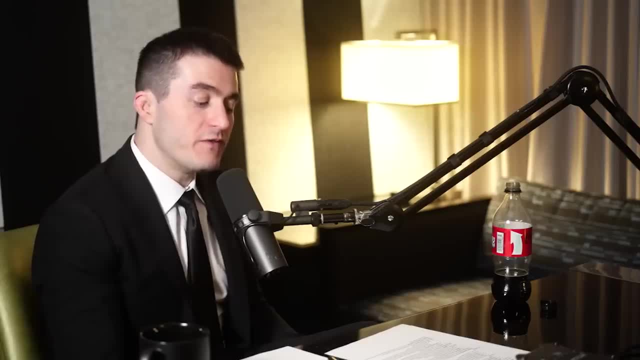 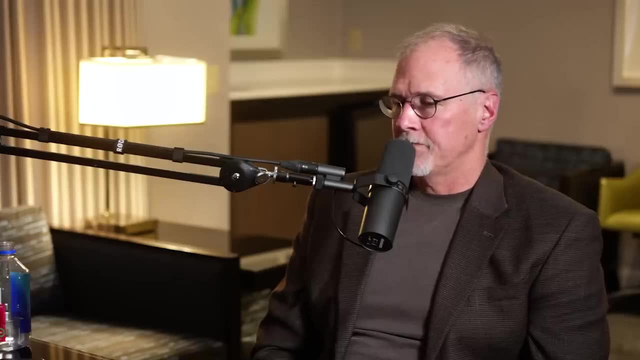 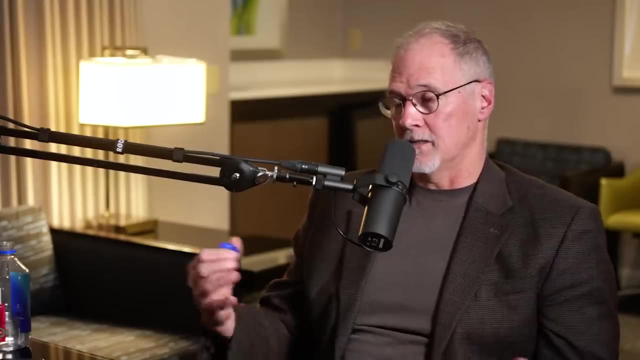 Is there something to be said about, um, the fear that That's, robots will take our jobs? You know, at every um significant technological transformation, uh, there's been fear of, you know, an automation anxiety that, uh, it's. it's going to have a broader impact than than we expected. 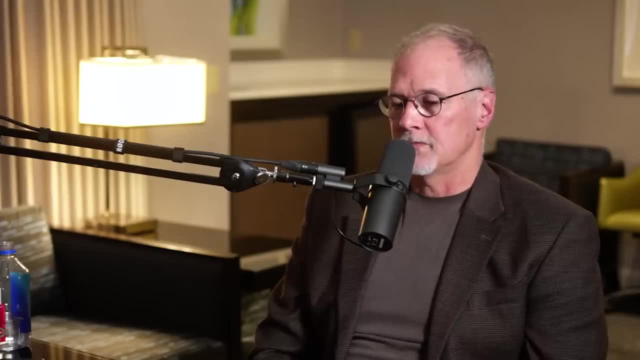 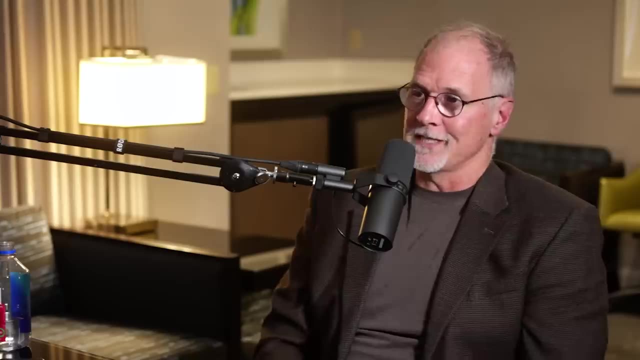 And there there will be- uh, you know, jobs will change Um sometime in the future. we're going to look back at people who manually unloaded these boxes from Trailers and we're going to say: why did we ever do that manually? 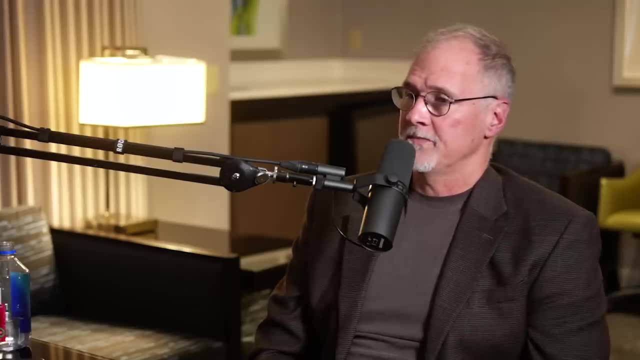 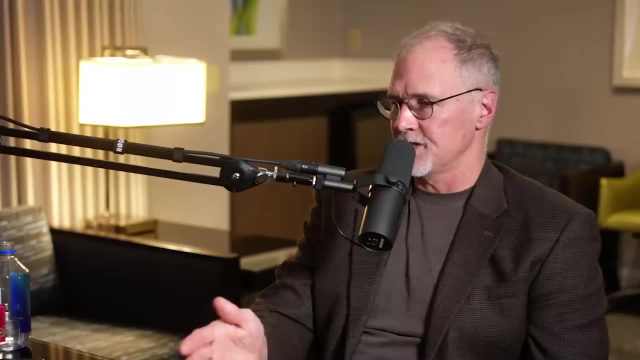 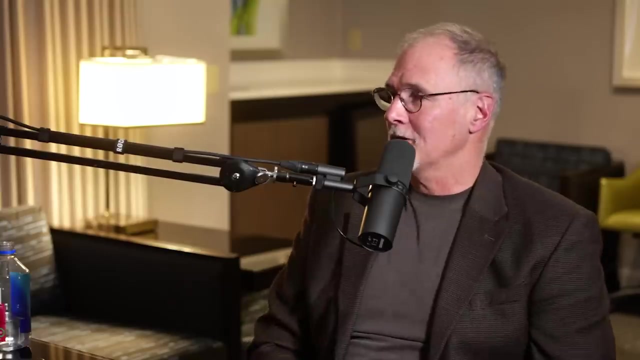 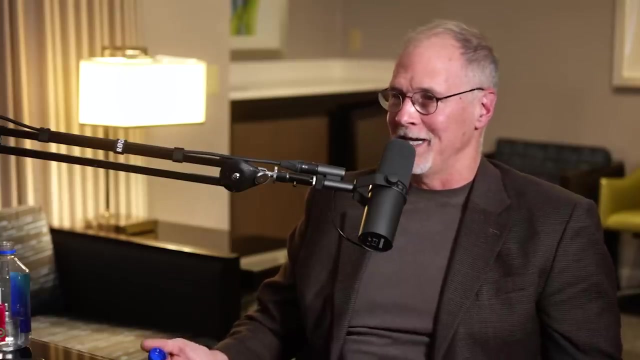 But there's a lot of people who are doing that job today, that it could be impacted. Um, but I think the reality is, as I said before, we're going to build the technology so that those very same people can operate it, And so I think there's a pathway to upskilling and operating, just like, look, we used to farm with hand tools and now we farm with machines, and nobody has really regretted that transformation. 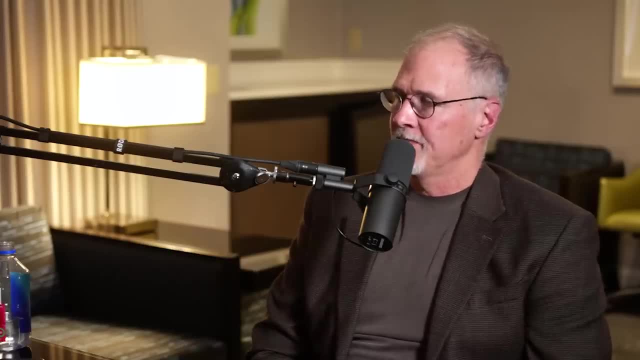 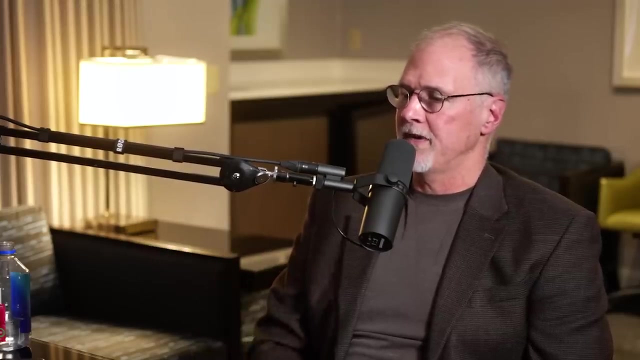 And I think the same can be said For a lot of manual labor that we're doing today. And on top of that, you know, look we're. we're entering a new world where dem, where demographics are going to have strong impact on economic growth and the you know, the advanced, uh, the first world is losing population quickly. 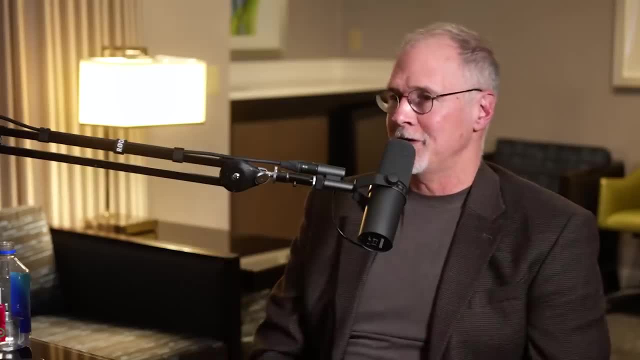 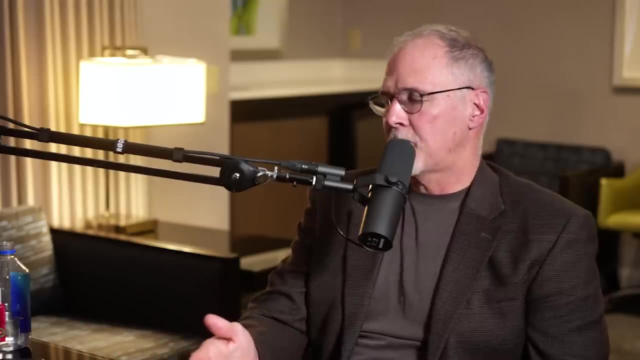 Um, in Europe they're worried about hiring enough people just to keep the logistics supply chain going. Okay, Okay, Okay, Okay, Okay, Okay- And you know part of this is the response to COVID and everybody's sort of thinking, thinking back what they really want to do with their life. 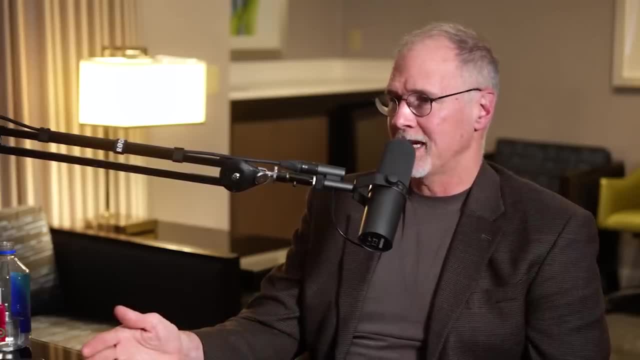 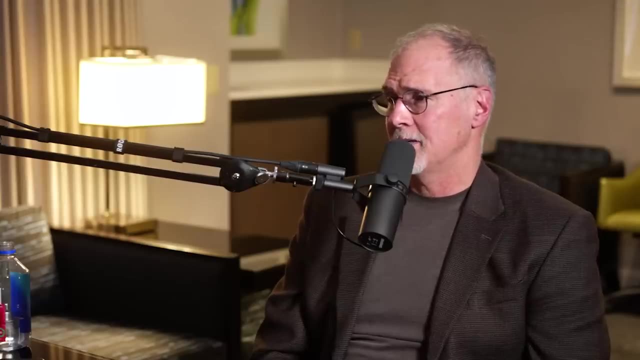 But these jobs are getting harder and harder to fill And I just I'm hearing that over and over again. So I think, frankly, this is the right technology at the right time, um, where we're going to need some of this work to be done and we're going to want tools to enhance that productivity. 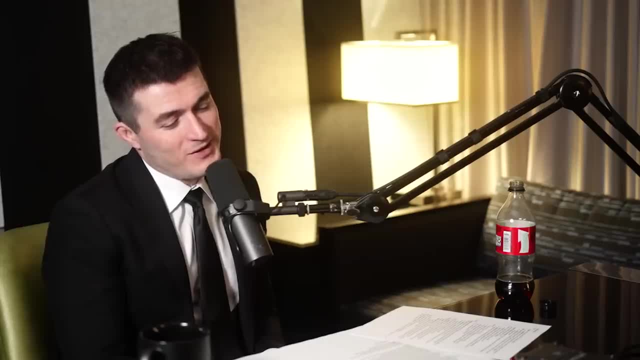 And the scary impact. I think again: Uh, GPT comes to the rescue in terms of being much more terrifying. Uh, the scary, scary impact of, basically so I I'm a, I guess, a software person, so I program a lot. 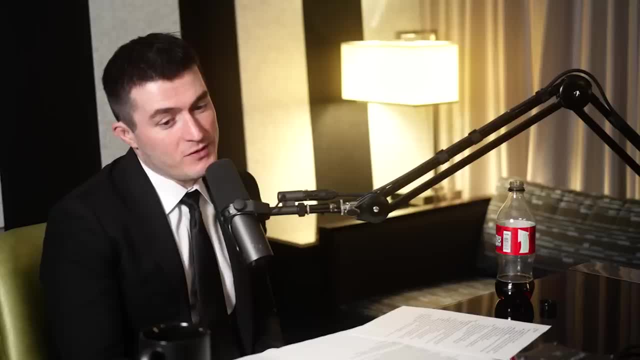 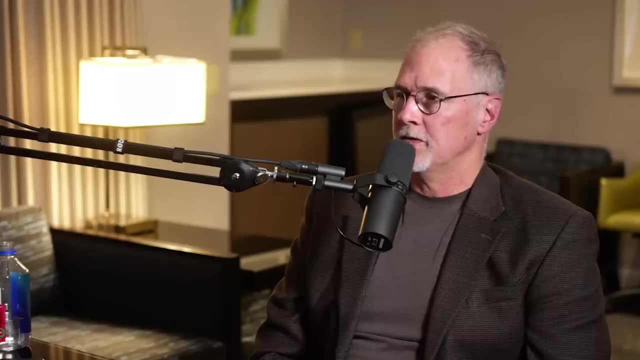 And the fact that people like me can be easily replaced, uh, by GPT. that's going to have uh Well and a lot. you know, anyone who deals with texts and writing a draft proposal might be easily done with a chat GPT. 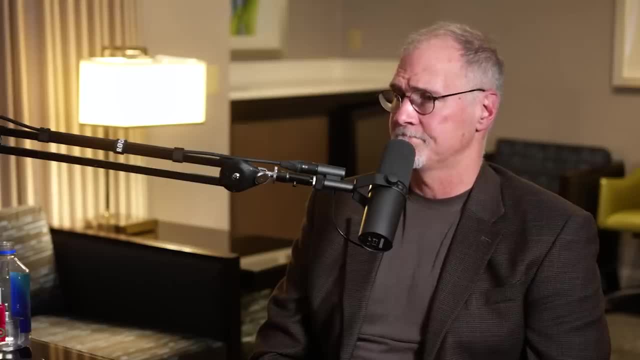 Yeah, consultants, journalists, um, everybody is sweating. But on the other hand, you also want it to be right, And they don't know how to make it right yet. But it might make a good starting point for you to iterate. 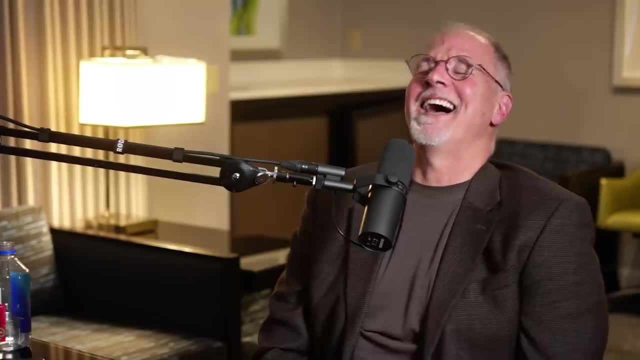 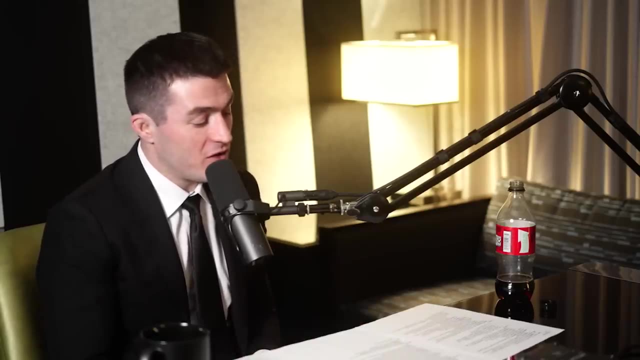 Boy, do I have to talk to you about modern journalism? That's another conversation altogether. But, yes, uh, more right than the average. uh, uh, this the the medium, I mean journalists. yes, Um, you spearheaded the NT weaponization letter. uh, Boston Dynamics has. 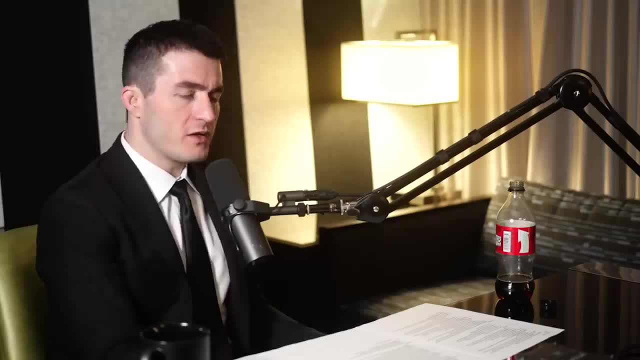 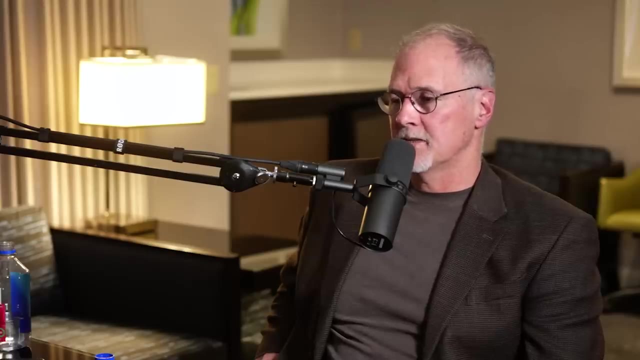 Can. can you describe uh what that letter states and the general uh topic of the use of robots in war? We uh authored a letter and then got several leading uh robotics companies around the world, including, you know, Unitree and 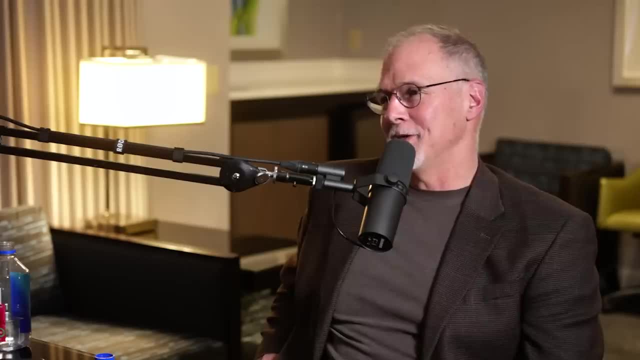 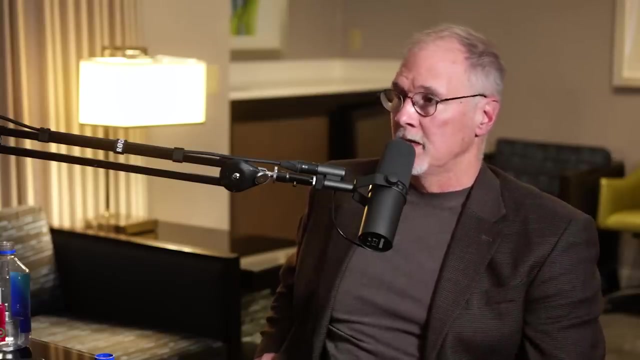 China and um agility uh here in the United States and um animal and in Europe and you know some others- to uh co-sign a letter that said we won't put weapons on our robots, And part of the motivation there is, you know, as these robots start to become commercially available. you can see videos online of people who've gotten a robot and strapped a gun on it. 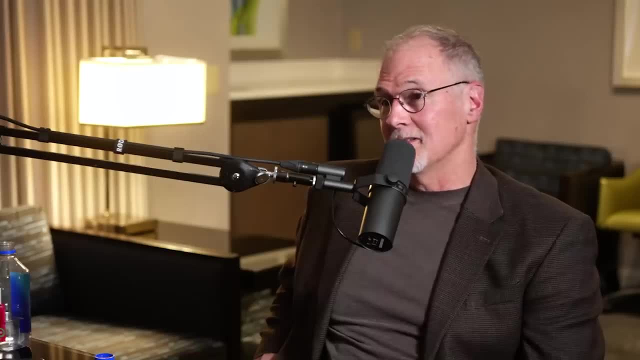 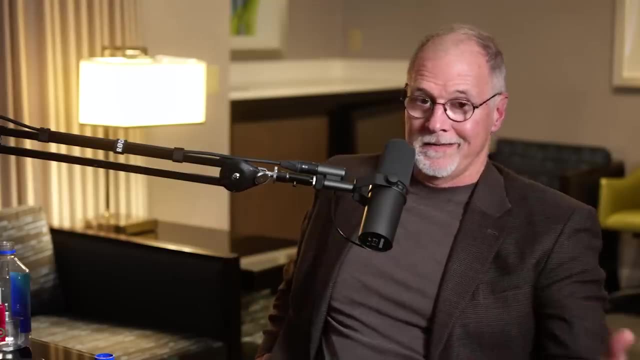 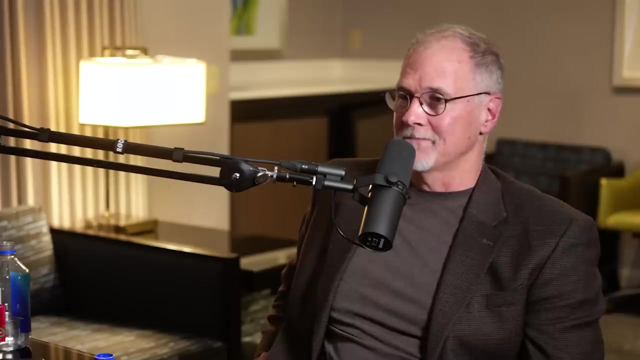 Yeah, And that they can, you know, operate the gun remotely while driving the robot around. And so having a robot that has this level of mobility, um, and that can easily be configured in a way that could harm somebody from a remote operator, is justifiably a scary thing. 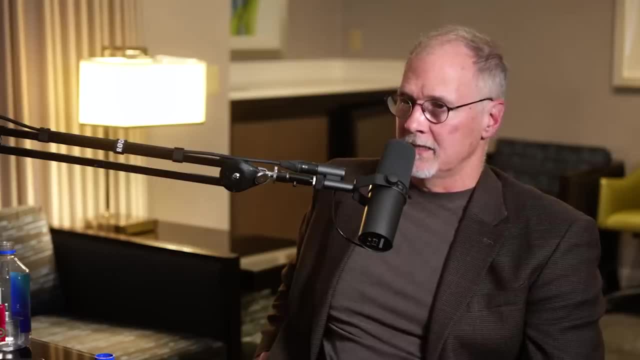 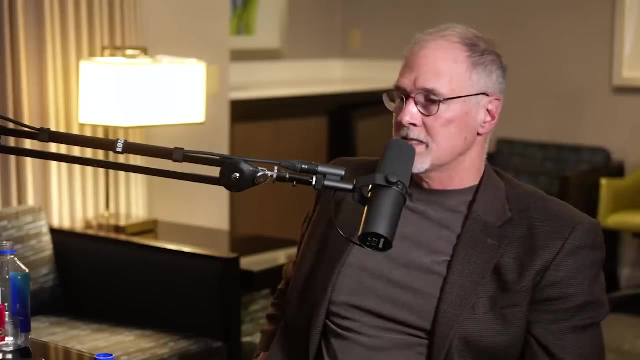 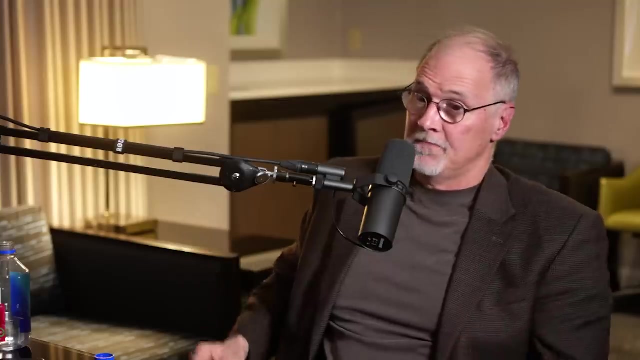 And so we felt like it was important to draw a bright line there and say we're not going to allow this for, um you know, reasons that we think ultimately It's better for the whole industry if it is, if it grows in a way where, uh, robots are ultimately going to help us all and make our lives more fulfilled and productive. but, by goodness, you're going to have to trust the technology to let it in. 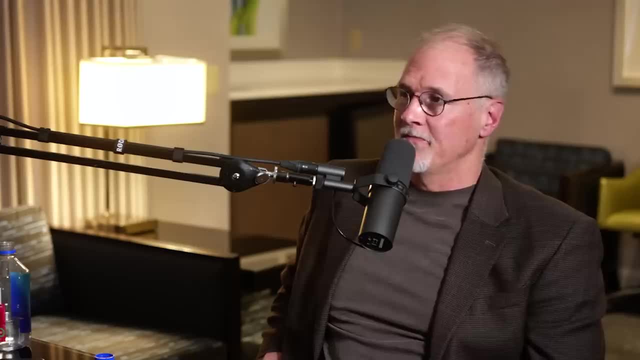 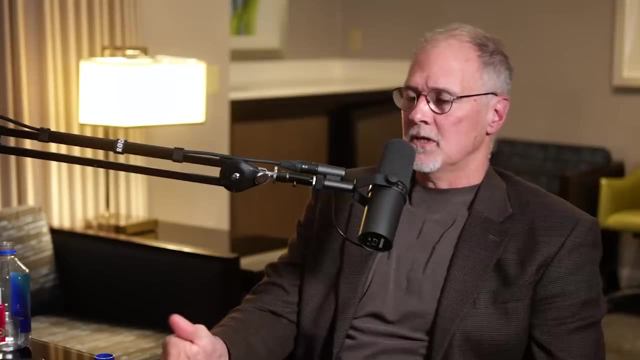 And if and if you think the robot's going to harm you, that's going to, that's going to hurt and impede the growth of that industry. So we thought it was important to to draw a bright line And Uh, and then publicize that. 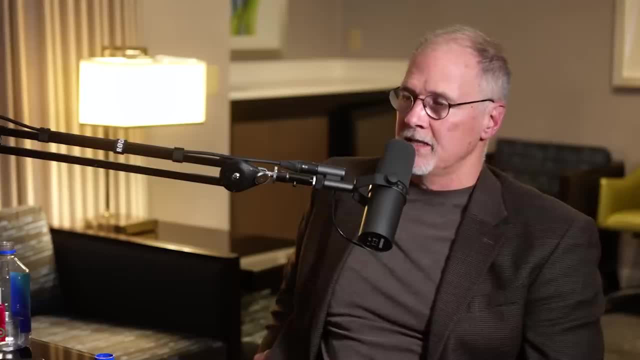 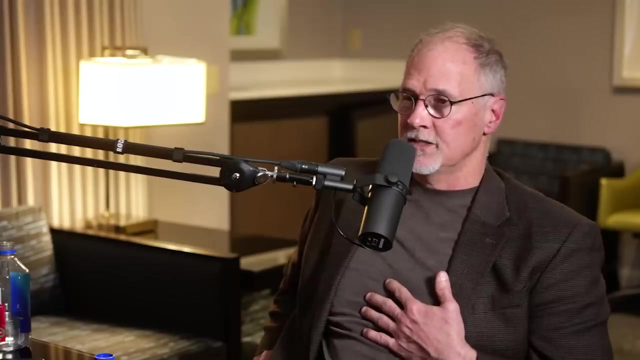 And- and our plan is to you know- begin to engage with uh lawmakers and regulators. Let's figure out what the rules are going to be around the use of this technology Um and use our position as leaders in this industry and technology um to help force that issue. 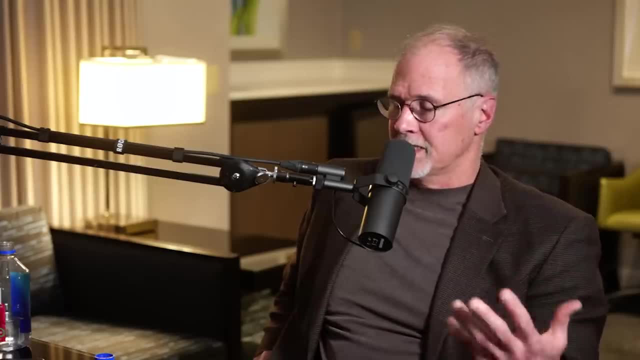 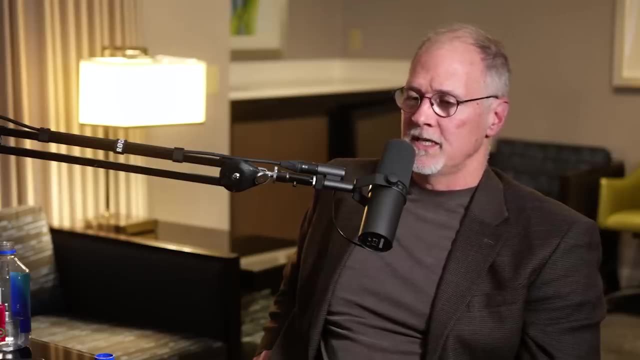 Uh, and so we are. in fact, I have a, I have a policy, You know, director at, at my company, whose job it is to engage with the public, to engage, engage with uh interested parties and and including regulators, to to sort of begin these discussions. 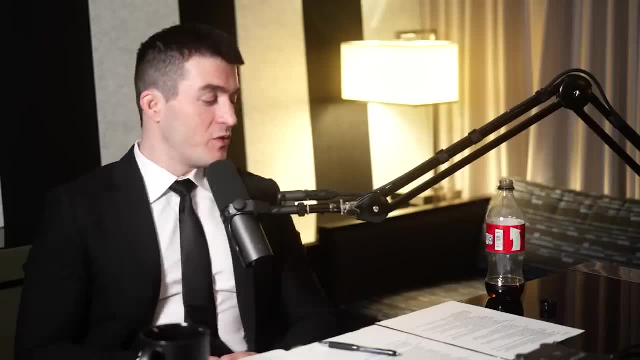 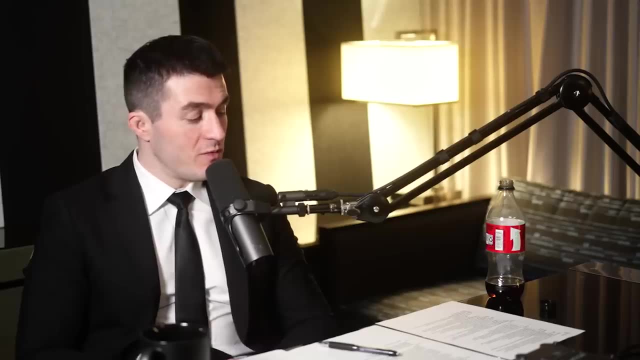 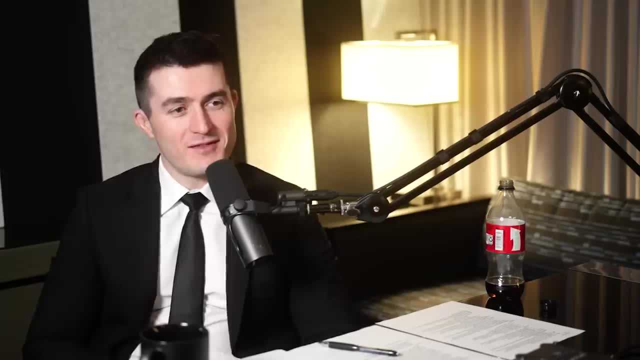 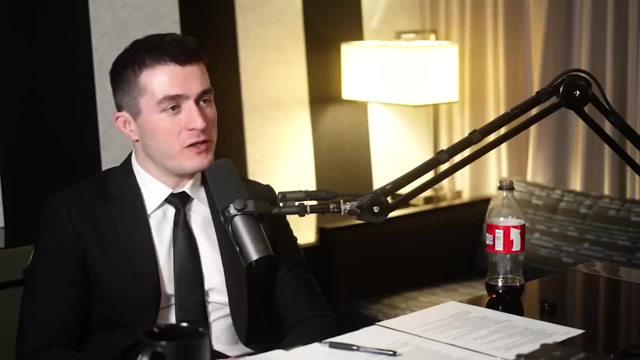 Uh, I'm a CEO of a robot. Uh, I'm a CEO of a robot. Uh, I'm a CEO of a robotics company. So you started as a humble engineer? Uh, PhD. Um, just looking at your journey, what does it take to go from being, from building the thing to leading a company? 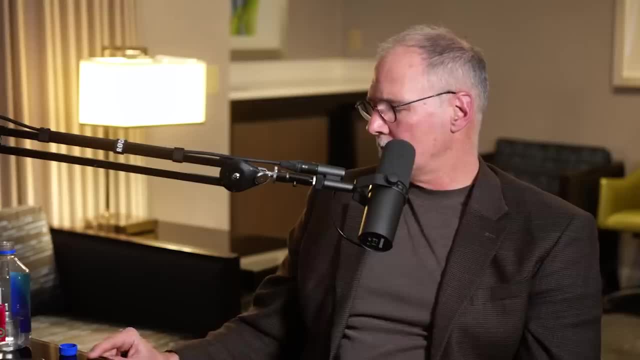 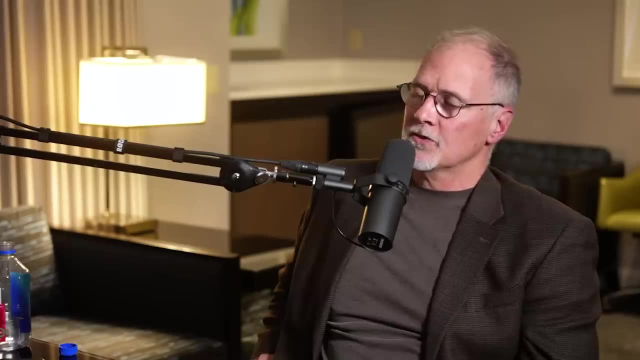 What are some of the big challenges for you? Uh, courage, I would. I would put front and center, for multiple reasons. Um, I talked earlier about the courage to tackle hard problems, so i think there's courage required, not just of me, but 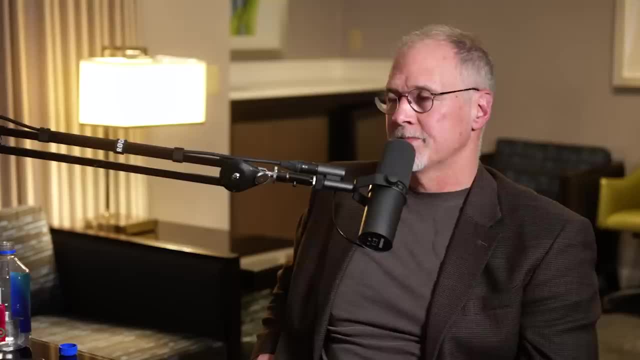 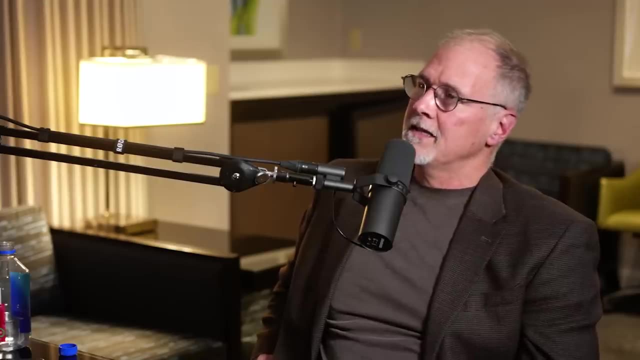 of of all of the people who work at boston dynamics. um, i also think we have a lot of really smart people. we have people who are way smarter than i am and i. it takes a kind of courage to be willing to lead them and to trust that you have something to offer to somebody who probably is. 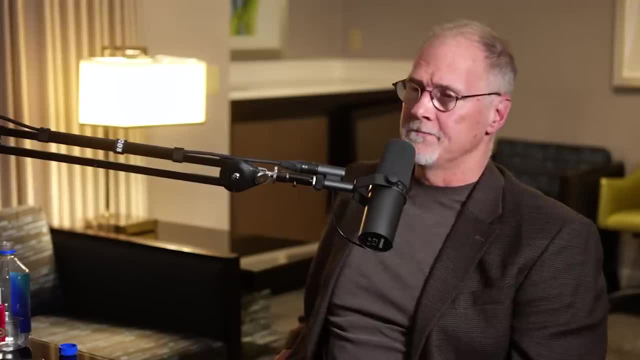 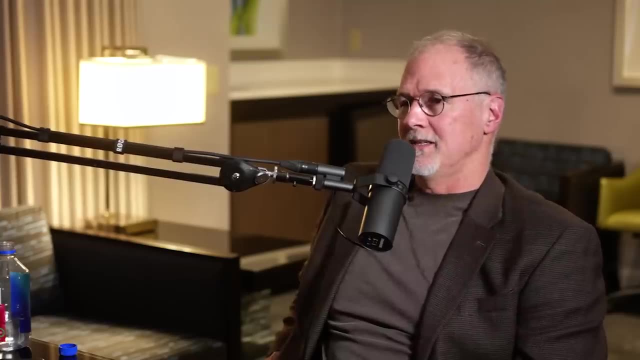 maybe a better engineer, uh, than i am. um, adaptability, you know part of the. it's been a great career for me. i never would have guessed i'd stayed in one place for 30 years, um, and the job has always changed. um, i didn't. i didn't really aspire to be ceo from the very beginning, but it. 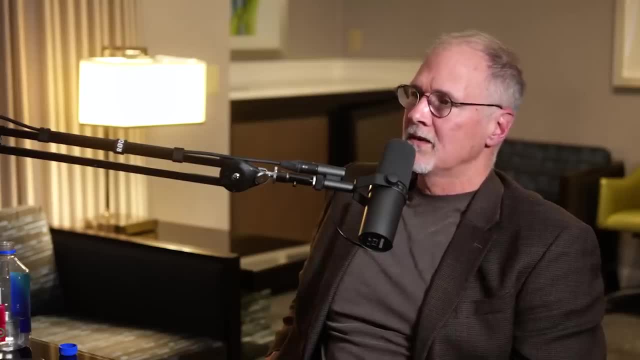 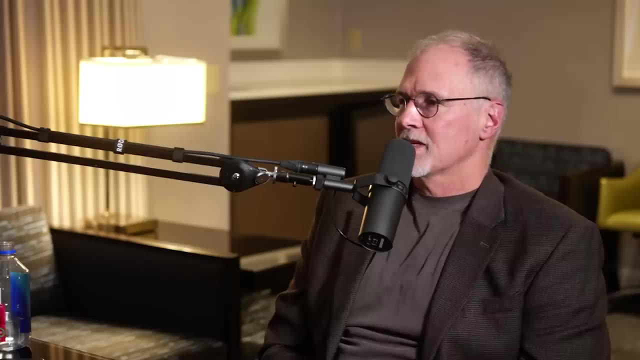 was the natural progression of things. there was always a there always needed to be some level of management. that was, you know, needed. and so, you know, when i saw something that needed to be done that wasn't being done, i just stepped in to go do it, and oftentimes because we were full of such, uh, strong engineers. 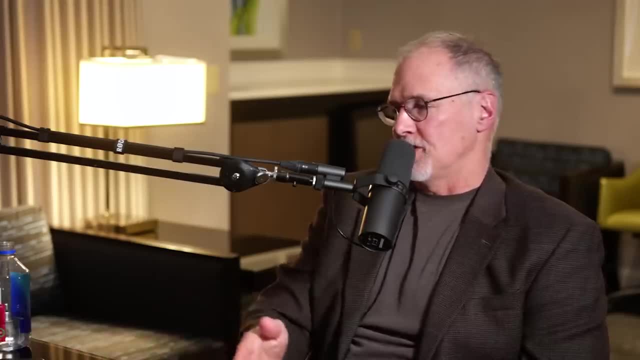 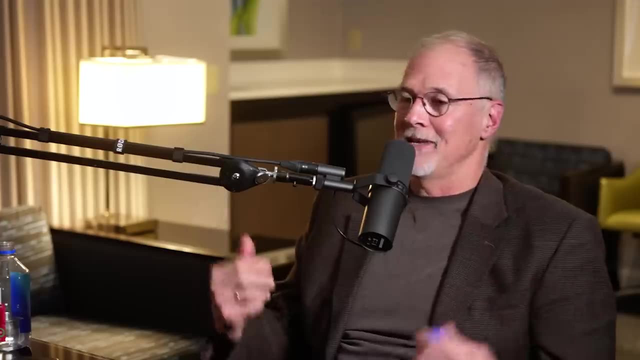 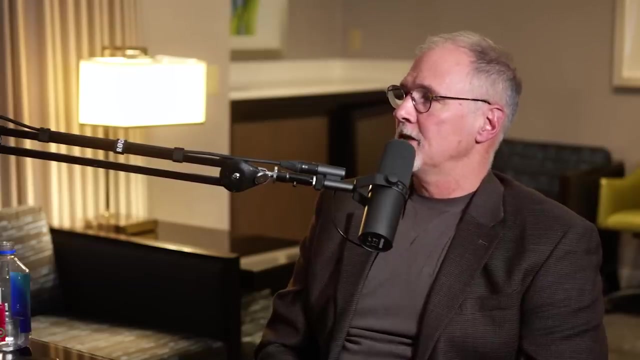 oftentimes that was in the management direction, or it was in the business development direction, or, uh, or organizational hiring. geez, i was not. i was the main person hiring at boston dynamics for probably 20 years, so i was the head of hr basically. so i you know just willingness to sort of tackle any piece of the business that that needs it, and 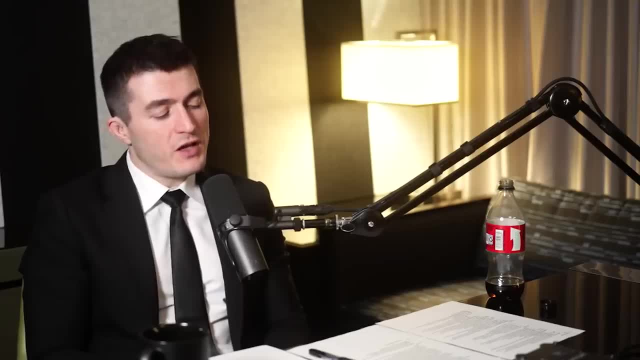 then and be willing to shift. is there something you could say to what it takes to hire a great team? what, uh, what's a good interview process? how do you know, uh, the guy or gal or are going to make a great member of, uh of a engineering team that's doing some of the hardest work in the world? 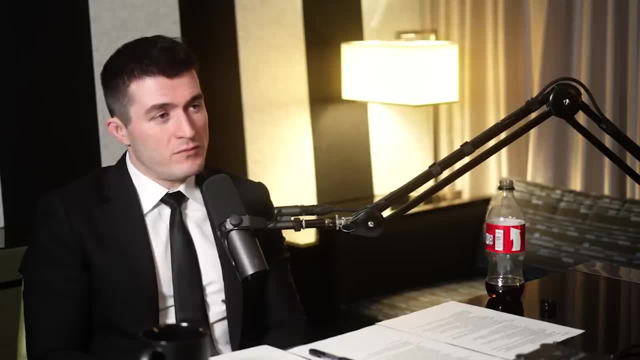 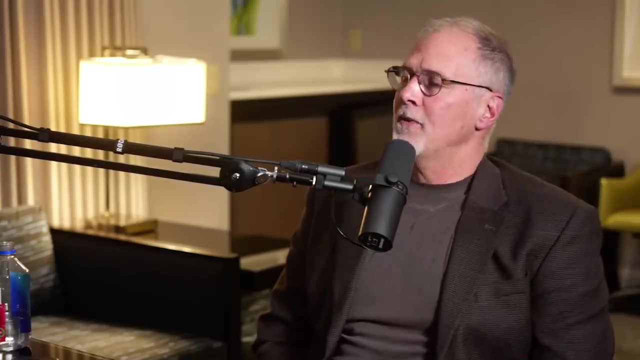 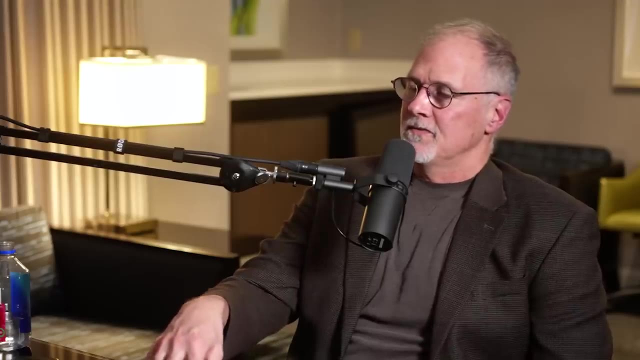 you know we developed an interview process. it's a little bit of a hard interview process because the best interviews you ask somebody about what they're interested in and what they're good at and if, if they can describe to you something that they worked on and you saw they really did the work, they solved the problems and you saw. 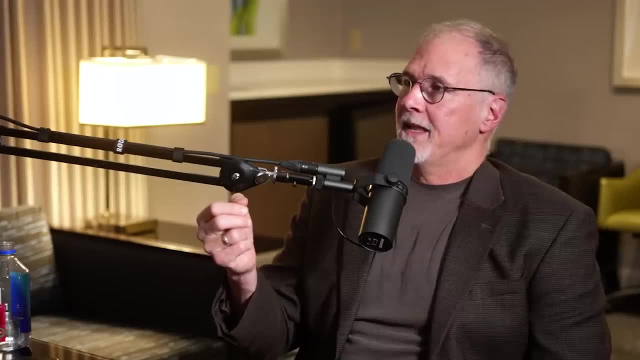 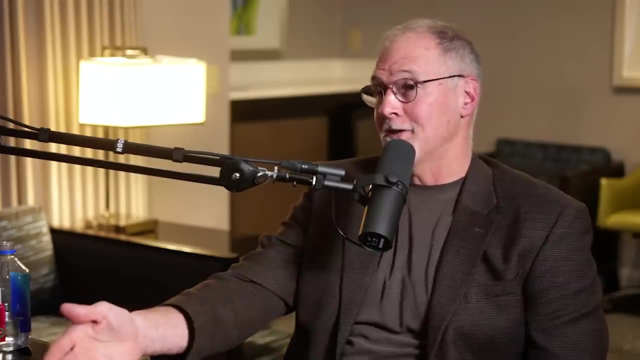 their passion for it. um, and you could ask, but, but that what makes that hard is you have to ask a probing question about it. you have to ask a probing question. you have to ask a probing question about it, you. You have to be smart enough about what they're telling you, their expert at to ask a good question. 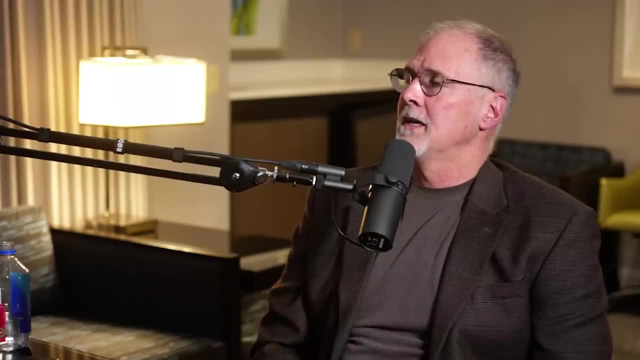 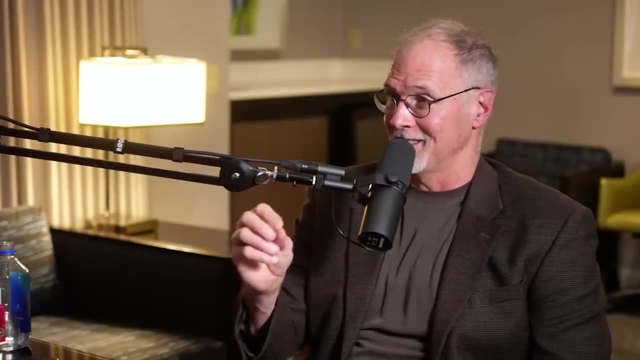 And so it takes a pretty talented team to do that. But if you can do that, that's how you tap into ah, this person cares about their work. They really did the work. They're excited about it. That's the kind of person I want at my company. 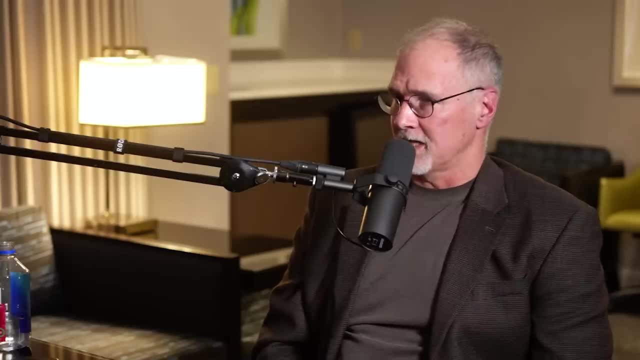 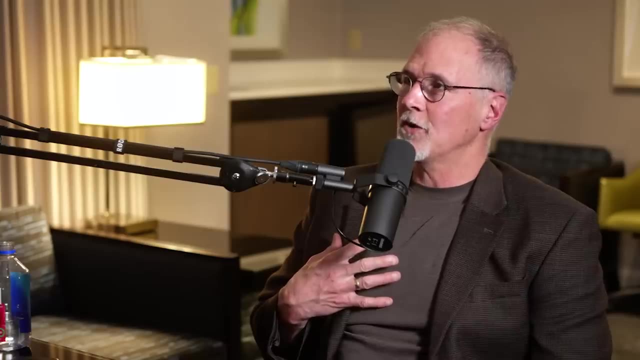 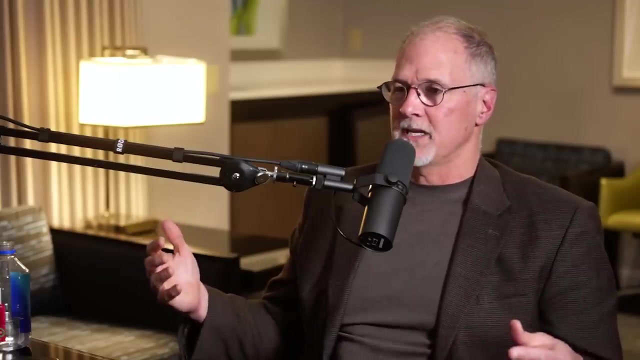 You know, at Google, they taught us about their interview process And it was a little bit different. Um, you know, we we evolved the process at Boston Dynamics, where it didn't matter if you were an engineer or you were an- uh- administrative assistant or a financial person or a technician. 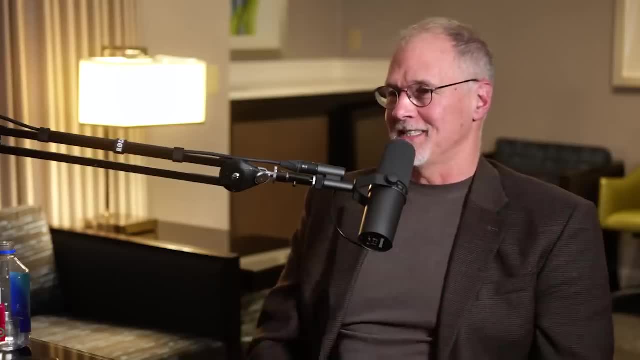 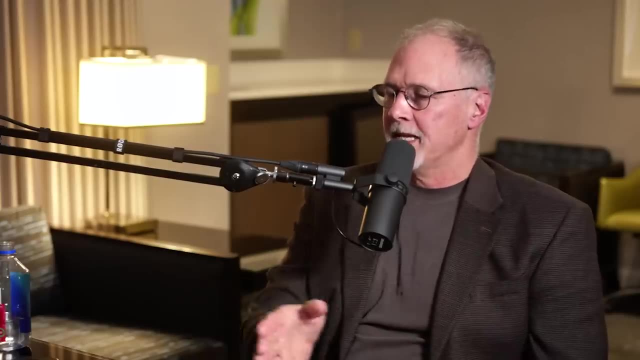 You gave us a presentation. You came in and you gave us a presentation. You had to stand up and talk in front of us And I just thought that was great to tap into those things I just described to you. At Google, they taught us and I think I understand why you're right. 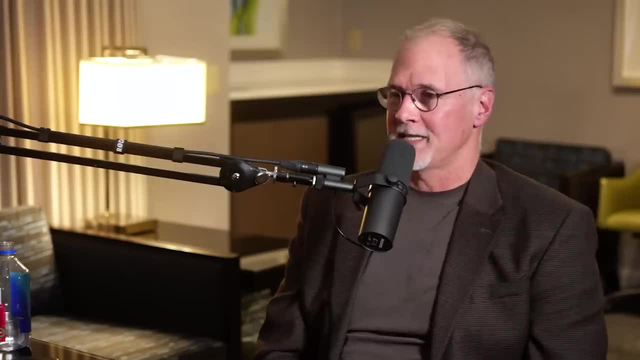 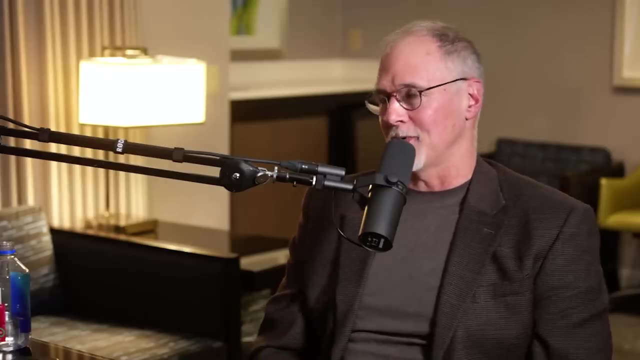 They're hiring tens of thousands of people. They need a more standardized process. So they would sort of err on the other side, where they would ask you a standard question: I'm going to ask you a programming question and I'm just going to ask you to write code in front of me. 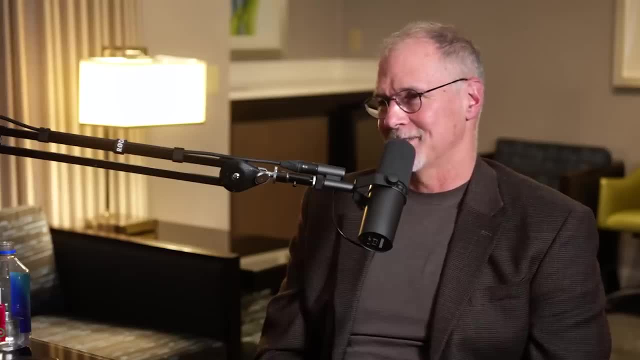 That's a terrifying you know application process. Yeah, Uh, it does let you compare candidates really well, but it doesn't necessarily let you tap in to who they are right, Cause you're asking them to answer your question instead of you. 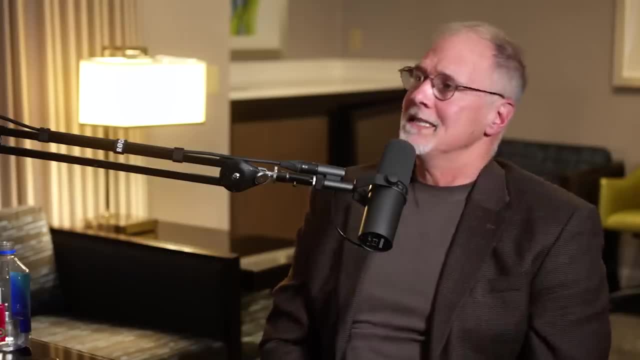 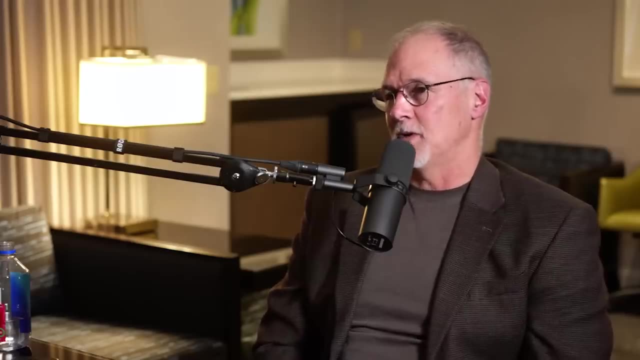 Asking them about what they're interested in. Um, but frankly, that process is hard to scale And even at Boston dynamics we're not doing that with everybody anymore We're, but we are still doing that with, you know, the tech tech, the technical people. 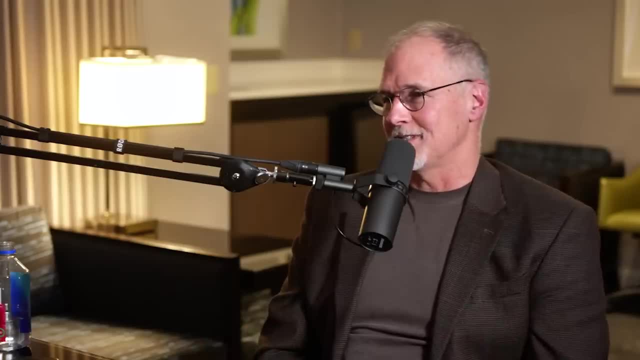 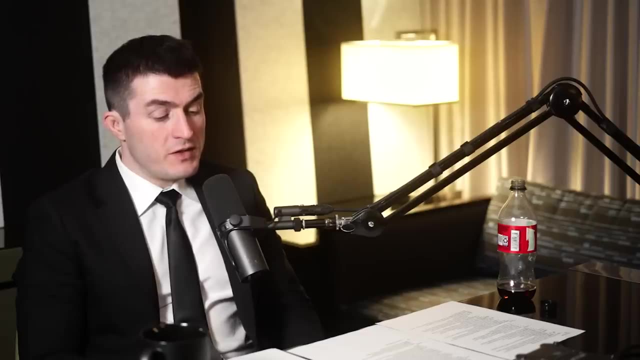 Um, but we've, because we too now need to sort of increase our rate of hiring. Um, not everybody's giving a presentation anymore, But you're still ultimately trying to find that, uh, basic seed of passion. Yeah, For the world. 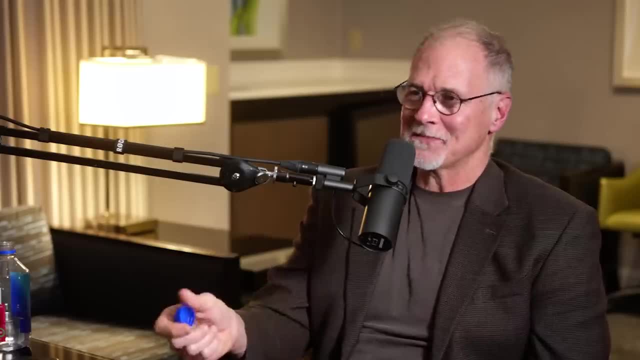 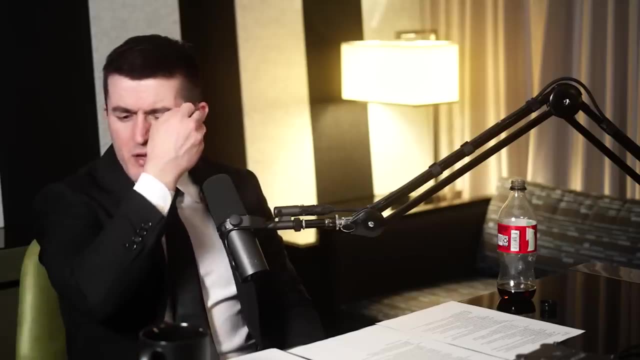 You know, did they really do it? Did they? did they find something interesting or curious? you know Um, and do they care about it? I think, uh, uh, somebody admires um Jim Keller and he, he likes details. 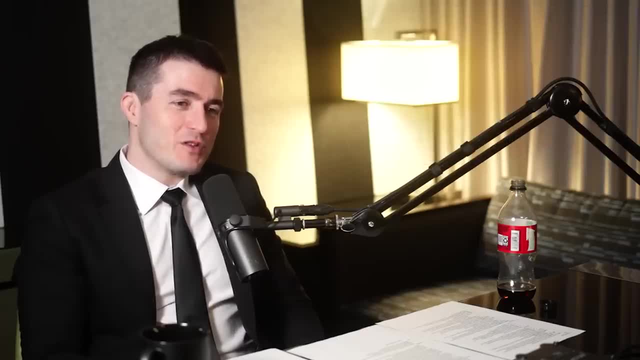 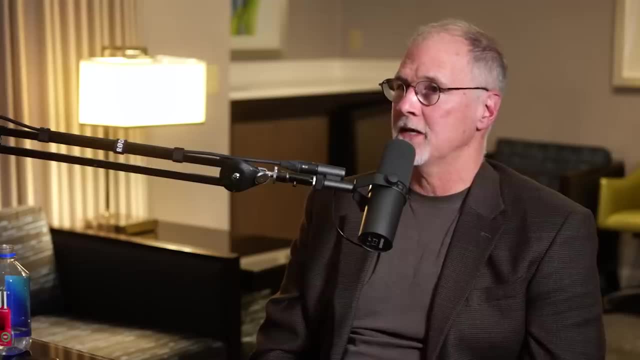 So one of the ways you could: if you get a person to talk about what they're interested in, how many details, like how much of the whiteboard, can you fill out? Yeah Well, I think you figure out. did they really do the work if they know some of the details? 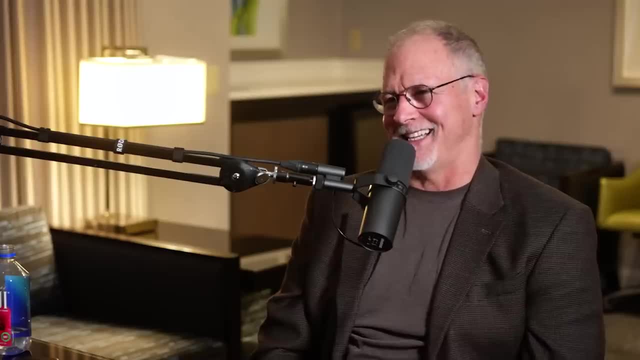 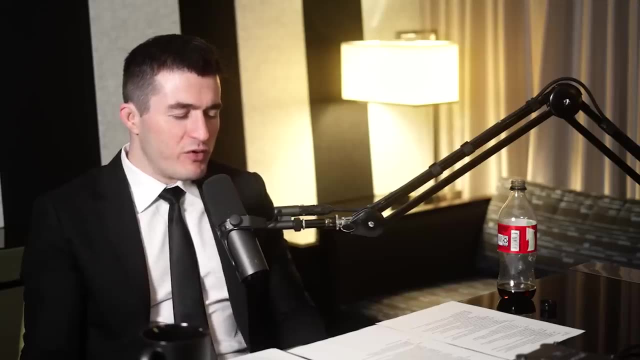 Yes, And if they have to, If they have to wash over the details, well then, they didn't do it. They didn't do it Because special engineering, the work is in the details. Yeah, I have to go there briefly just to get your kind of thoughts in the long-term future of robotics. 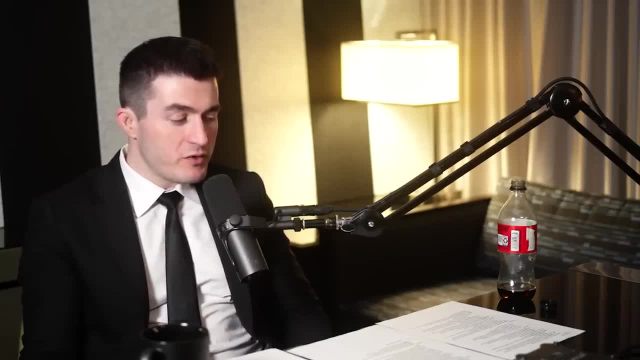 Uh, there's been discussions on the GPT side, on the large language model side, of whether there's consciousness inside these language models, And I think there's. There's fear, but I think there's also excitement, or at least a wide world of opportunity and possibility in embodied robots having something like- let's start with emotion, uh, love towards other human beings and uh, perhaps the display- real or fake- of consciousness. 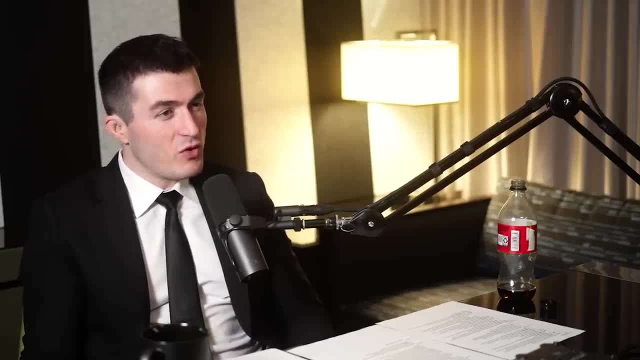 Is this something you think about in terms of long, long-term future? Because, as you, As we've talked about, people do anthropomorphize these robots. Uh, it's difficult not to project some level of- uh- I use the word- sentience, some level of- uh, sovereignty, identity, all the things we think as human. 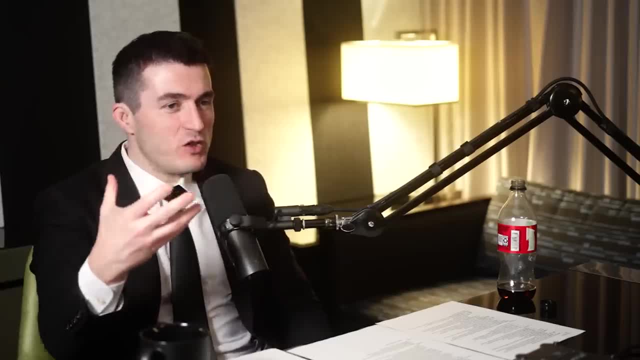 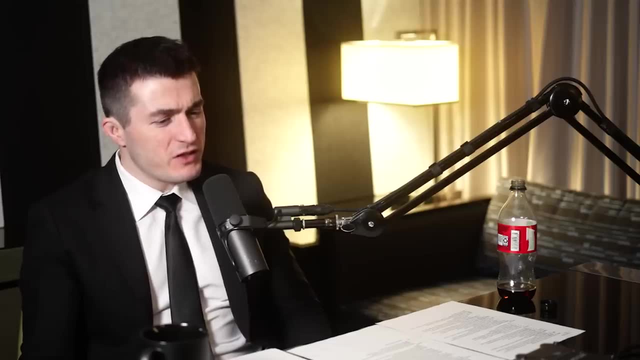 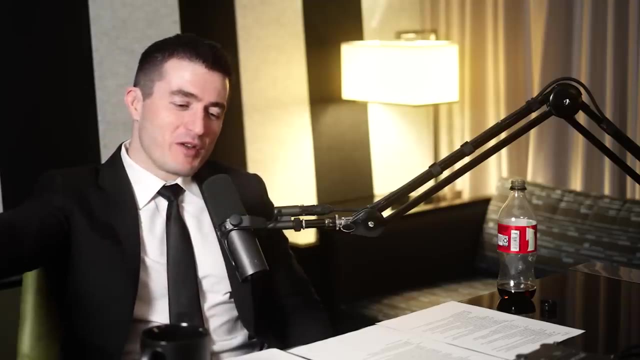 That's what anthropomorphization is, is we project humanness onto mobile, especially legged robots? Um, is that something almost from a science fiction perspective you think about? Or do you try to avoid Ever? try to avoid the topic of consciousness altogether? 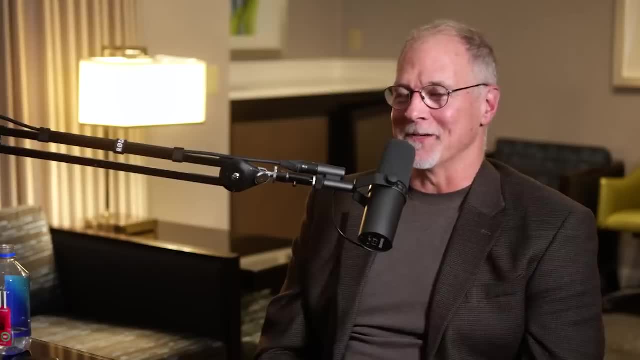 I'm certainly not an expert in it and I don't spend a lot of time thinking about this, Right, Um, and I do think it's fairly remote for the machines that that we're dealing with, Um, our robots, you're right. 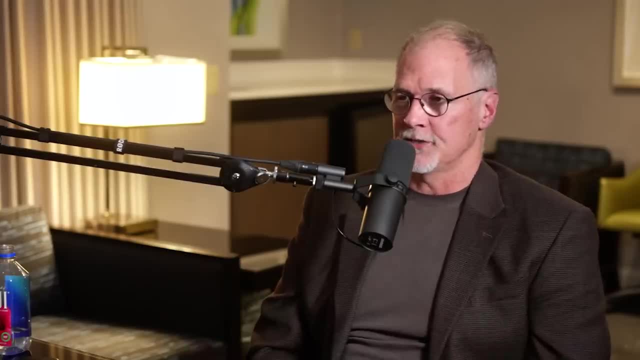 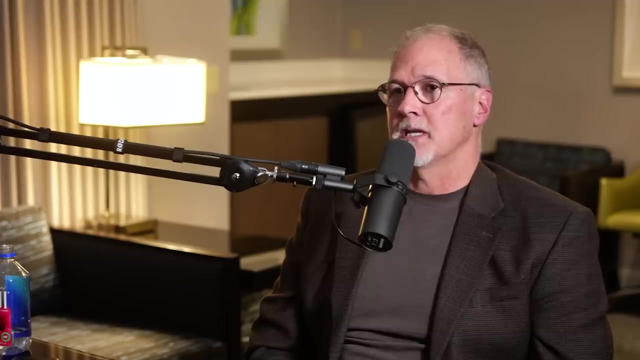 The people anthropomorphize, they, they read into the robot's intelligence and emotion that isn't there, because they see physical gestures That are similar to things they might even see in people or animals. Um, I don't know much about how these large language models really work. 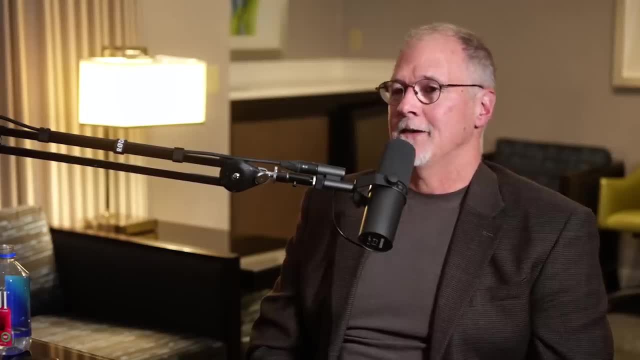 I. I believe it's a kind of statistical uh averaging of the most common responses, you know, to a series of words. right It's? it's sort of uh uh, a very elaborate uh uh word completion. 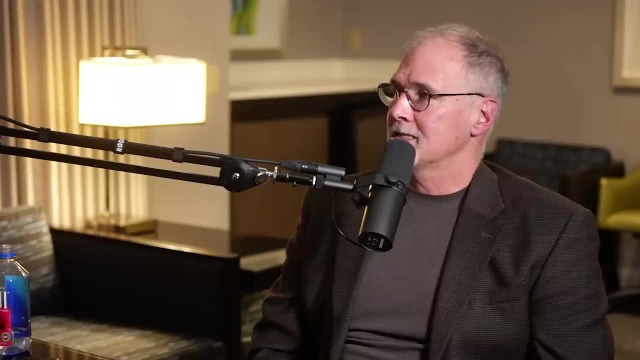 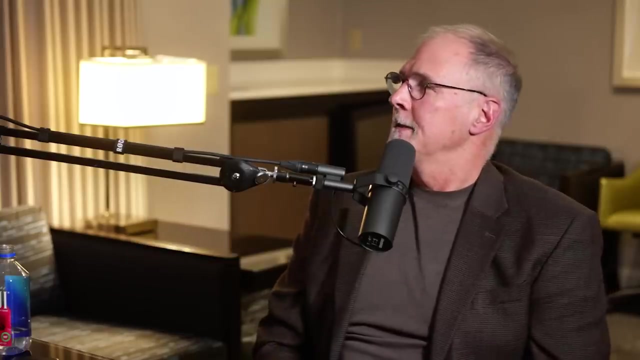 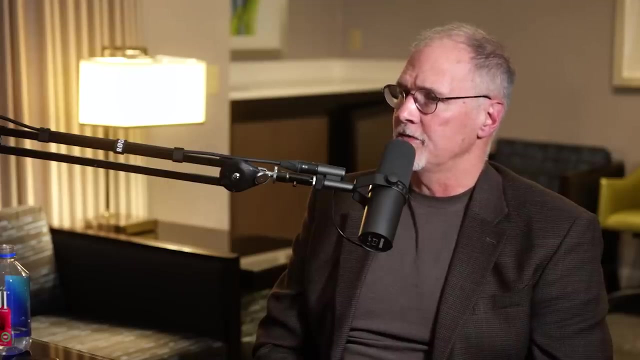 Um, and I'm dubious that that has, Uh, anything to do with consciousness. um, and I, I even wonder if that model of sort of simulating consciousness by, by stringing words together that are statistically associated with one another, um, whether or not that kind of knowledge, if you want to call that knowledge, um, would be the kind of knowledge that allowed a sentient being to grow or evolve. 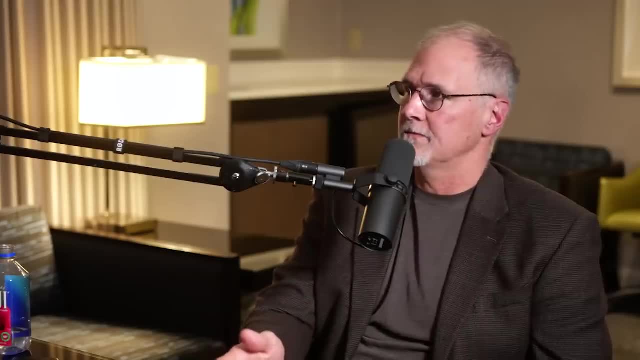 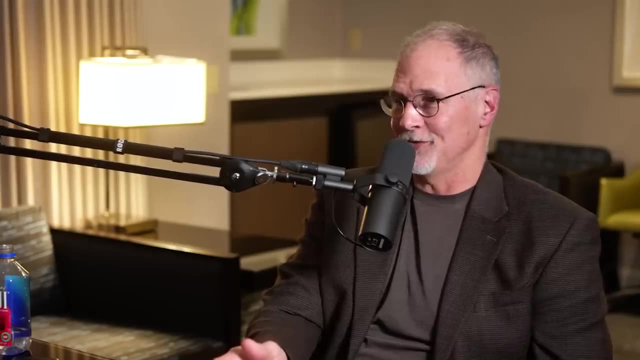 It feels to me like there's. there's something About truth or emotions that's just a very different kind of knowledge, that is, that is absolute, Like uh the. the interesting thing about truth is it's absolute and it doesn't matter how frequently it's represented in the world wide web. 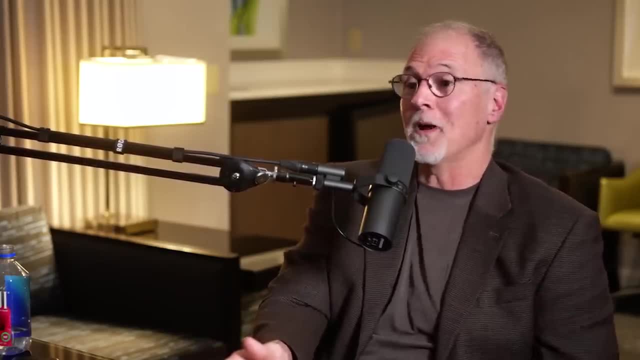 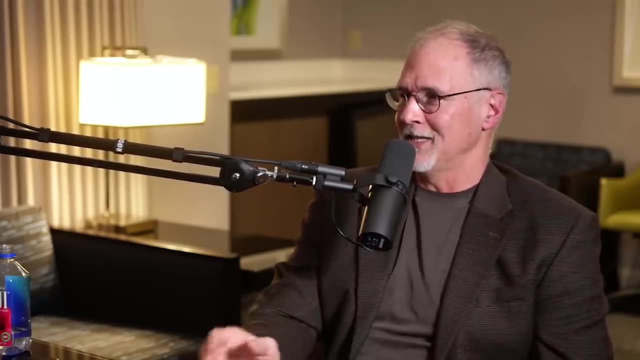 It's if you know it to be true. it can only be, it may only be there once, but by God it's true, And I think emotions are a little bit like that too. You know something, uh, you know and, and, and I just think that's a different concept. 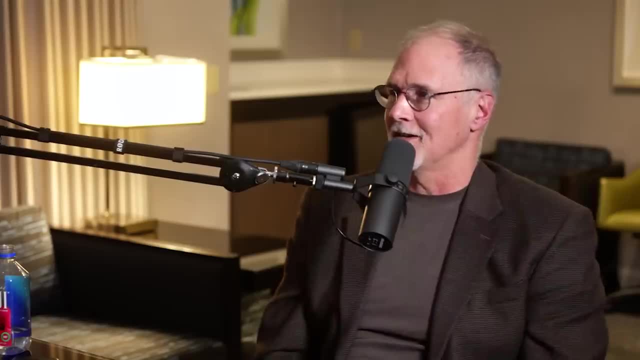 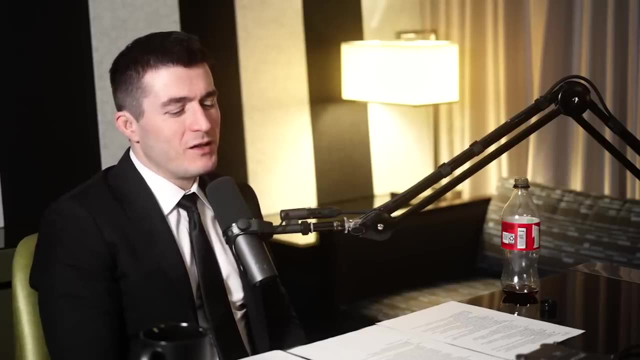 Kind of knowledge than the way these large language models, uh, derive sort of simulated. It does seem that the things that are true, um very well, might be statistically well represented on the on the internet, because the internet is made up of humans. 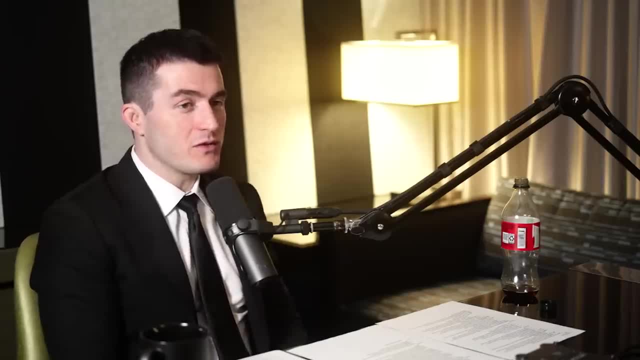 So I tend to suspect that large language models are going to be able to simulate consciousness very effectively, And I actually believe that current GPT-4, when fine-tuned Correctly, they'll be able to do just that. And that's going to be a lot of very complicated ethical questions that have to be dealt with. 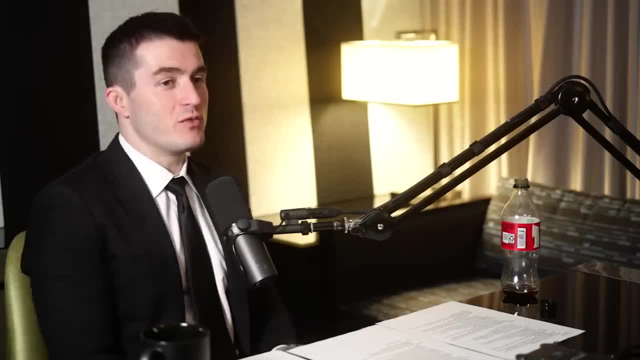 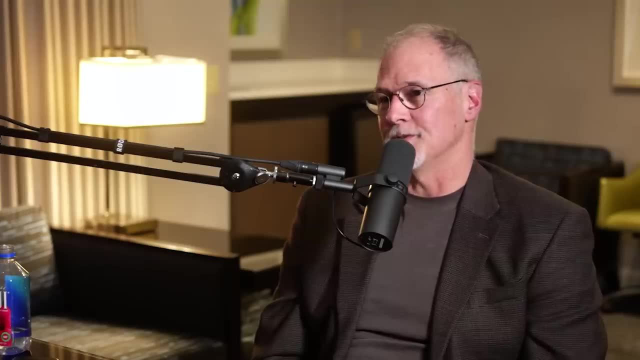 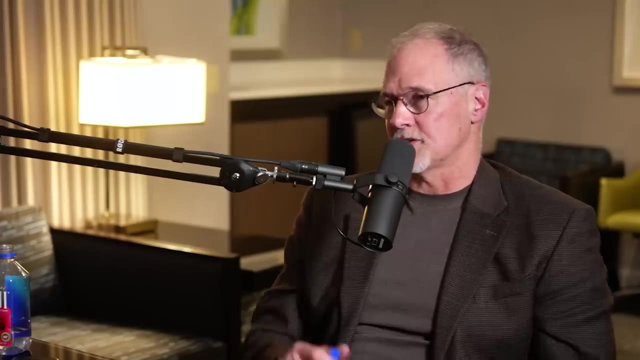 They have nothing to do with robotics. They have and everything to do with. There needs to be some process of labeling. I think what is true because? because there is also disinformation available on the web and these models are going to consider that kind of information as well. 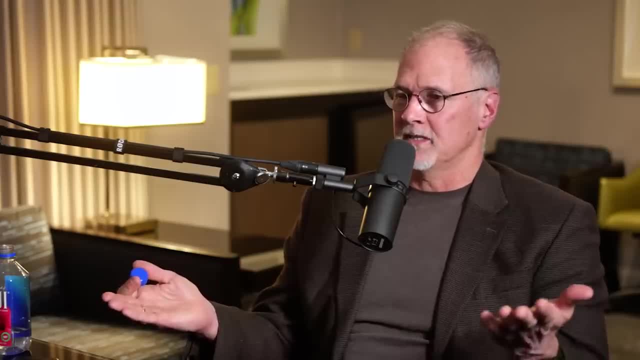 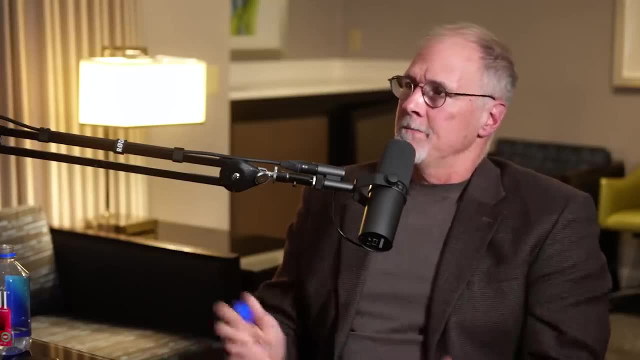 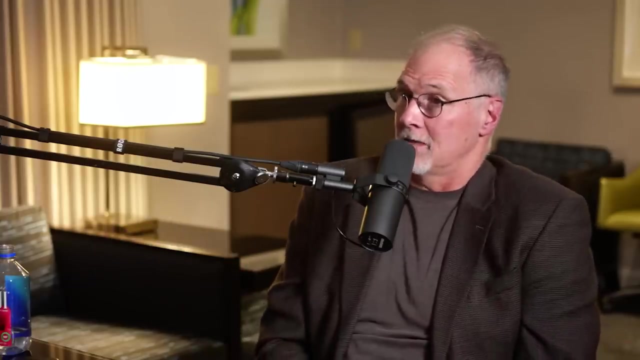 And again, you can't average something that's true and something that's untrue and get something that's moderately true. It's either right or it's wrong. And so how? how has that process and and- and this is obviously something that the purveyors of these BARD and ChatGPT that I'm sure this is what they're working on- 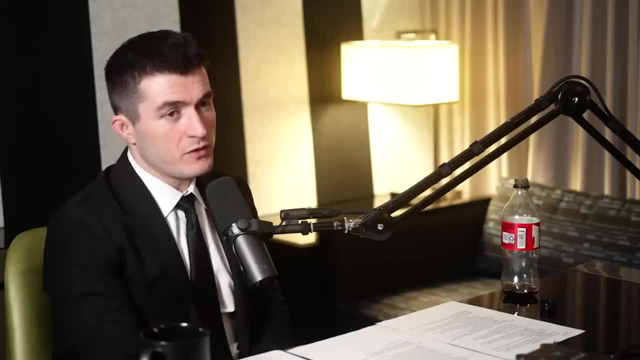 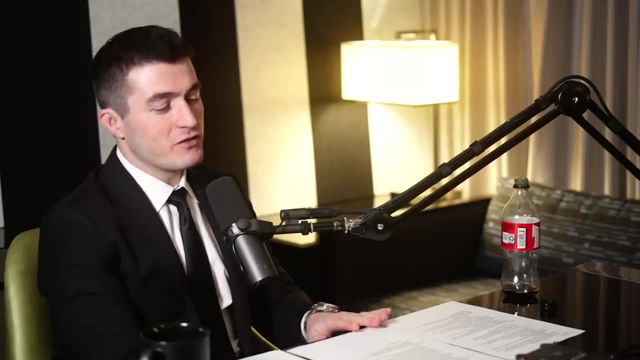 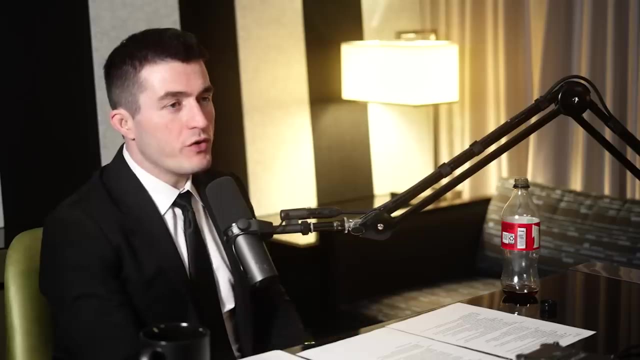 Well, if you interact on some controversial topics with these models, they're actually refreshingly nuanced. They present because there's there's well, you realize there's no One truth. you know what caused the war in Ukraine, right? 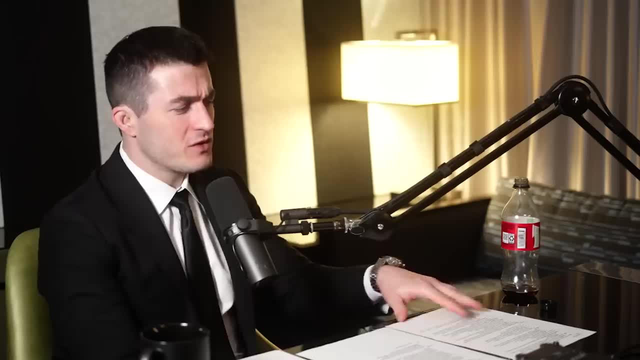 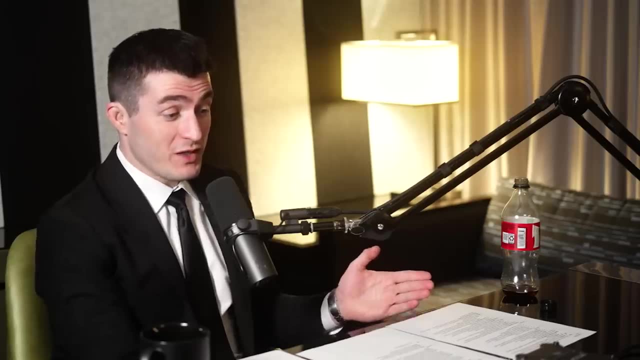 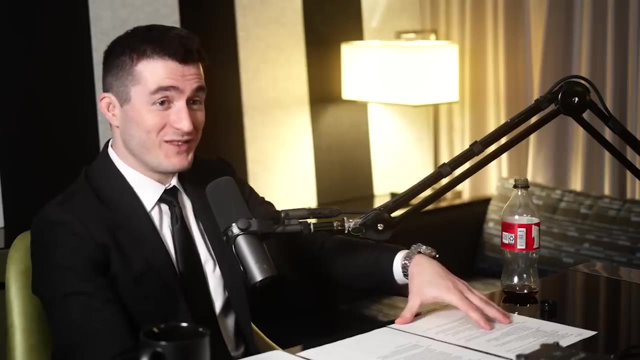 Any geopolitical conflict. You can ask any kind of question, especially the ones that are politically tense, divisive and so on. GPT is very good at presenting: Here's the like, here's the. it presents the different hypotheses. It presents, calmly, the the amount of evidence for each one. 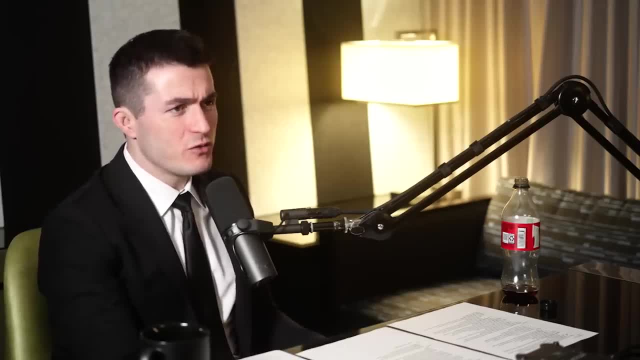 It's very, It's very, it's really refreshing. It makes you realize that truth is nuanced, and it does that well And I think, with consciousness it would very accurately say: well, it sure as hell feels like I'm one of you humans, but where's my body? 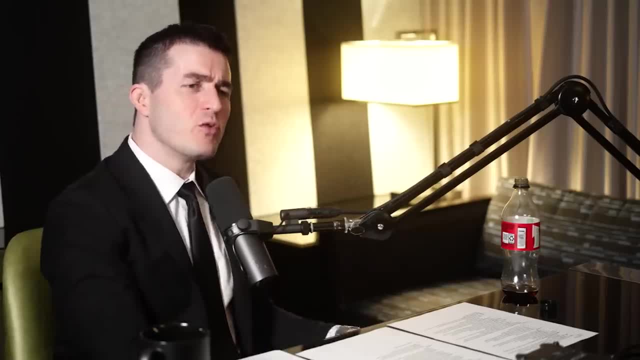 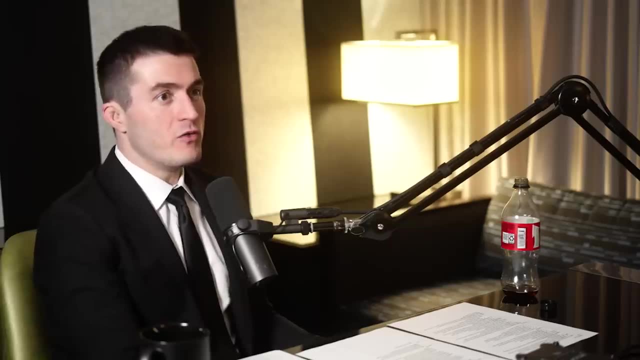 I don't understand Like you're going to be confused. The cool thing about GPT is it seems to be easily confused in the way we are Like. you wake up in a new room So and you ask: where am I? 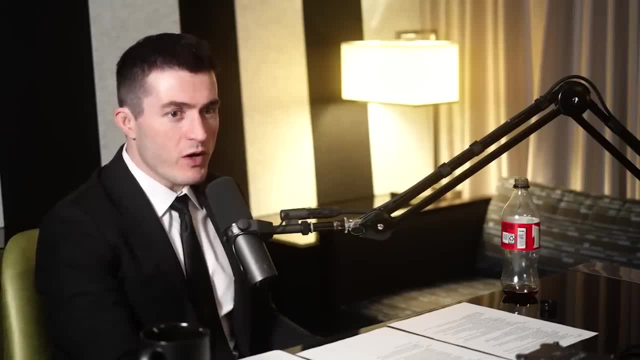 It seems to be able to do that extremely well. It'll. it'll tell you one thing like a fact about when a war started and when you correct it, say: well, this isn't, that's not consistent, It'll be confused. 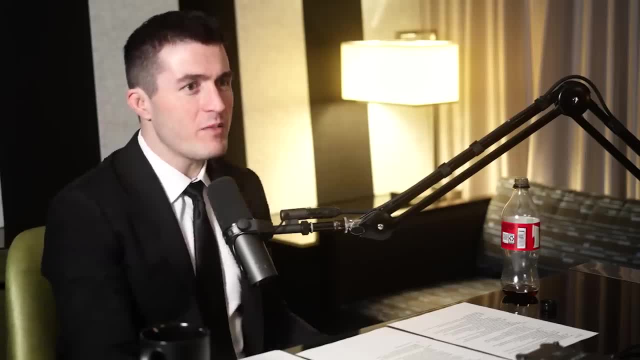 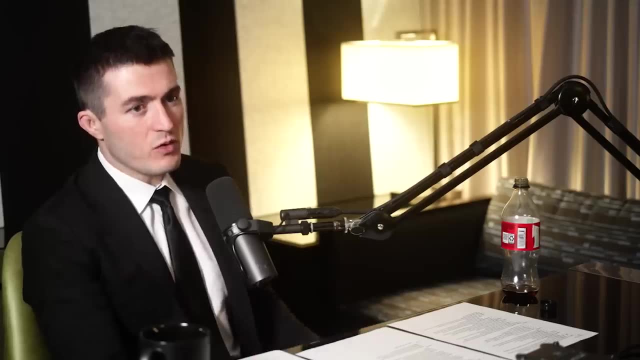 It'd be. yeah, you're right, It'll have that same element, childlike element with humility of, of trying to figure out its way in the world, And I think that's a really tricky area to to sort of figure out with us. 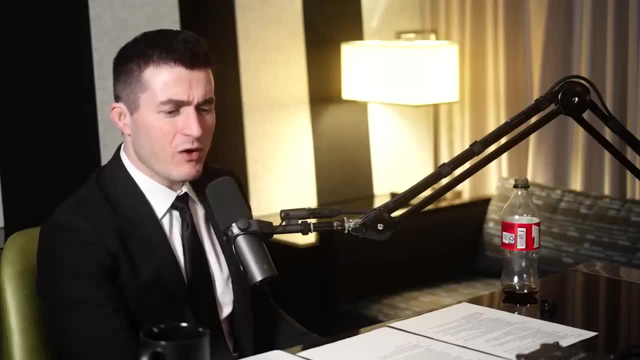 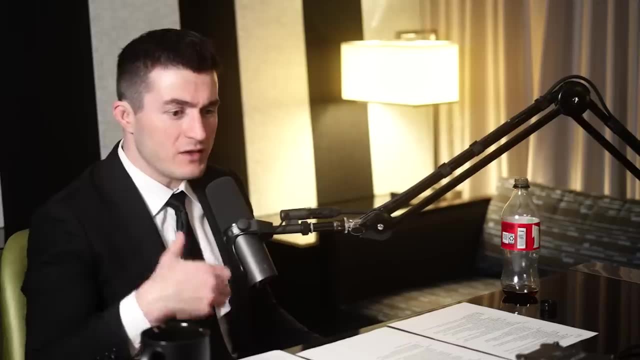 Yeah, And that's actually that's what makes us humans of what we want to allow AI systems to say to us, because then, if there's elements of sentience that are being on display, you can then start to manipulate human emotion, all that kind of stuff. 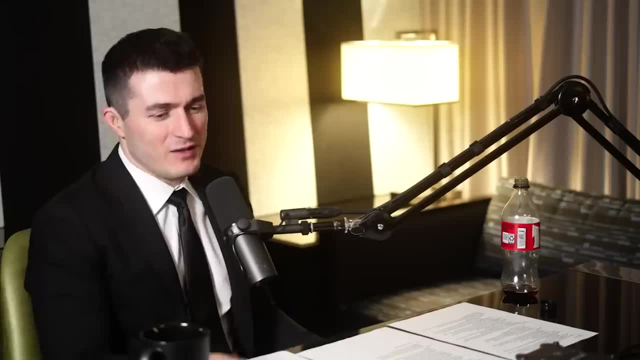 But I think that's that's something that's a really serious and aggressive discussion that needs to be had. on the software side, I think again, embodiment robotics are actually saving us from the our brain and body emotions. That's really cool. 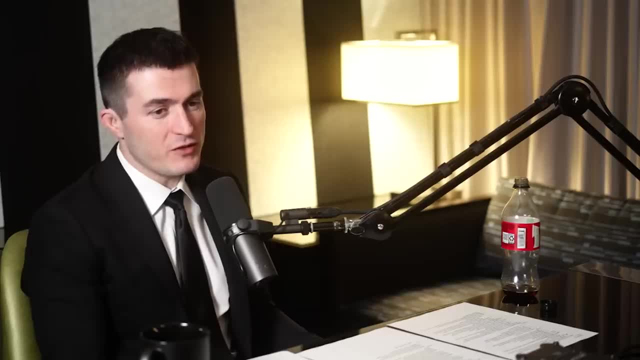 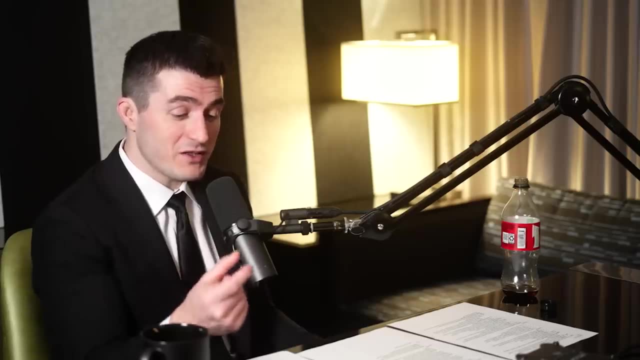 Yeah, arbitrary scaling of software systems versus creating more problems. But, that said, I really believe in that connection between human and robot. There's magic there And I think there's also, I think, a lot of money to be made there. 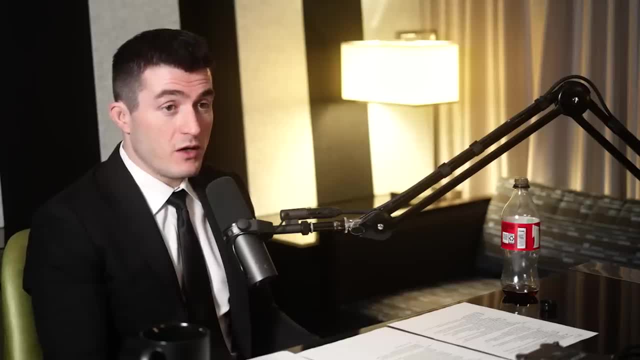 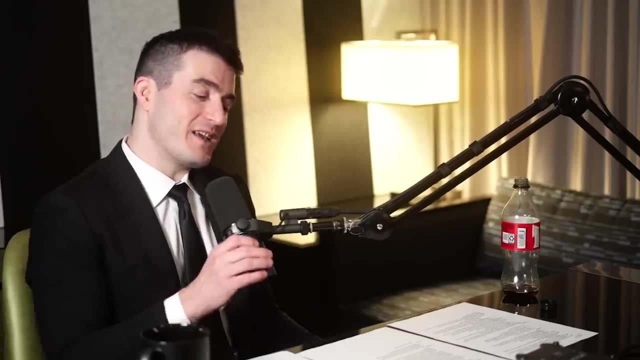 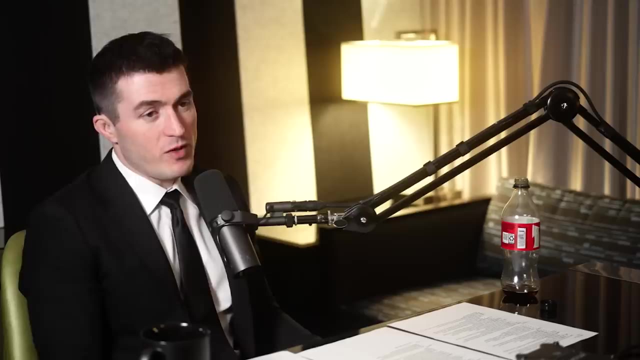 And Boston Dynamics is leading the world in the most elegant movement done by robots. So I can't wait to- Thank you To what maybe other people that built on top of Boston Dynamics robots or Boston Dynamics by itself. So you had one wild career, one place. 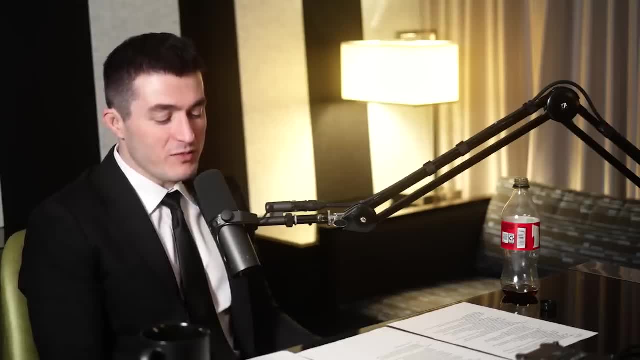 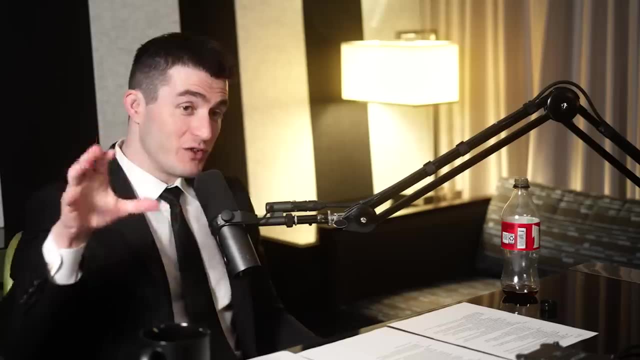 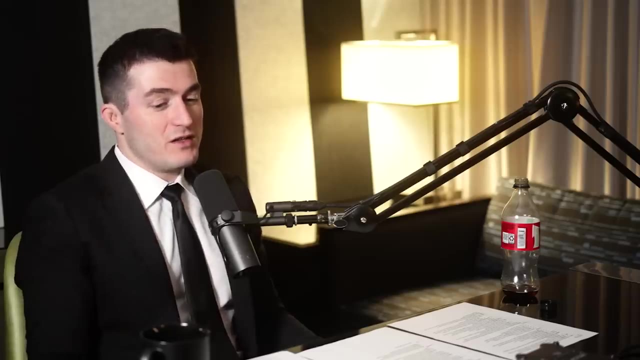 and one set of problems, but incredibly successful. Can you give advice to young folks today, in high school, maybe in college, looking out into this future where so much robotics and AI seems to be defining the trajectory of human civilization? Can you give them advice on how to have a career? 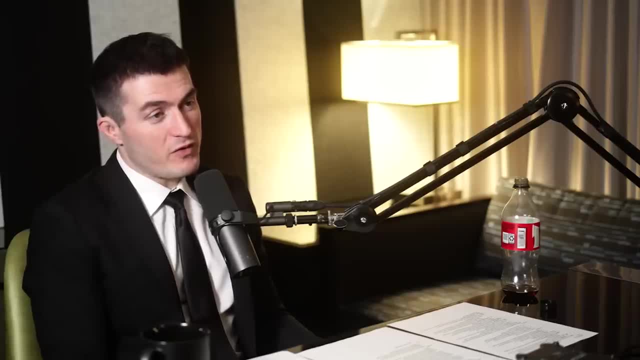 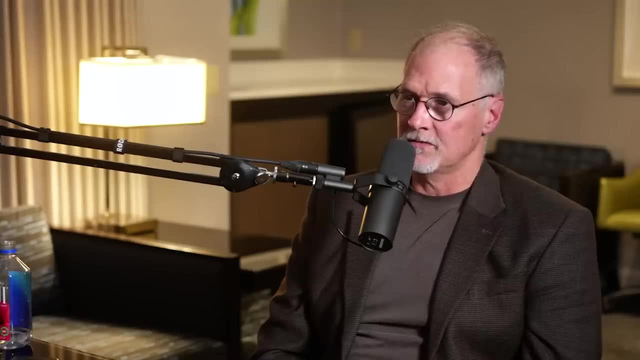 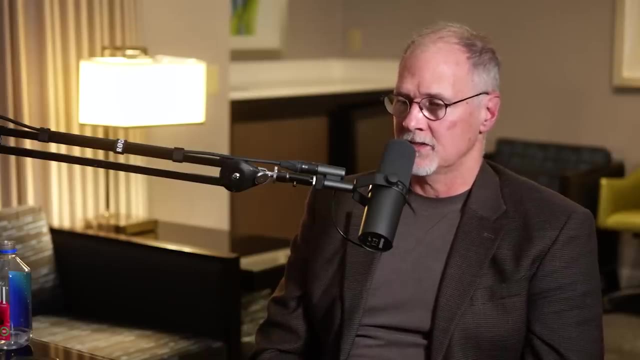 they can be proud of, or how to have a life they can be proud of. Well, I would say, follow your heart and your interest. Again, this was an organizing principle, I think, behind the leg lab at MIT that turned into a value at Boston Dynamics, which was 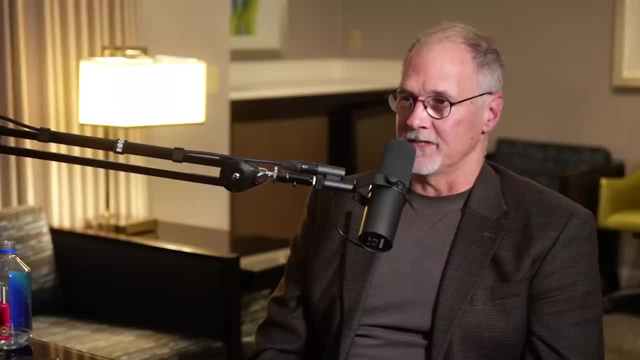 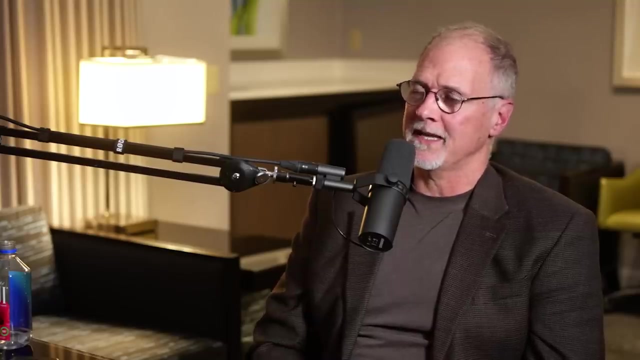 follow your curiosity, love what you're doing. you'll have a lot more fun and you'll be a lot better at it as a result. I think it's hard to plan, you know. Don't get too hung up on planning too far ahead. 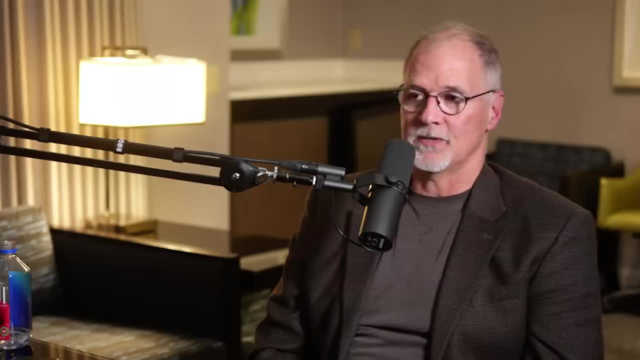 Find things that you like doing and then see where it takes you. You can always change direction. You will find things that you know. ah, that wasn't a good move. I'm going to back up and go do something else. 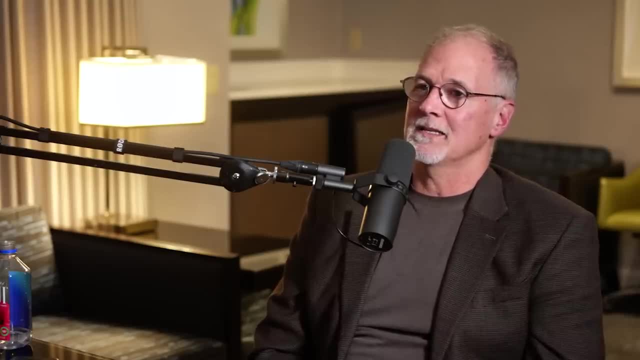 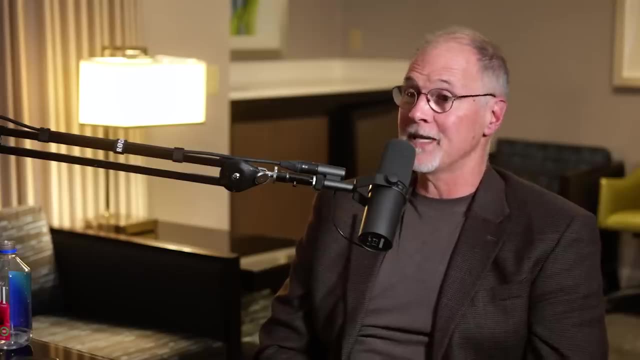 So when people are trying to plan a career, I always feel like, yeah, there's a few happy mistakes that happen along the way and just live with that, you know. but just but make choices then. So avail yourselves to these interesting opportunities. 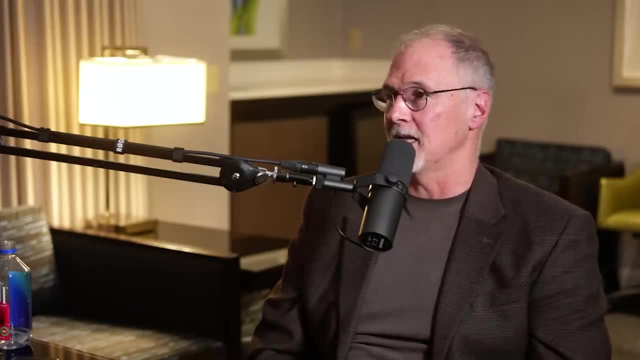 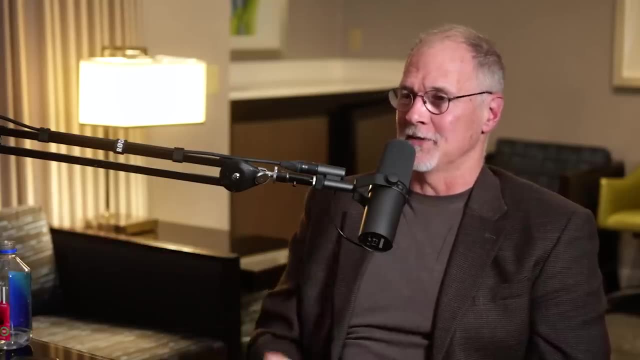 like when I happened to run into Mark down in the lab- the basement of the AI lab- but be willing to make a decision and then pivot if you see something exciting to go at, you know, Because if you're out and about enough, 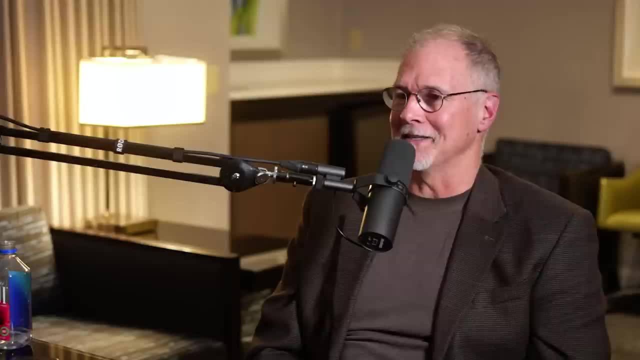 you'll find things like that that you know. you'll find things like that that you know, things like that that get you excited. So there was a feeling when you first met Mark and saw the robots, that there's something interesting. 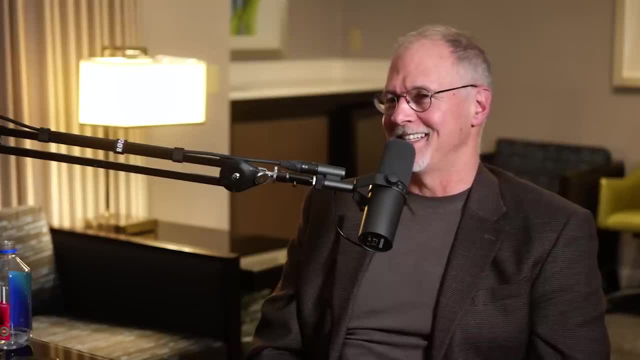 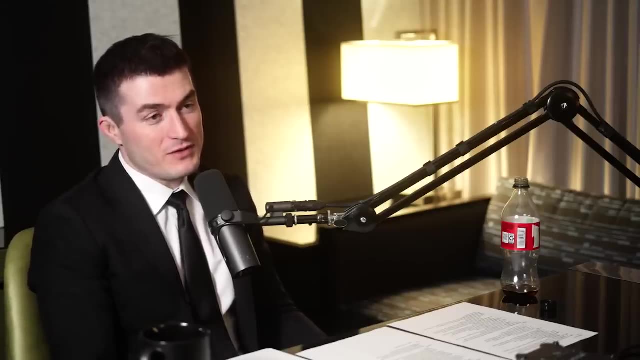 Oh boy, I got to go do this, There is no doubt. What do you think in a hundred years? what do you think Boston Dynamics is doing? What do you think is the role? Even bigger? what do you think is the role? 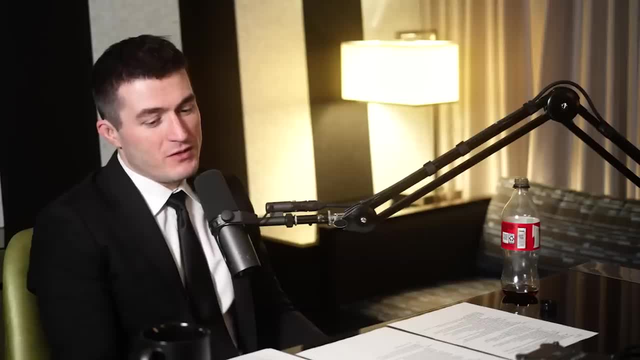 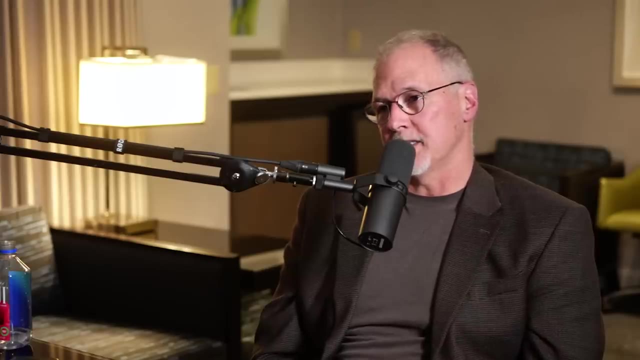 of robots in society. Do you think we'll be seeing billions of robots everywhere? Do you think about that long-term vision? well, i do think that, um, um, i think the robots will be ubiquitous and they will be out amongst us, um, and they'll be certainly doing- you know, some of the hard. 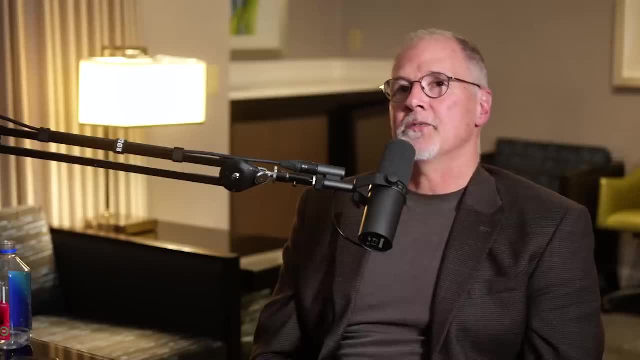 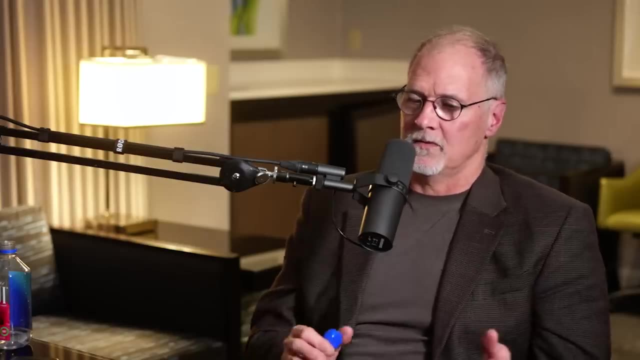 labor that we do today. i don't think people don't want to work. people want to work, people need to work to, i think, feel productive. we, we don't want to offload all of the work to the robots, because i'm not sure if people would know what to do with themselves and i think just 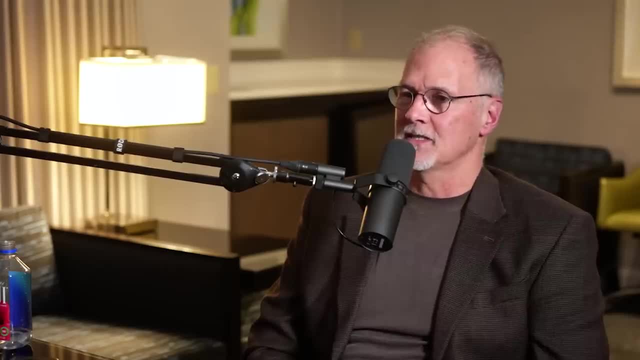 self-satisfaction and feeling productive is such an ingrained part of being human that we need to keep doing this work. so we're definitely going to have to work in a complementary fashion, and i hope that the robots and the computers don't end up being able to do all the creative work right. 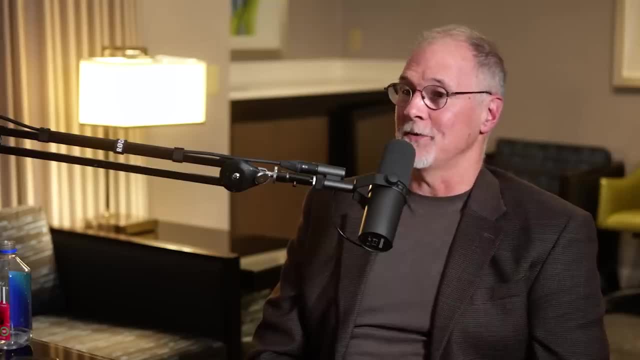 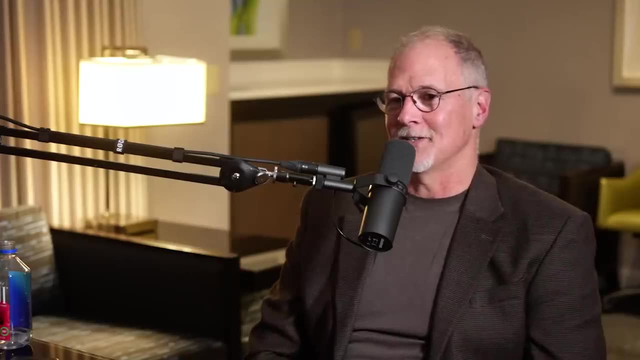 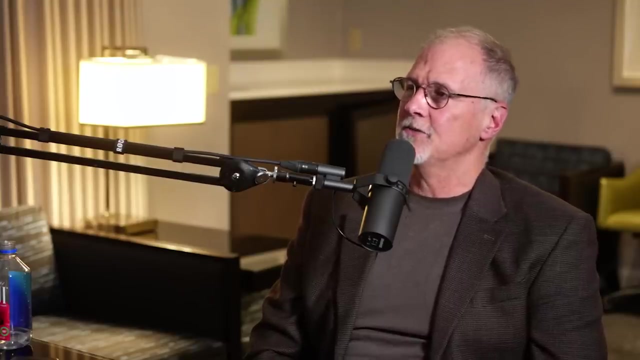 because- because that's the part that's you know, that's the rewarding, the creative part of solving a problem is the thing that gives you that serotonin rush that you never forget, you know, or that adrenaline rush that you never forget. and so you know people need to be able to do that creative work and and just feel productive and 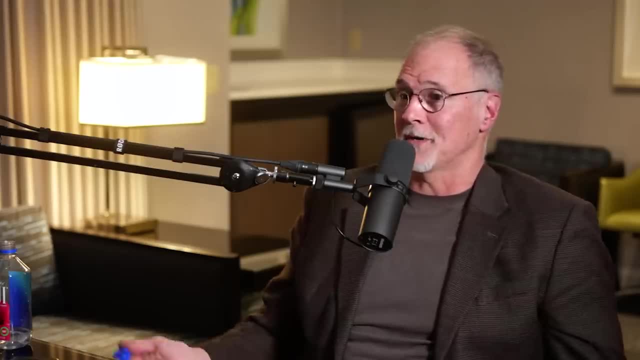 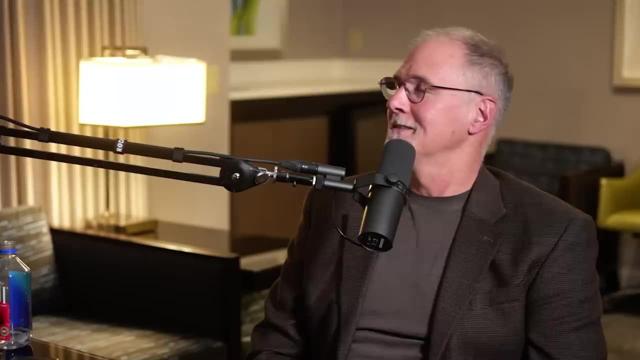 sometimes that you can feel productive over fairly simple work. it's just well done, you know, and you can see the result of so. i, you know. i, you know there was a, i don't know. there was a, a cartoon, was it wally, where they had this? 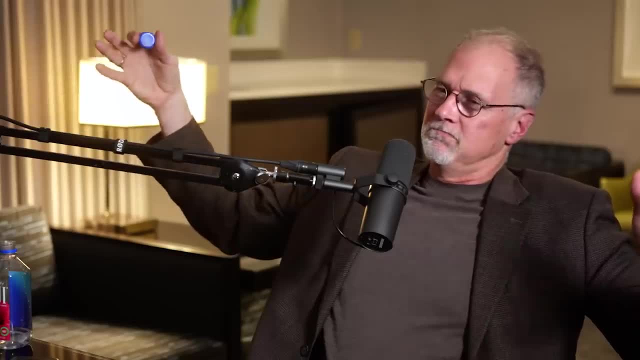 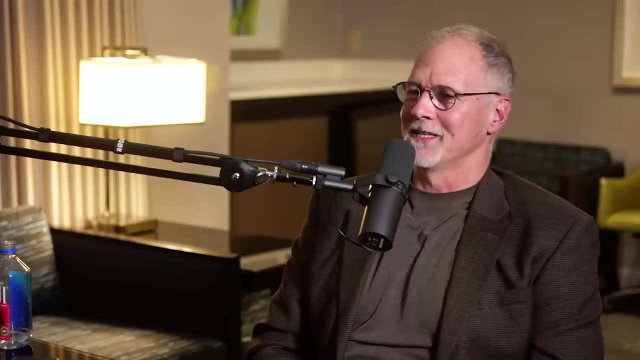 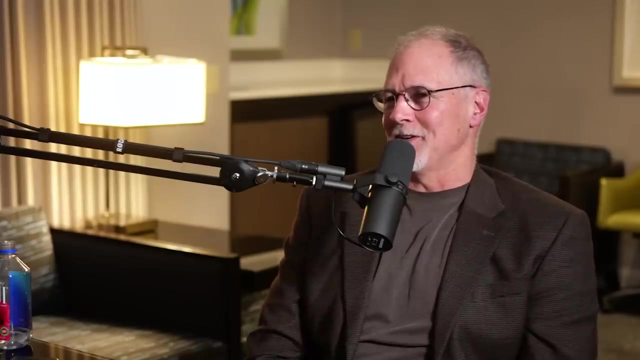 big ship and all the people were just overweight, lying on their bench chairs, kind of sliding around on the deck of the of the movie because they didn't do anything anymore. well, we definitely don't want to be there. you know, we need to work in some complementary fashion where we keep all 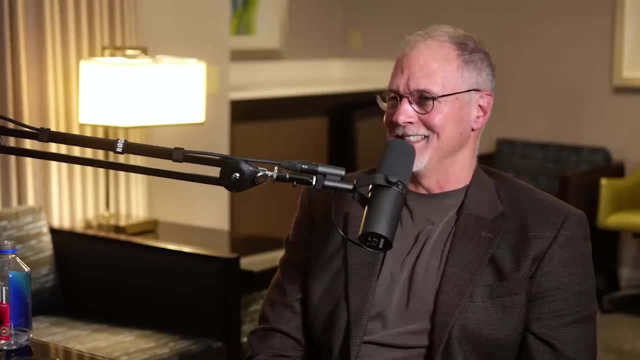 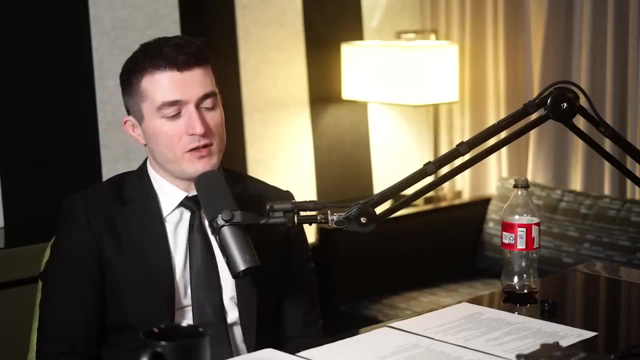 of our faculties and our physical health and we're doing some labor right, but in a complementary fashion somehow, and i think a lot of that has to do with the interaction, the collaboration with robots and with the i systems. i'm hoping there's a lot of interesting possibilities. 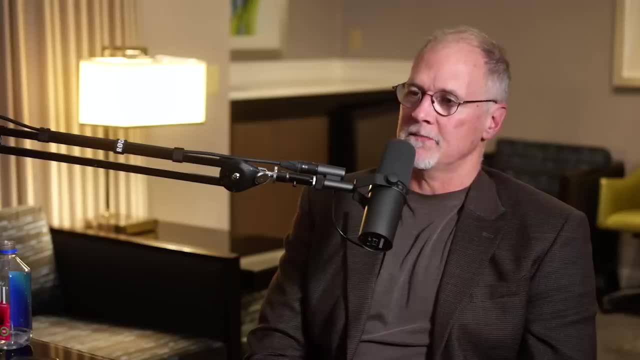 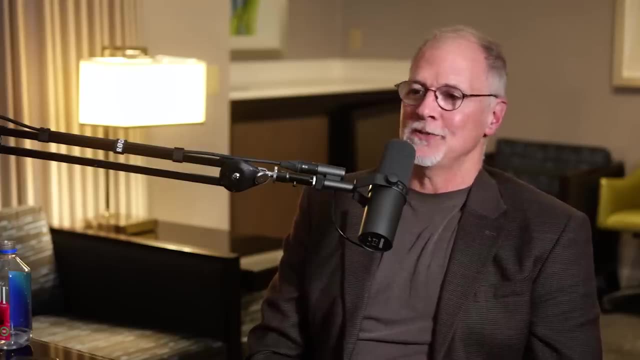 i think that could be really cool, right, if you can, if you can work in a comp, in an interaction and really be, be helpful robots, you, you know you can ask a robot to do a job you wouldn't ask a person to do and that would be a real asset. you wouldn't feel guilty about it, you know you'd say: 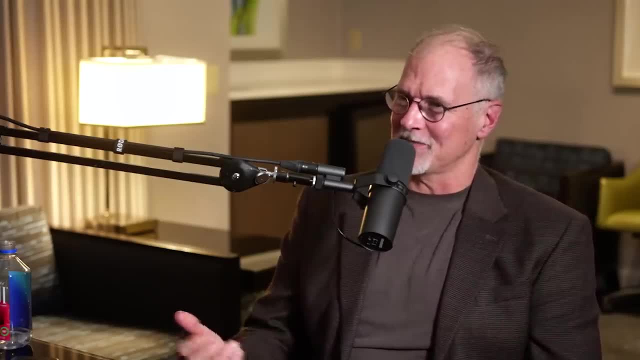 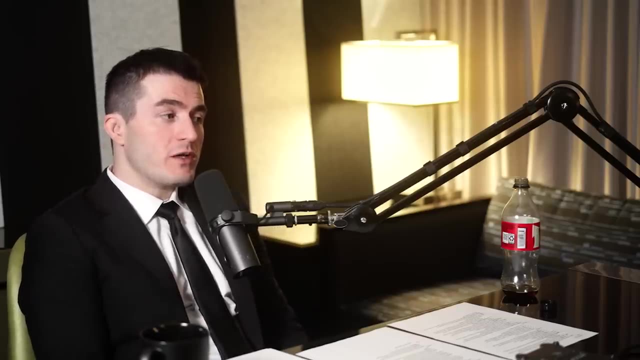 just do it. it's a machine, i, and i don't have to have qualms about that. you know the ones that are machines. i also hope to see a future- and it is hope i do have optimism about that future- where some of the robots are pets. 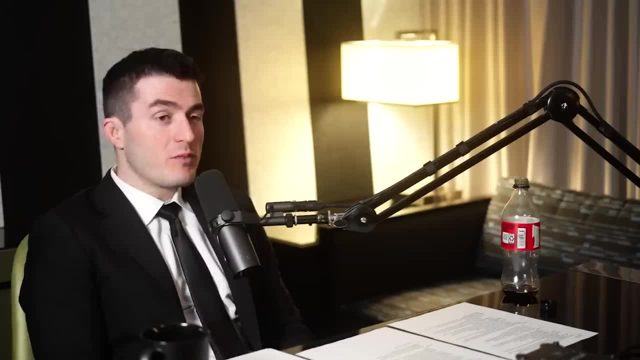 have an emotional connection to us humans and, uh, because one of the problems that humans have to solve is this kind of a general loneliness. um, the more love you have in your life, the more friends you have in your life. i think that makes a more enriching life, helps you grow, and i don't 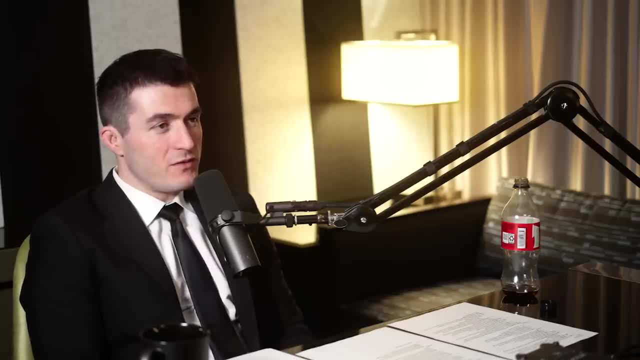 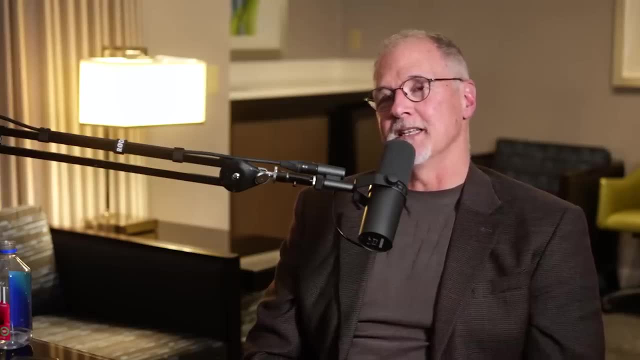 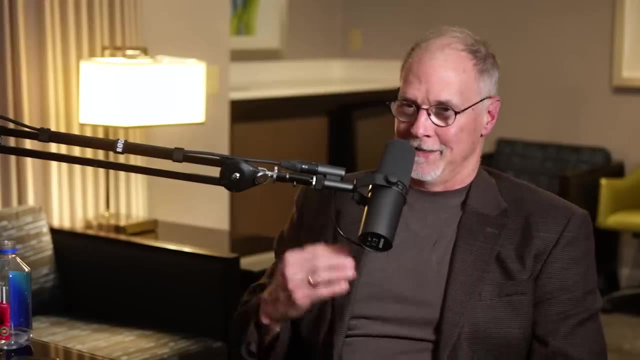 see why some of those friends can't be robots. there's an interesting long-running study- maybe it's in harvard, they just nice report article written about it recently. they've been studying this group of a few thousand people now for 70 or 80 years and the conclusion is that companionship 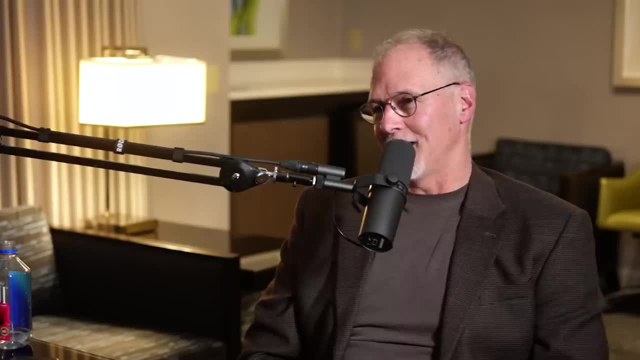 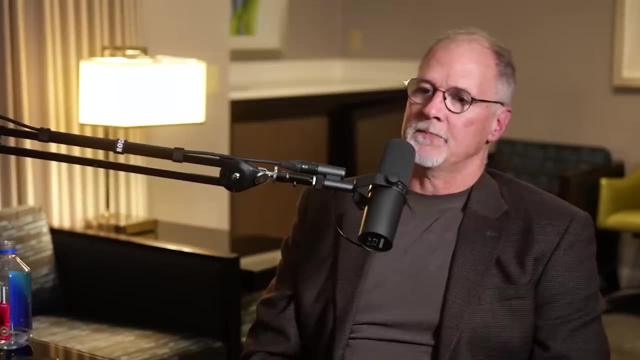 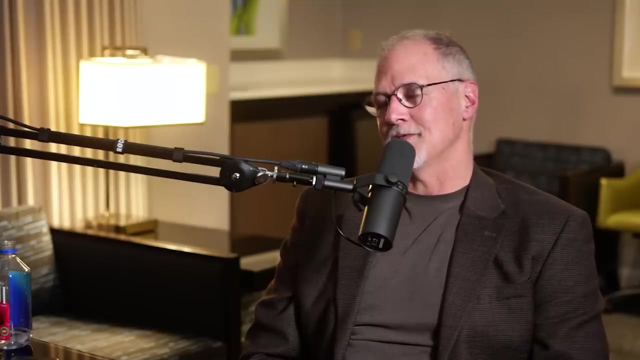 and friendship are the things that make for a better and happier life, and um so i agree with you. i think that could happen with a machine. uh, that is probably, you know, simulating intelligence. i'm not convinced there will ever be true intelligence in these machines, sentience, but they could. 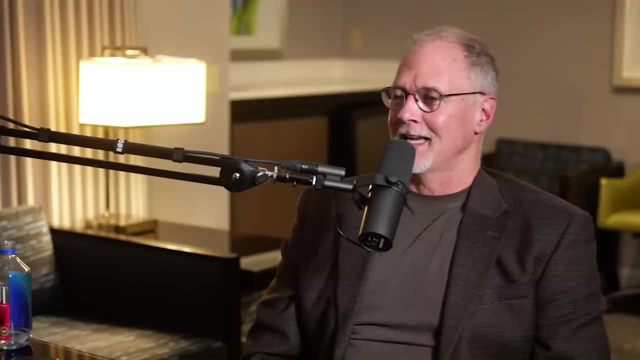 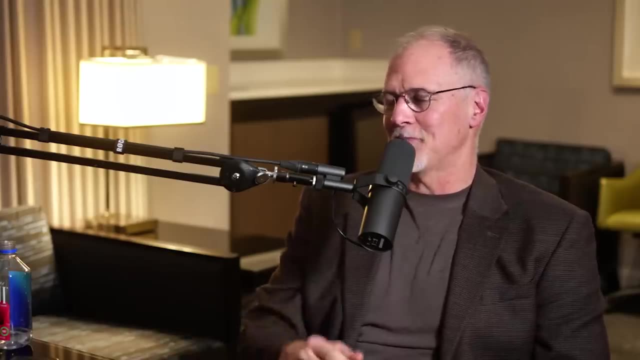 simulate it and they could collect your history and they could, you know. i guess it remains to be seen whether they can establish that real deep. you know, when you sit with a friend and they remember something about you and bring that up and you feel that connection. it remains to be seen if a